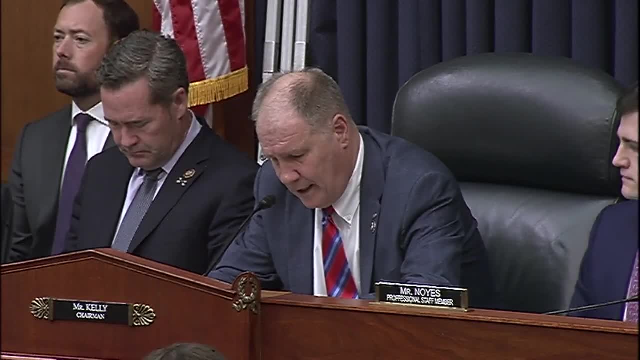 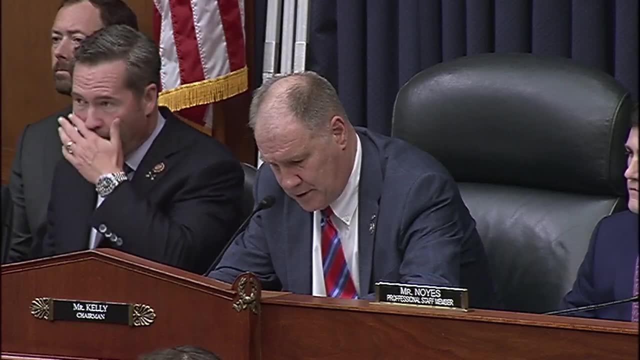 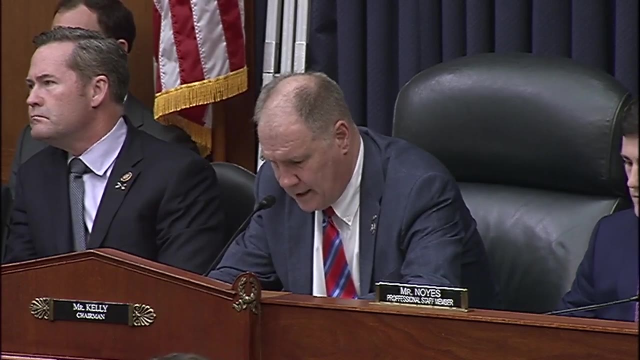 Force projection is only possible because of the sea airlift and refueling operations carried out by Transportation Command, Transcom, with support from the Marad, the Maritime Administration. Transcom and Marad support the full range of military operations, including everything from humanitarian aids to operations like those underway in the Red Sea. 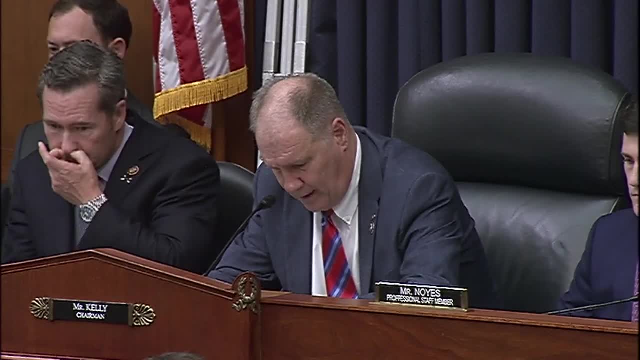 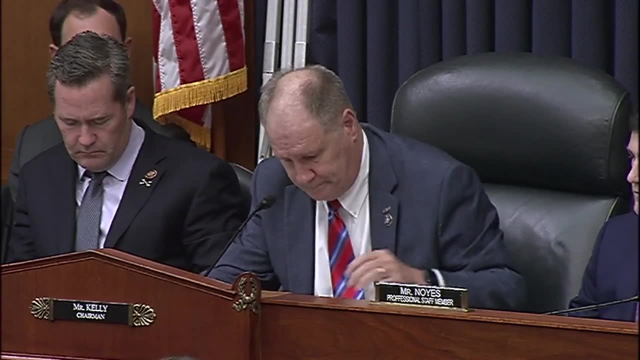 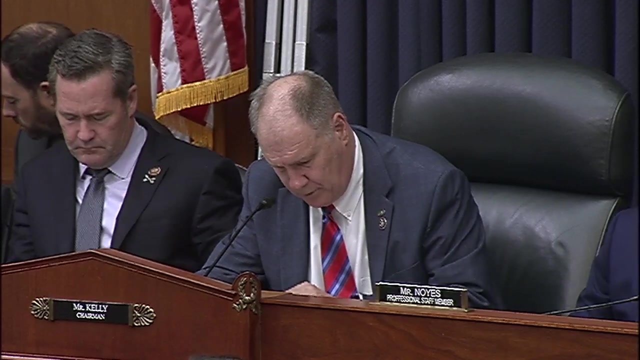 However, we cannot take our logistics capabilities for granted. We must be prepared to meet the logistic demands of a conflict against peer competitors halfway around the globe. The tyranny of distance will strain our logistics capability and we must make decisions now to meet our operational requirements for the future. 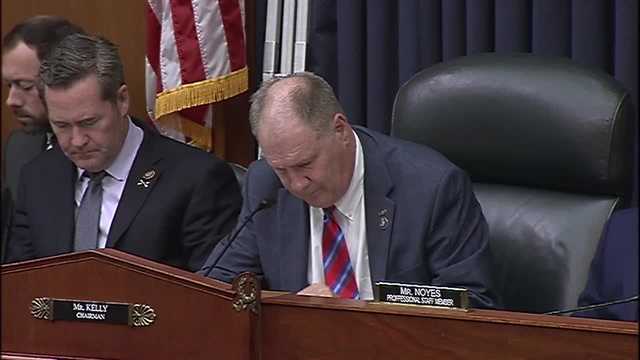 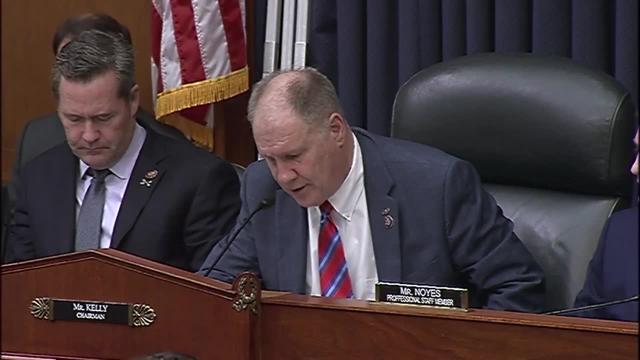 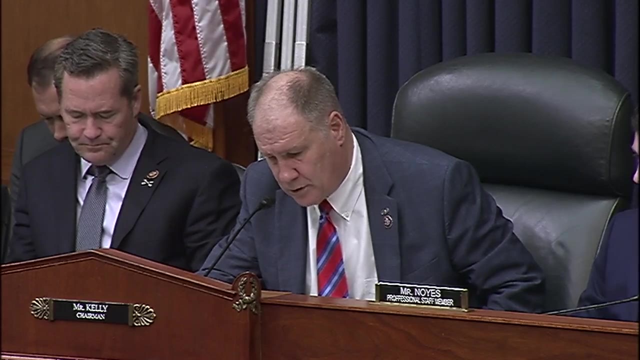 The committee has legislated several key efforts that bolster our lift capability and prevent potential backsliding. For example, Congress required a minimum of 275 inter-theater aircraft to ensure we can meet our needs for long-range aircraft, For heavier lift, we rely on commercial vehicles supported by the Maritime Security Program. 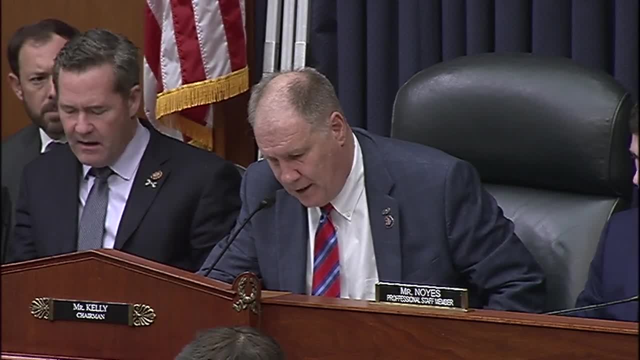 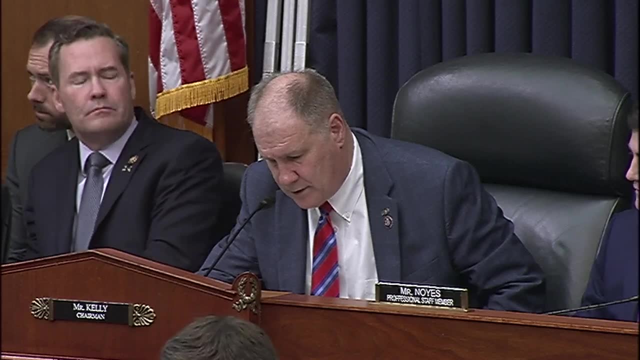 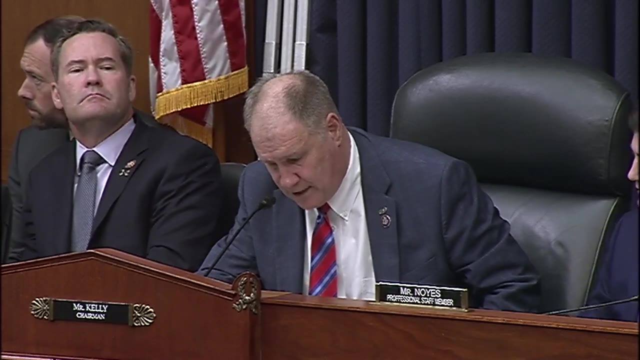 as well as an increasing airspace, We need a major aging reserve fleet to move mountains of iron and material. Sea lift recapitalization is a priority, but we need to go about it the right way. General Van Ovos, in your prepared testimony you state that the purchase of used sea lift vehicles is complementary to an effort to build new sea lift vessels. 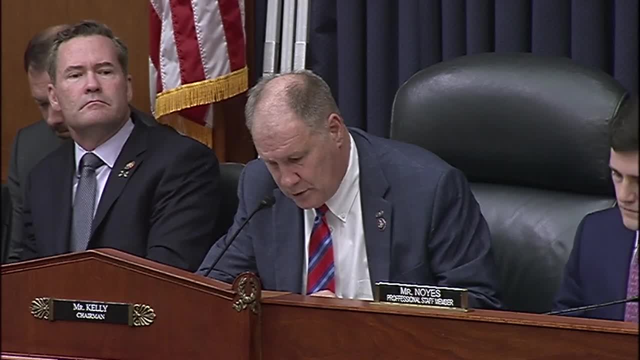 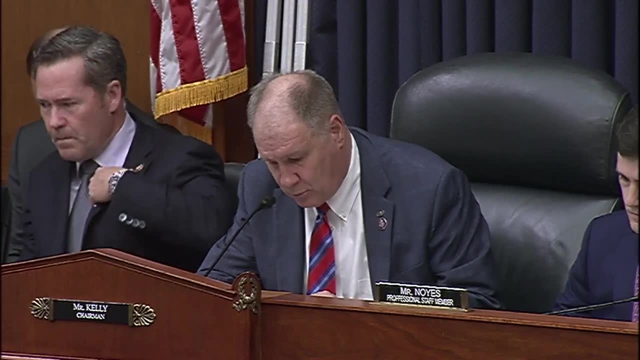 We have the Congressional intent reversed. Used personage authorities should be a complement to a new build effort. Unfortunately, years of collective feet-dragging has brought us to where we are now. I agree we need to recapitalize. I agree we need to rebuild. 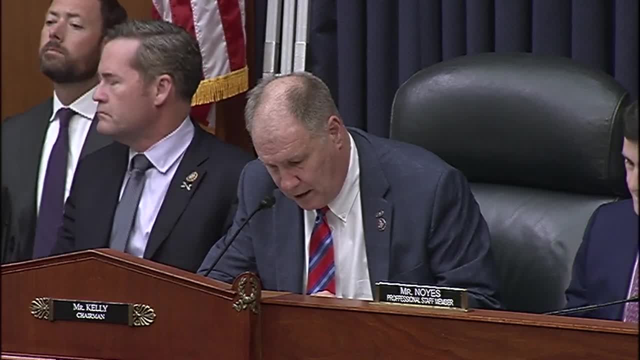 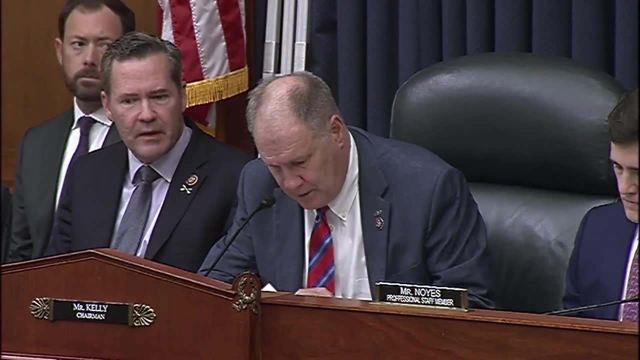 I agree we need to rebuild. I agree we need to realize the sea lift fleet, but there must be a dose of reality in the cost and availability of foreign-built 15-year-old ships that need hardened decks and retrofit. after the fact, The results of the market assessment required in last year's NDA will hopefully be informative. 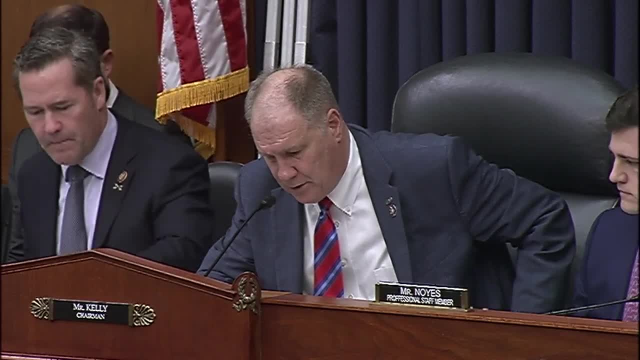 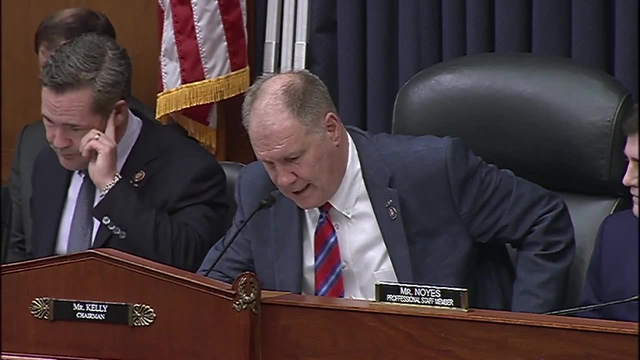 I thank our witnesses for being here today and I look forward to your testimony. I'm joined by my colleagues Ranking Member Joe Courtney, Chairman Walts and Ranking Member Garamendi today. I want to thank them for their partnership and continued leadership on these important issues before our subcommittee. 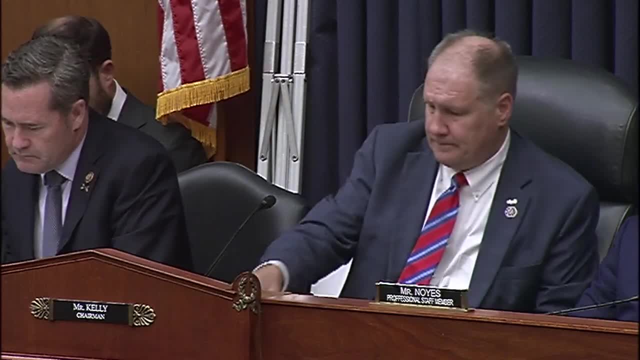 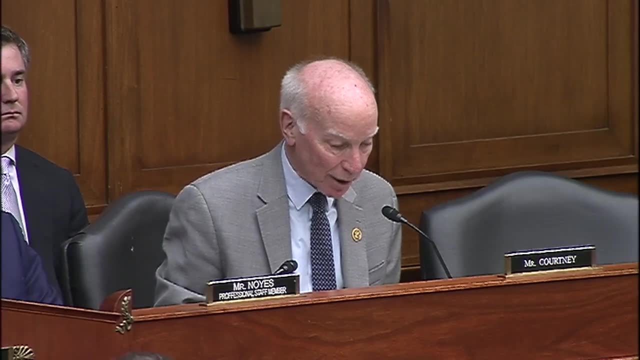 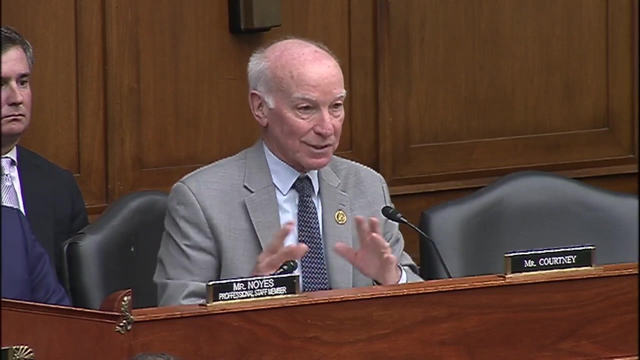 With that, I recognize Ranking Member Courtney. Thank you, Chairman Kelly, and thank you to the witnesses. Again, time is going to be tight with votes coming up, so I'll try and just truncate my remarks, But I just want to really foot-stop what Trent said. that you know, sometimes our committee seems like our focus is on, you know, Big Navy and Air Force in terms of some of these programs. 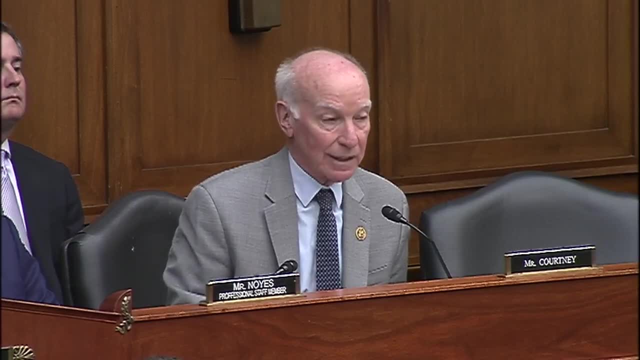 But I think I speak for both of us and really most of the committee, that your departments we view as on par with what we're doing. I think I speak for both of us and really most of the committee, that your departments we view as on par with what we're doing. 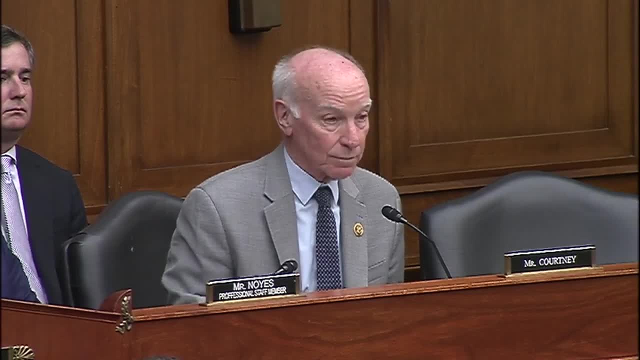 I think I speak for both of us and really most of the committee, that your departments we view as on par with what we're doing. I think I speak for both of us and really most of the committee, that your departments we view as on par with what we're doing. 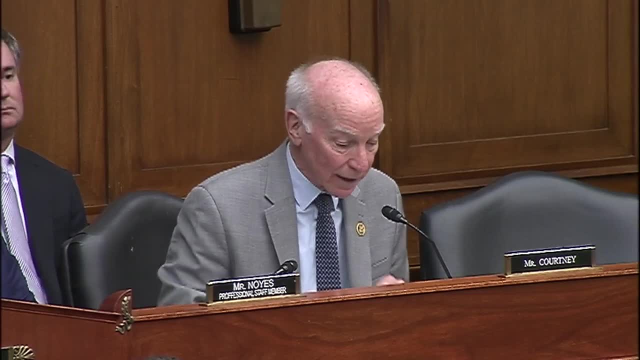 I think I speak for both of us and really most of the committee, that your departments we view as on par with what we're doing. I think I speak for both of us and really most of the committee, that your departments we view as on par with what we're doing. 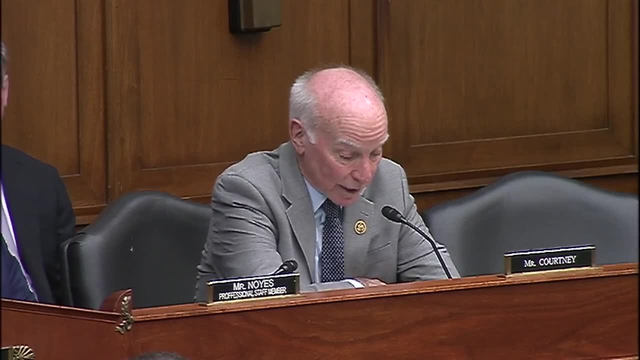 I think I speak for both of us and really most of the committee, that your departments we view as on par with what we're doing. I think I speak for both of us and really most of the committee, that your departments we view as on par with what we're doing. 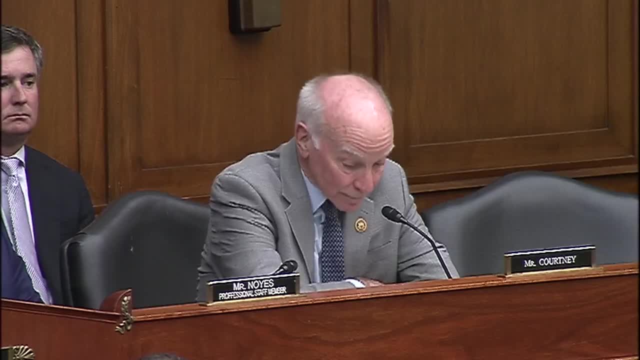 I think I speak for both of us and really most of the committee, that your departments we view as on par with what we're doing. I think I speak for both of us and really most of the committee, that your departments we view as on par with what we're doing. 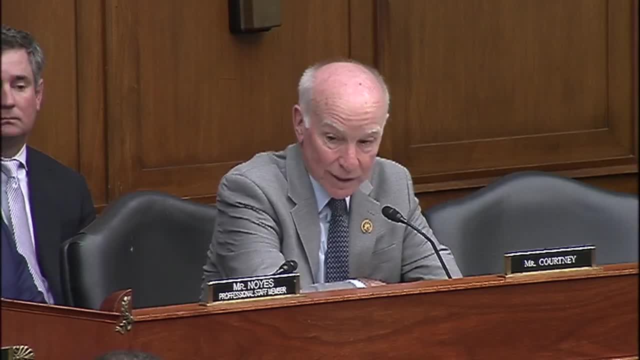 I think I speak for both of us and really most of the committee, that your departments we view as on par with what we're doing. I think I speak for both of us and really most of the committee, that your departments we view as on par with what we're doing. 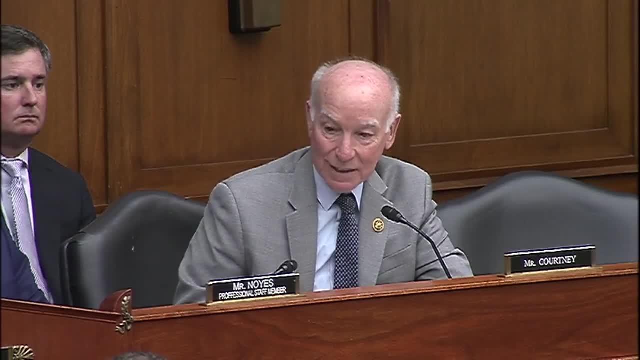 I think I speak for both of us and really most of the committee, that your departments we view as on par with what we're doing. I think I speak for both of us and really most of the committee, that your departments we view as on par with what we're doing. 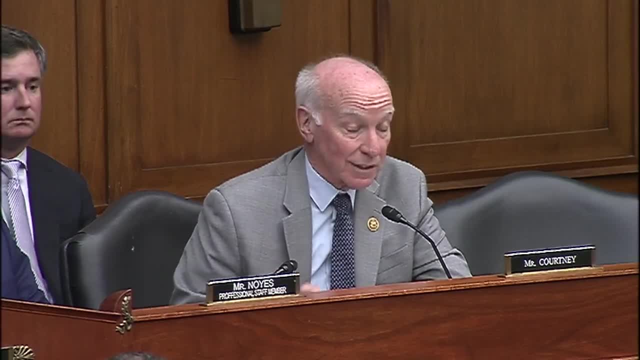 I think I speak for both of us and really most of the committee, that your departments we view as on par with what we're doing. I think I speak for both of us and really most of the committee, that your departments we view as on par with what we're doing. 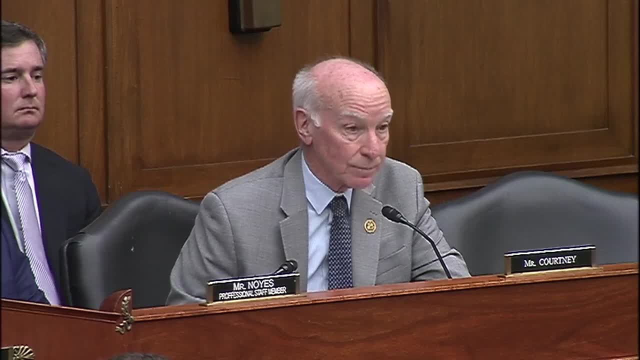 I think I speak for both of us and really most of the committee, that your departments we view as on par with what we're doing. I think I speak for both of us and really most of the committee, that your departments we view as on par with what we're doing. 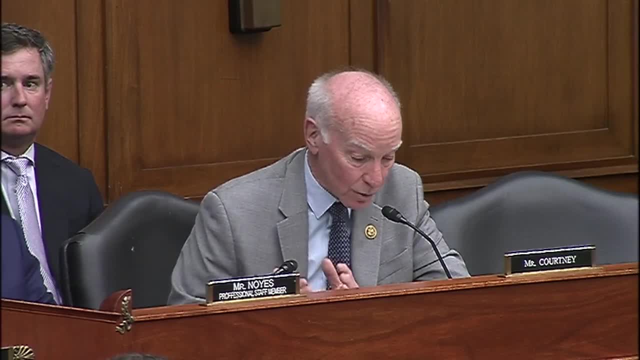 I think I speak for both of us and really most of the committee, that your departments we view as on par with what we're doing. I think I speak for both of us and really most of the committee, that your departments we view as on par with what we're doing. 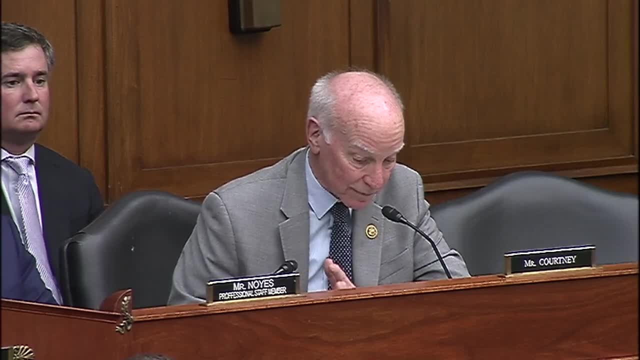 I think I speak for both of us and really most of the committee, that your departments we view as on par with what we're doing. I think I speak for both of us and really most of the committee, that your departments we view as on par with what we're doing. 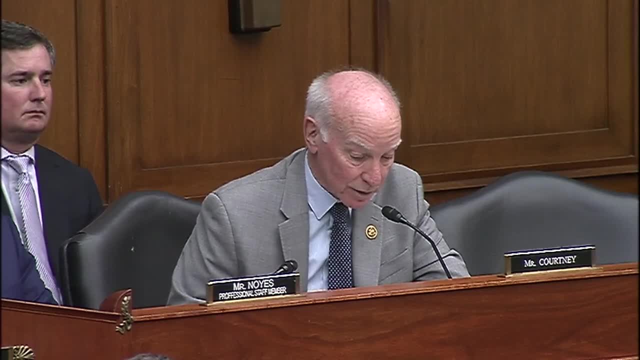 I think I speak for both of us and really most of the committee, that your departments we view as on par with what we're doing. I think I speak for both of us and really most of the committee, that your departments we view as on par with what we're doing. 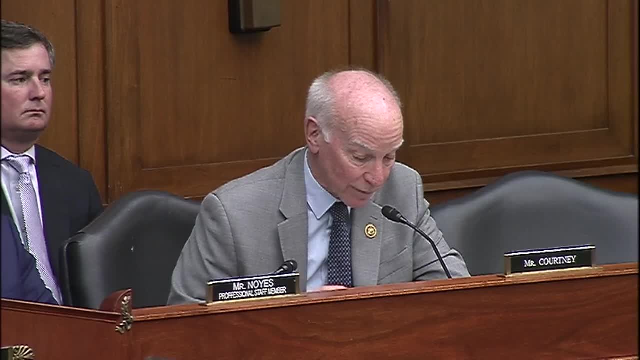 I think I speak for both of us and really most of the committee, that your departments we view as on par with what we're doing. I think I speak for both of us and really most of the committee, that your departments we view as on par with what we're doing. 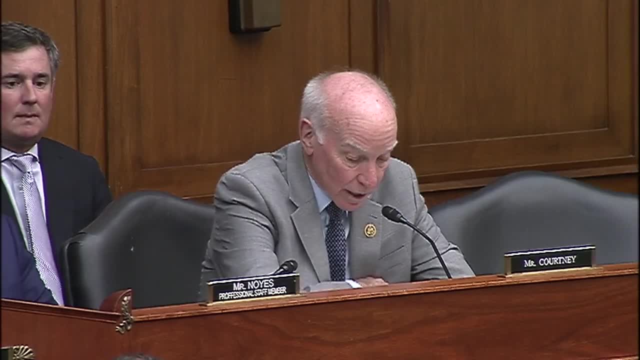 I think I speak for both of us and really most of the committee, that your departments we view as on par with what we're doing. I think I speak for both of us and really most of the committee, that your departments we view as on par with what we're doing. 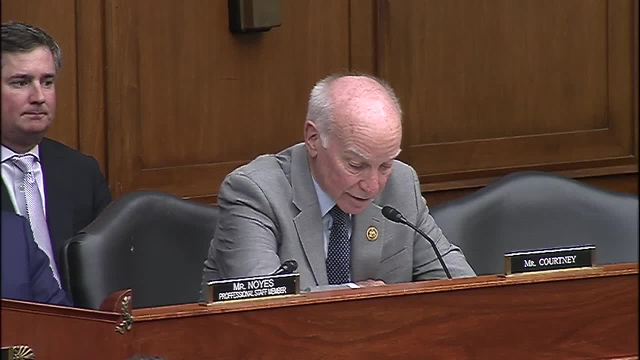 I think I speak for both of us and really most of the committee, that your departments we view as on par with what we're doing. I think I speak for both of us and really most of the committee, that your departments we view as on par with what we're doing. 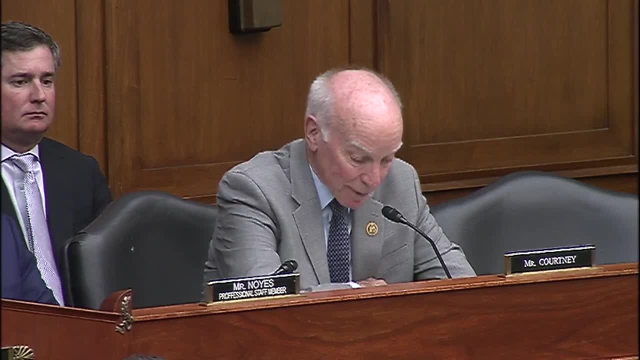 I think I speak for both of us and really most of the committee, that your departments we view as on par with what we're doing. I think I speak for both of us and really most of the committee, that your departments we view as on par with what we're doing. 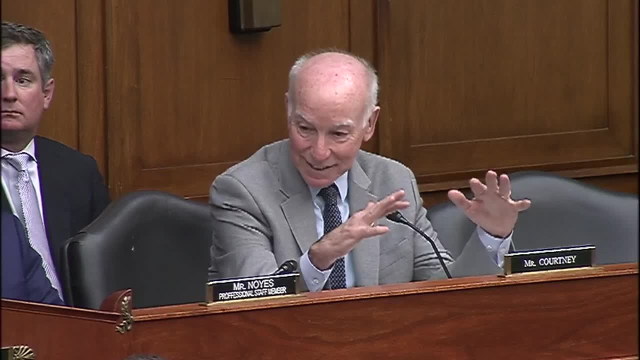 I think I speak for both of us and really most of the committee, that your departments we view as on par with what we're doing. I think I speak for both of us and really most of the committee, that your departments we view as on par with what we're doing. 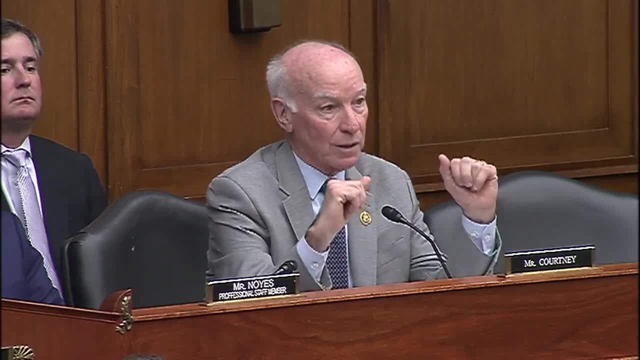 I think I speak for both of us and really most of the committee, that your departments we view as on par with what we're doing. I think I speak for both of us and really most of the committee, that your departments we view as on par with what we're doing. 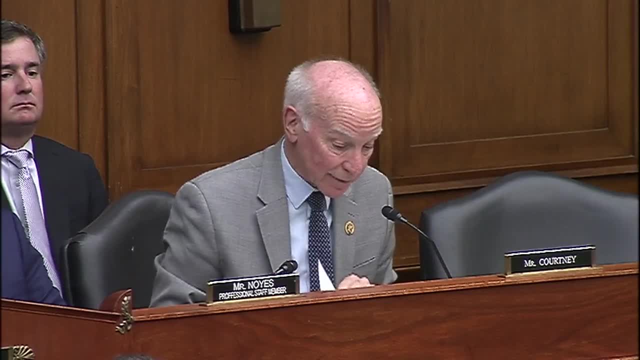 I think I speak for both of us and really most of the committee, that your departments we view as on par with what we're doing. I think I speak for both of us and really most of the committee, that your departments we view as on par with what we're doing. 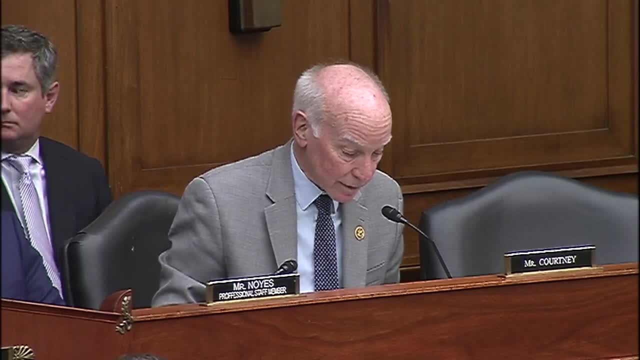 I think I speak for both of us and really most of the committee, that your departments we view as on par with what we're doing. I think I speak for both of us and really most of the committee, that your departments we view as on par with what we're doing. 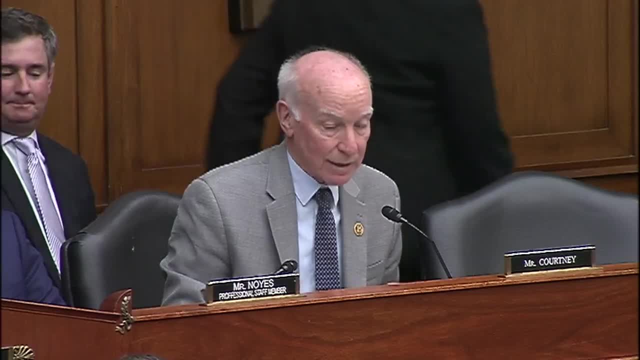 I think I speak for both of us and really most of the committee, that your departments we view as on par with what we're doing. I think I speak for both of us and really most of the committee, that your departments we view as on par with what we're doing. 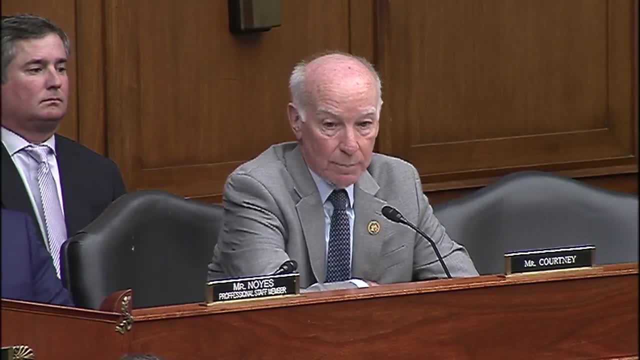 I think I speak for both of us and really most of the committee, that your departments we view as on par with what we're doing. I think I speak for both of us and really most of the committee, that your departments we view as on par with what we're doing. 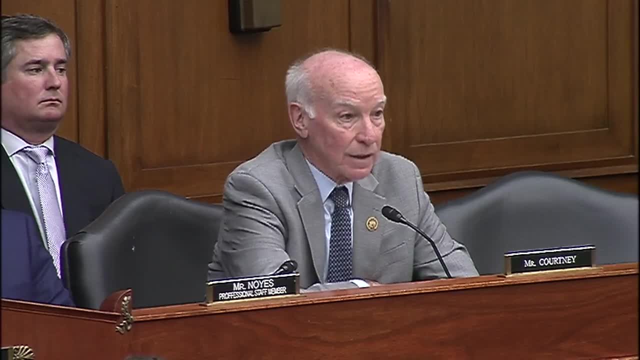 I think I speak for both of us and really most of the committee, that your departments we view as on par with what we're doing. I think I speak for both of us and really most of the committee, that your departments we view as on par with what we're doing. 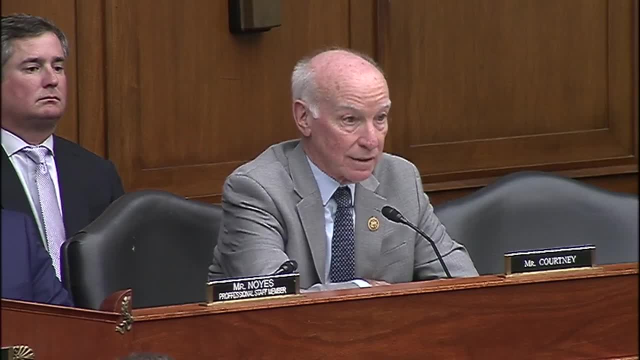 I think I speak for both of us and really most of the committee, that your departments we view as on par with what we're doing. I think I speak for both of us and really most of the committee, that your departments we view as on par with what we're doing. 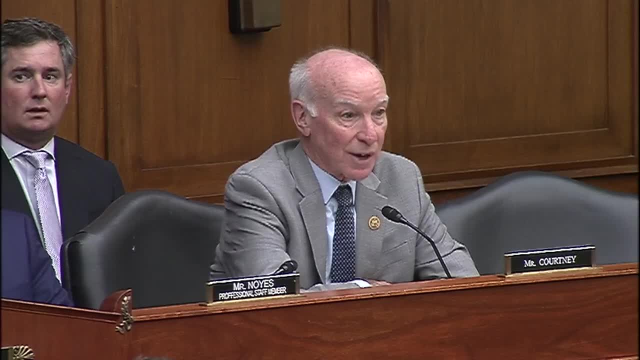 I think I speak for both of us and really most of the committee, that your departments we view as on par with what we're doing. I think I speak for both of us and really most of the committee, that your departments we view as on par with what we're doing. 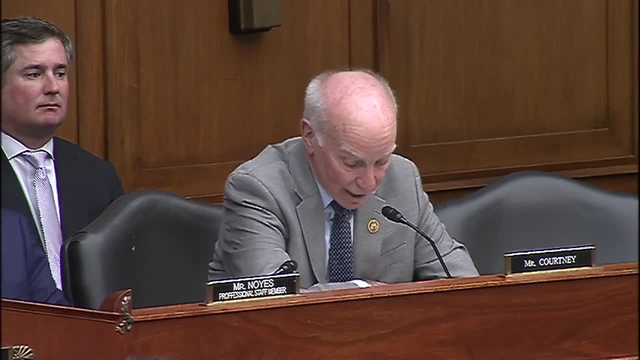 I think I speak for both of us and really most of the committee, that your departments we view as on par with what we're doing. I think I speak for both of us and really most of the committee, that your departments we view as on par with what we're doing. 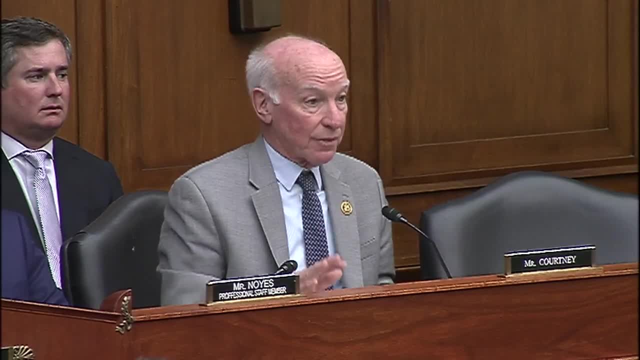 I think I speak for both of us and really most of the committee, that your departments we view as on par with what we're doing. I think I speak for both of us and really most of the committee, that your departments we view as on par with what we're doing. 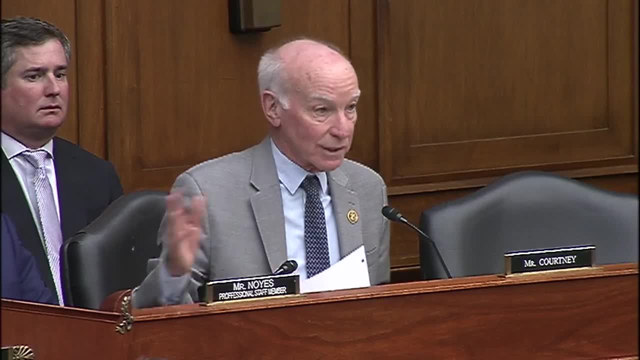 I think I speak for both of us and really most of the committee, that your departments we view as on par with what we're doing. I think I speak for both of us and really most of the committee, that your departments we view as on par with what we're doing. 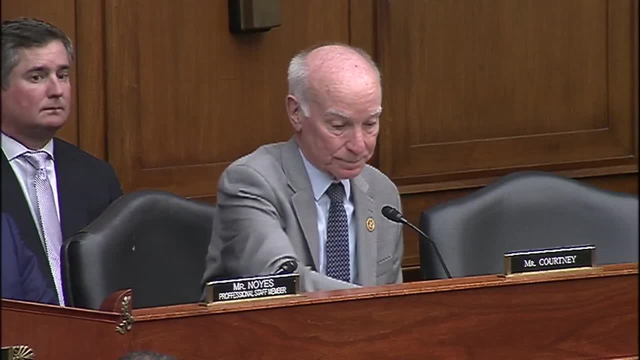 I think I speak for both of us and really most of the committee, that your departments we view as on par with what we're doing. I think I speak for both of us and really most of the committee, that your departments we view as on par with what we're doing. 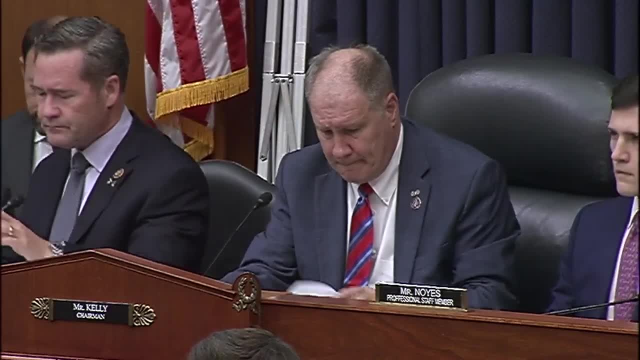 I think I speak for both of us and really most of the committee, that your departments we view as on par with what we're doing. I think I speak for both of us and really most of the committee, that your departments we view as on par with what we're doing. 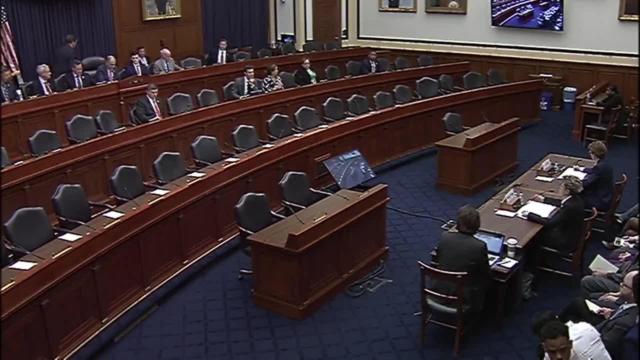 I think I speak for both of us and really most of the committee, that your departments we view as on par with what we're doing. I think I speak for both of us and really most of the committee, that your departments we view as on par with what we're doing. 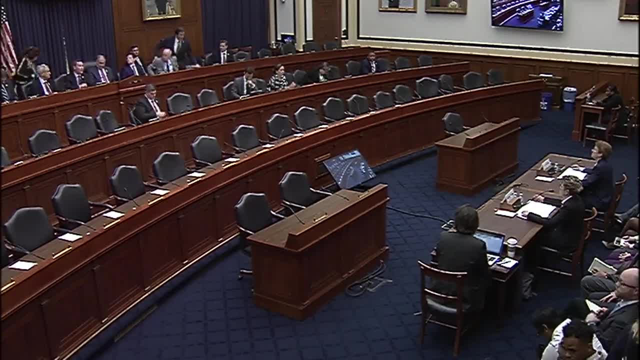 I think I speak for both of us and really most of the committee, that your departments we view as on par with what we're doing. I think I speak for both of us and really most of the committee, that your departments we view as on par with what we're doing. 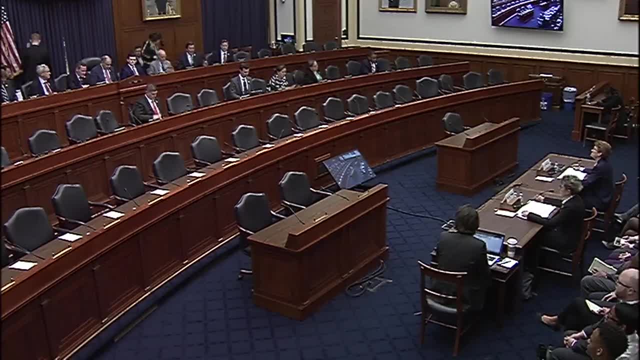 I think I speak for both of us and really most of the committee, that your departments we view as on par with what we're doing. I think I speak for both of us and really most of the committee, that your departments we view as on par with what we're doing. 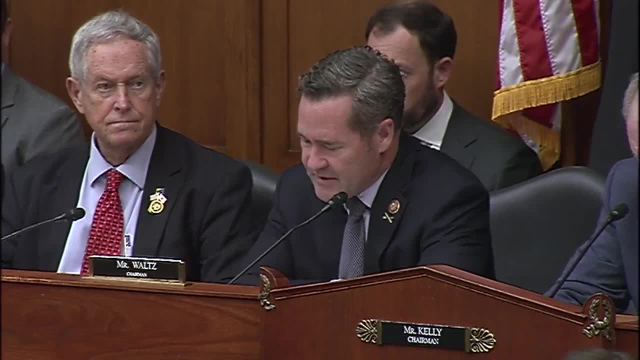 I think I speak for both of us and really most of the committee, that your departments we view as on par with what we're doing. I think I speak for both of us and really most of the committee, that your departments we view as on par with what we're doing. 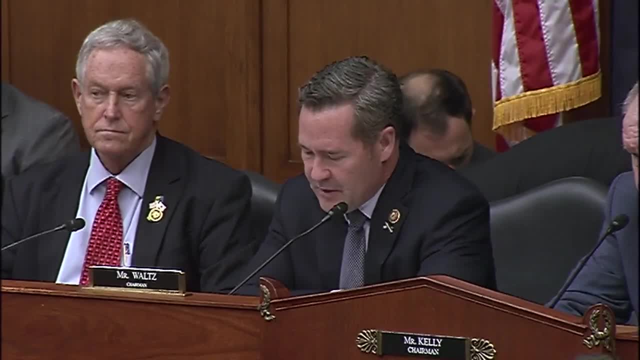 I think I speak for both of us and really most of the committee, that your departments we view as on par with what we're doing. I think I speak for both of us and really most of the committee, that your departments we view as on par with what we're doing. 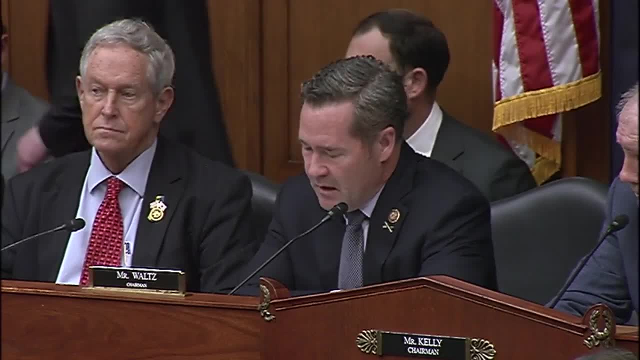 I think I speak for both of us and really most of the committee, that your departments we view as on par with what we're doing. I think I speak for both of us and really most of the committee, that your departments we view as on par with what we're doing. 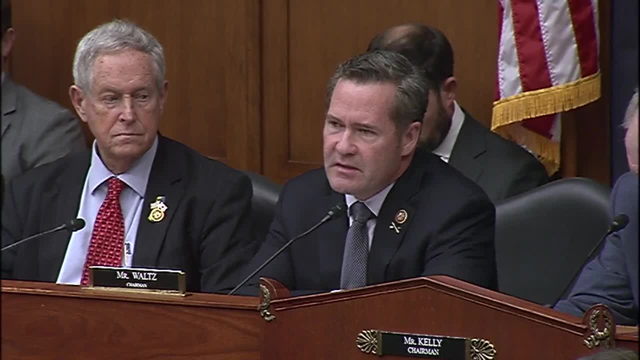 I think I speak for both of us and really most of the committee, that your departments we view as on par with what we're doing. I think I speak for both of us and really most of the committee, that your departments we view as on par with what we're doing. 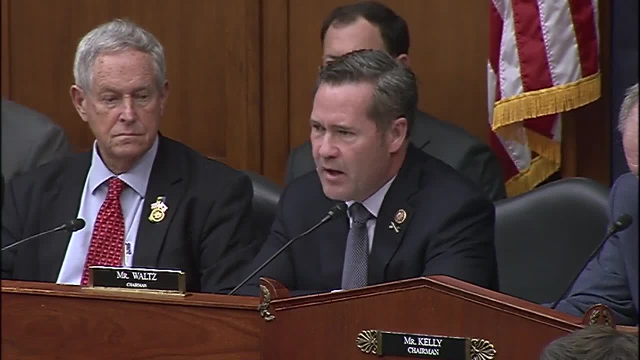 I think I speak for both of us and really most of the committee, that your departments we view as on par with what we're doing. I think I speak for both of us and really most of the committee, that your departments we view as on par with what we're doing. 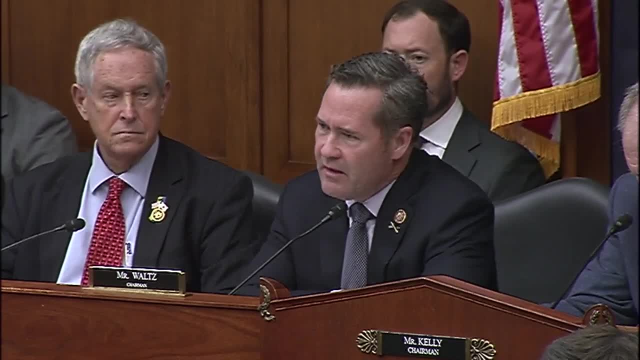 I think I speak for both of us and really most of the committee, that your departments we view as on par with what we're doing. I think I speak for both of us and really most of the committee, that your departments we view as on par with what we're doing. 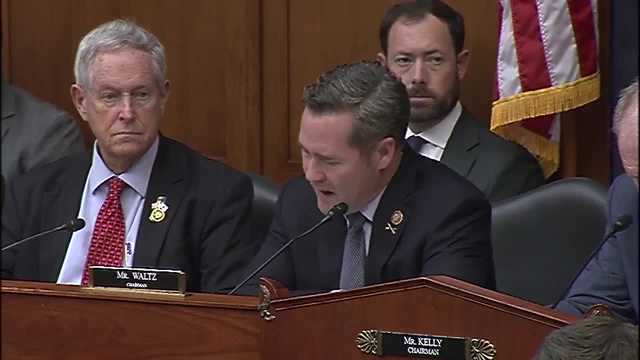 I think I speak for both of us and really most of the committee, that your departments we view as on par with what we're doing. I think I speak for both of us and really most of the committee, that your departments we view as on par with what we're doing. 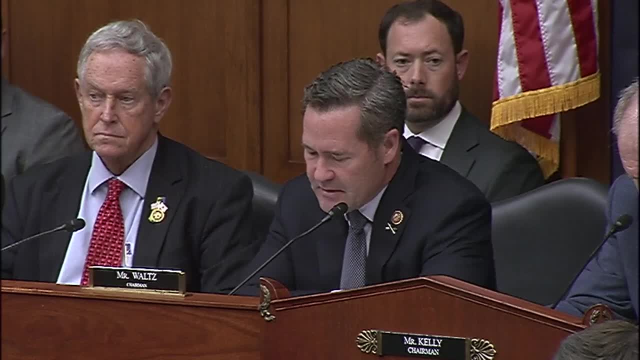 I think I speak for both of us and really most of the committee, that your departments we view as on par with what we're doing. I think I speak for both of us and really most of the committee, that your departments we view as on par with what we're doing. 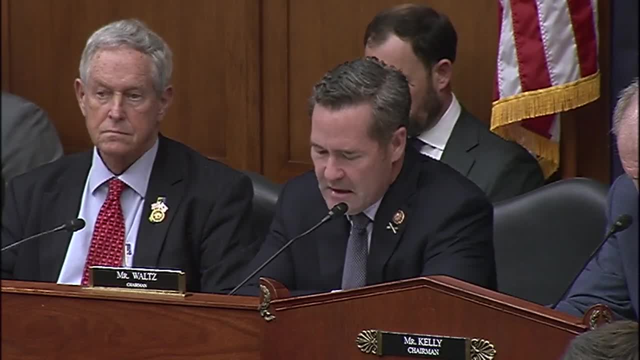 I think I speak for both of us and really most of the committee, that your departments we view as on par with what we're doing. I think I speak for both of us and really most of the committee, that your departments we view as on par with what we're doing. 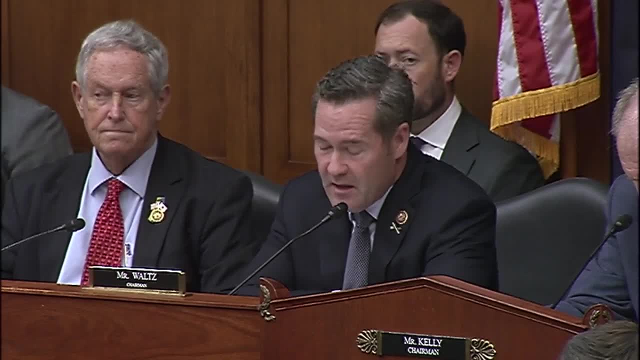 I think I speak for both of us and really most of the committee, that your departments we view as on par with what we're doing. I think I speak for both of us and really most of the committee, that your departments we view as on par with what we're doing. 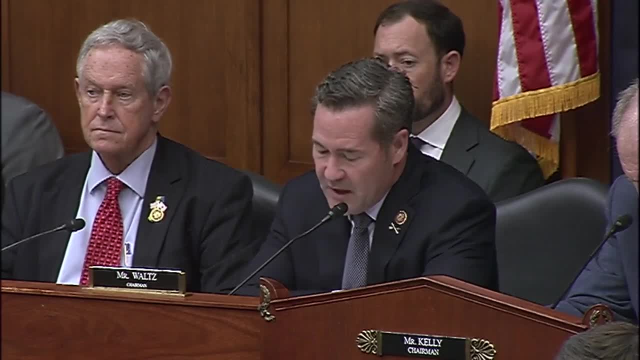 I think I speak for both of us and really most of the committee, that your departments we view as on par with what we're doing. I think I speak for both of us and really most of the committee, that your departments we view as on par with what we're doing. 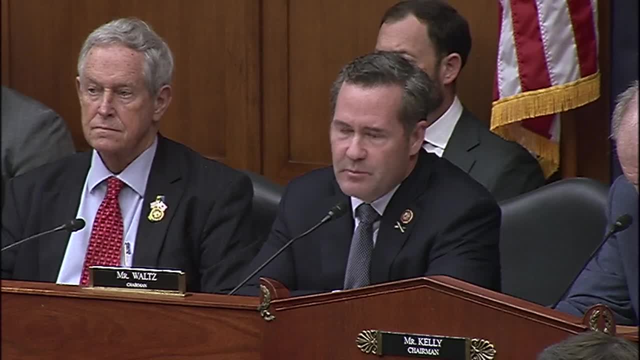 I think I speak for both of us and really most of the committee, that your departments we view as on par with what we're doing. I think I speak for both of us and really most of the committee, that your departments we view as on par with what we're doing. 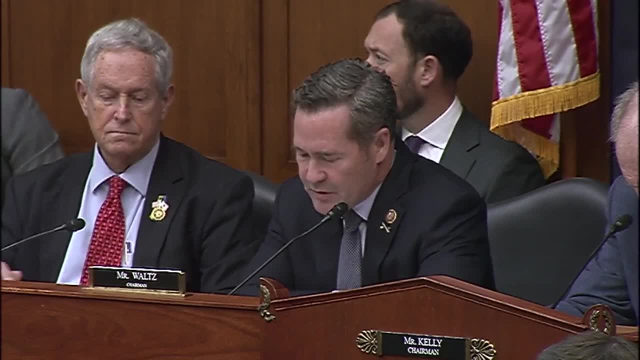 I think I speak for both of us and really most of the committee, that your departments we view as on par with what we're doing. I think I speak for both of us and really most of the committee, that your departments we view as on par with what we're doing. 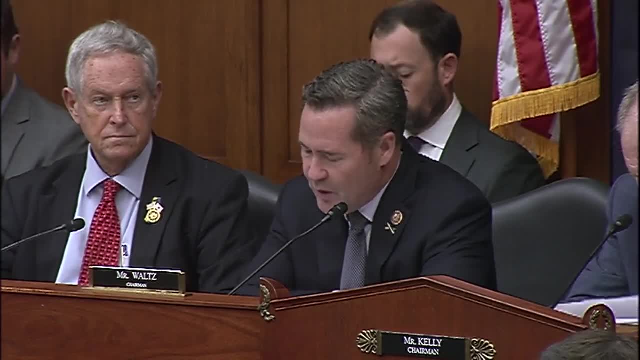 I think I speak for both of us and really most of the committee, that your departments we view as on par with what we're doing. I think I speak for both of us and really most of the committee, that your departments we view as on par with what we're doing. 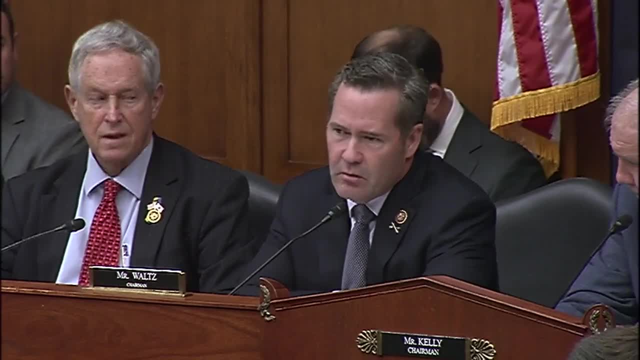 I think I speak for both of us and really most of the committee, that your departments we view as on par with what we're doing. I think I speak for both of us and really most of the committee, that your departments we view as on par with what we're doing. 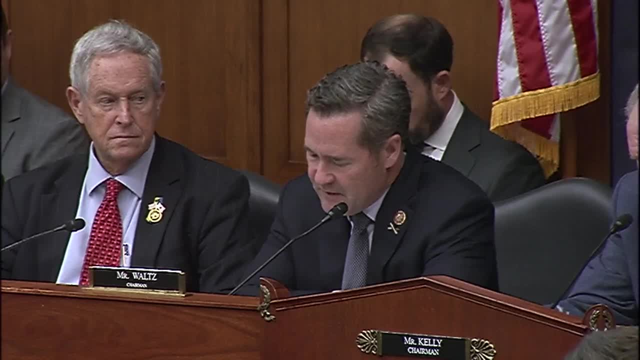 I think I speak for both of us and really most of the committee, that your departments we view as on par with what we're doing. I think I speak for both of us and really most of the committee, that your departments we view as on par with what we're doing. 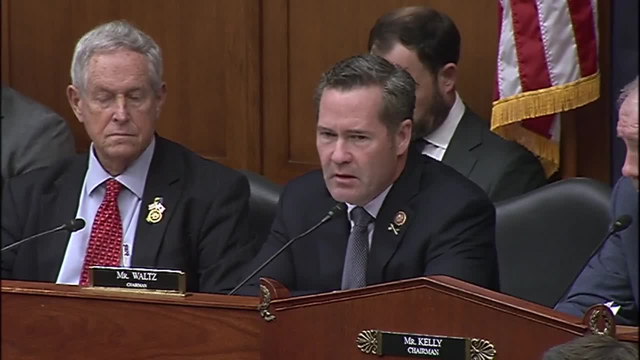 I think I speak for both of us and really most of the committee, that your departments we view as on par with what we're doing. I think I speak for both of us and really most of the committee, that your departments we view as on par with what we're doing. 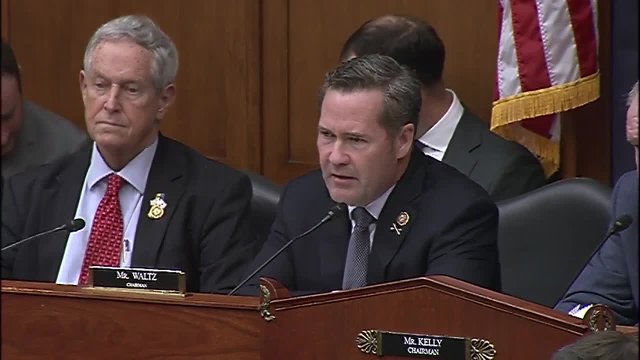 I think I speak for both of us and really most of the committee, that your departments we view as on par with what we're doing. I think I speak for both of us and really most of the committee, that your departments we view as on par with what we're doing. 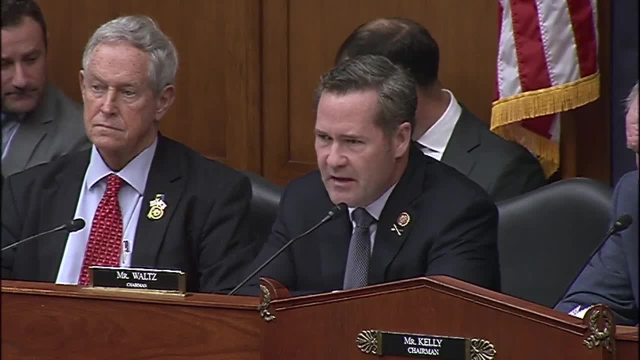 I think I speak for both of us and really most of the committee, that your departments we view as on par with what we're doing. I think I speak for both of us and really most of the committee, that your departments we view as on par with what we're doing. 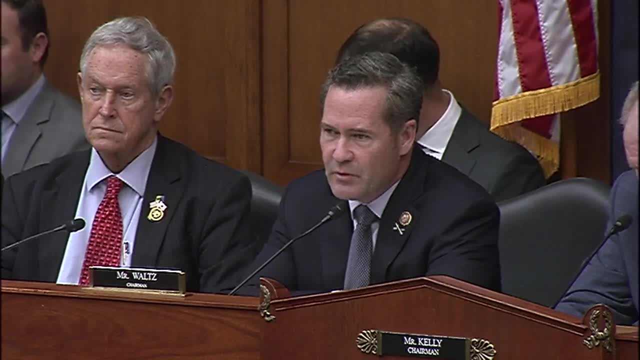 I think I speak for both of us and really most of the committee, that your departments we view as on par with what we're doing. I think I speak for both of us and really most of the committee, that your departments we view as on par with what we're doing. 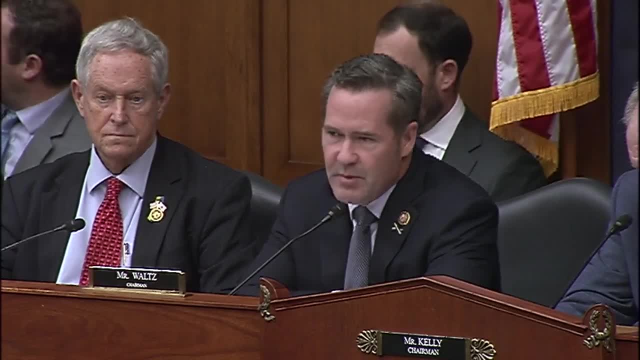 I think I speak for both of us and really most of the committee, that your departments we view as on par with what we're doing. I think I speak for both of us and really most of the committee, that your departments we view as on par with what we're doing. 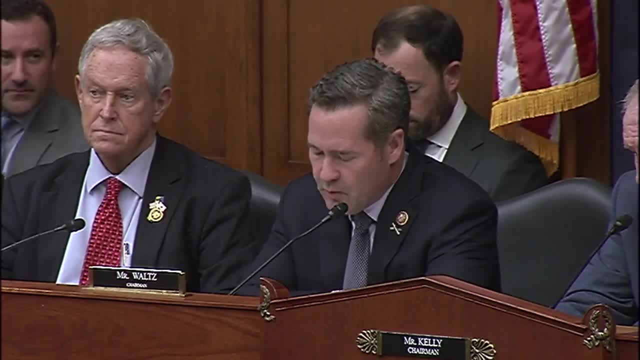 I think I speak for both of us and really most of the committee, that your departments we view as on par with what we're doing. I think I speak for both of us and really most of the committee, that your departments we view as on par with what we're doing. 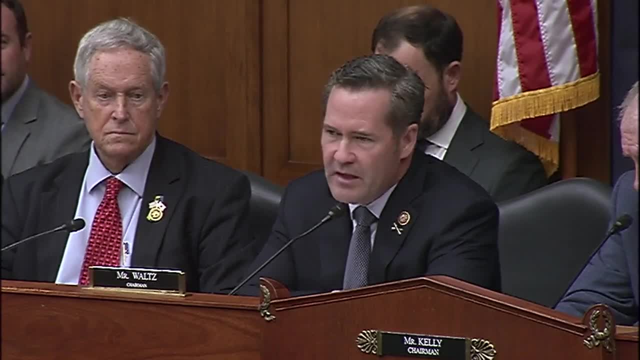 I think I speak for both of us and really most of the committee, that your departments we view as on par with what we're doing. I think I speak for both of us and really most of the committee, that your departments we view as on par with what we're doing. 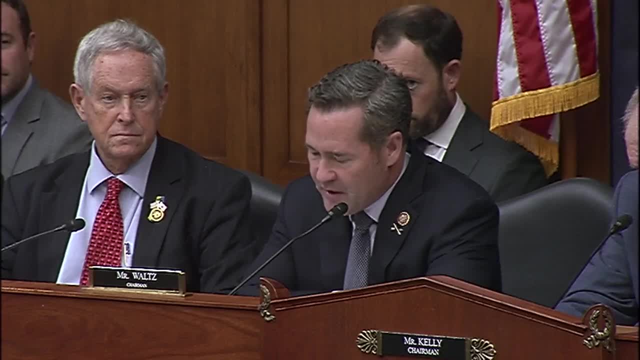 I think I speak for both of us and really most of the committee, that your departments we view as on par with what we're doing. I think I speak for both of us and really most of the committee, that your departments we view as on par with what we're doing. 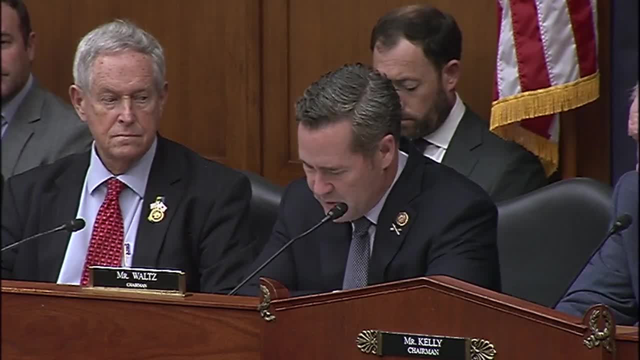 I think I speak for both of us and really most of the committee, that your departments we view as on par with what we're doing. I think I speak for both of us and really most of the committee, that your departments we view as on par with what we're doing. 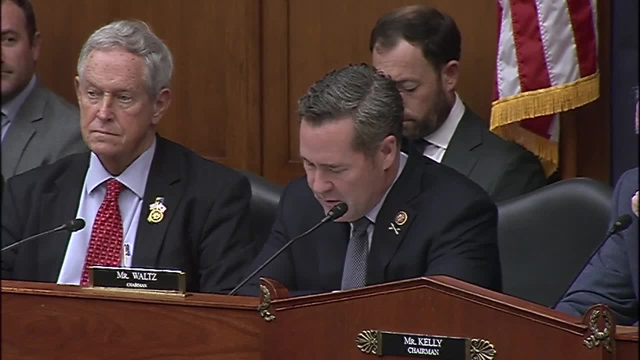 I think I speak for both of us and really most of the committee, that your departments we view as on par with what we're doing. I think I speak for both of us and really most of the committee, that your departments we view as on par with what we're doing. 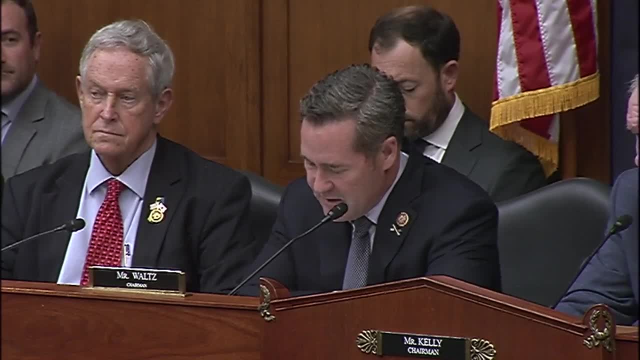 I think I speak for both of us and really most of the committee, that your departments we view as on par with what we're doing. I think I speak for both of us and really most of the committee, that your departments we view as on par with what we're doing. 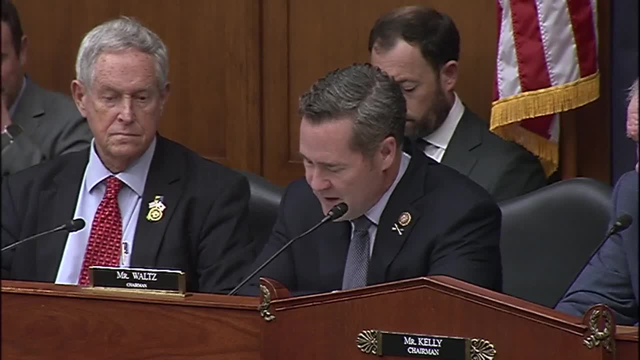 I think I speak for both of us and really most of the committee, that your departments we view as on par with what we're doing. I think I speak for both of us and really most of the committee, that your departments we view as on par with what we're doing. 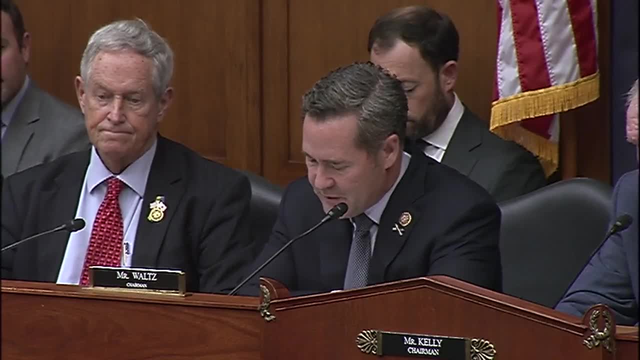 I think I speak for both of us and really most of the committee, that your departments we view as on par with what we're doing. I think I speak for both of us and really most of the committee, that your departments we view as on par with what we're doing. 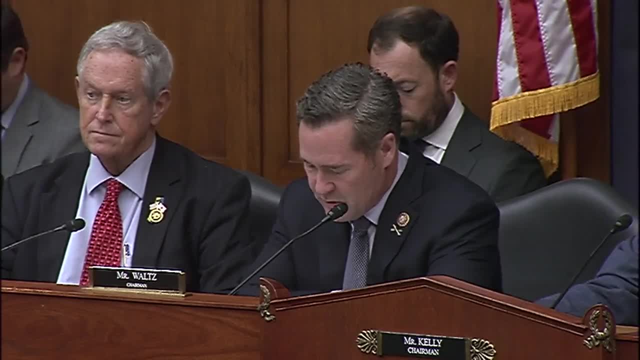 I think I speak for both of us and really most of the committee, that your departments we view as on par with what we're doing. I think I speak for both of us and really most of the committee, that your departments we view as on par with what we're doing. 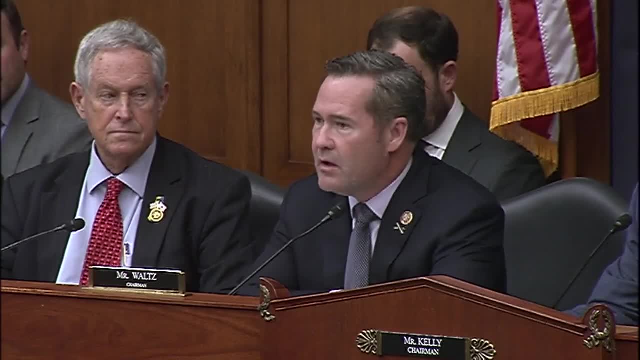 I think I speak for both of us and really most of the committee, that your departments we view as on par with what we're doing. I think I speak for both of us and really most of the committee, that your departments we view as on par with what we're doing. 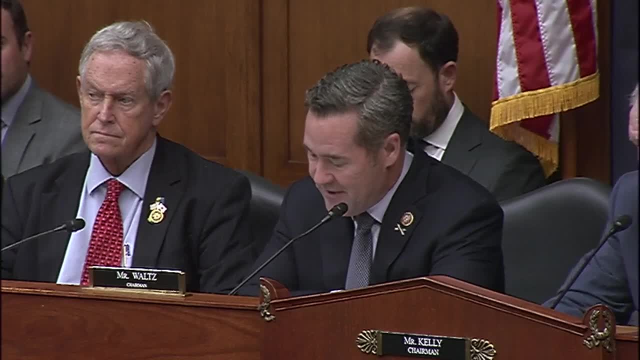 I think I speak for both of us and really most of the committee, that your departments we view as on par with what we're doing. I think I speak for both of us and really most of the committee, that your departments we view as on par with what we're doing. 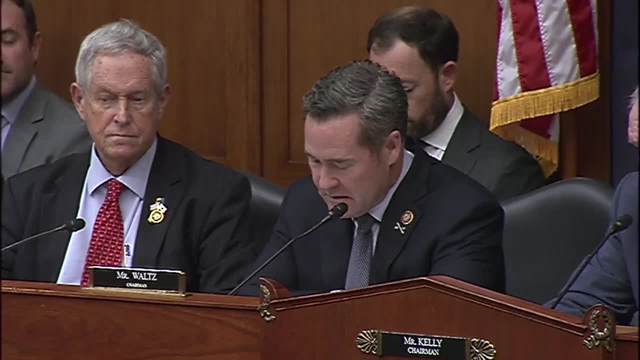 I think I speak for both of us and really most of the committee, that your departments we view as on par with what we're doing. I think I speak for both of us and really most of the committee, that your departments we view as on par with what we're doing. 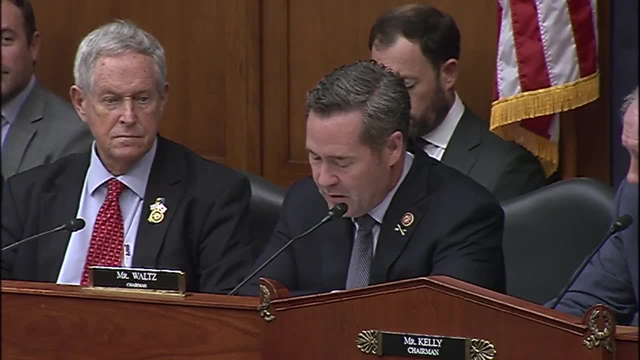 I think I speak for both of us and really most of the committee, that your departments we view as on par with what we're doing. I think I speak for both of us and really most of the committee, that your departments we view as on par with what we're doing. 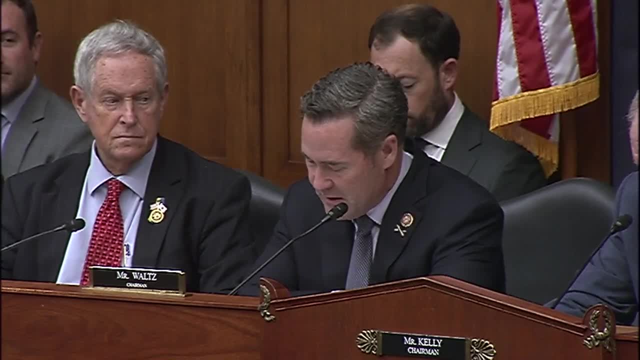 I think I speak for both of us and really most of the committee, that your departments we view as on par with what we're doing. I think I speak for both of us and really most of the committee, that your departments we view as on par with what we're doing. 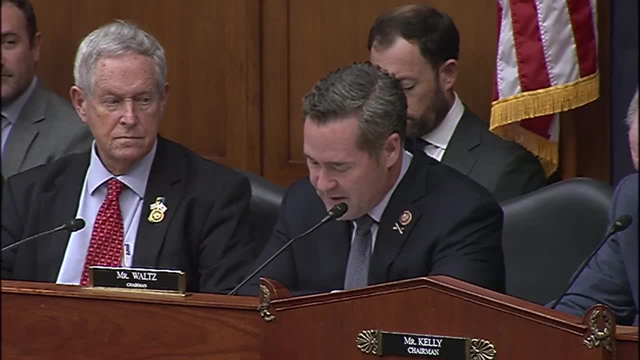 I think I speak for both of us and really most of the committee, that your departments we view as on par with what we're doing. I think I speak for both of us and really most of the committee, that your departments we view as on par with what we're doing. 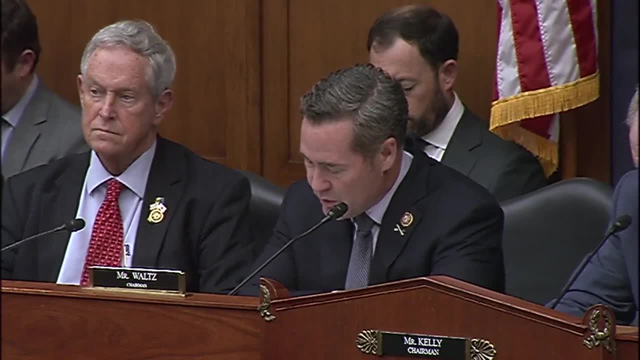 I think I speak for both of us and really most of the committee, that your departments we view as on par with what we're doing. I think I speak for both of us and really most of the committee, that your departments we view as on par with what we're doing. 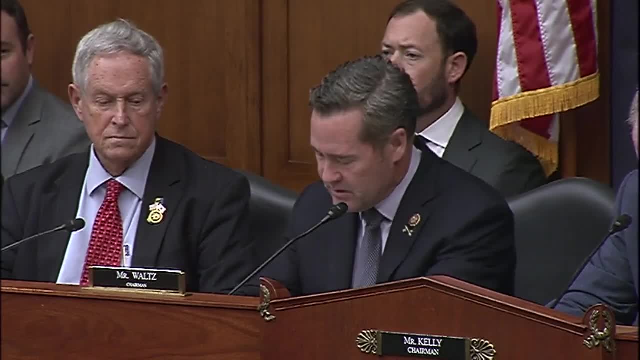 I think I speak for both of us and really most of the committee, that your departments we view as on par with what we're doing. I think I speak for both of us and really most of the committee, that your departments we view as on par with what we're doing. 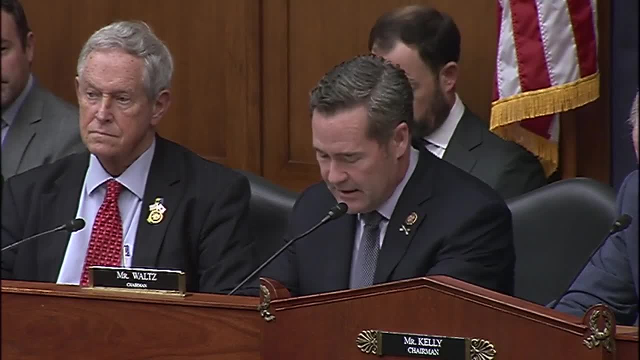 I think I speak for both of us and really most of the committee, that your departments we view as on par with what we're doing. I think I speak for both of us and really most of the committee, that your departments we view as on par with what we're doing. 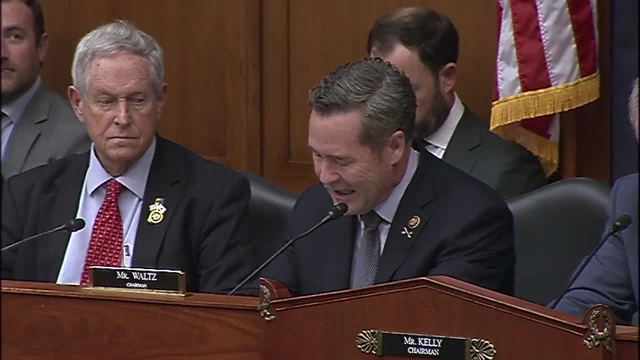 I think I speak for both of us and really most of the committee, that your departments we view as on par with what we're doing. I think I speak for both of us and really most of the committee, that your departments we view as on par with what we're doing. 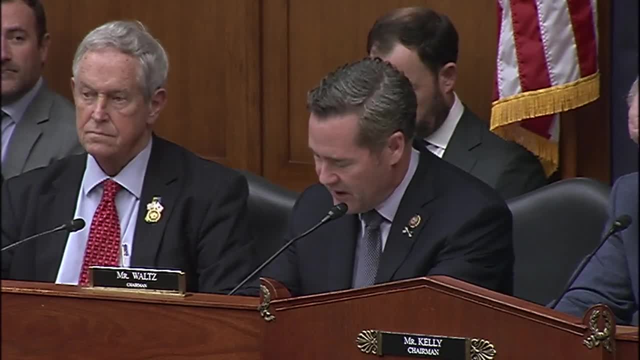 I think I speak for both of us and really most of the committee, that your departments we view as on par with what we're doing. I think I speak for both of us and really most of the committee, that your departments we view as on par with what we're doing. 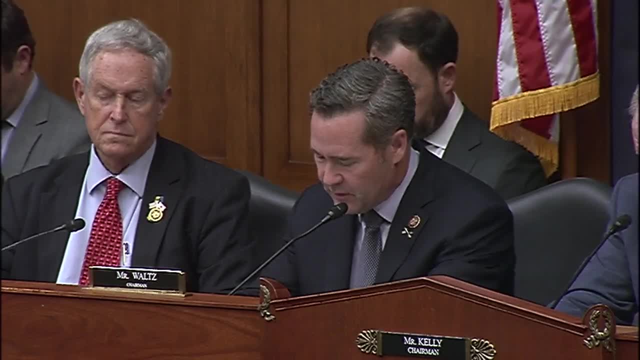 I think I speak for both of us and really most of the committee, that your departments we view as on par with what we're doing. I think I speak for both of us and really most of the committee, that your departments we view as on par with what we're doing. 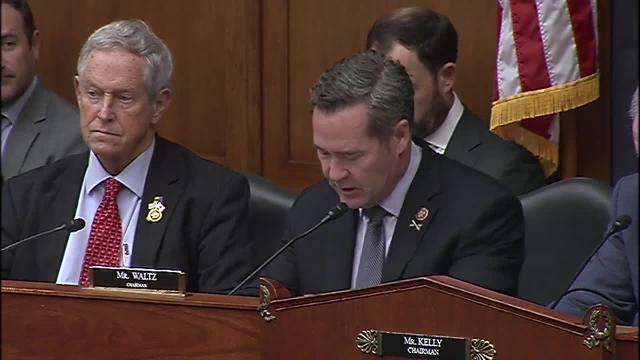 I think I speak for both of us and really most of the committee, that your departments we view as on par with what we're doing. I think I speak for both of us and really most of the committee, that your departments we view as on par with what we're doing. 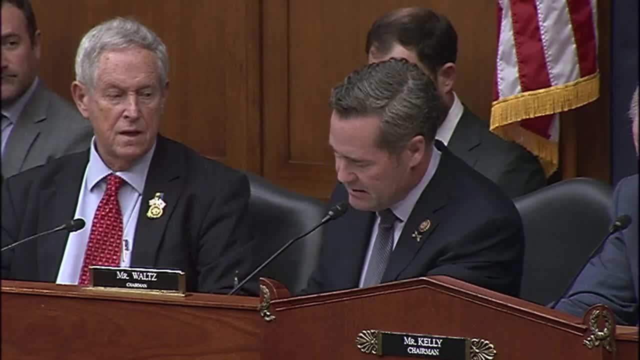 I think I speak for both of us and really most of the committee, that your departments we view as on par with what we're doing. I think I speak for both of us and really most of the committee, that your departments we view as on par with what we're doing. 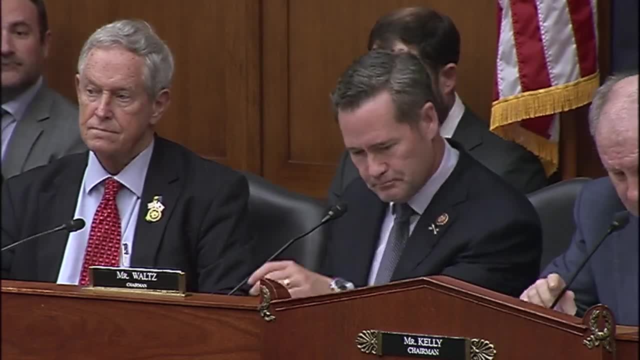 I think I speak for both of us and really most of the committee, that your departments we view as on par with what we're doing. I think I speak for both of us and really most of the committee, that your departments we view as on par with what we're doing. 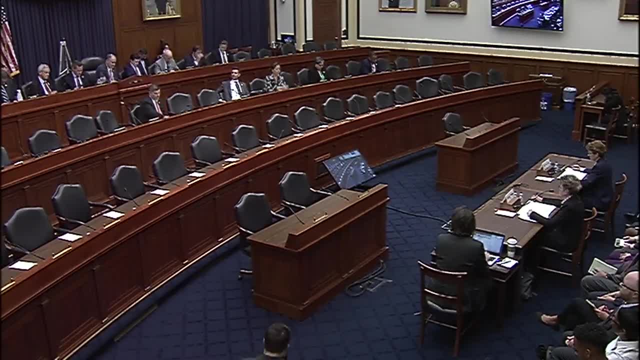 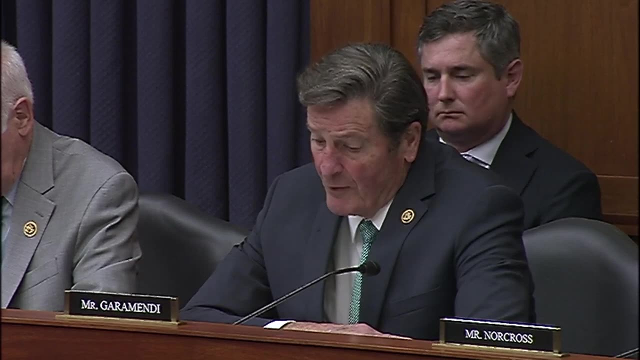 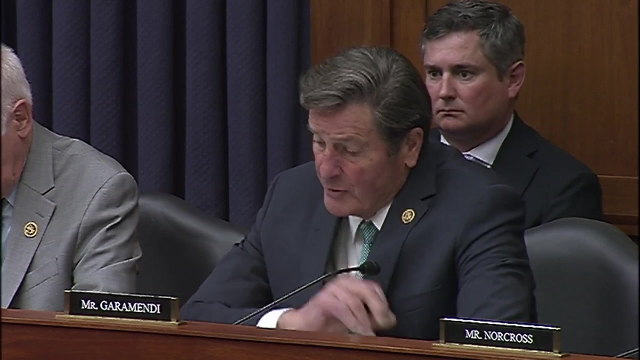 Thank you. Thank you, Gut 363.. Thank you, Thank you, Look who's here. Thank you for joining us today, Obviously very important. I want to start thanking both of you for the leadership. I'm proud to represent the district with some of our nation's most vital assets. 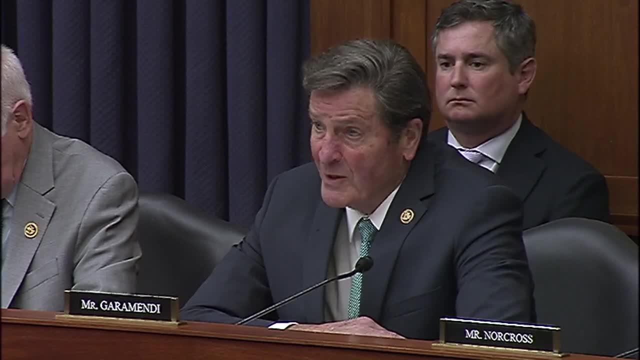 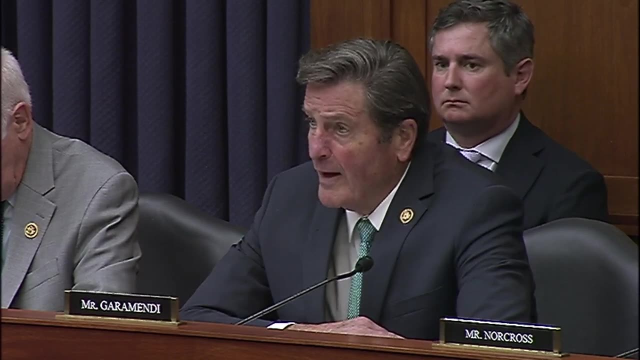 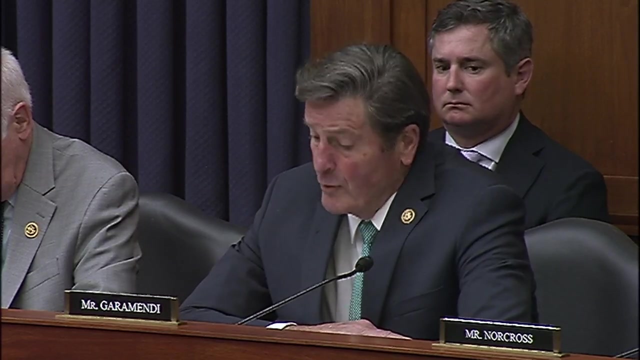 And we also have Mare Island and Matco and a few other key assets in my district that are essential for our presence and activities in the Pacific. And, General Van Oost, thank you for recognizing and providing in your testimony the critical importance of Matco. 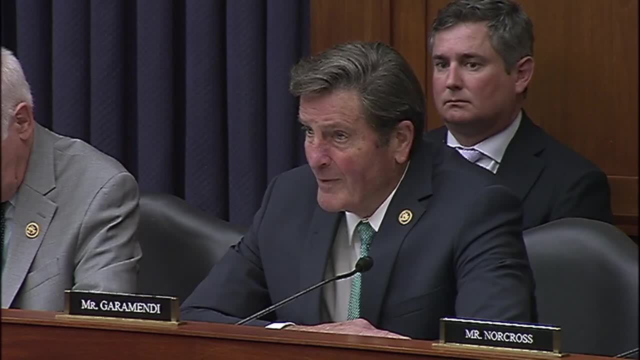 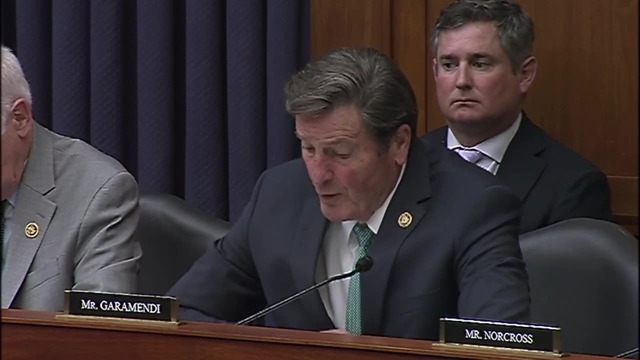 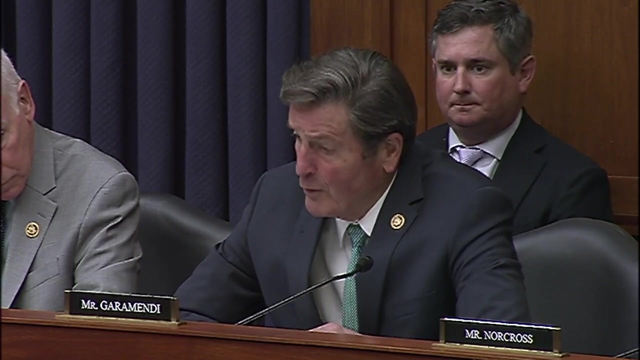 By the way, there's a hill overlooking Matco that's going to be developed. You may want to purchase an easement and prevent that development from going forward. Let's talk about air mobility. I remain concerned with the low readiness levels of the air refueling fleets. 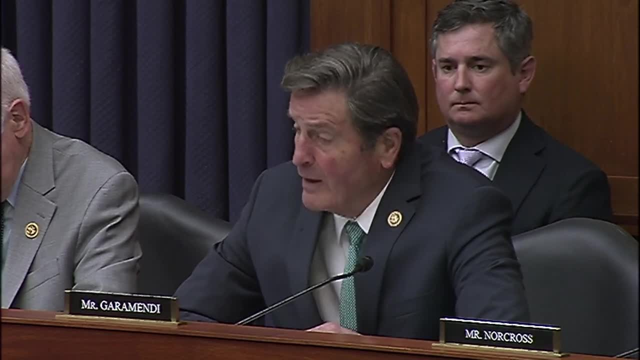 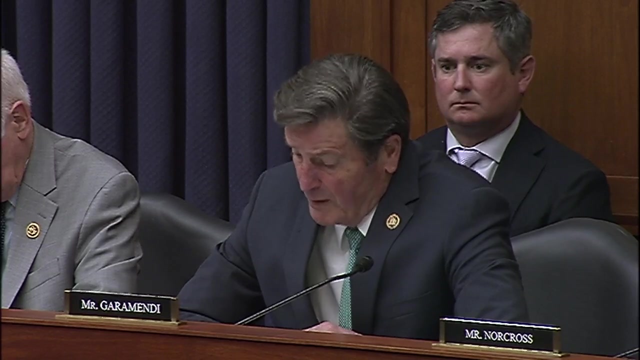 This, combined with the sunsetting of the KC-10 and the unresolved issues of the KC-46, increased the concerns. Unfortunately, we continue to accept operational risks for the KC-46 program, Notably deficiencies that threaten the already low readiness levels of the airframes. 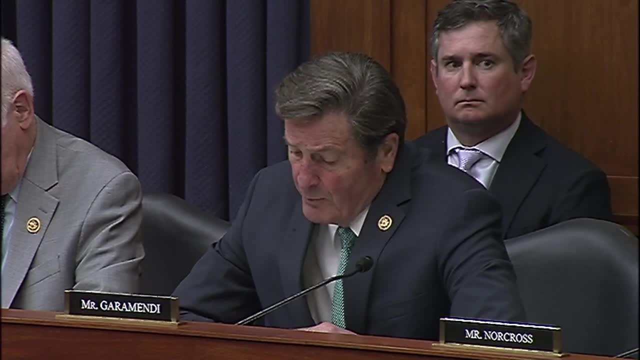 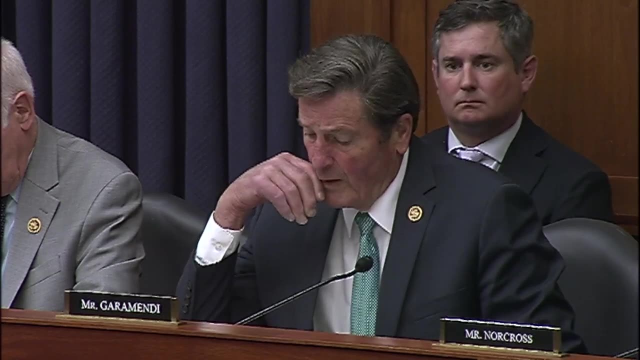 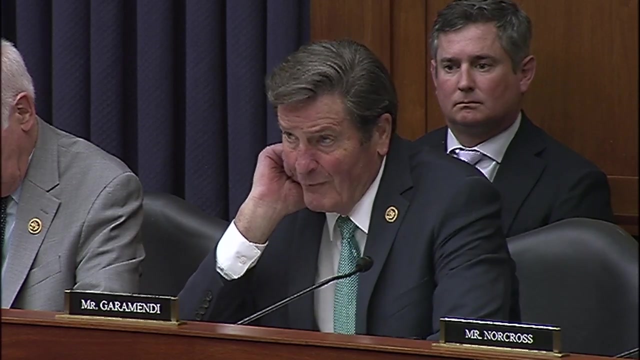 Transcom, you're going to have to ensure that, given the unresolved issues of the 46, we're not divesting at a rate which exposes the US to unacceptable air refueling risks. Speaking of unacceptable risks, our mobility fleets have been operating without connectivity for decades. 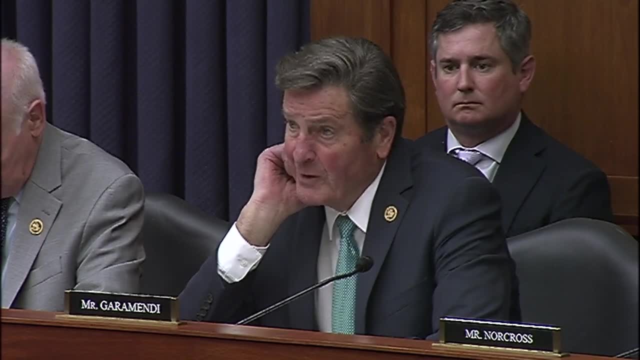 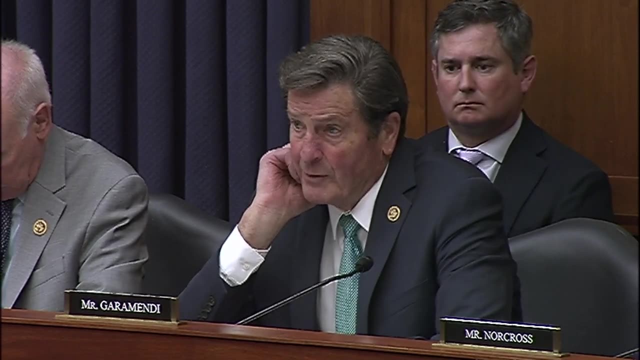 We've talked about this. I guess people that don't- People that don't fly in these planes- really don't care much about it. but if you're in one of these airplanes, you basically don't know what's going on around you and you are at great risk. 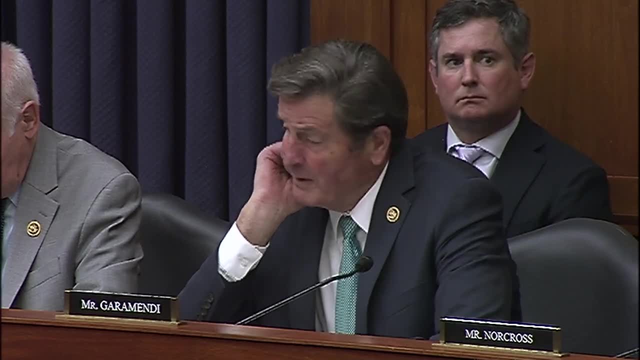 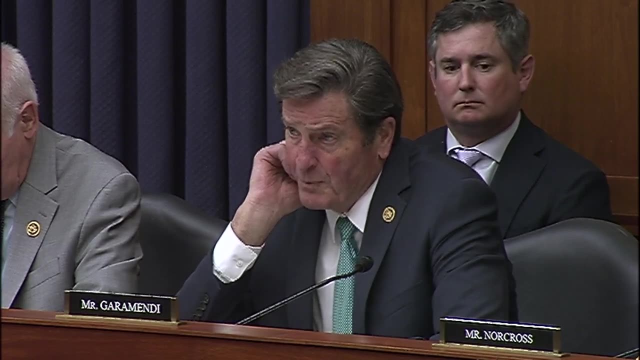 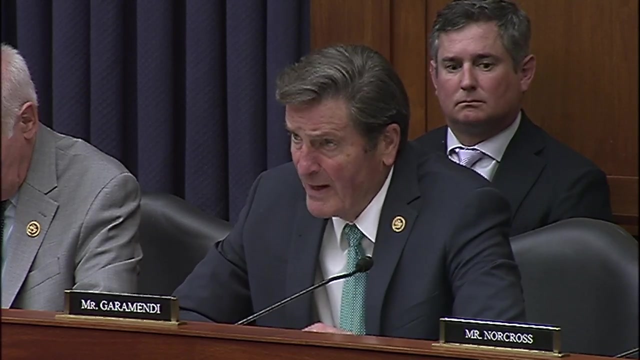 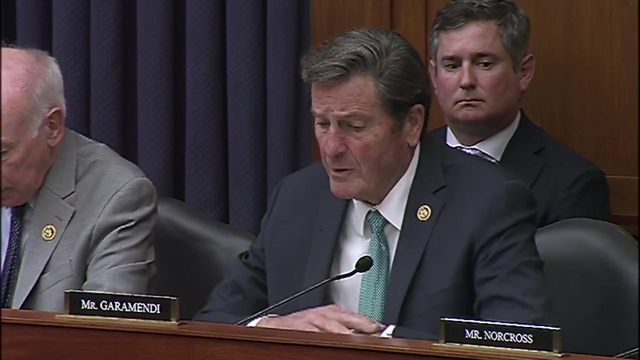 And so it's just unacceptable. A minimum investment- and I draw this to the attention of my colleagues here- a minimal investment in these transport platforms can significantly increase the ability of that platform to operate. A minimum investment- and I draw this to the attention of my colleagues here- a minimal investment in these transport platforms can significantly increase the ability of that platform to operate. 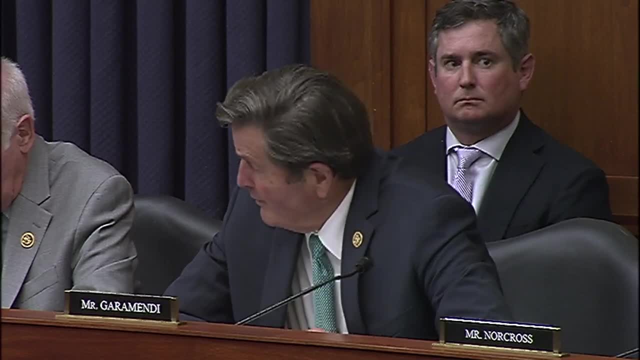 Maritime. thank Mr Walts for raising it, as have two of my colleagues, other colleagues here, As have two of my colleagues, other colleagues here. we've got to deal with this issue maritime. thank Mr Walts for raising it, as have two of my colleagues, other colleagues here. 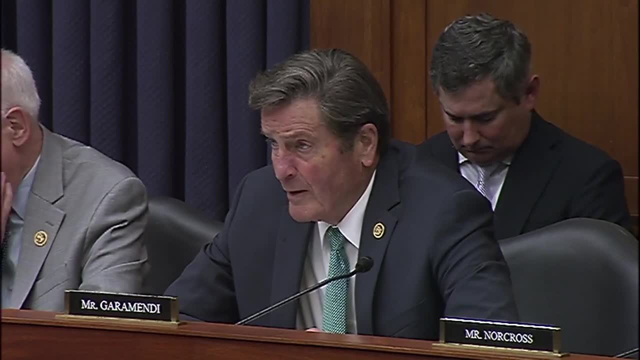 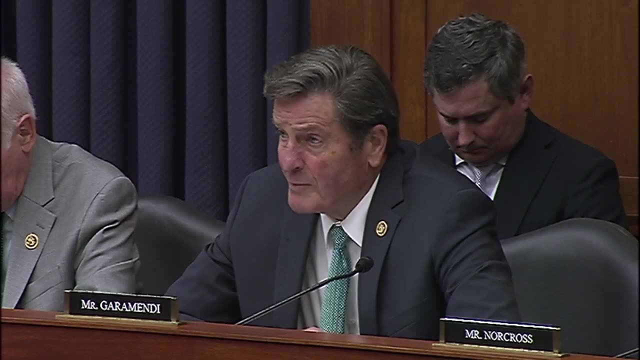 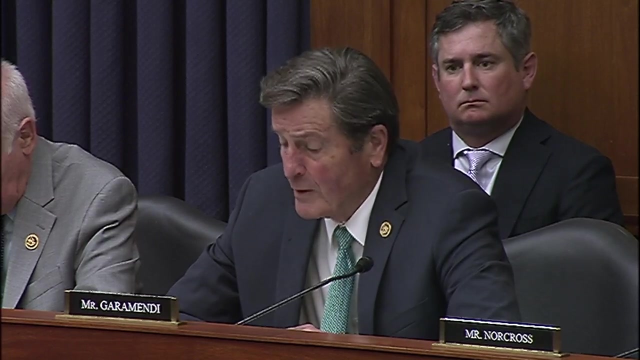 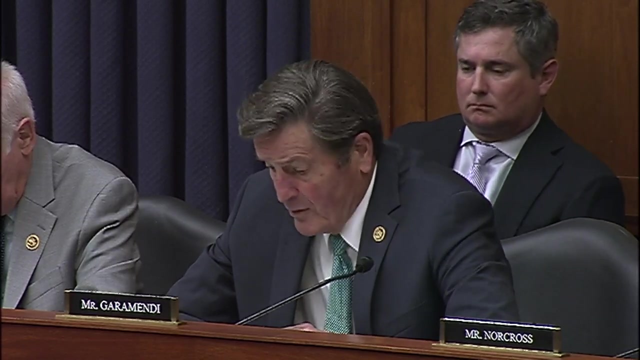 I know that Ben Adler from B akin to: We're gonna buy used ships. We're 25 years old And spend about $1, recipe a whole lot of money refurbishing them, perhaps sufficiently, and they're going to age out very, very quickly. we're going to need a different strategy here. some of this has been talked. i 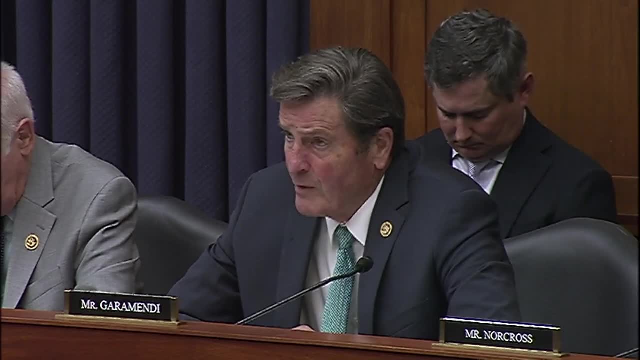 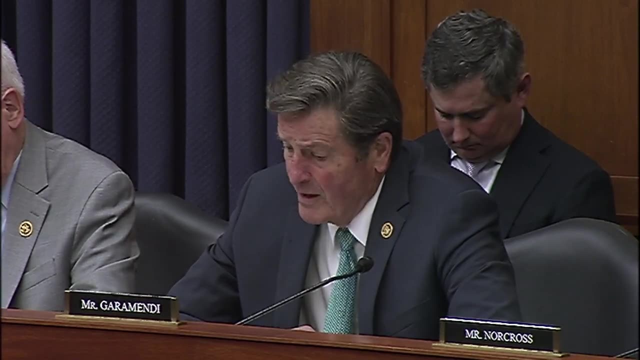 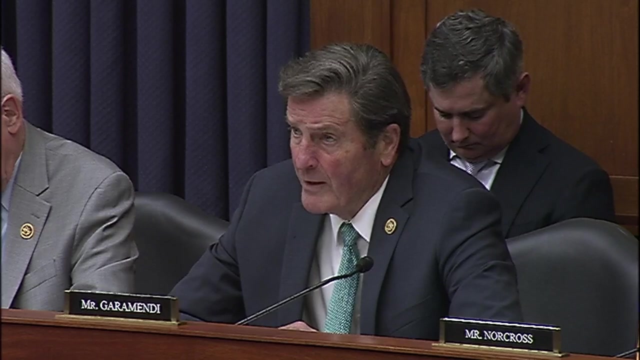 know mr waltz and i have talked about a national maritime strategy in which we would use jones act vessels and other vessels that are in the american maritime trade, that they would be available, made to be militarily useful, and then call them up when we need them, building a reserve fleet, that's. 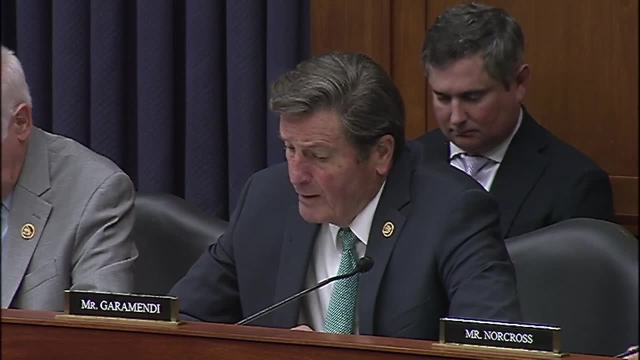 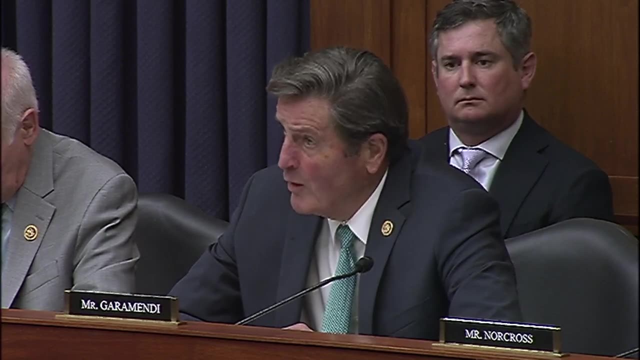 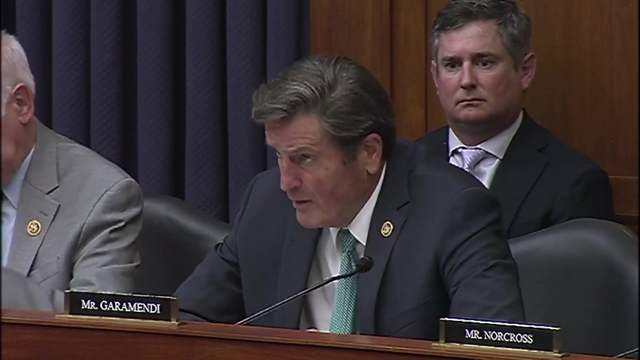 quite different than our current reserve fleets. i want to- i'm going to continue to look at how this might be done. it does not require that the military own all the ships. it simply requires that the military make those ships that are privately owned militarily useful with an additional. 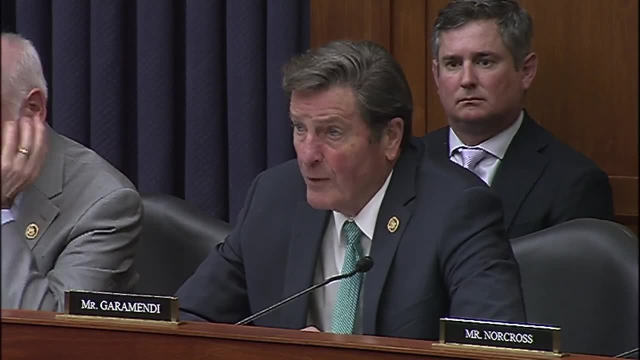 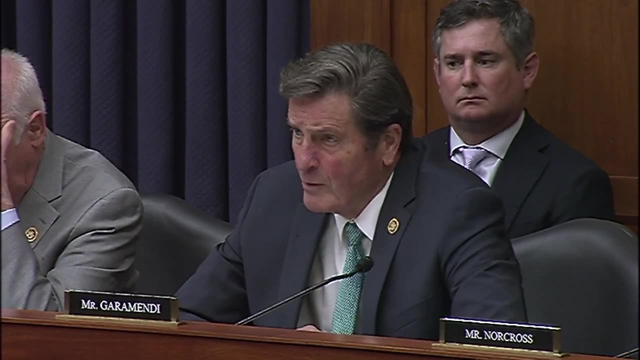 investment and probably some stipend to keep them available if and when needed. general van oost, i know you do this with airplanes. in fact, i think you took two of the planes i needed to fly back and forth non-stop from sacramento, so you put me on a route. 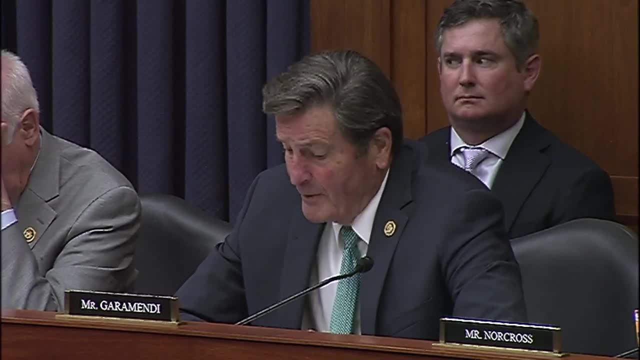 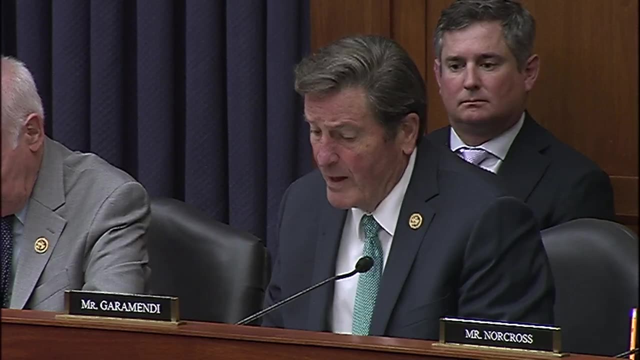 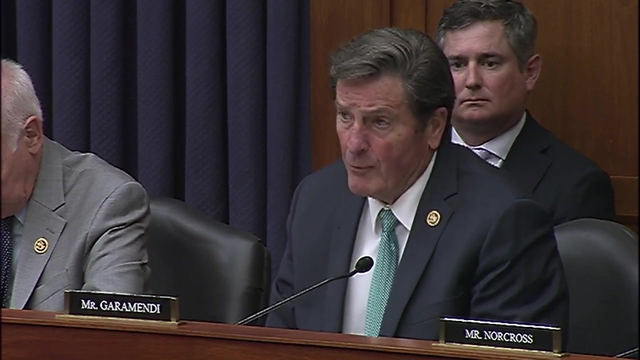 through chicago. i'll blame it on you. so this is part of what we need to do. the ready reserve fleet: we've had this discussion about how we might be able to create a national maritime security program using the jones act fleet, using the other privately owned vessels that are on the water. 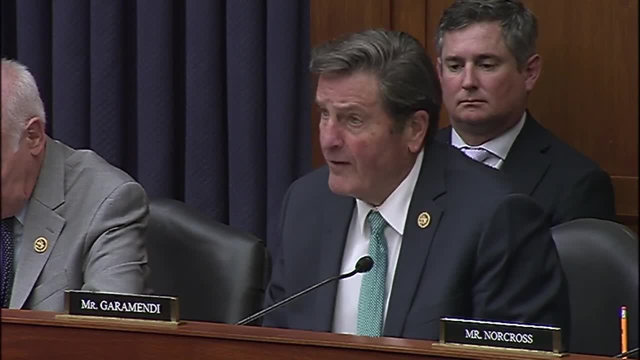 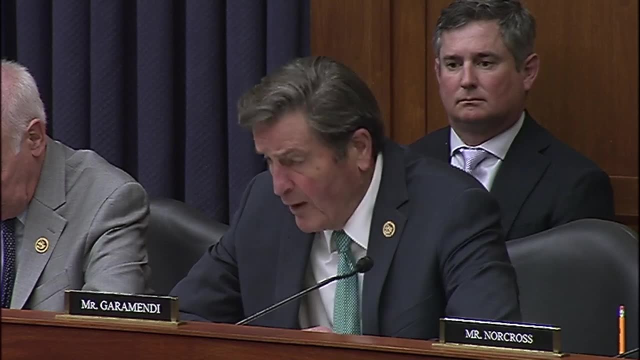 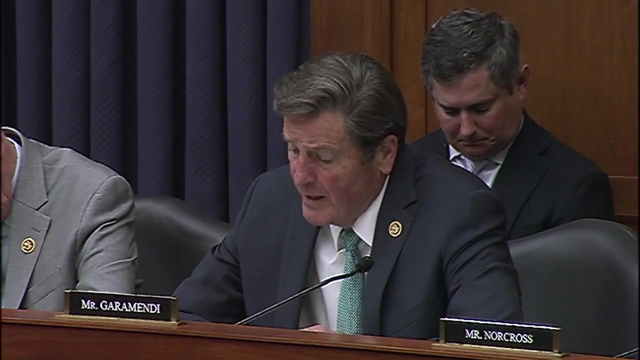 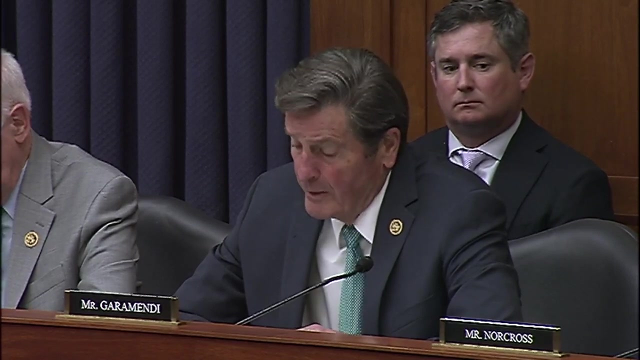 my final point deals with title 11, financing to support our shipyards to on the private side. big issues on the government-owned shipyards- we could talk about that ad nauseum. but on the privately owned side we need to. if we are building ships, we will in the commercial or the private side. 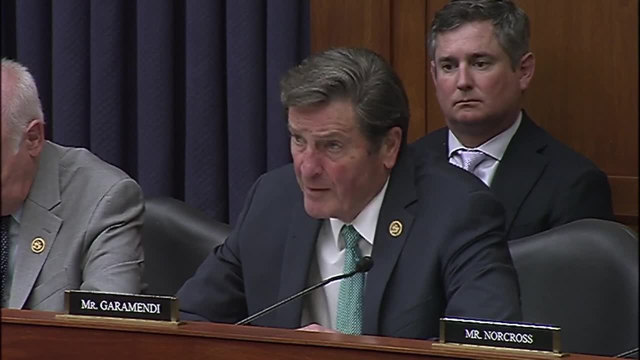 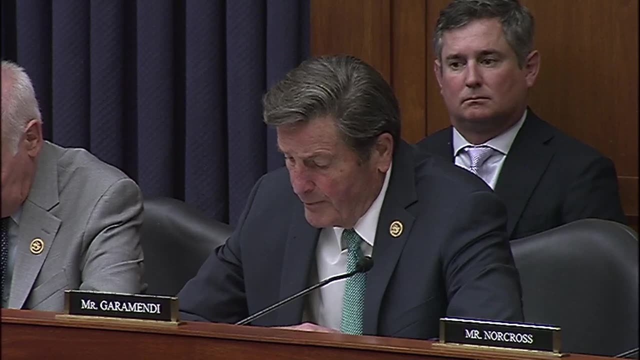 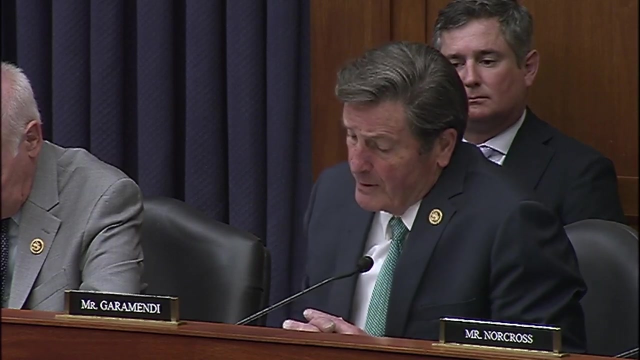 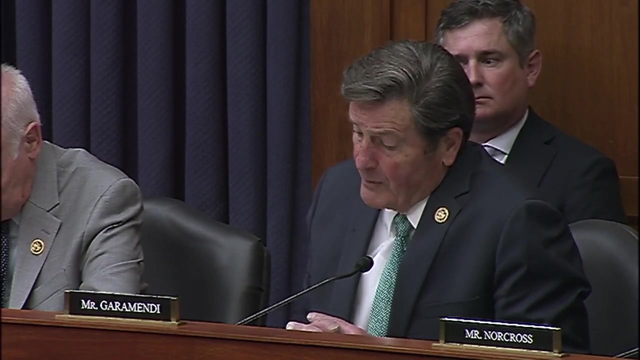 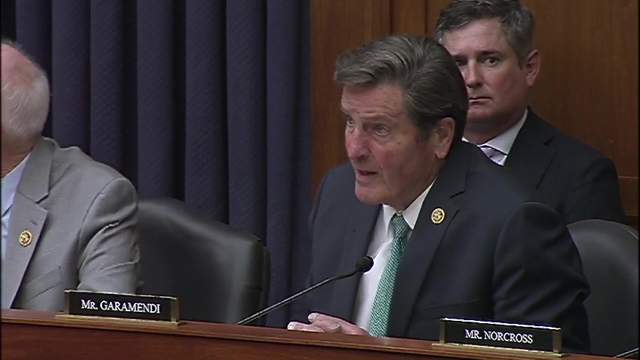 we will invariably improve our shipyards, and the capacity for those shipyards to be able to repair government ships and other ships are necessary in the face of a conflict. we've enacted legislation to reaffirm mirad's authority to determine cargo preference. we want that to be effectively put in place. we want to make sure that if there's cargo, cargo is king, i'm told. 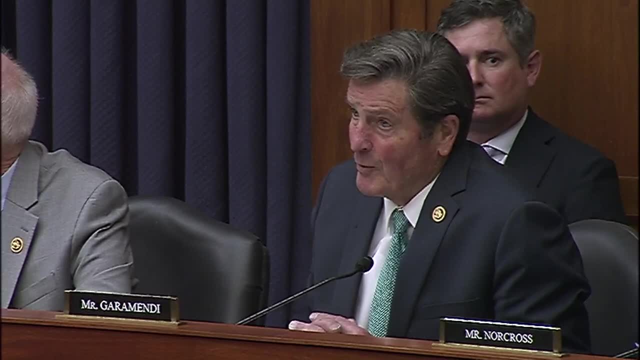 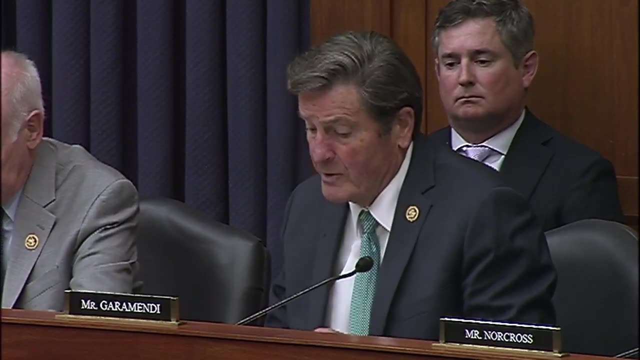 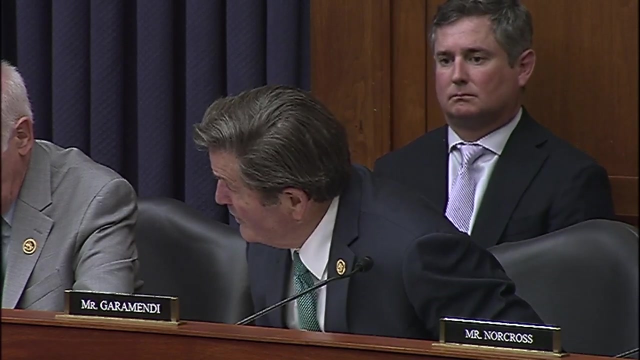 military cargo is critically important. so let's support our maritime industry by using, by making sure that what is in the new law is actually engaged- a lot of other things to talk about the fact that both of you are here. i want to thank the chairman of the committees. you've done. 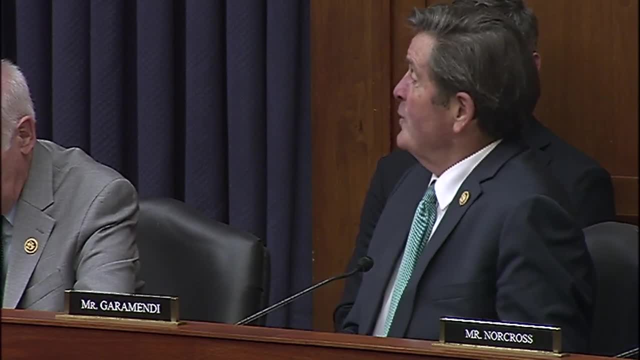 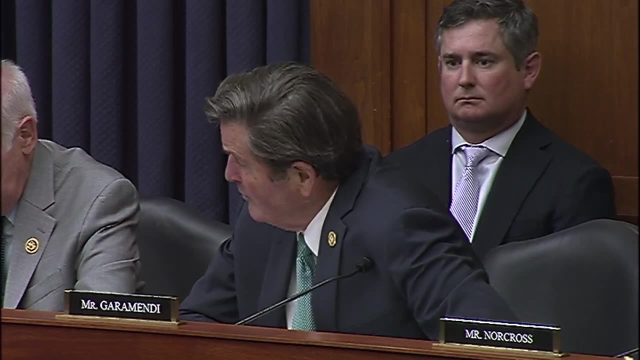 something unique which i had. oh, i should have expected you would do it, but i hadn't. but you brought us. you brought together two of the key critical issues that are important for us and is players in one hearing. thank you for doing so. with that, I yield back. thank. 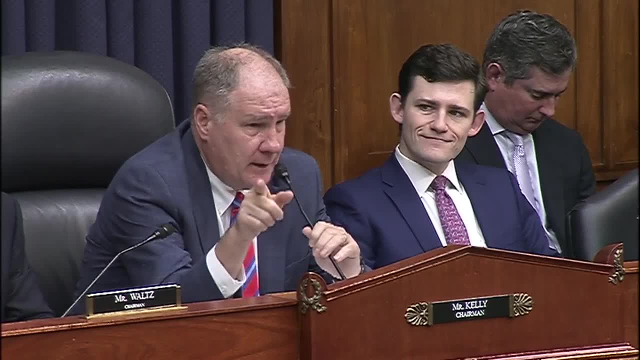 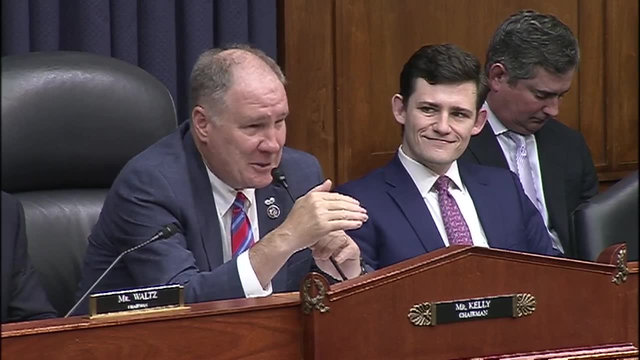 you before I start. we're going to put us on the clock so that we give everybody a chance because we've got votes. but, General Van Ovos, I would go. I need to make sure. hopefully this is not your last posture hearing, but I think that it. 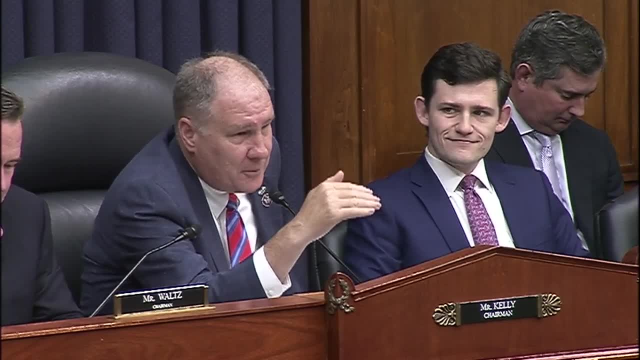 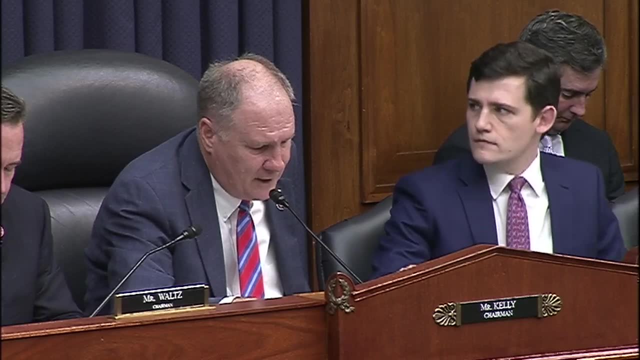 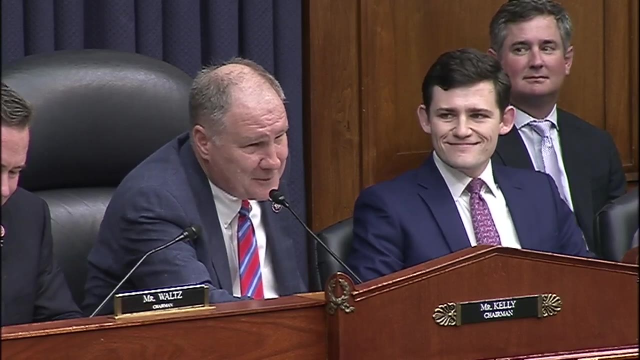 may be, and if it is, thank you for your tremendous service to our nation, and thank you also, Admiral Phillips. my first question is General Van Ovos. oh, oh, I'm so sorry I'm getting ahead. I still mean that, though. so if y'all okay, you're. 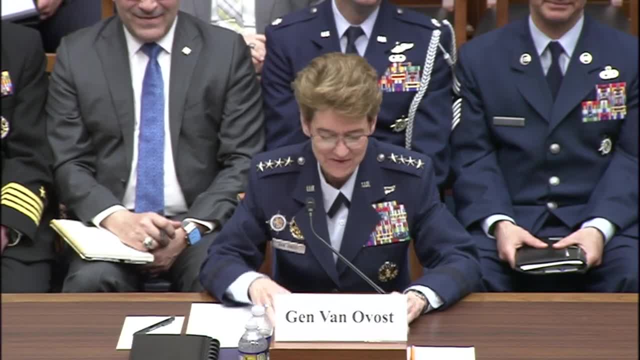 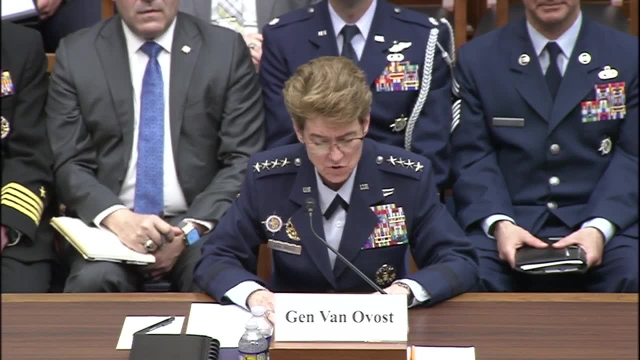 recognized. great thank you, chairman, chairman Kelly, chairman Waltz, ranking member Courtney. ranking member Gurmundi, distinguished members of the committee's good afternoon. it's my honor to join you today with my senior enlisted leader, Chief Master Sergeant Brian Krizelnik, to represent the men and women of 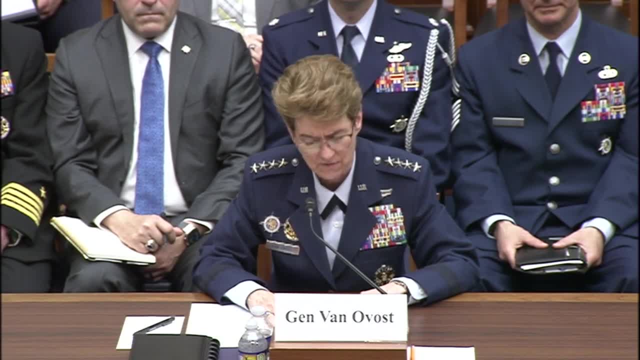 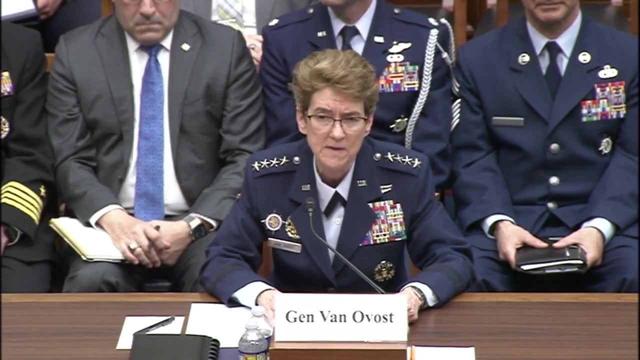 United States Army and the United States Army and the United States Army and the United States Transportation Command. as we defend the nation, take care of our people and succeed through teamwork. I'm extremely proud of our team of logistics professionals who lead the joint deployment and distribution enterprise, continually exceed expectations and ensure hope deterrence. 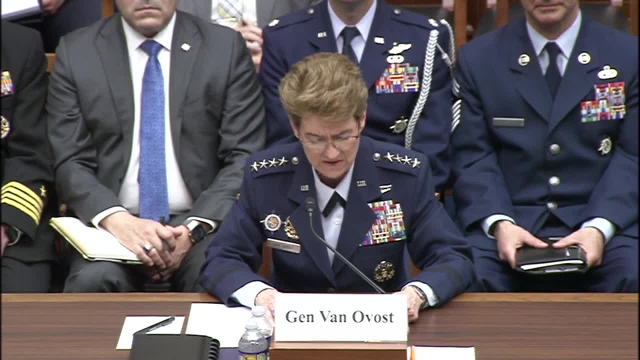 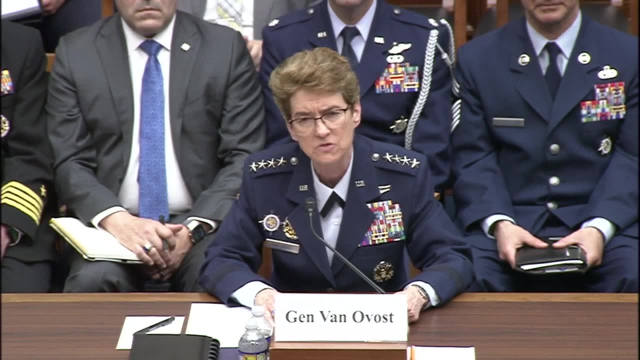 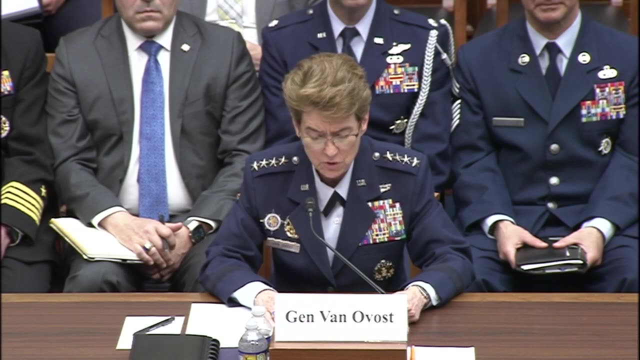 and victory are assured as we contribute to our nation's defense from competition to crisis. the entire enterprise proudly delivers for our nation, allies and partners. we know our success around the globe would not be possible without the steadfast support of this committee and the whole of Congress. the fiscal year 25. 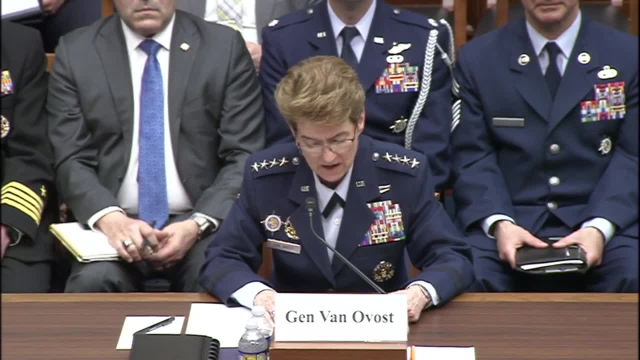 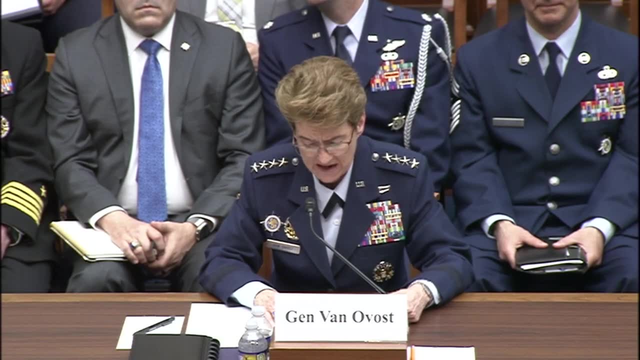 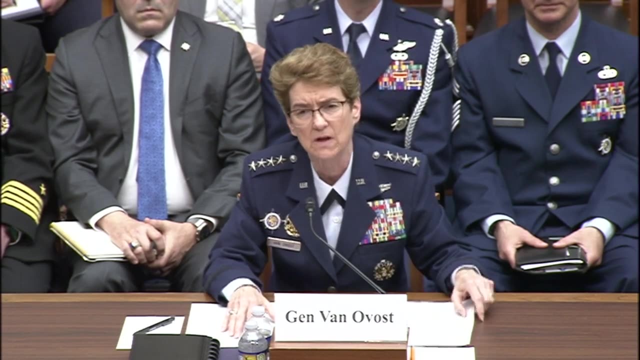 budget request continues to make strides in closing gaps in our mobility areas as we prepare for Global operations in a contested environment. a contested environment is the reality of today, whether it's in the homeland or abroad. we cannot presume freedom of maneuver to execute operations or full access to our lines of communication, our organic fleets, coupled with 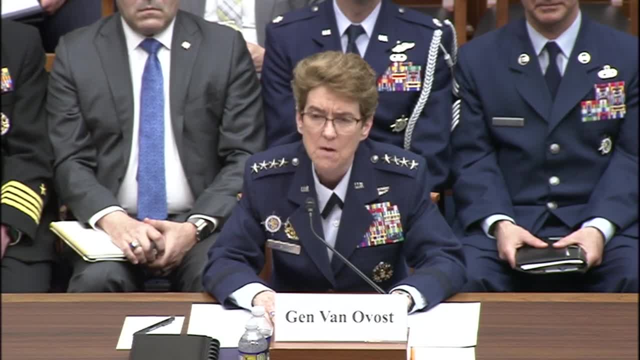 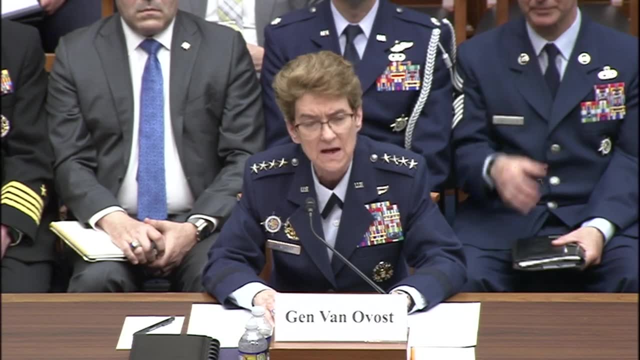 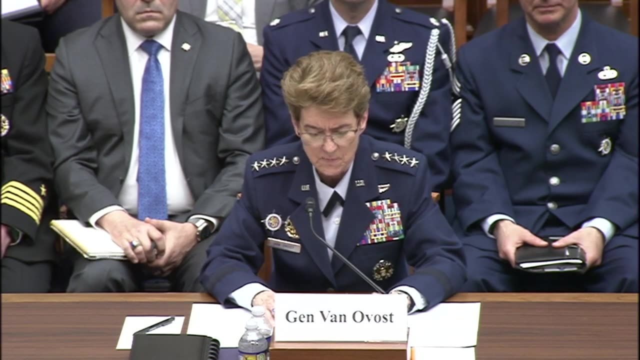 the vital capacity provided by our commercial transportation partners must continue to present credible capacity, meaning we must modernize our mobility capabilities to include cyber resiliency and digital modernization initiatives. a connected, aware and survivable mobility fleet and Network is needed to maintain our Advantage against a capable and determined 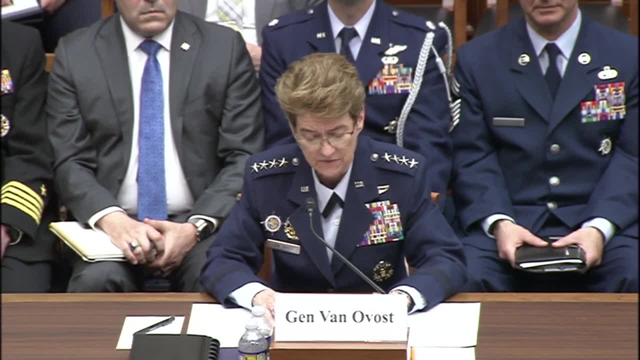 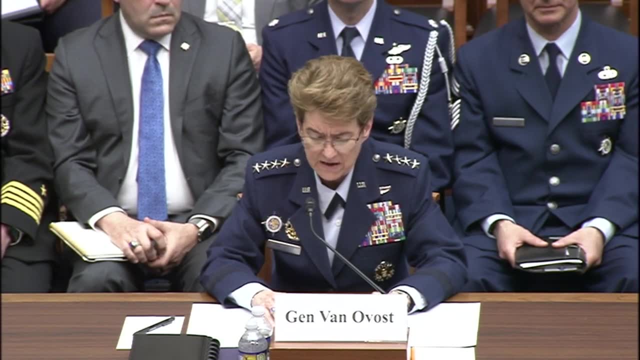 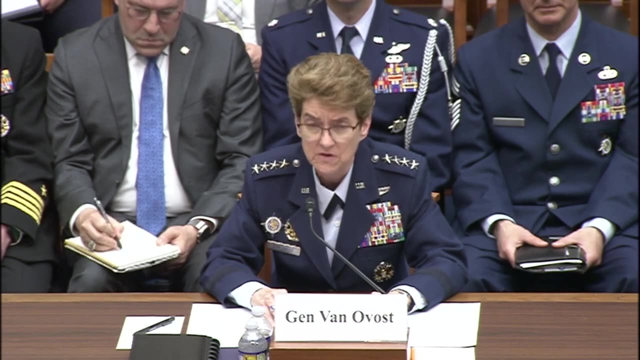 near-peer adversary. my top readiness concerns remain sea lift and air refueling. see lift is the backbone of our ability to deliver a decisive joint force. however, the age of the fleet is dragging readiness rates to alarming levels. 17 of the 47 organic ready Reserve Force ships are 50 years or older. to address readiness and 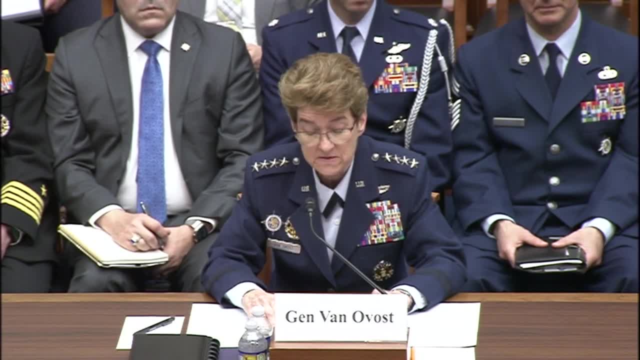 the decrease in capacity due to the planned retirements of 27 ships in the next eight years, we must add younger ships to the fleet. transcom supports the Navy strategy to acquire Uc lift vessels from the commercial market and further request to provide the Secretary of Defense. 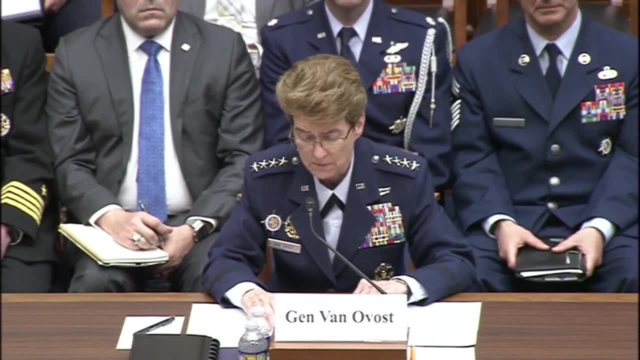 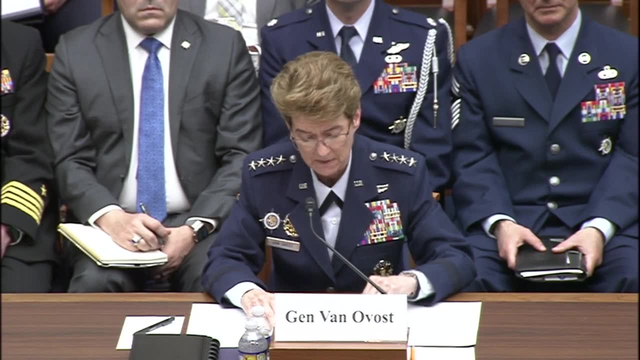 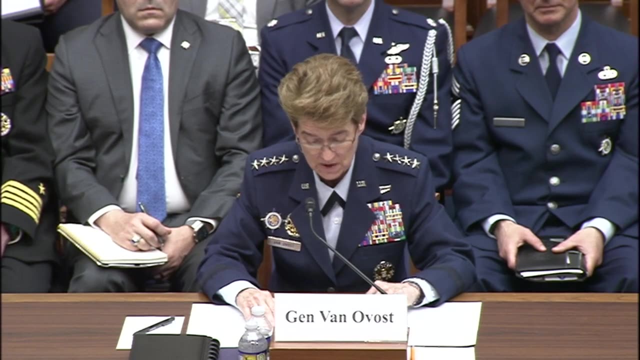 discretionary Authority to purchase foreign-built U ships under favorable market conditions without restrictions. we acknowledge Congress's intent to include domestic new build sea lift ships to recapitalize the ready Reserve Force and we're working with the Navy and the Maritime Administration to create an acquisition strategy for new construction that will complement the by-use program. Admiral Phillips and I recently 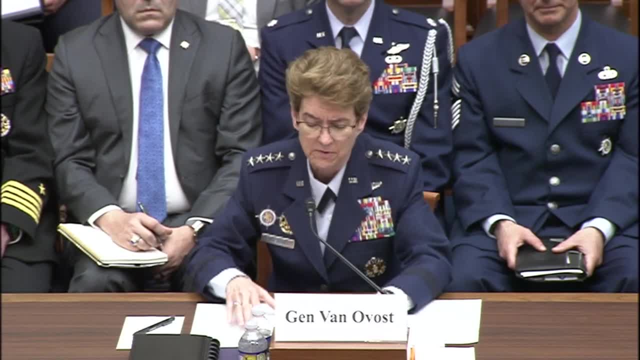 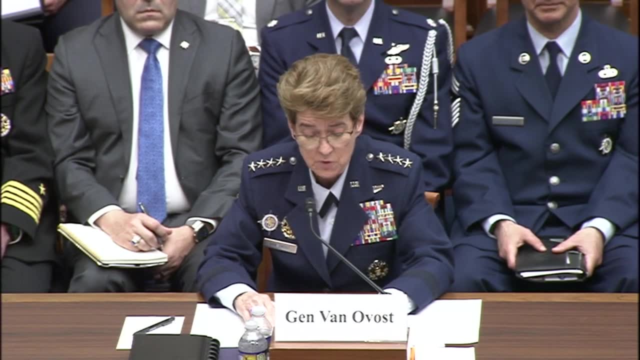 toured the Philadelphia shipyard and saw ship building capacity available there. I believe the vessel construction manager model is a viable option for future sea lift construction program. I greatly appreciate your support for timely, predictable and stabilized funding to meet our recapitalization requirements. similarly, air refueling is foundational to our nation's power. 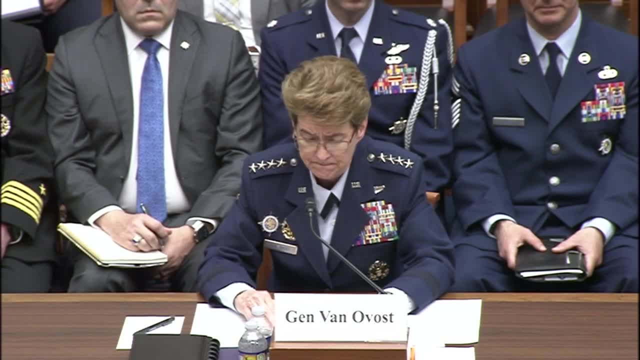 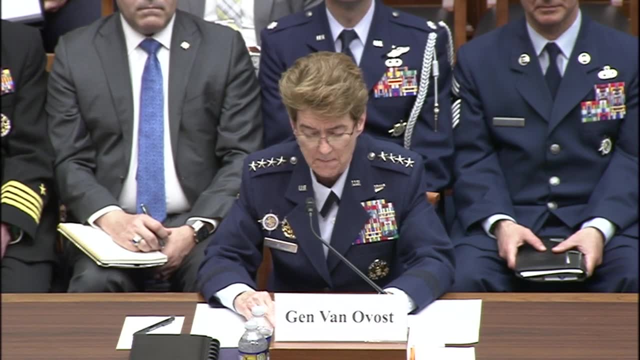 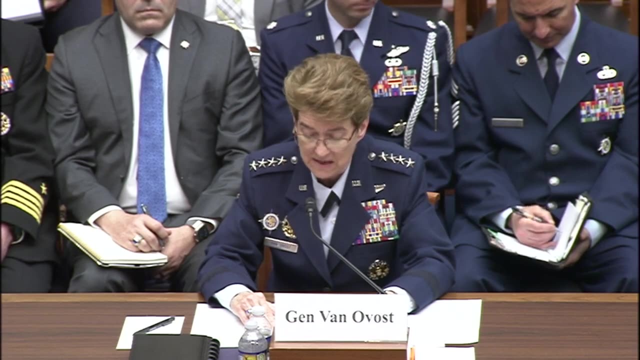 projection advantage. it is our most stressed capability. we must ensure continuous modernization and recapitalization of the aging Fleet to meet the operational requirements of the modern battle space. transcom supports the Air Force strategy for uninterrupted tanker recapitalization and accelerated fielding of the next generation air refueling system. over the past year we have made 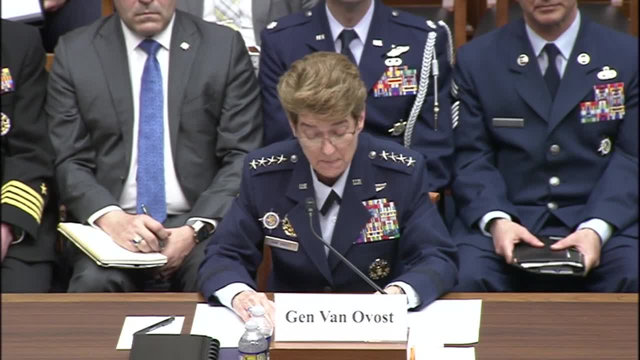 great strides diversifying our bulk fuel distribution and delivery posture by having an increased forward presence with fuel afloat in contracted Maritime tankers, and increasing capacity and access to the US flag Maritime tanker Fleet through the tanker security program. in addition, we fully support the Maritime security. 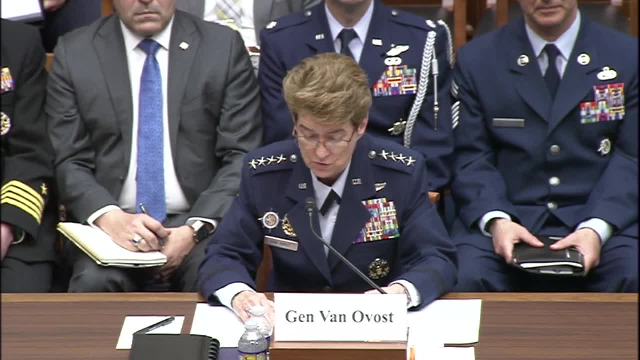 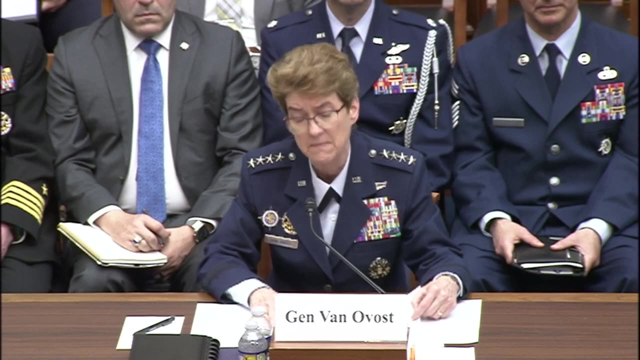 program, Jones Act and cargo preference laws that all work to ensure we have the necessary US flag capability and US merchant Mariners ready to move sensitive defense materials during a national emergency. Maritime stakeholders have been experiencing challenges with recruiting and retaining qualified Mariners and we support Marat and industry efforts to identify strategies that address the 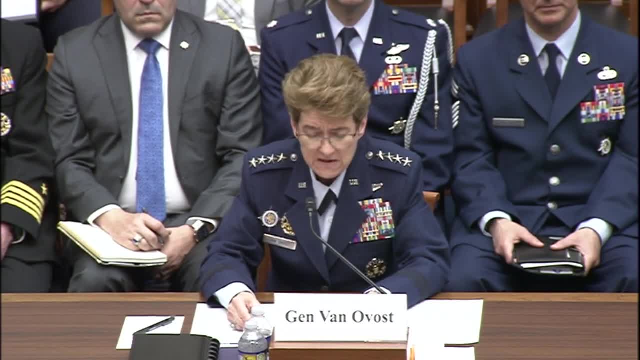 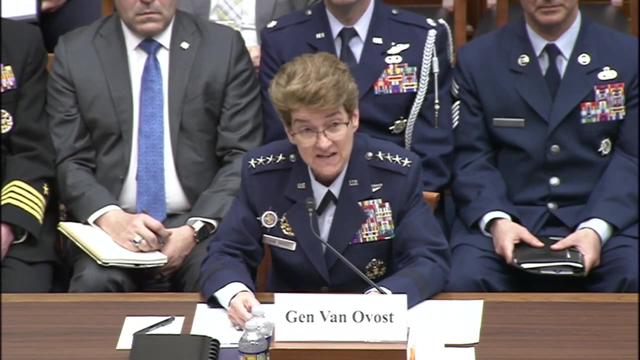 Mariner shortage and ensure their readiness to effectively sense adversary threats and activities in our logistics networks, both home and abroad. the nation must utilize all available resources. section 702 of the foreign intelligence surveillance Act provides me insights into adversaries, intense capabilities, activities to contest our logistics capabilities. the loss of this Authority adds risk to my mission. 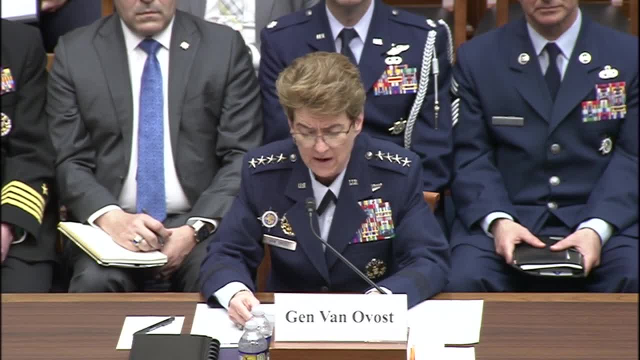 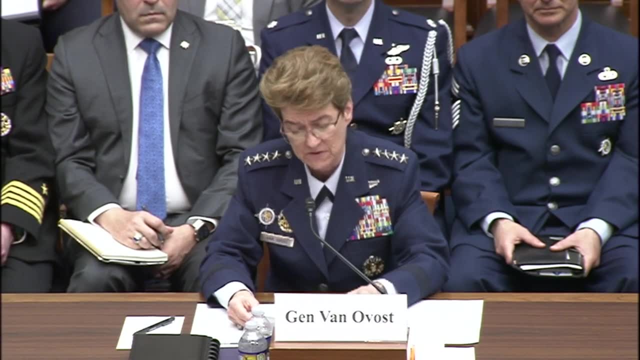 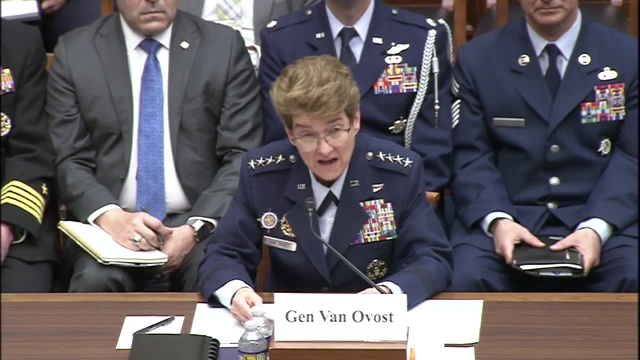 additionally, passing a National Defense supplemental is vital for the health of the transportation working capital fund, which preserves essential readiness and ensures response options for the Secretary of Defense. I'm honored to join real Admiral Ann Phillips. the relationship between transcom and Merritt has never been stronger. as we work together to strengthen our National 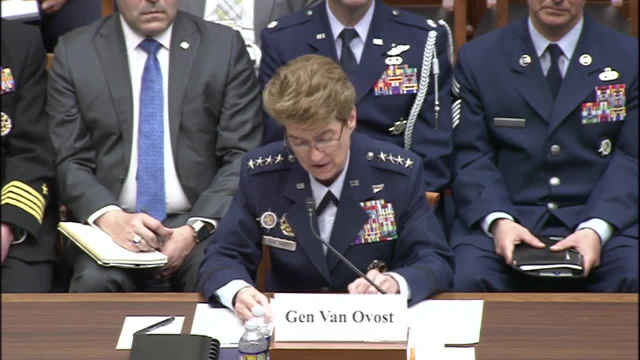 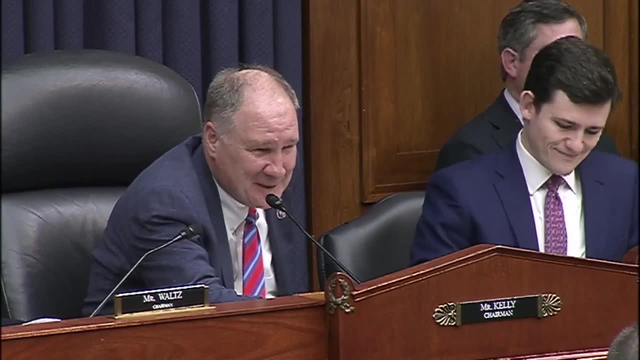 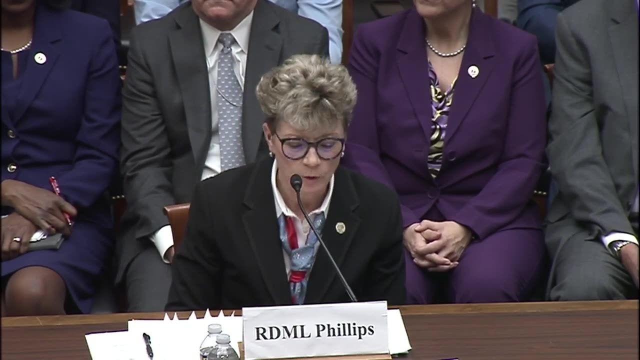 security. thank you once again for your leadership and the support you provide our workforce. look forward to your questions. Admiral Administrator Phillips, you are now recognized for five minutes. thank you, Mr Chair. good afternoon Chairman Walts and Chairman Kelly, ranking member Garamendi and ranking member Courtney and members of the subcommittee, thank you for your tremendous 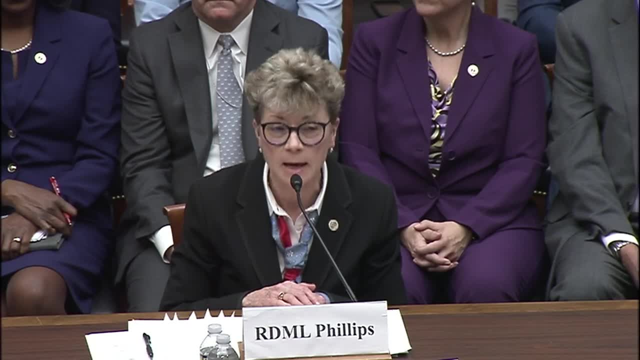 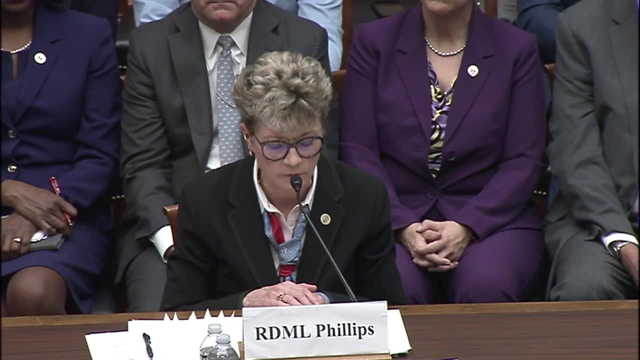 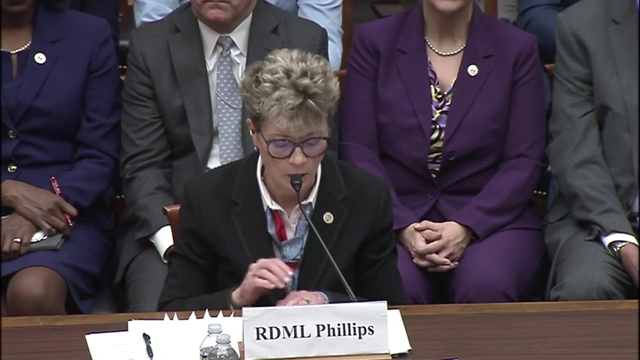 support for the Maritime Administration, the US merchant Marine Academy and the US Maritime industry. before I go further, allow me to express our condolences, on behalf of the Department of Transportation, to the families of those who lost their lives earlier this month when the Francis bridge collapsed in Baltimore. events like this highlight how important our Maritime transportation. 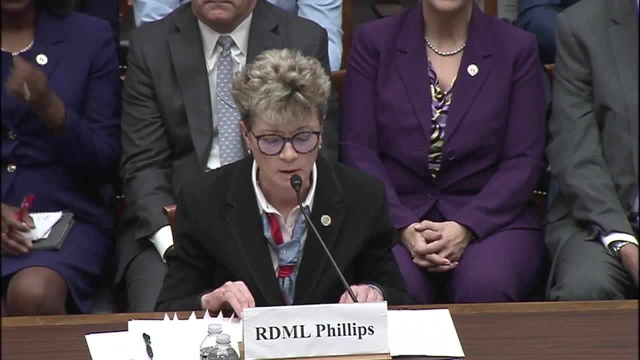 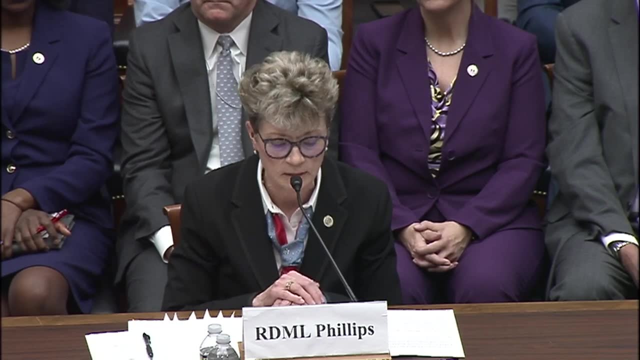 system is to our nation's National and economic security. marit's mission is to foster, promote and develop the Maritime industry of the United States to meet the nation's economic and security needs. in that context, the president's fy 2025 budget request of 859.7 million for raids will 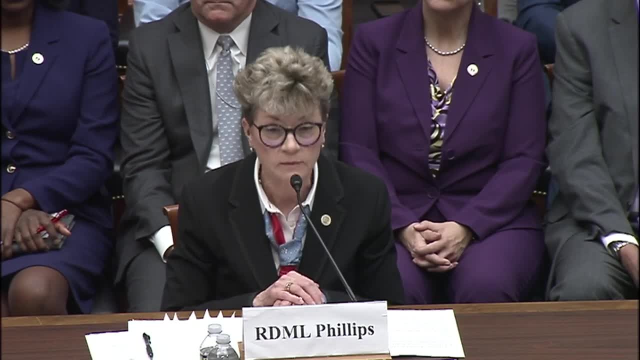 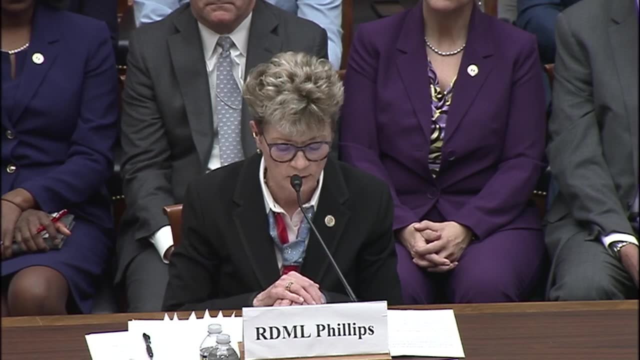 enable the agency to continue to strengthen our sealage Enterprise by advancing recapitalization of the ready Reserve Force and vital commercial seal of program that support US flag vessels operating in foreign trade. Let me begin by discussing our Ready Reserve, an area of focus today. 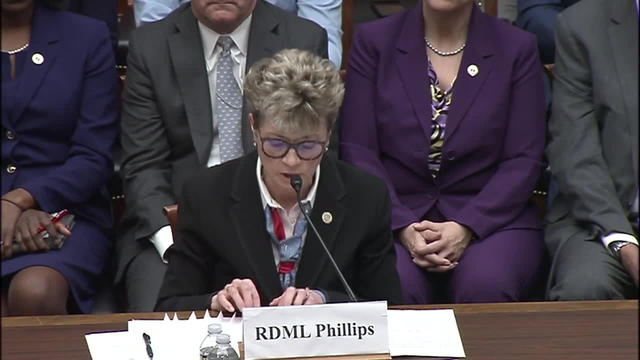 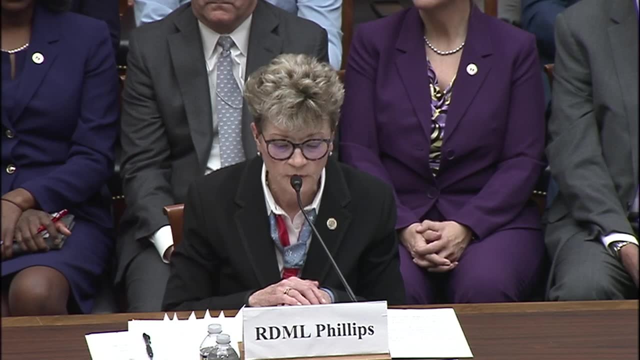 Our 2025 budget requests $974 million from DOD Budgetary Authority for MARAD to acquire, upgrade and maintain vessels in the NDRF and Ready Reserve Force. These funds help MARAD to keep the fleet in a ready, reliable and responsive condition. 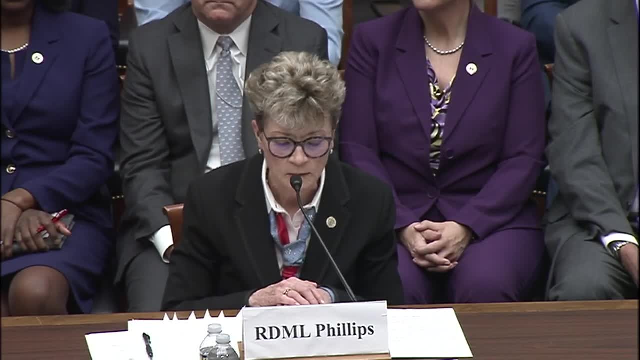 to ensure MARAD can meet the nation's strategic sealift needs. The RRF consists of 48 vessels today averaging over 45 years in age, and they are maintained in reduced operating status. This fleet will expand to 51 vessels by the end of FY 2025. 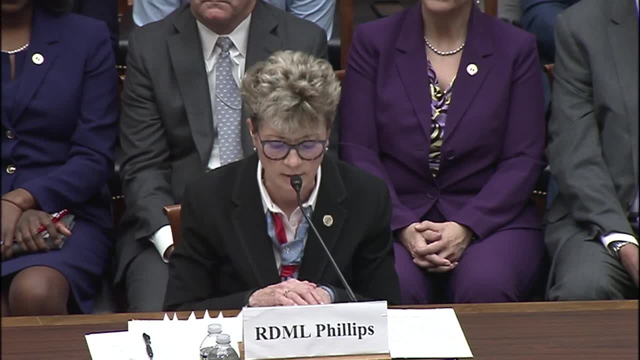 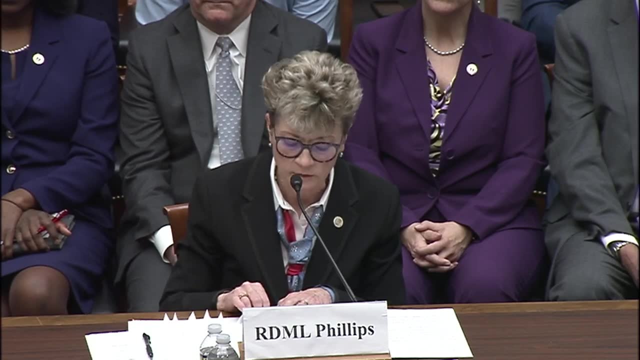 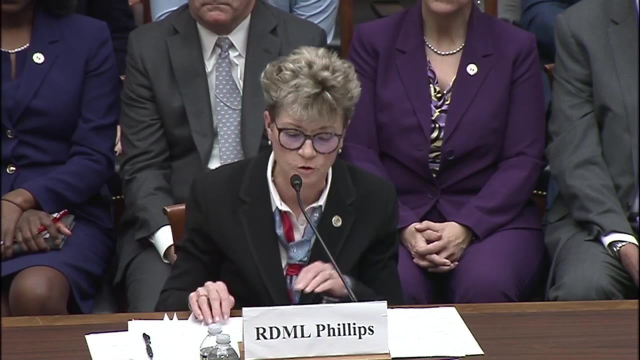 with the planned transfer of vessels from the Military Sealift Command. MARAD is responsible for maintaining these aging ships. as part of the Navy Sealift Recapitalization Plan, We are actively advancing urgent recapitalization of the RRF, using congressional authority to purchase vessels through a contracted Vessel Acquisition Manager. 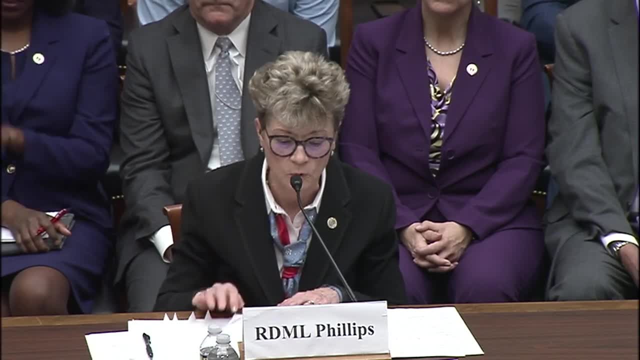 This is a very important step in the RRF's mission to ensure that the Navy's vessels This approach successfully acquired two ships in FY 2022 and in FY 2023, purchased three more: one 10 years old and two 11 years old. 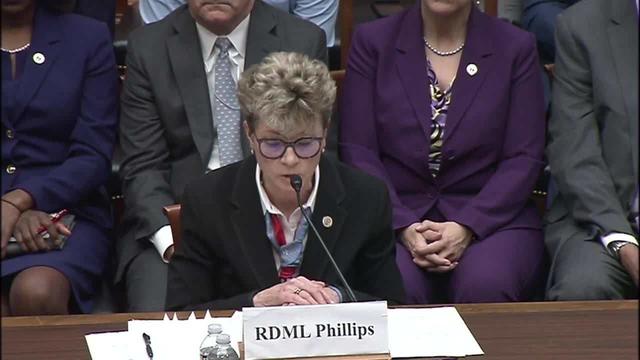 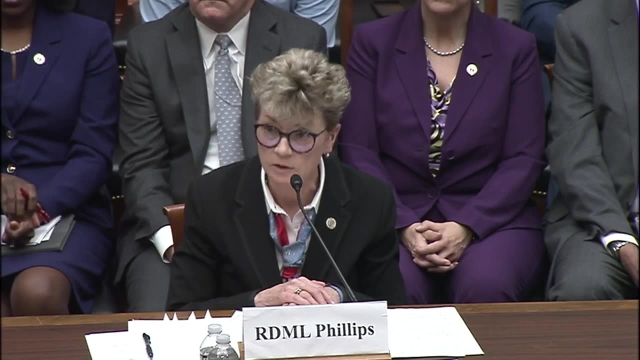 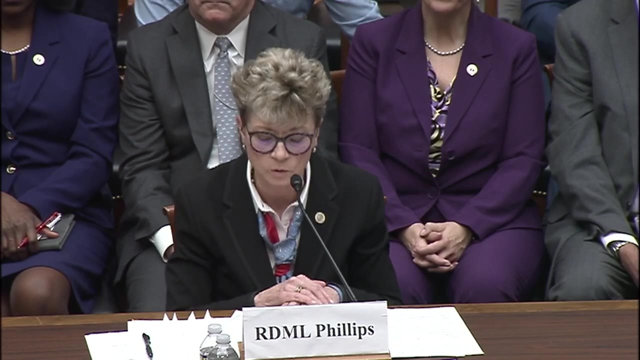 The ongoing reflagging process following the stringent Alternate Compliance Program will make all five vessels ready for use by the third quarter of 2024.. We continue to collaborate with the Vessel Acquisition Manager and have identified several potential ships for purchase, with the goal of reaching the congressionally limited number of nine used vessels. 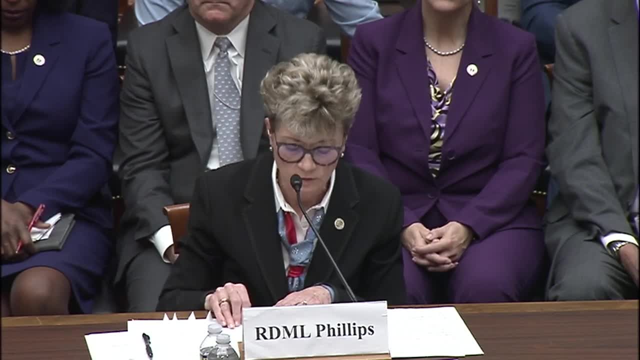 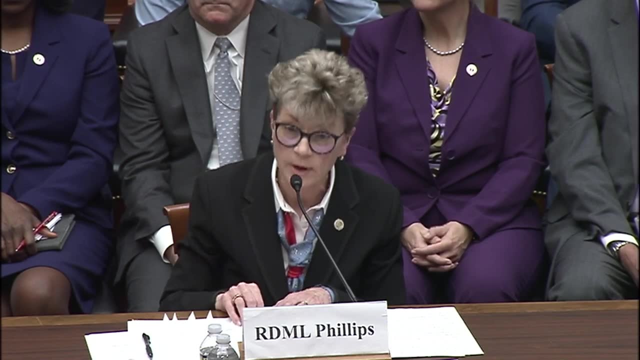 by the end of FY 2025.. In the FY 2023, Navy NDAA MARAD was directed to develop a sealift ship design for the construction of 10 new vessels for the NDRF. I offer my thanks to Congress for appropriating $12 million in FY 2024 funds. to begin this vessel design. The 2025 budget also requests the full authorization level of $318 million for the Maritime Security Program to support 60 commercially viable, militarily useful vessels currently enrolled. We have also fully implemented the 10-vessel tanker security program. 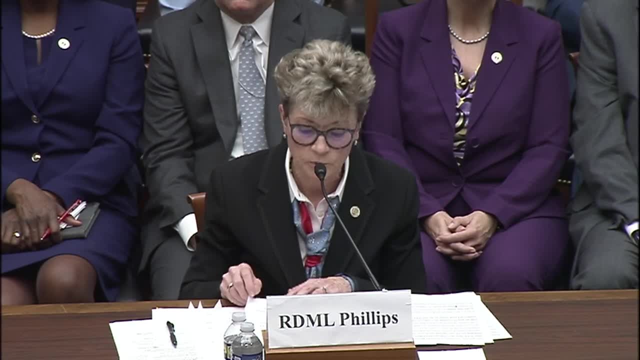 and are requesting $60 million for the Provincial Maritime Security Program. We are also requesting $60 million for the Provincial Maritime Security Program, the program. These ships will provide DOD with reliable access to product tankers, supporting national economic security. One program participant withdrew after accepting a long-term US government charter and MARIT 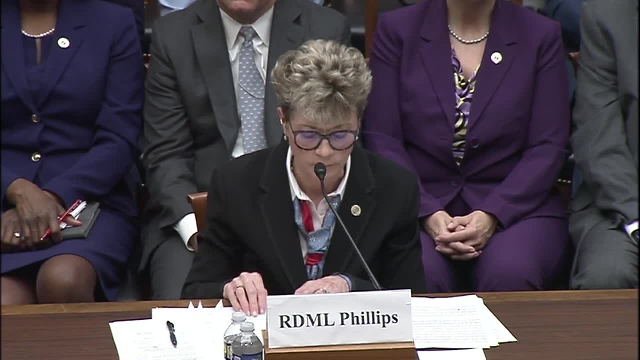 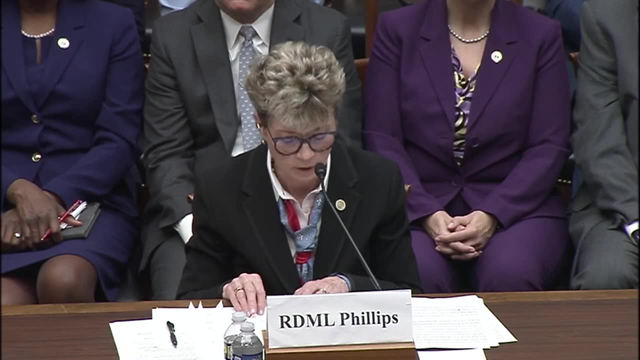 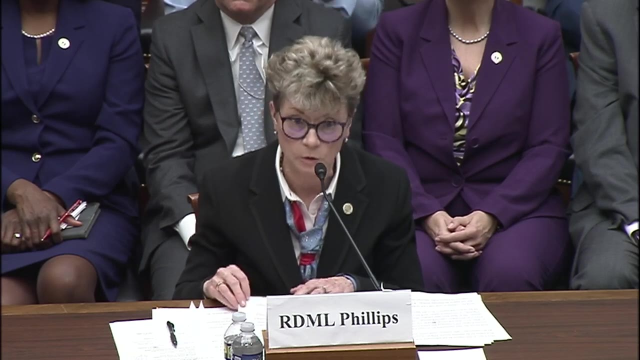 is actively working to fill the vacancy and we expect to do so later this summer. We continue to work with the Center for Naval Analysis on the body of analysis that will support the maritime strategy and we understand Congressional interest in this important effort. We continue to collaborate as well with stakeholders to address the mariner shortage. 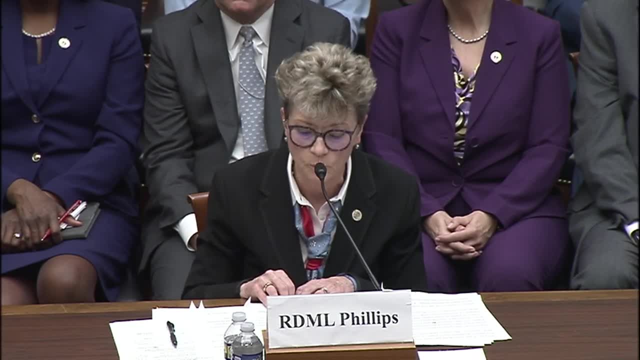 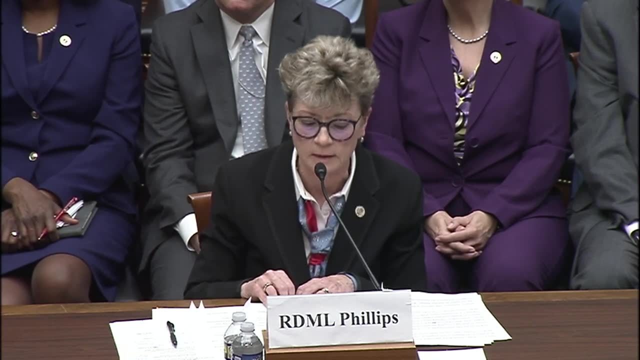 We recently convened the FY2024 Directed Maritime Workforce Working Group to identify the number of licensed and unlicensed mariners, recommended improvements in recruiting and detention and evaluate how we can best recruit, train and retain and reduce barriers to retention to grow our pool of merchant mariners. 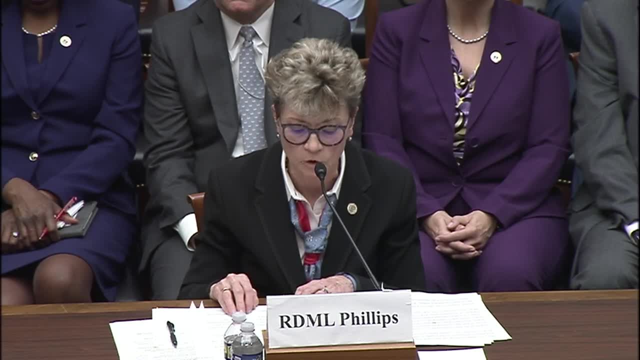 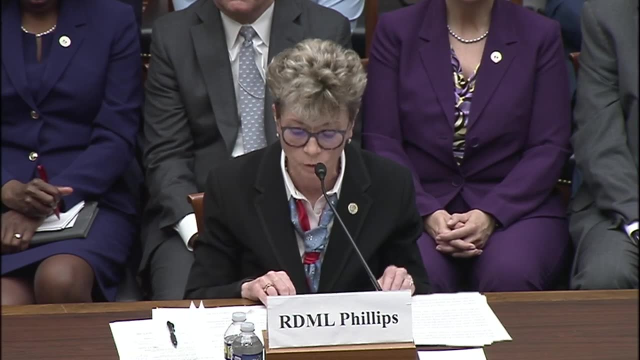 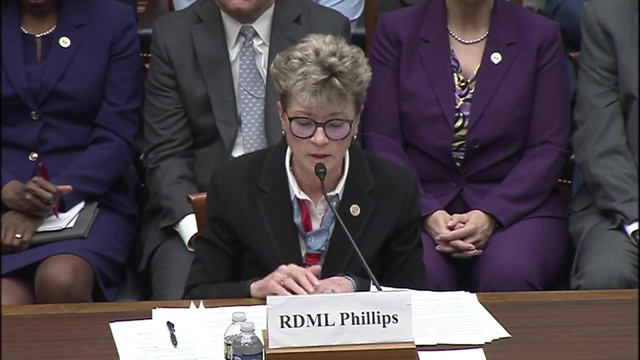 We also continue to expand Embark participation. Today, there are 21 commercial operators enrolled which operate over 180 vessels. We are working to develop a proposed Embark rule pursuant to the 2023 NDAA. In addition, the FY2025 budget request includes $191 million to support US Merchant Marine. 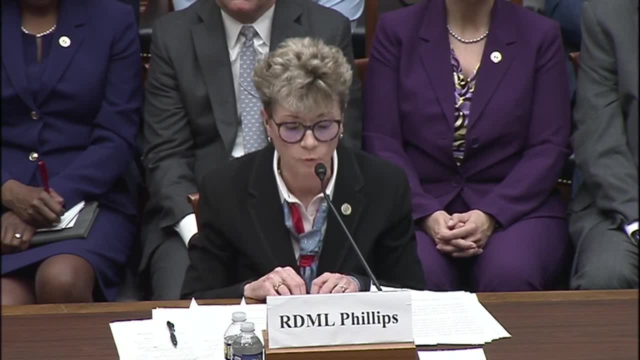 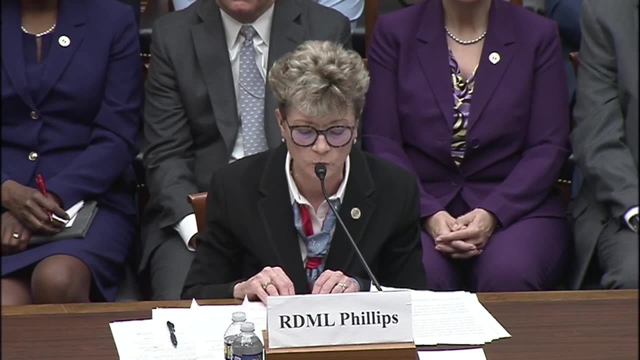 Academy operations and our capital asset management program for USMMA. It also requests $87 million to support the six state maritime academies, including continuing to build out new training vessels. Four national security multi-mission vessels are under construction using the VCM process. 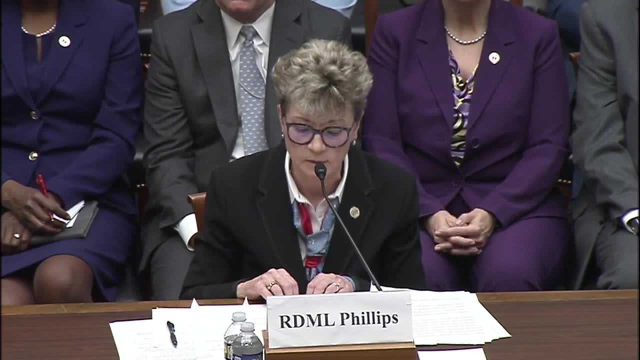 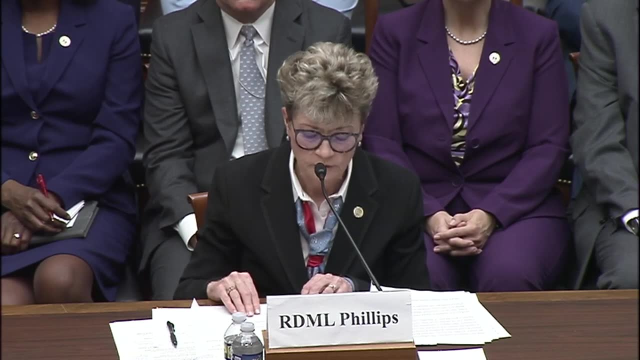 with one delivered last fall: Empire State. The second Patriot State, Patriot State expected to be delivered later this summer. and State of Maine just launched last Friday The FY2024 NDAA doubles the Student Incentive Payments Program amount from $32,000 to $64,000. 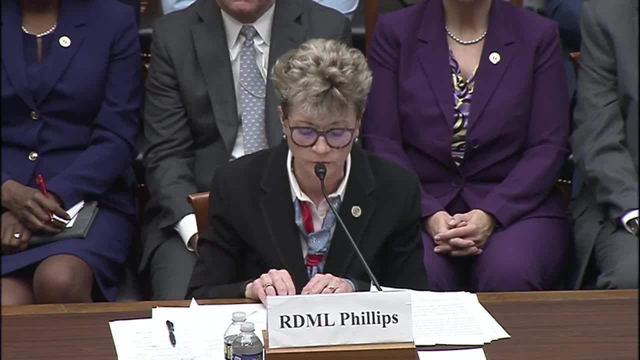 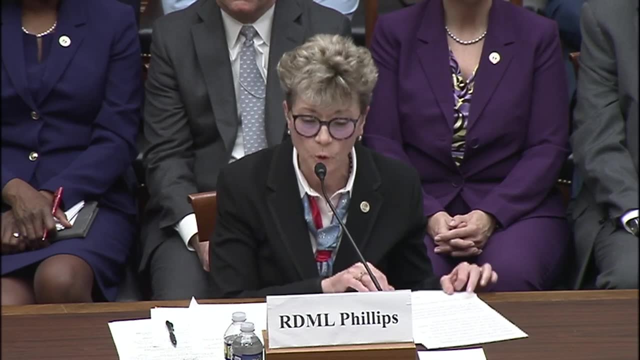 This will offer more financial support for cadets in the Strategic Sealift Midshipmen Program at our SMAs. We thank Congress for this authorization. These programs reflect MARAD's priorities, supported by the President's budget. We plan to keep you updated, of course, on our progress in these areas. 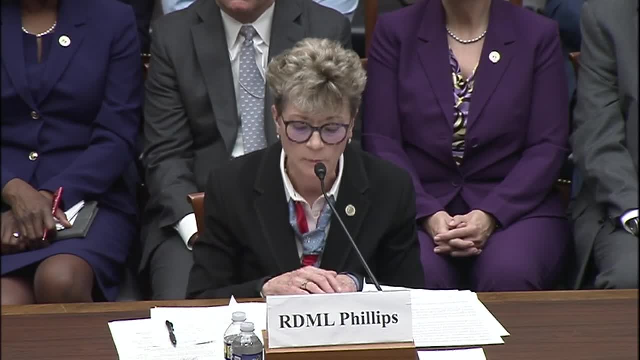 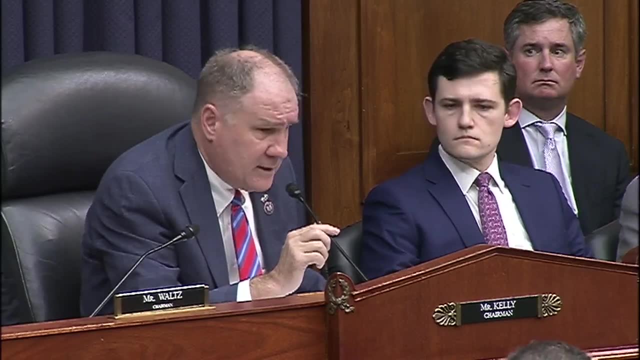 We are honored to testify here today. We look forward to questions you may have. Thank you, Thank you, And I'm going to be really strict on the clock today, guys, so I may give you 10 seconds, but no more. 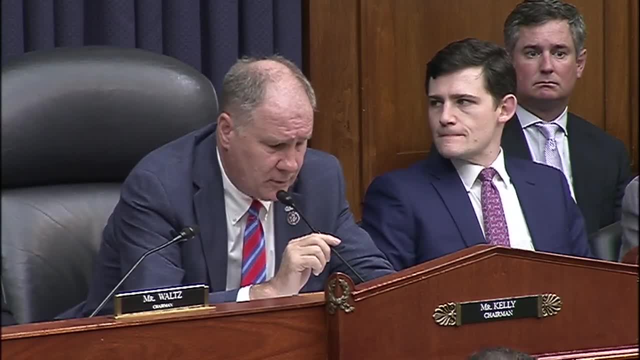 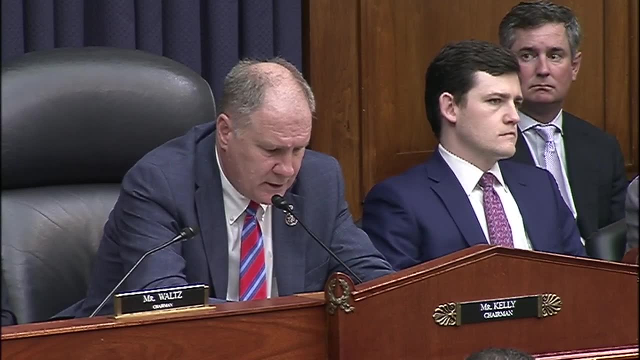 And I will cut off answers And with that, if you'll put me on the clock. General Van Ovost, how do you communicate the results of the Mobility Capability Requirement Study to the military services to inform shipbuilding, air refueling and airlift procurements? 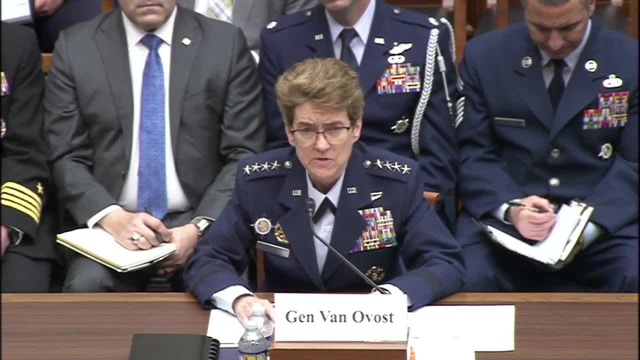 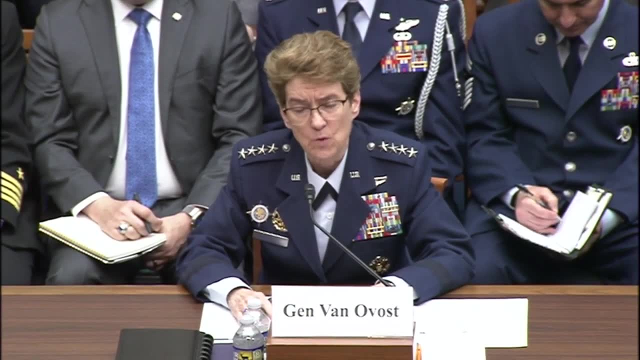 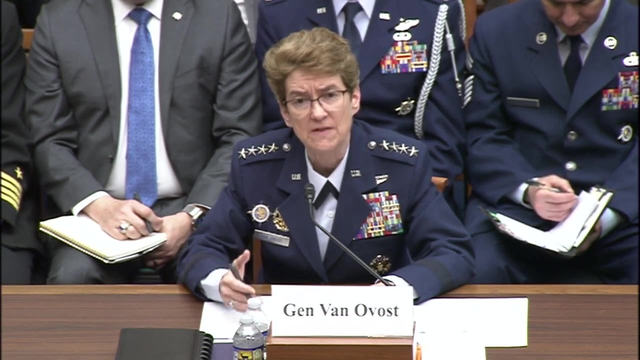 Thank you, Chairman. We use the Mobility Capability Requirement Study to provide our assessment of mobility sufficiency of the fleet. We work very carefully with the services, OSD and the Joint Staff. They're with us throughout the entire process and we outbrief the recommendations and then 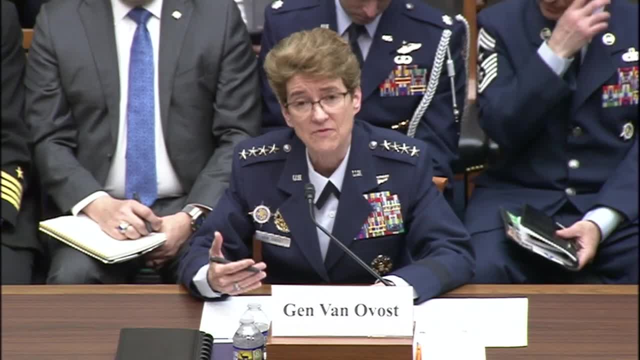 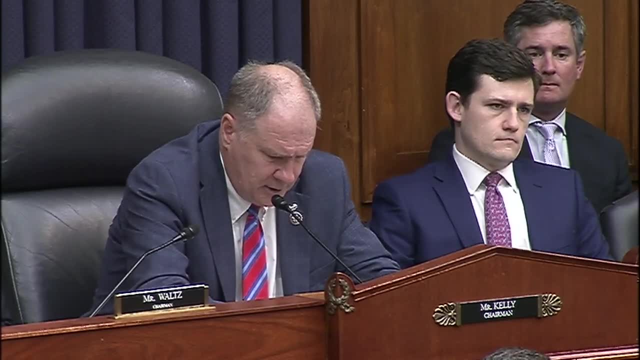 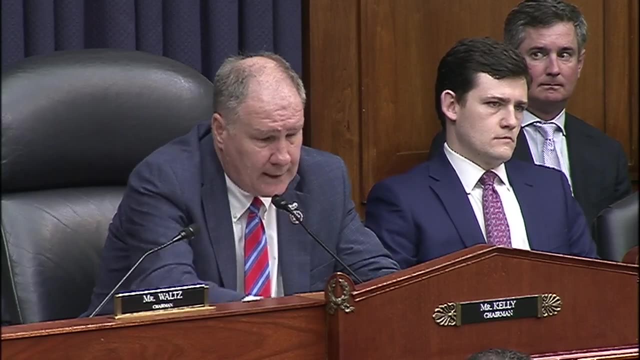 that turns into the budget process where we go after the gaps to try to close them. And, Admiral Phillips, what is your assessment of the interest in the Tanker Security Program and ability to meet the authorized requirements? Thank you for that question, Chairman Kelly sir. 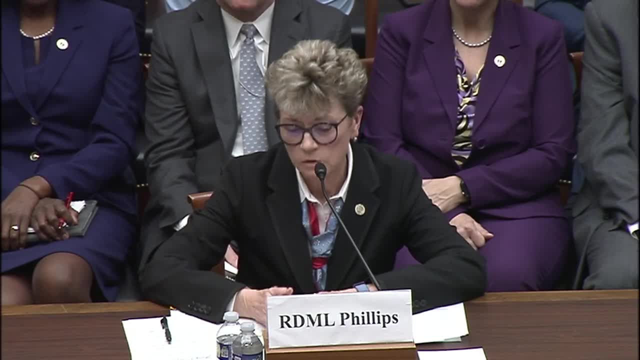 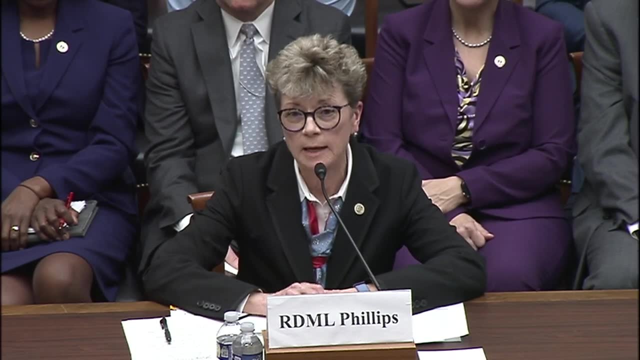 We find that there is interest in the program. As I've said, we had 10 vessels enrolled. One had an option to leave for a long-term charter. We thank Congress for the $25 million to help us, as we have discussed in the past, prepare. 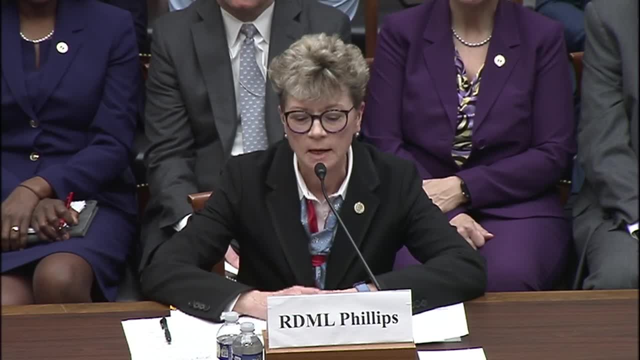 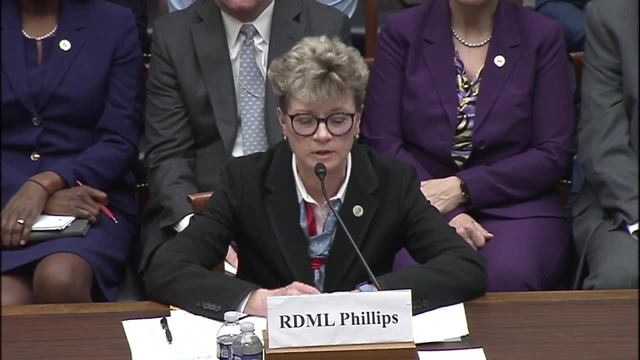 for additional training opportunities to ensure we are able to man these vessels, And of course, it also depends on the ability of government cargoes to help assist and offset the cost of manpower. So we're going to be managing a tanker under the TSP program. 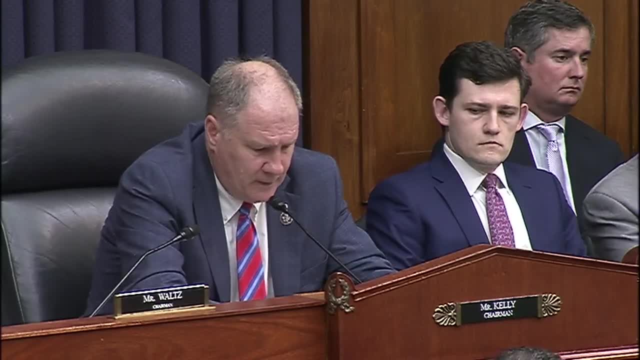 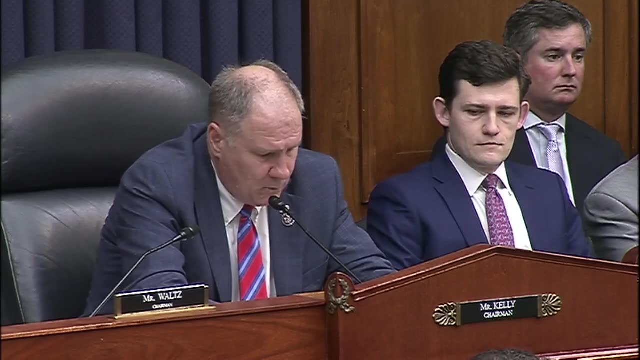 Thank you. Thank you And General Van Ovos. our air refueling fleet is comprised of mostly second-generation aircraft who have to key to Mike to receive threats. What is the way ahead on connecting the aircraft to information that makes them more survivable? 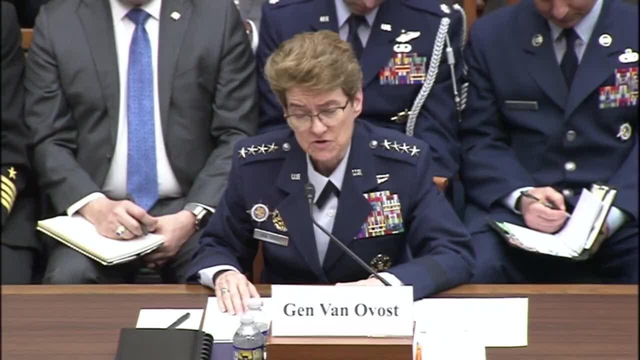 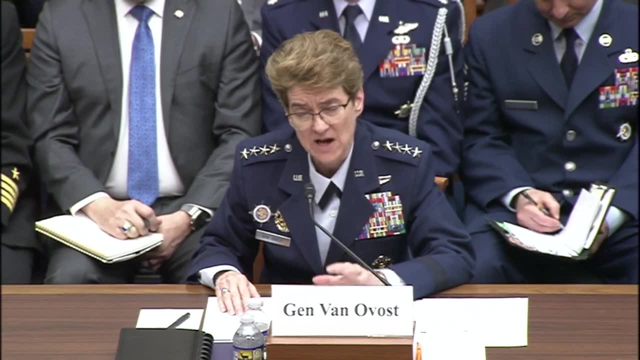 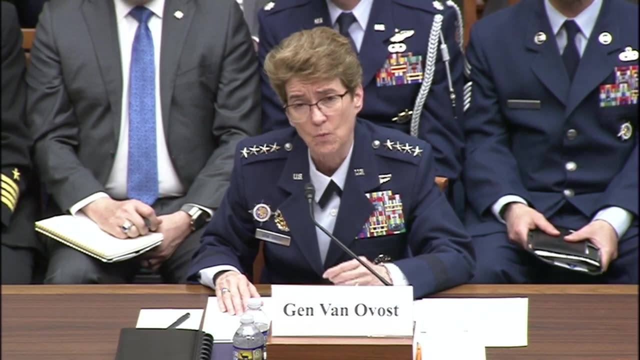 in a contested environment. Thank you, I say logistics is foundational to any strategy and we have got to be able to move our air. refueling is foundational to the ability to project and sustain the joint service. We must ensure that they're connected and they have battle space awareness, and so I'm 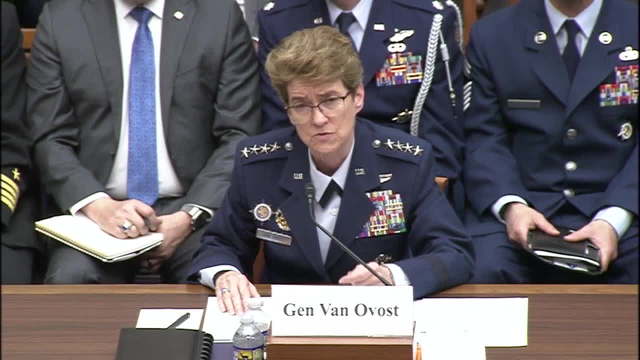 working with the United States Air Force to define those requirements for all of those aircraft. It looks a lot like the types of capabilities we have in the KC-46 aircraft, which is sort of the future of air refueling, And do you have an assessment of the cost of that? 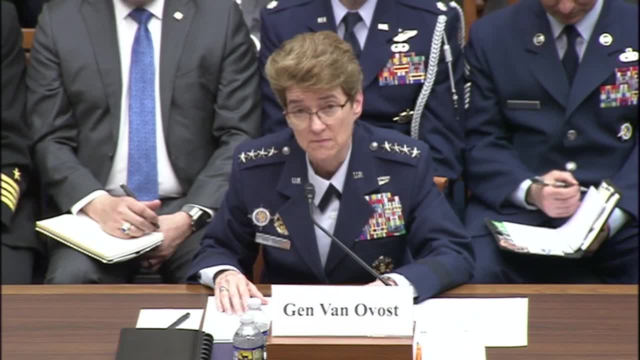 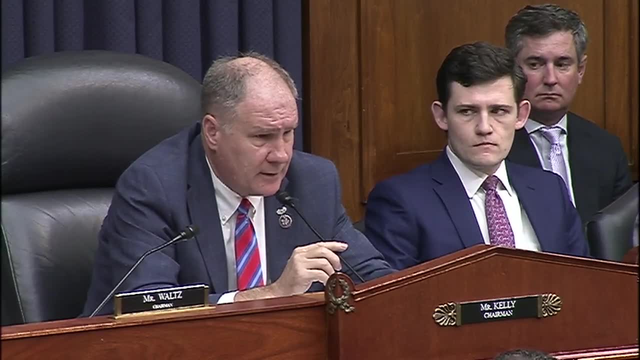 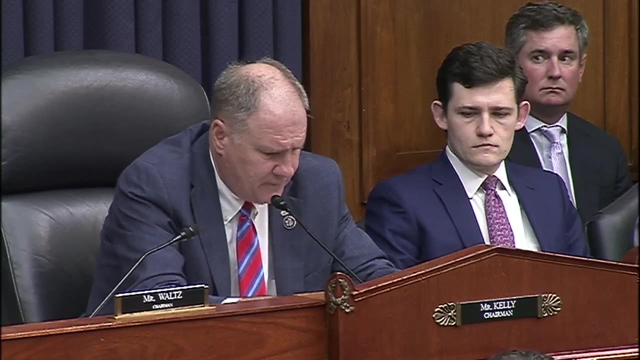 I do not have an assessment of the full cost. however, the Air Force does. Okay, If you could, if you can, provide that, just so that we have an assessment of that. I think that is very helpful for us to understand. And then, General Van Ovos, how is a contested environment expected to affect Transcom's? 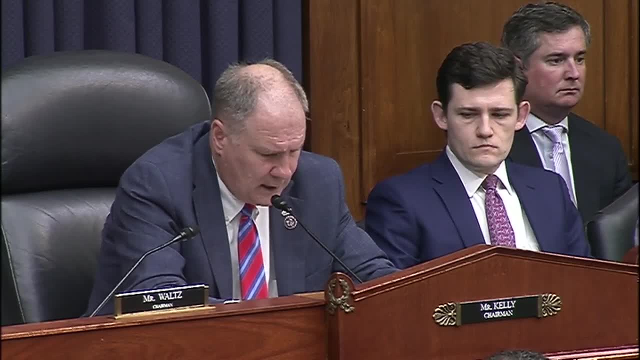 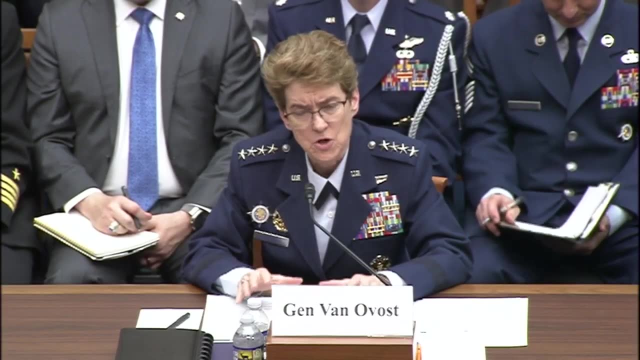 ability to use the Ready Reserve Force as well as commercial contractor logistics partners. more broadly, The contested environment is going to require us to be able to communicate securely with civilian and military assets of the fleets And therefore we are working on installing security. 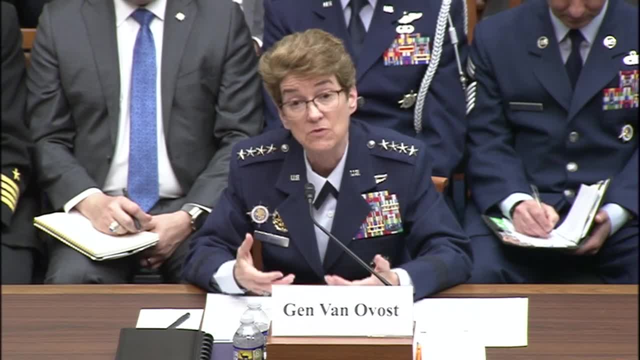 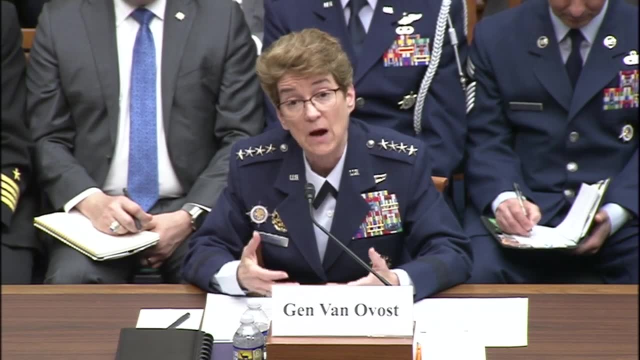 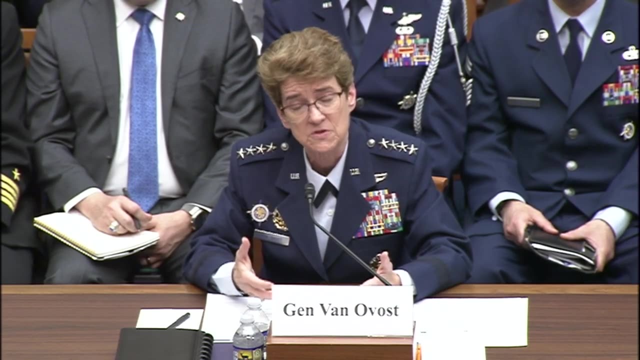 Okay- Secure communications on the Ready Reserve Force ships, as well as working with our commercial shipping to try to understand how we're going to get them information. We have been learning a lot with respect to the Red Sea as we are doing escort operations for US flagged ships. 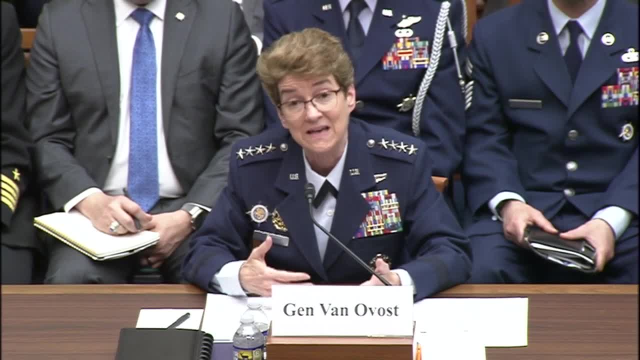 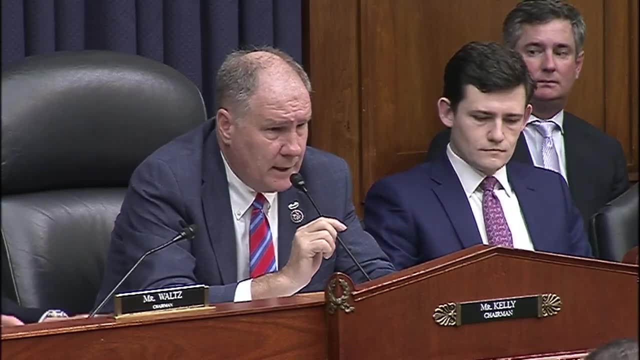 And so we're taking those lessons learned and we'll be folding them into what we're doing in the Indo-Pacific for communications with them, And I'm going to seize some of my time back, but I want to thank both of you for being here today. 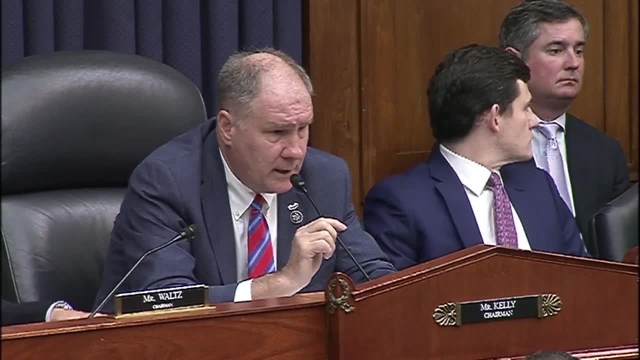 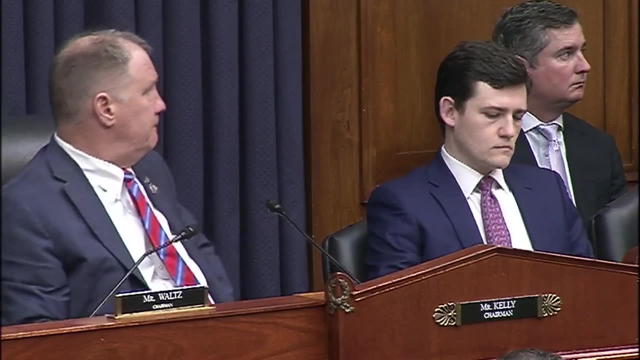 And I want to thank you for the visit in the office yesterday, where we talked much more deeply. And, with that being said, I now recognize Ranking Member Courtney. Thank you, Mr Chairman, And this is a question, I guess, to both witnesses, which is that I think you know from your meetings. 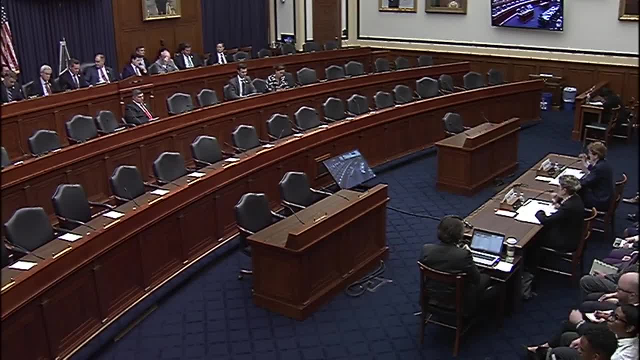 with members and you know past hearings that the subcommittee is very focused on the availability of used SELA vessels on the global market and in fact in last year's NDAA we directed Transcom and MARAD to conduct a market analysis. 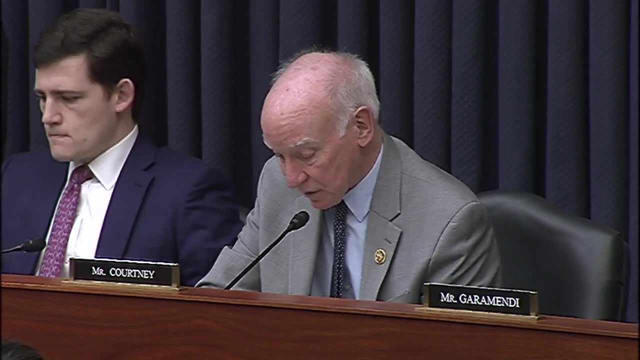 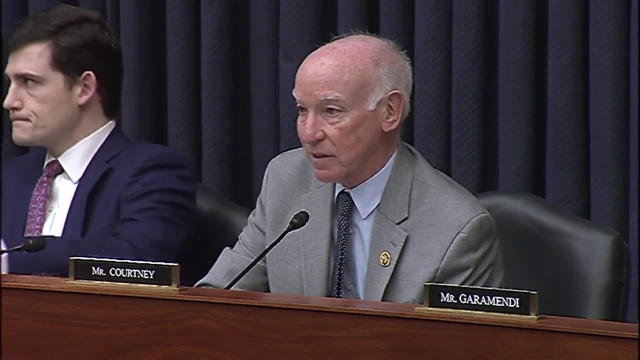 Thank you. So this is the SELA report that you had mentioned about the availability of used SELA, and you took a look at the reports and we're going to take a look at the numbers from the plan And they're all very important to have. 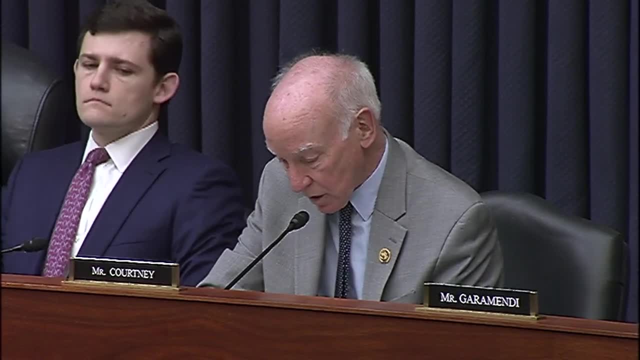 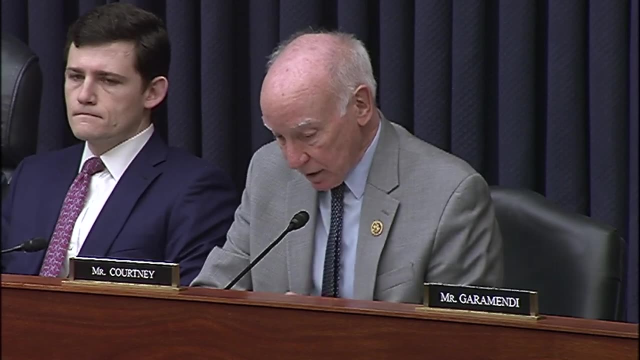 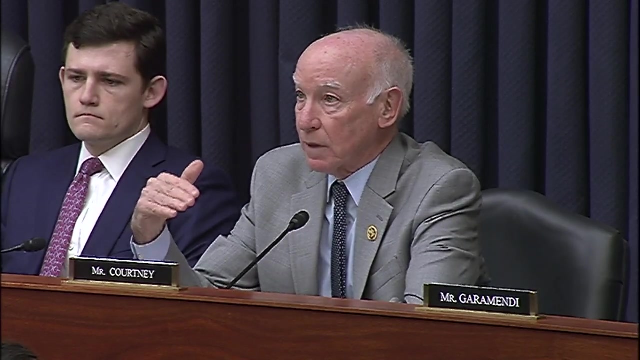 So this is the report of the SELA report and they're very useful for this increase in the availability of used SELA And I think these are some of the largest reports of those available to us in the United States And I want to see the results of that and I hope that these results will be helpful. 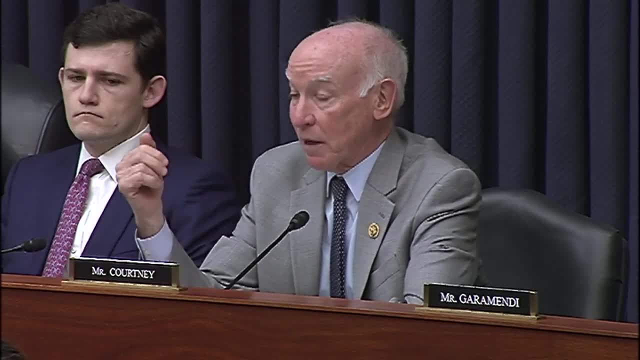 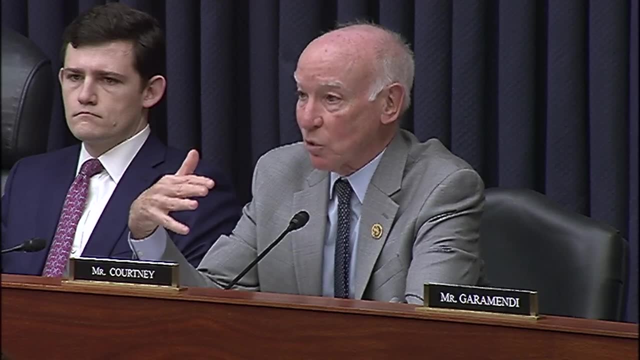 to the US economy. I guess the last prior round for about $90 million a boat. Is that correct? Yes, sir, All right, But that doesn't represent the total cost because there's an additional cost to actually convert that used vessel to meet your specifications. 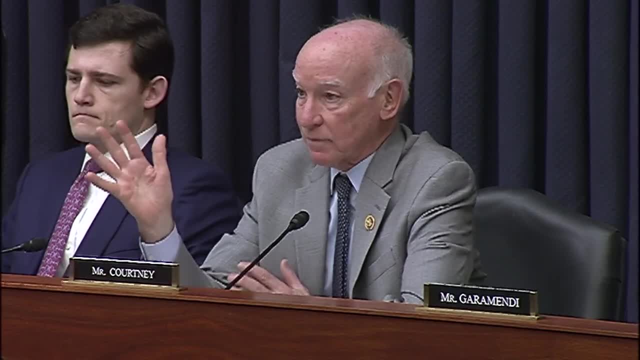 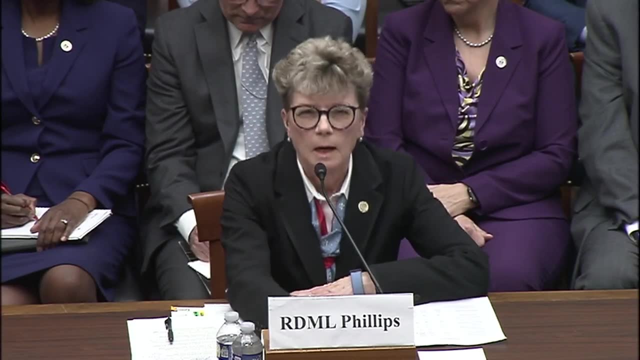 There is yes, sir, And can you give us sort of a round, some kind of estimate in terms of what that number looks like? I think I would take that question for the record, sir, to be absolutely certain that I give you a good idea. 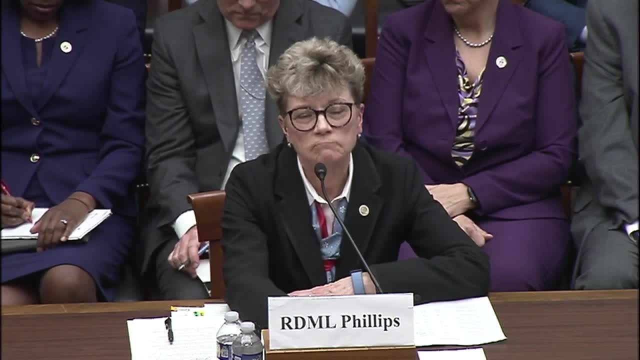 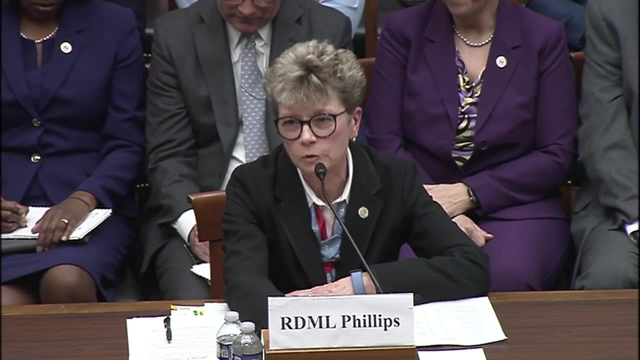 But it is certainly on the order of between $10 and $20 million for the Jolly class vessels, And that again I'll take it for the record so we give you an accurate number. Well, we do sort of need that number and I appreciate your willingness to share that with us. 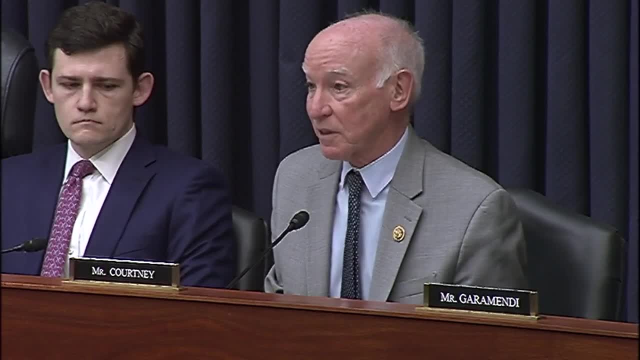 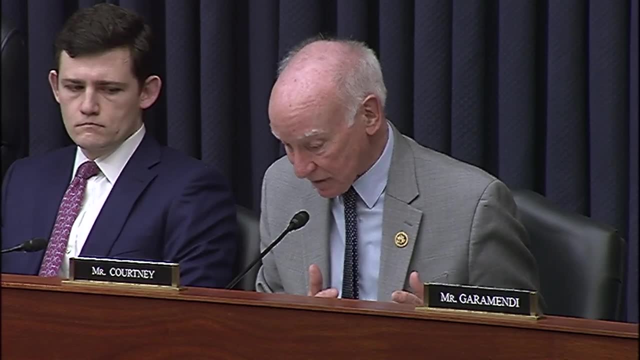 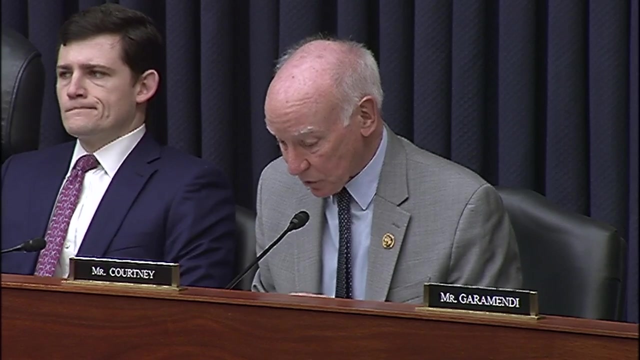 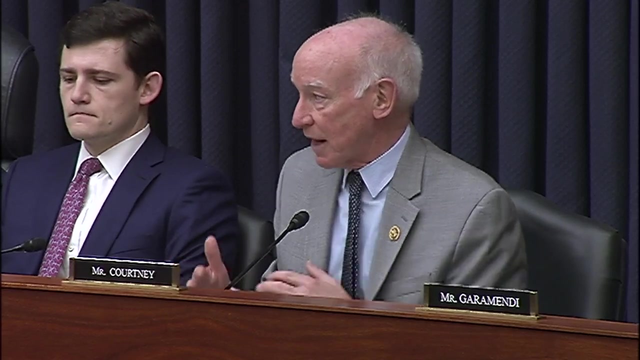 I mean, we've heard $20 to $30 from some other folks that have visited The office, our offices, Because, again, just sort of going back to the math of last year's spending bill, in FY24, Congress appropriated the request of $142 million for two vessels, which, again, if you take $90 million and add the conversion cost on top of that, 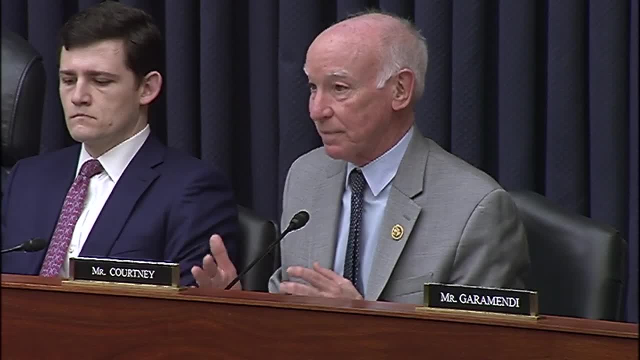 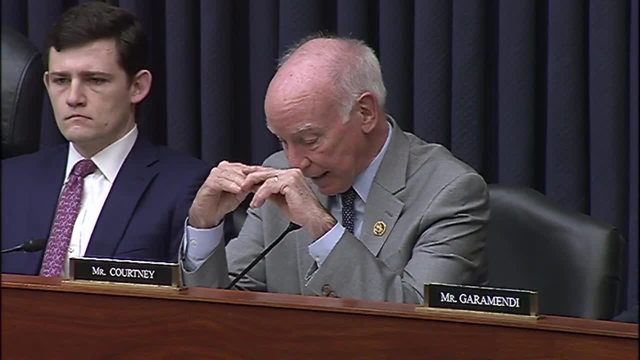 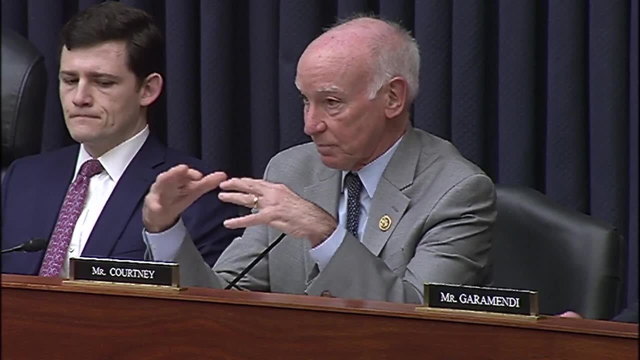 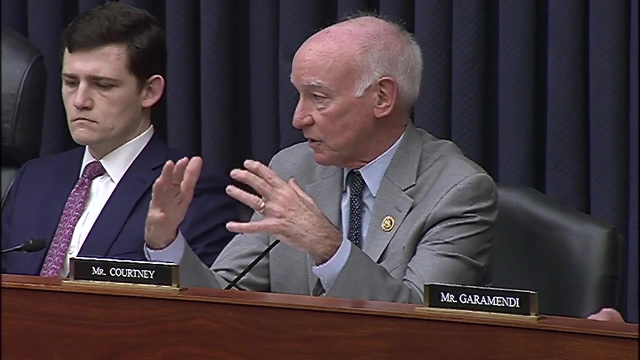 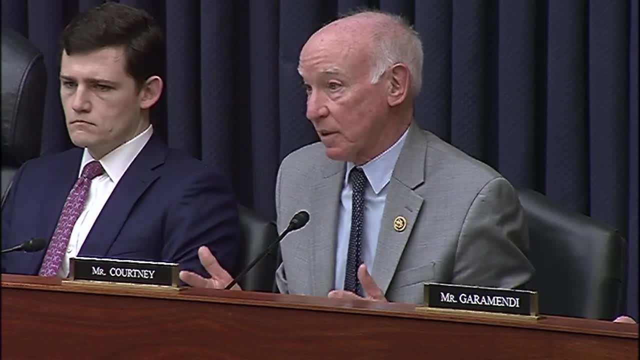 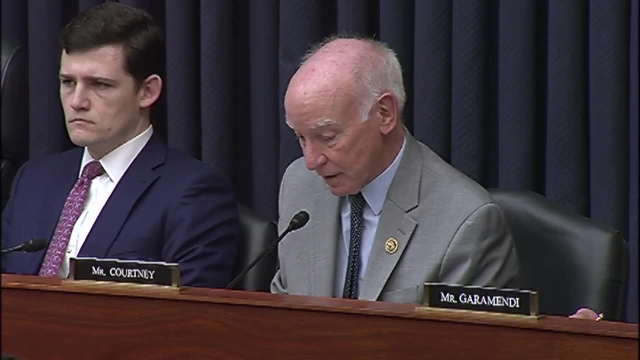 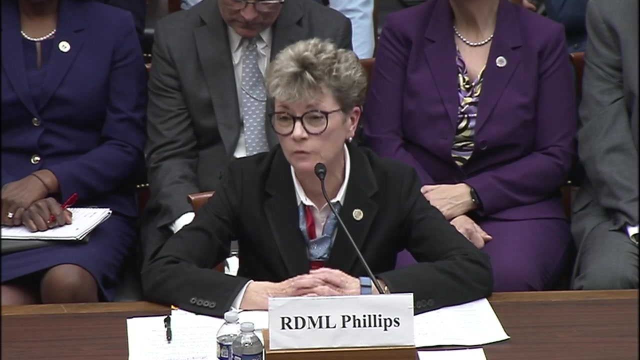 So again, do you feel that you can use last year's spending appropriation to buy two vehicles and convert them? Right, Right, Right? We do think that we will be able to buy two vessels with the appropriation that we have and start the conversion process, and hopefully complete it as well, using those funds. 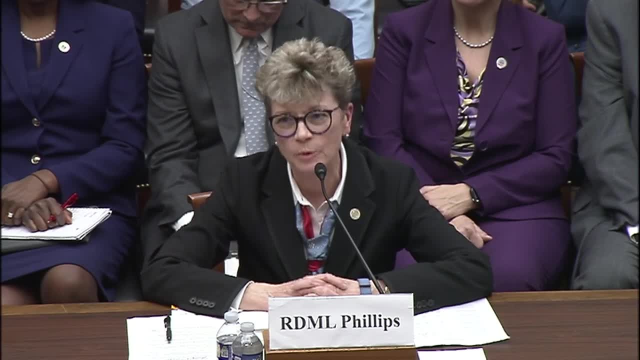 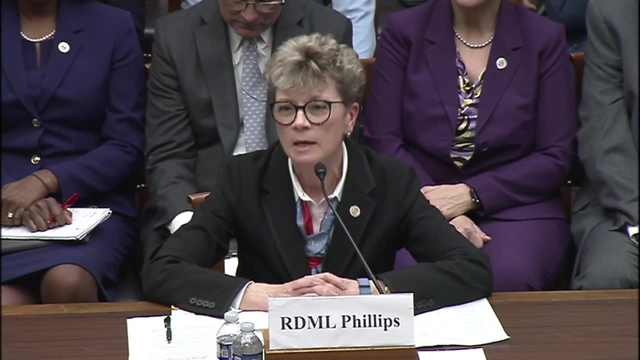 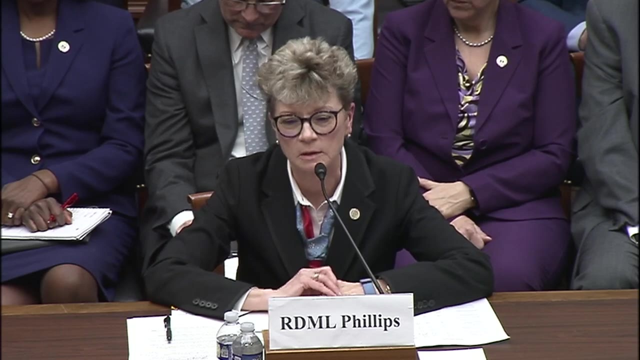 But I would add that the key is: newer vessels cost less money to convert, And when we buy older vessels, we find things that we didn't know were there. The alternate compliance program is quite strict And we find ourselves in a similar situation to where we find ourselves with the ready reserve, sometimes chasing our tail, trying to catch up with things that have been in existence for a very long time. 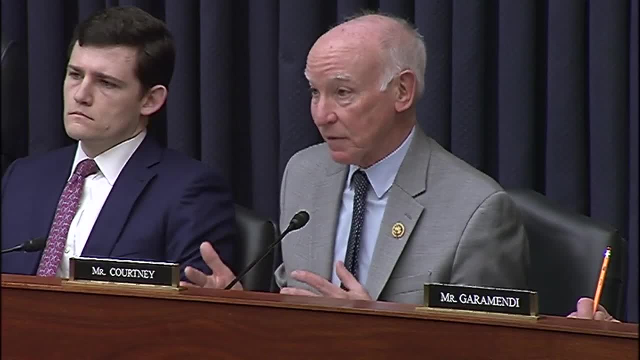 And that adds to the cost. No, and I think that describes the dilemma well Again. the problem is that we just don't know what's in the market from one day to the next in terms of whether older or newer are actually available there. 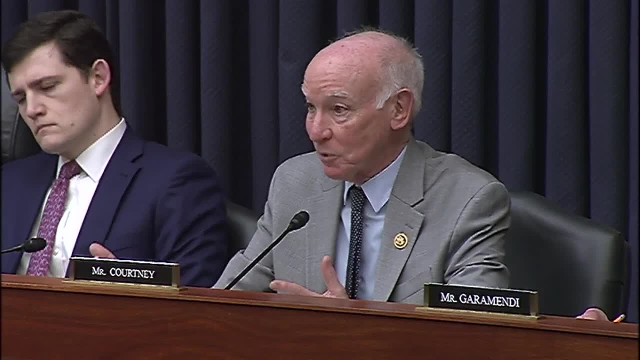 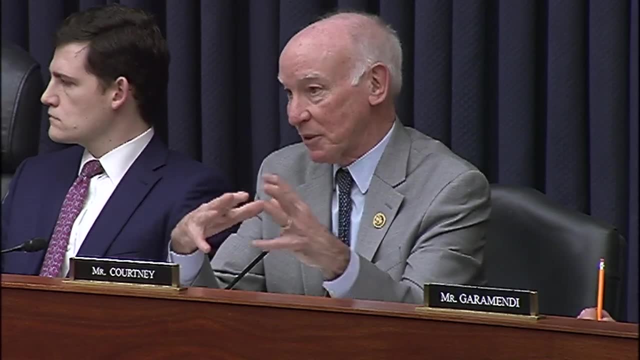 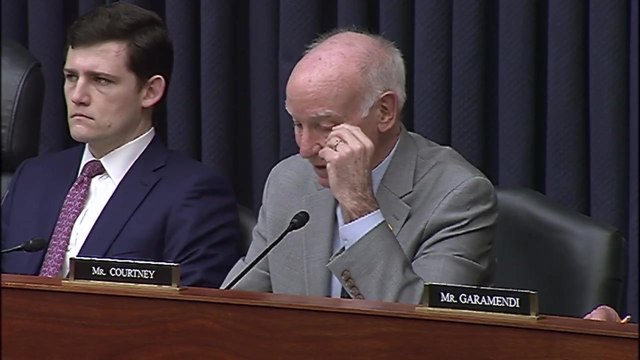 So we did provide money for design of new sea lifts, as you point out And as I mentioned, it seems like the vessel contract, The vessel acquisition manager model, seems to be something that people are embracing. I think it was in both of your testimonies. that's there. 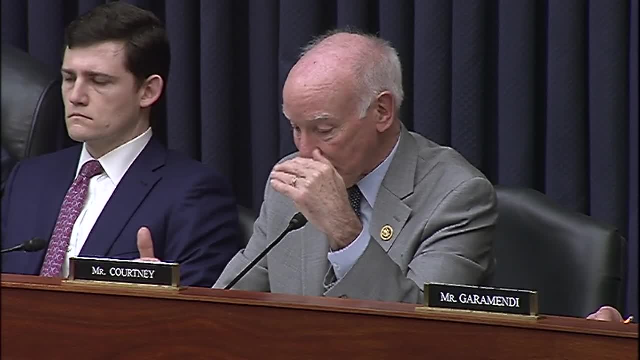 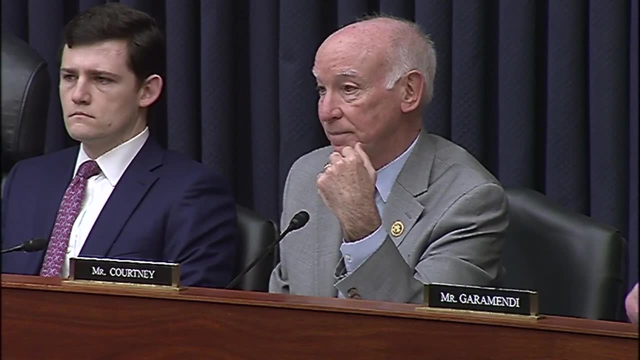 So if we were to give you the money for a new build sea lift program in this year's budget, could you put that on contract in FY25?? Sir, I think it would be a stretch to put it in a contract in FY25 without having 100% design at this point in time. We would have to have 100% design and I would estimate roughly two years to be able to get it under contract, Because I don't want to overpromise something that I can't deliver. Okay, Again, that's helpful and it's a question that I think we're going to keep asking. 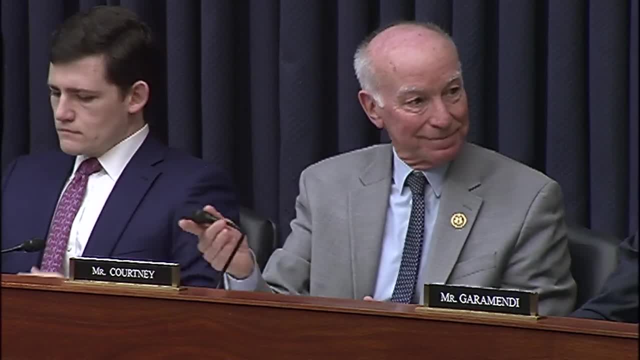 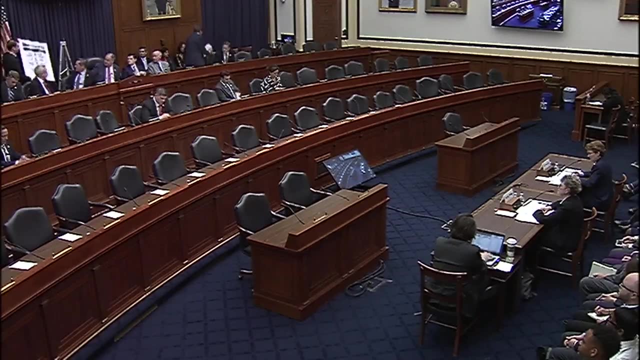 Okay, With that, I yield back. I now recognize Chairman Waltz. Thank you, Mr Chairman, and forgive me trying to get a sign up here, But I think this visual is powerful. We're all aware of Chinese Communist Party. 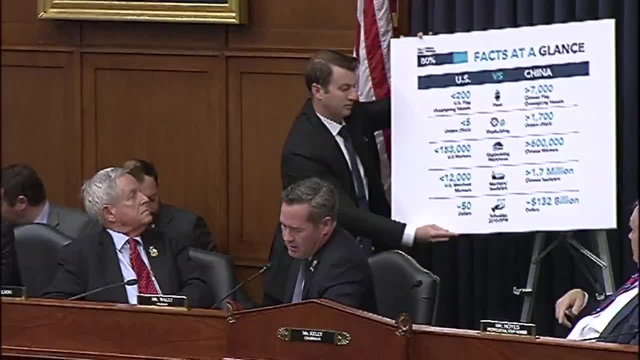 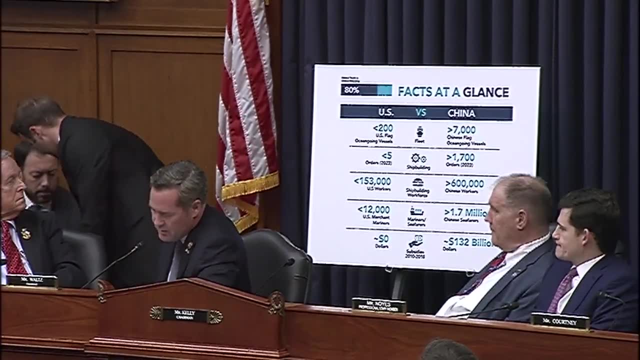 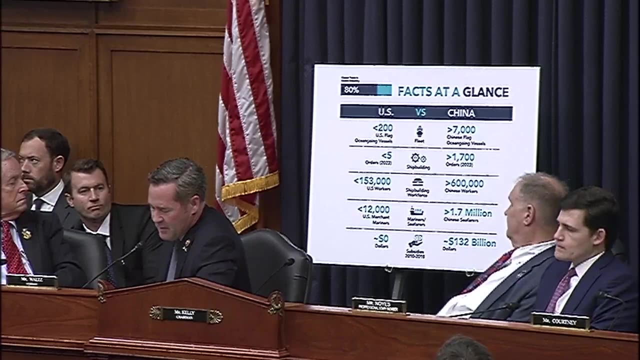 We're all aware of Chinese Communist Party influence and how far the People's Republic of China has come and its influence over shipbuilding, over shipping, the industry, maritime infrastructure. It's to the point where I think the People's Republic of China could exact economic warfare, economic coercion on the high seas, even during peacetime. 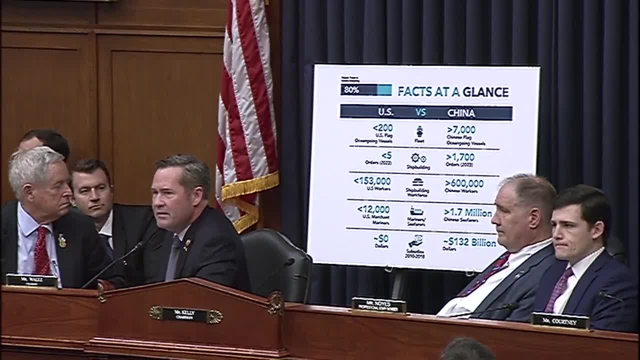 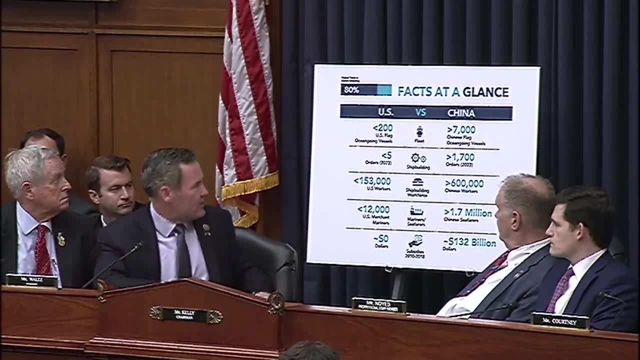 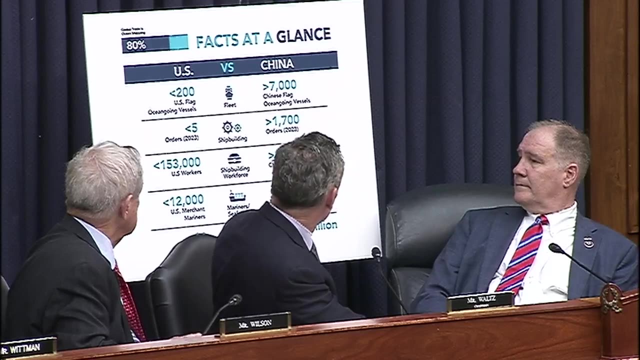 And when we see the PRC with 50% of the civilian global shipbuilding capacity, that's. That is incredibly concerning. And just by point of some numbers here: 7,000 Chinese-flagged ocean-going vessels compared to less than 200.. 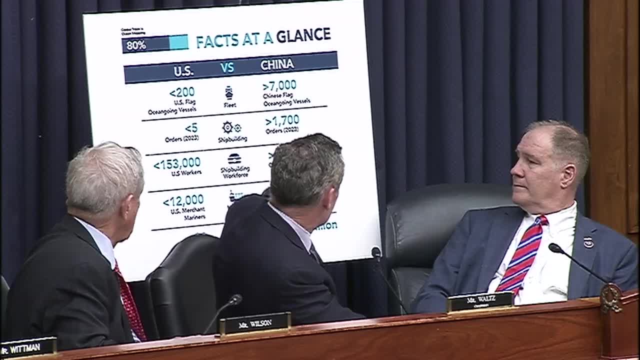 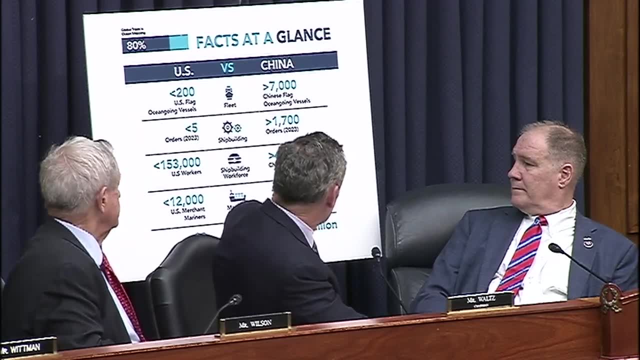 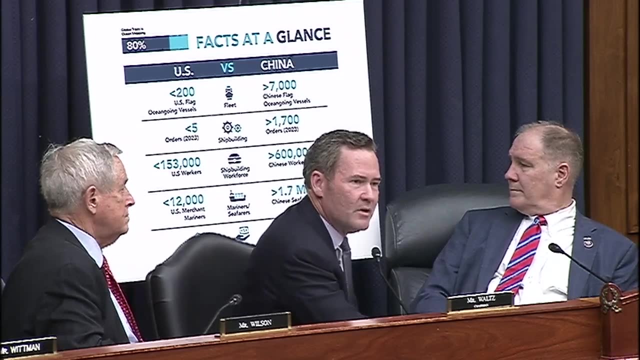 1,700 orders last year that the Chinese are going to build less than five. The people, the American people, need to understand this: 600,000 workers, 1,500 ships, large ships. they're going to build, We're going to build. 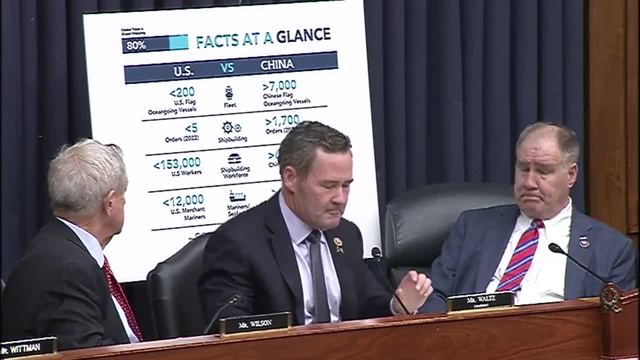 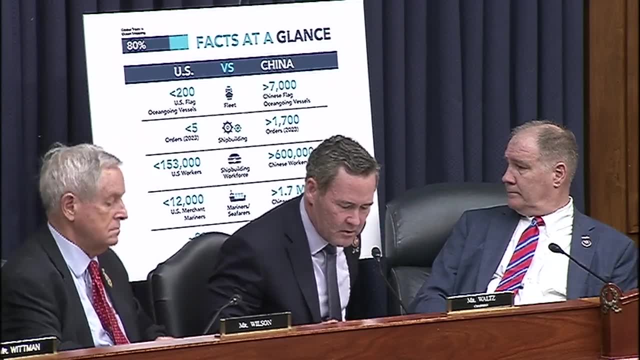 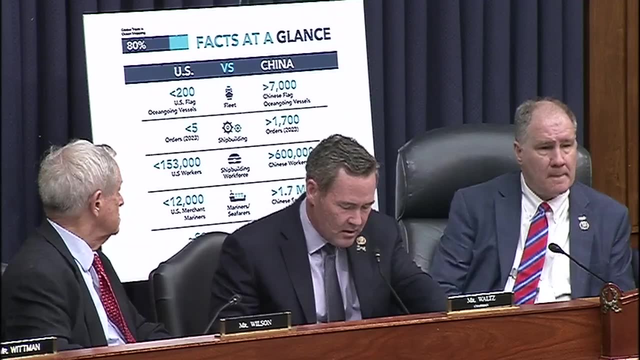 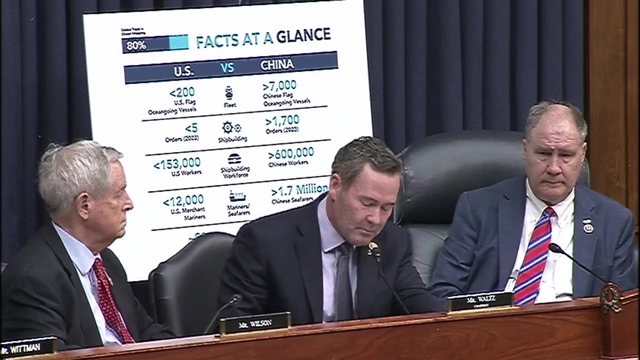 Mr Chairman, we're going to build 20.. So I think you are both aware of the recent petition filed by the administration advocating for an investigation into unfair and uncompetitive practices by the PRC and the maritime sector Behavior. I believe that the CCP is doing as part of a long-term strategy to basically make it nearly impossible for the US to build or operate ships that we need. 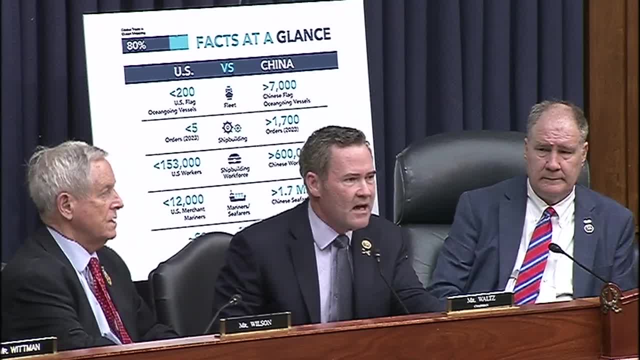 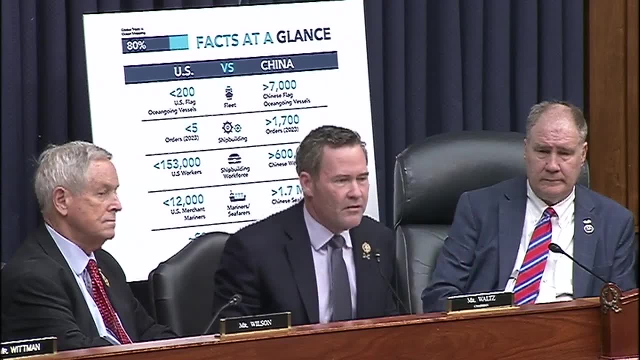 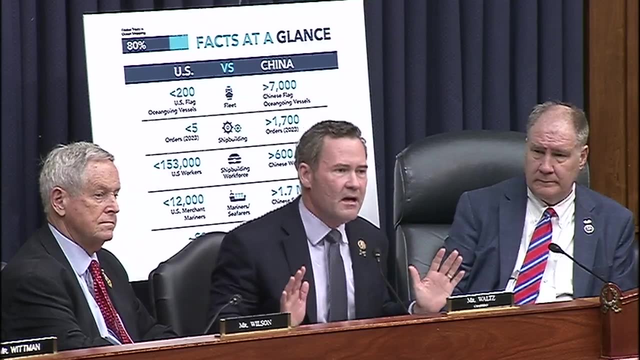 Not only for economic vitality, but to support our warfighter. Admiral Phillips, I'm going to give you the floor on this. What policy decisions and resources does MARAD need from Congress to help the maritime sector rise above these challenges? This is an all-of-society. 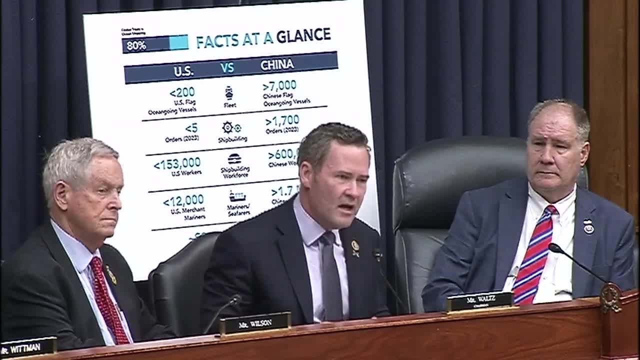 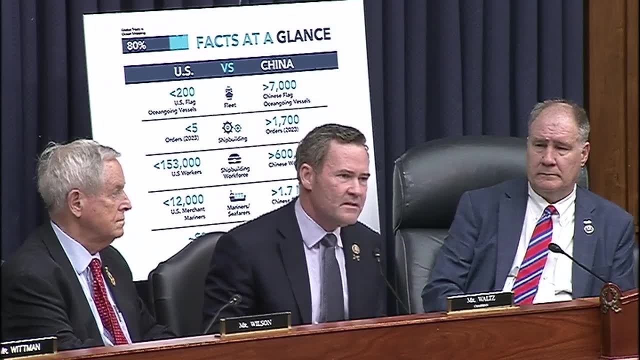 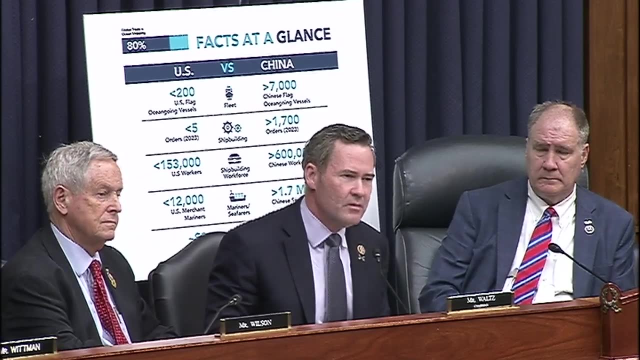 This is steel, aluminum, shipyards, dry docks, workers, wrench turners. We've asked for a national maritime strategy. My office, in concert with others, both the House and the Senate, have issued our thoughts on it. Talk to me about how we get here as a nation and start digging ourselves out of this hole. 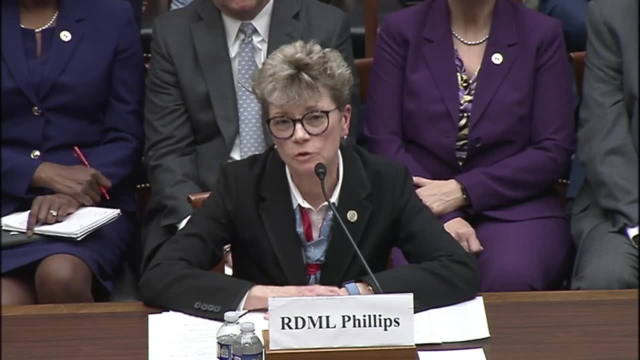 Thank you, sir, And thank you for the opportunity. What we need is a clear signal from Congress that this is a serious issue, that you take it seriously- which I know you do- and that you are intent on finding solutions. By that I mean I will frame out: 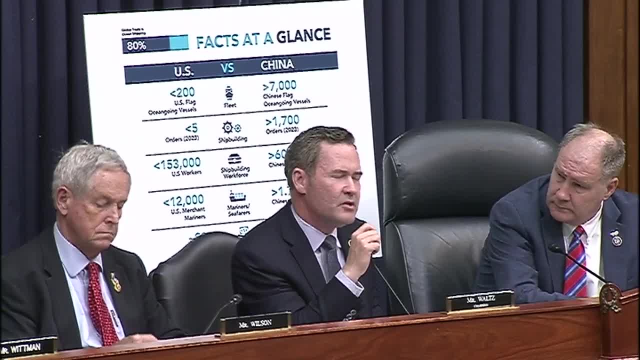 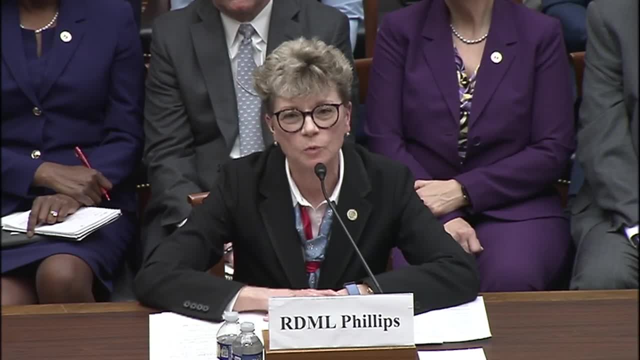 How about if I can just interrupt you? how about if we gave you a separate budget line? Is that a clear signal? It is a clear signal, sir, And of course appropriations would be required as well, But to put a fine point on it, with the ready reserve, as you have mentioned. 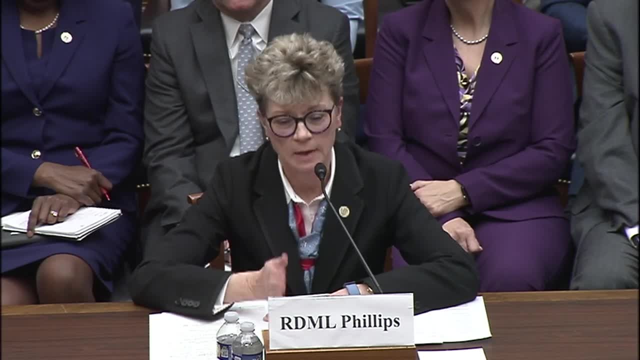 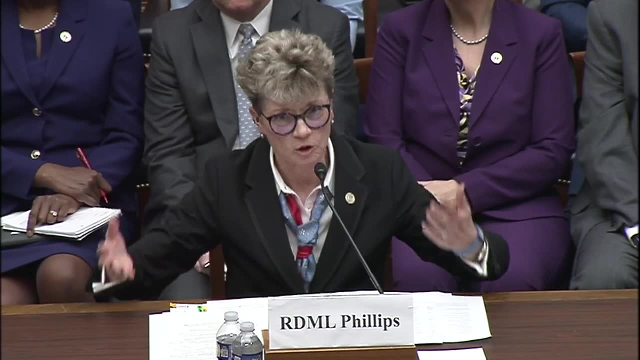 at the end of 25, I have authority to buy four more ships and then I'm done. I have $12 million, for which we thank you, to do a design for a sealant vessel, But we would need additional appropriations, authorizations and capacity. 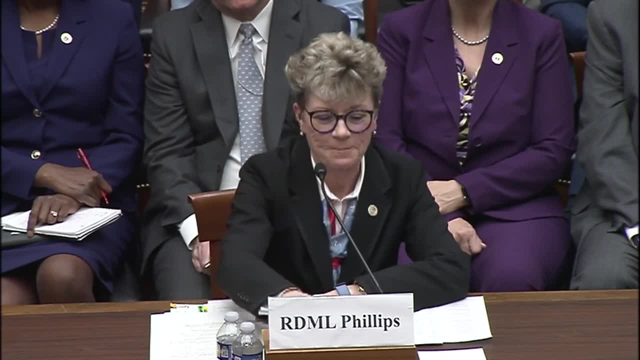 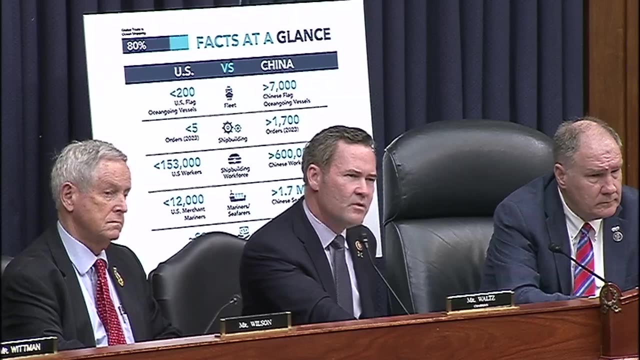 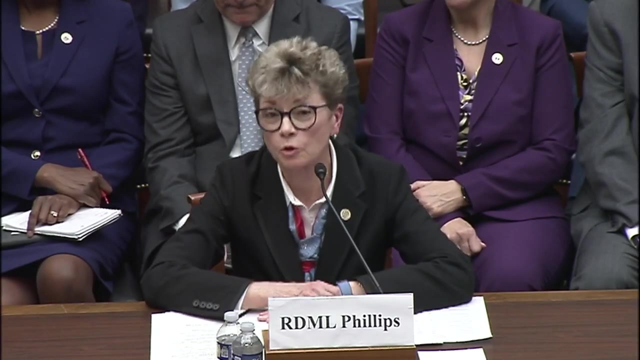 We need to move forward from there. Correct me if I'm wrong. In the first Gulf War, approximately what was it about? 400 ships that took our ground forces over? Now you're sitting on 40 to 60? Well, that also would have included, sir, the commercial vessels that were available. 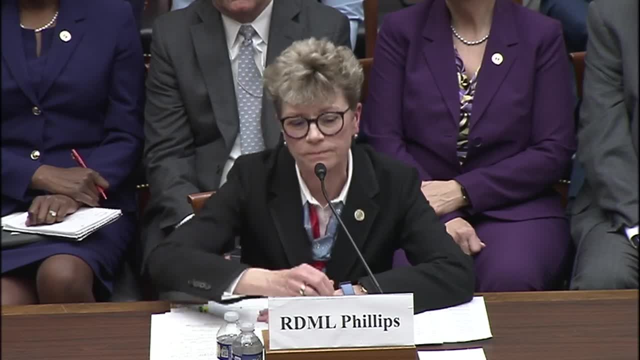 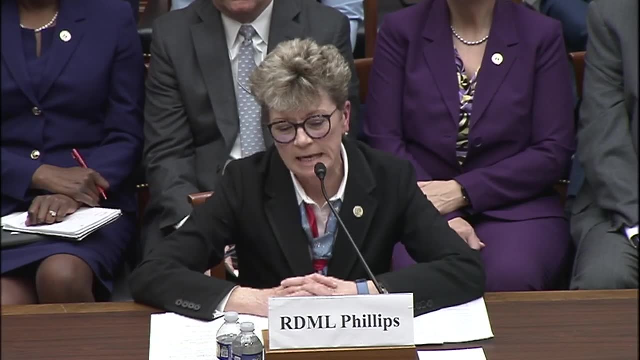 but they were approaching 200 ready reserve force vessels at that time. Okay, Keep going, though. What do we need to do? What else? Clear signal, Yes, sir. Clear signal with intent to move forward. Clear signal with intent to move forward. 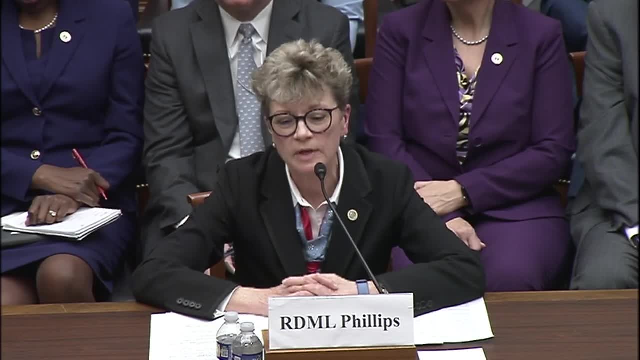 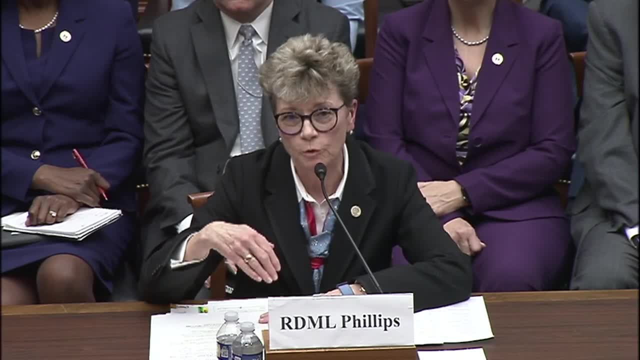 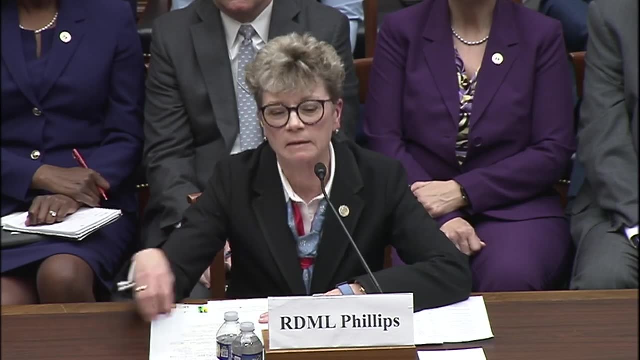 And this could include not only building, but it could include programs that are similar to things that we've done before, where we have either built and then leased, or leased and then we provided the leases as the US government and industry built to meet those leases long-term. 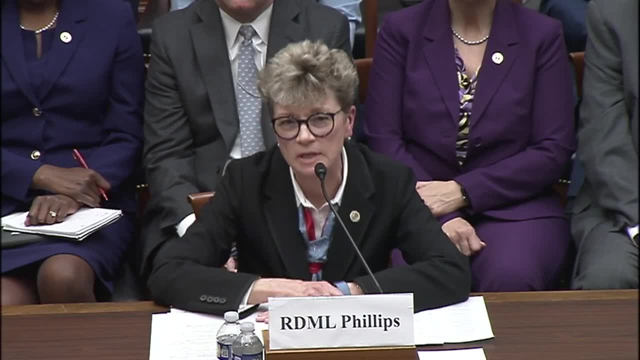 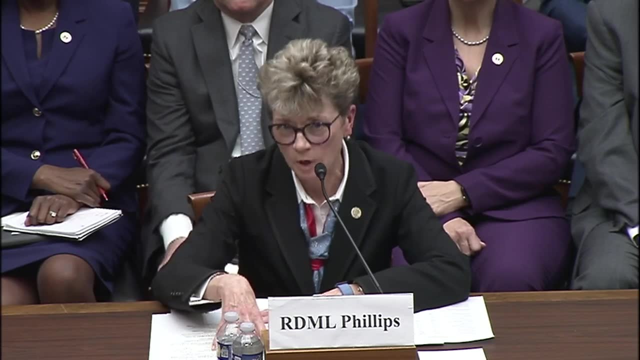 It would be a 20 to 25-year commitment. Those are options or ideas for things that could be considered for the future. But what comes with that is, of course, a clear signal that we care this and we're going to move forward. support from congress to make that happen- that also, of course. 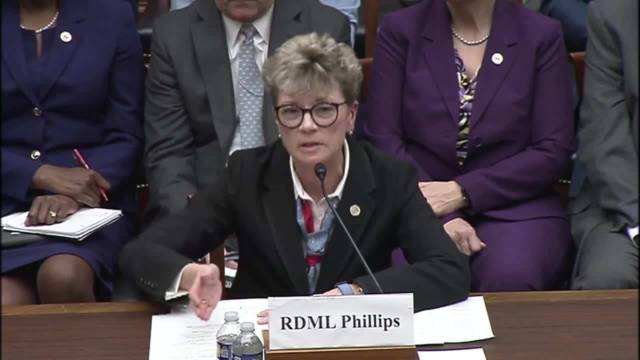 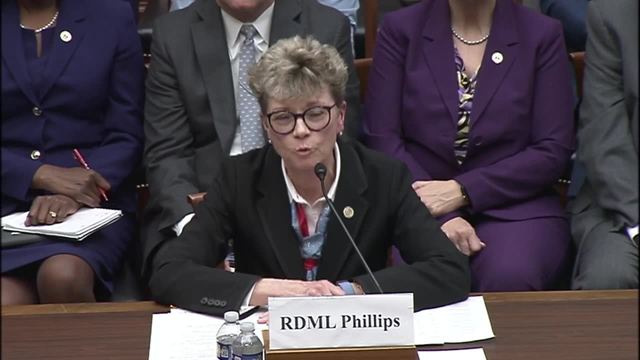 impacts our ability to provide crews too, because then the industry sees: aha, i have a future here, i have a way to move forward. without that, we have the, we have the fleet that we are authorized and appropriated to have, using the cargo preference laws that we have, and our and our dod cargo. 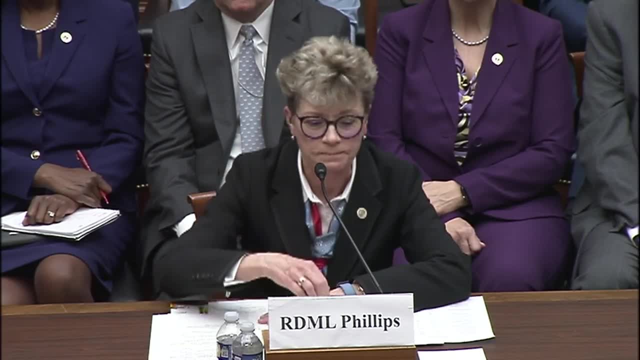 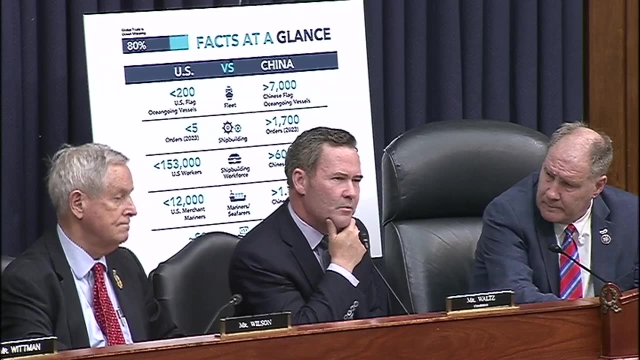 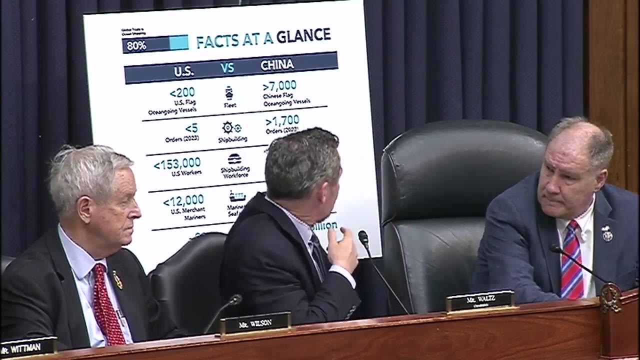 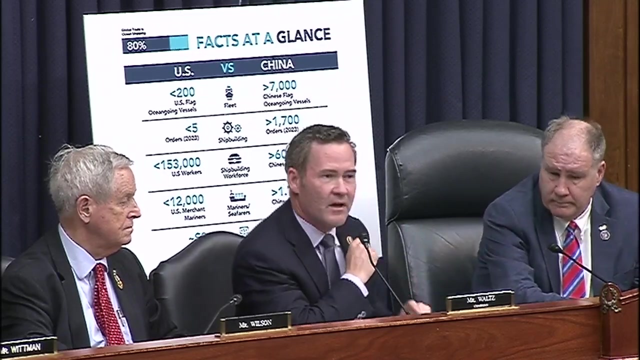 requirements over time, which is what largely supports what we have today. i think there's a the, the chinese communist party, now has the largest navy in the world because they have the largest civilian shipbuilding industry in the world. and those thousands of ships, every one of them can be a warship just like that, and i think we are have. 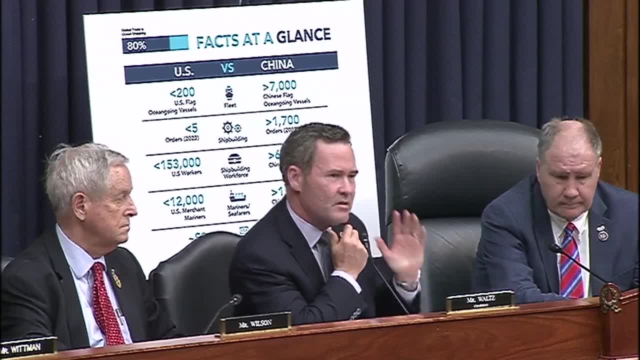 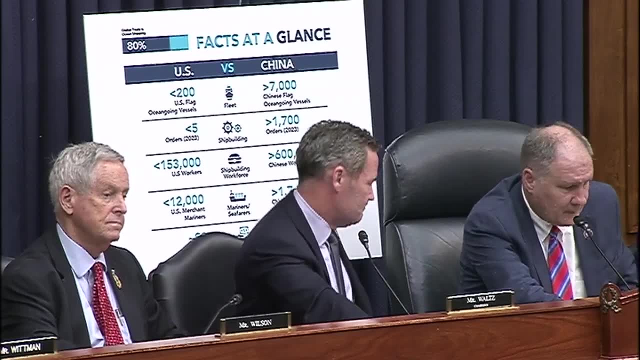 talked about. we've talked about this sea lift, recapitalization, this issue since i've been here. but, mr chairman, i think it's time both of these committees start moving out and support america. thank you, gentlemen's time's expired. i now recognize, uh, mr garamendi. ranking member garamendi. 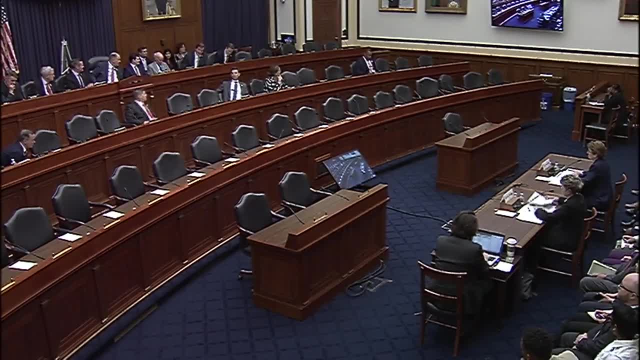 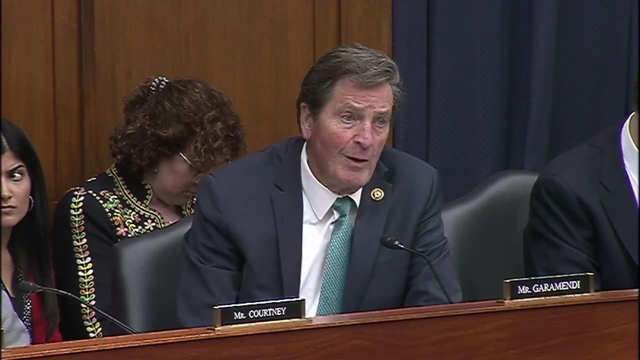 chairman waltz is marching down a path that i have just given the rest of my time. it's interesting to note that those used ships that you're about to buy- uh, the owners of those ships will take that- was it? 90 million dollars and then go buy a chinese-built. 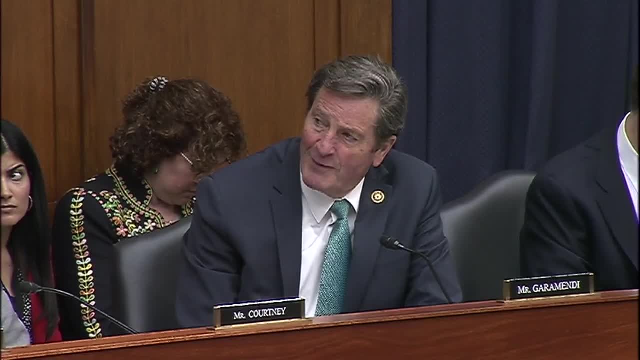 ship and then go buy a chinese-built ship. the owners of those ships will take that- was it 90 million dollars? and then go buy a chinese-built ship. i'm trying to figure out, mr walsh, how that fits into the concerns that you so adequately put. 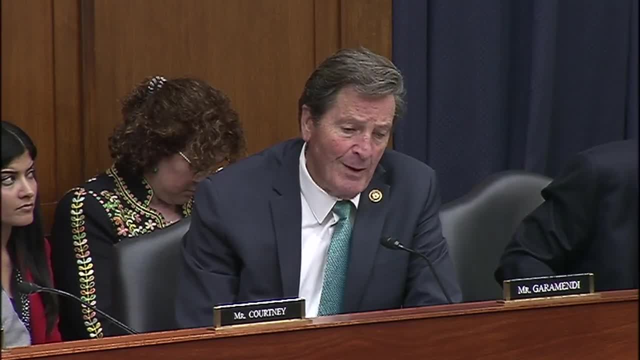 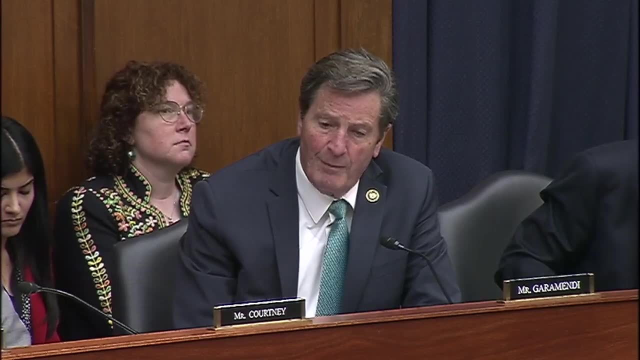 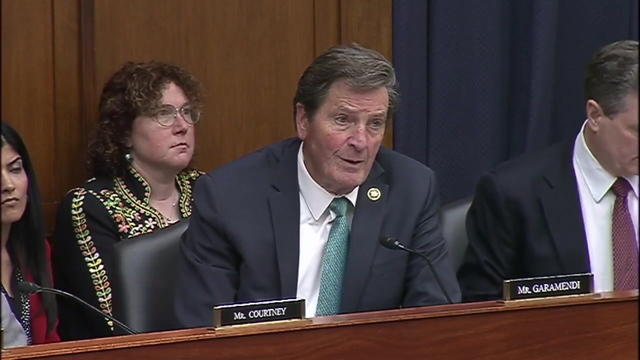 forward seems to me that we're headed down the wrong path. there are strategies that we really can and should put forward. bottom line of this: until we authorize and appropriate, we're not going to succeed. now there's some ways we can do this less expensively. i'd like to say on the cheap, but just less expensively. 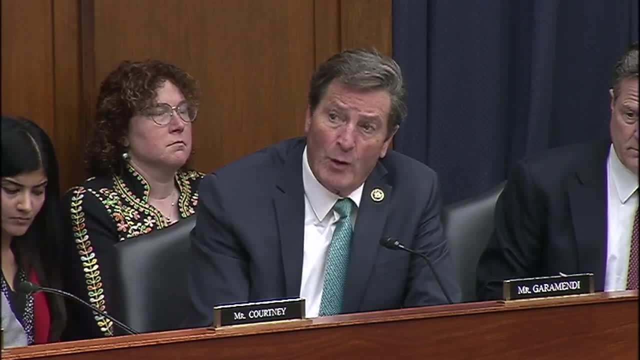 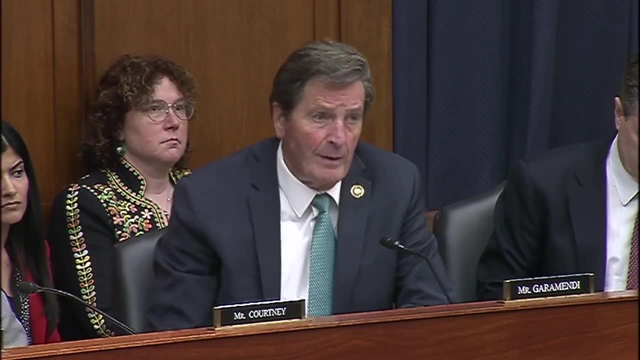 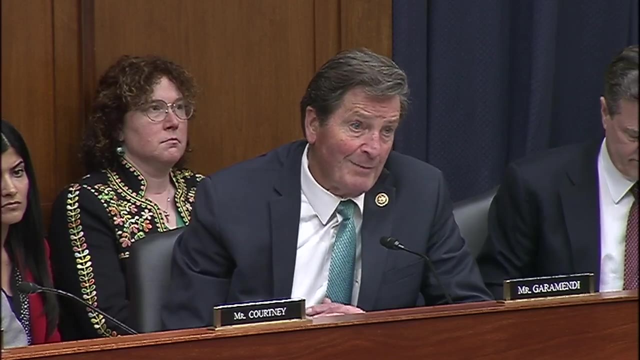 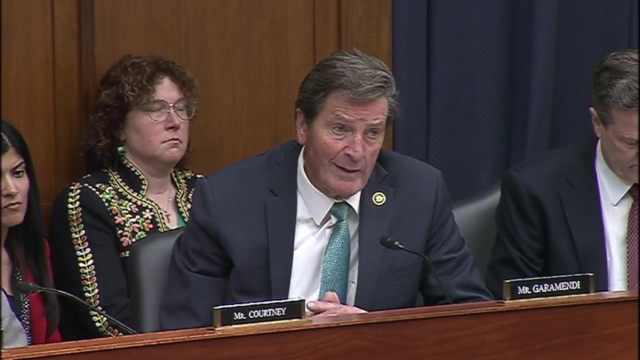 for example, we're going to need a lot of oilers if we're going to have a problem in the pacific. in fact, we need them today. the john l lewis ship runs what? just under a billion a copy. is that about right? we're not going to build many of them, however, if we were to pass a piece of legislation that 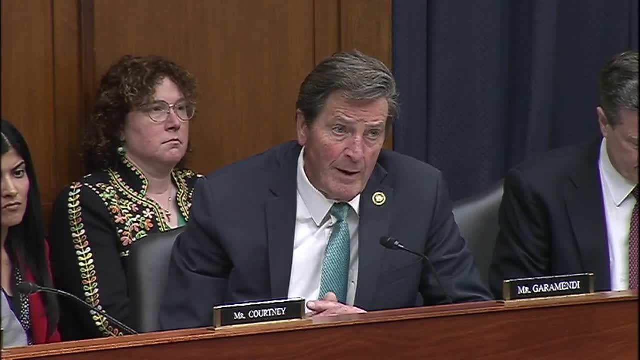 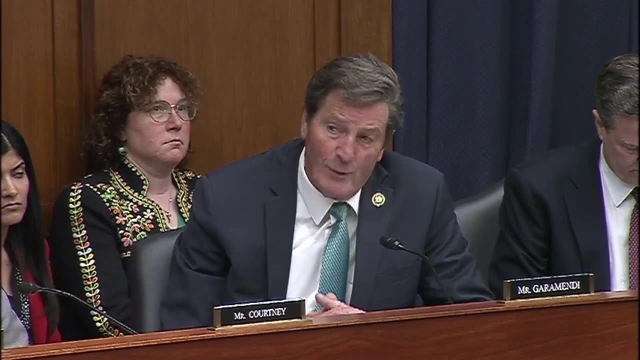 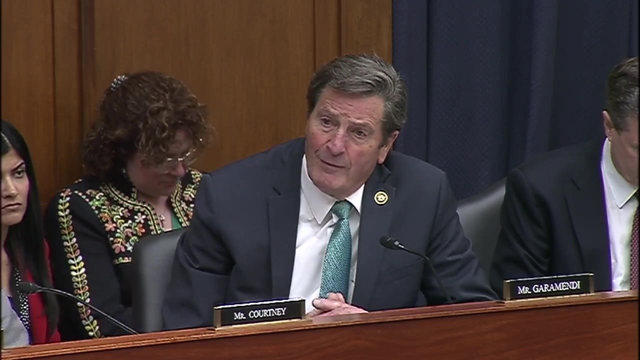 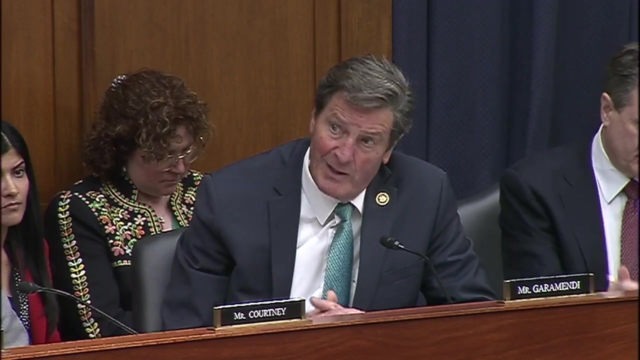 senator wicker and i put forward which is called the the american shipbuilding industry, admirals in general. this is not for you, this is for my colleagues. if we were to do that and say that 10 of the export of petroleum products from the largest petroleum product export nation in the world, the united states, was on american-built ships, 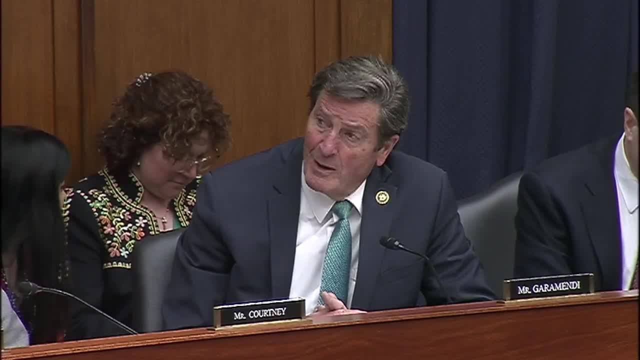 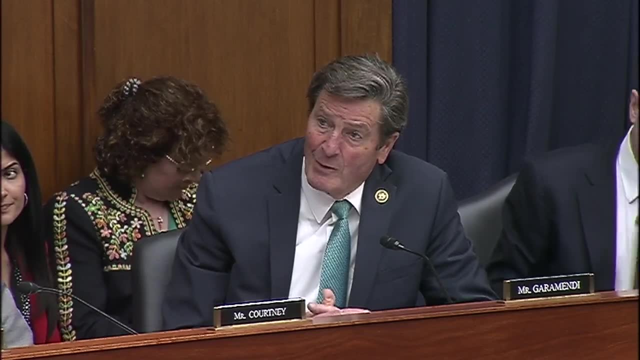 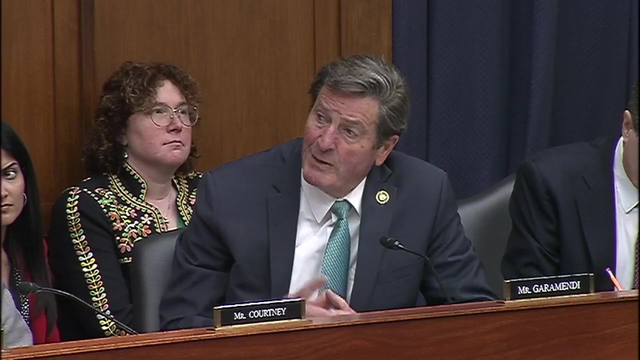 we would build probably 40 to 50 ships in the next decade to 15 years, energizing our ship building industry. the cost to the government? not much. however, we would want to put in a small requirement that those ships be- the word you use, mr walsh- militarily useful, have a king post in the 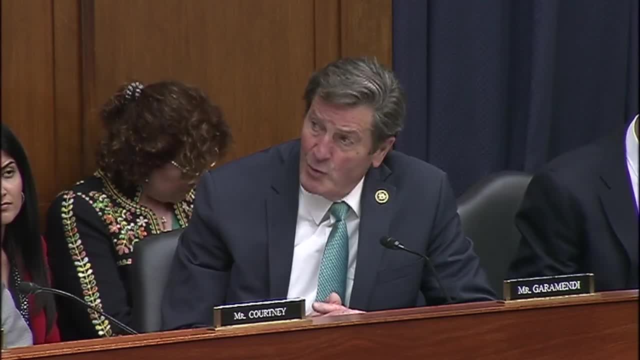 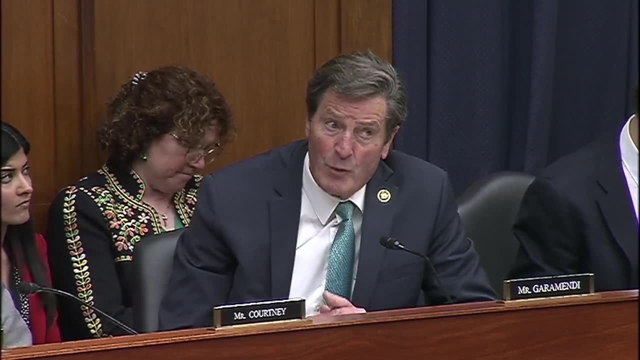 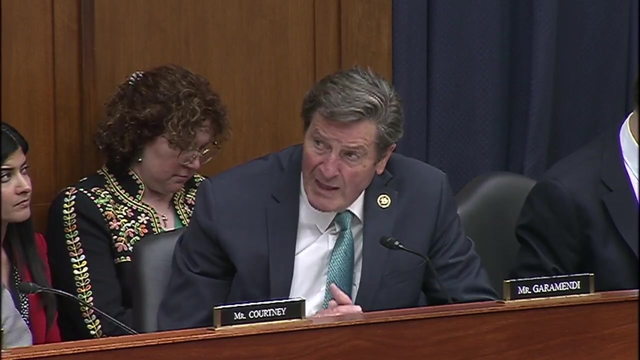 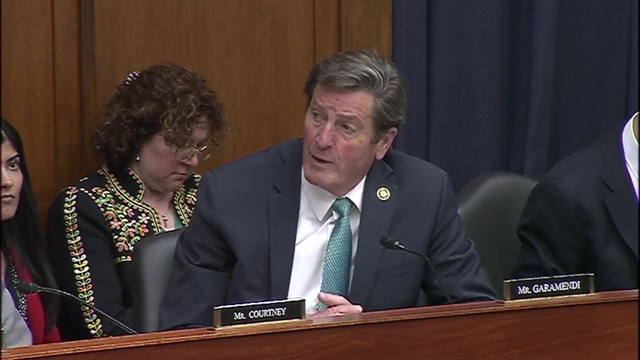 middle and some communication systems. we could do this by simply changing the law which we once had. all of the oil from the north slope in the original 25 years was brought to the continental United States refineries on American-built ships And then we allowed that to go offshore to other refineries over the years. 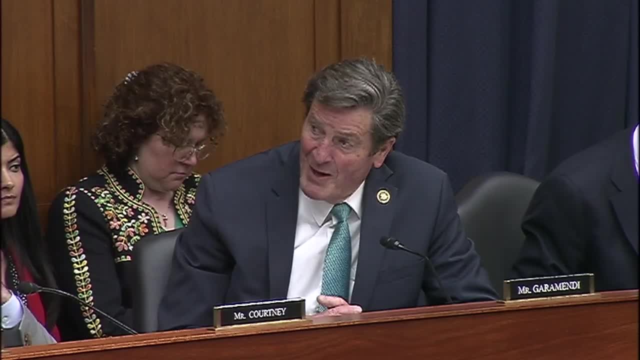 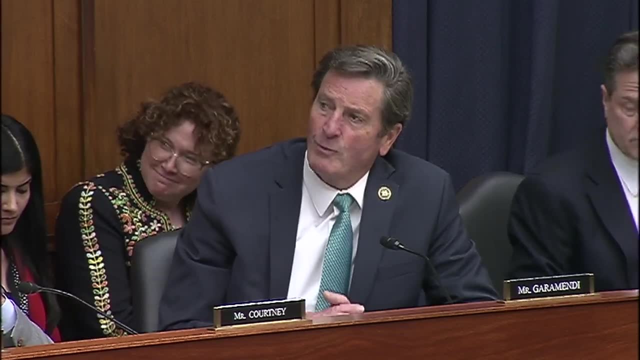 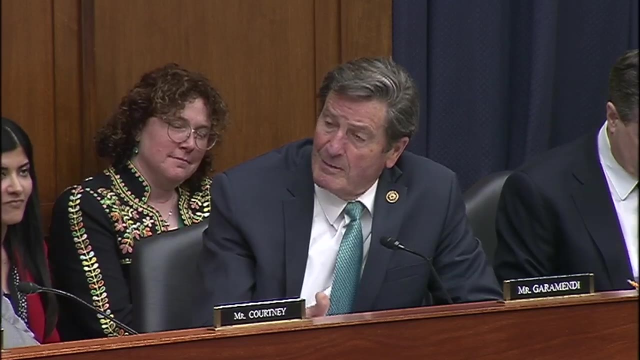 and then we did away with the ships And now we are where we are energizing the American shipbuilding industry. Anybody from Mr Wicker's state here There are ways we can do this Jones Act. Allow and use the Jones Act military useful ships. 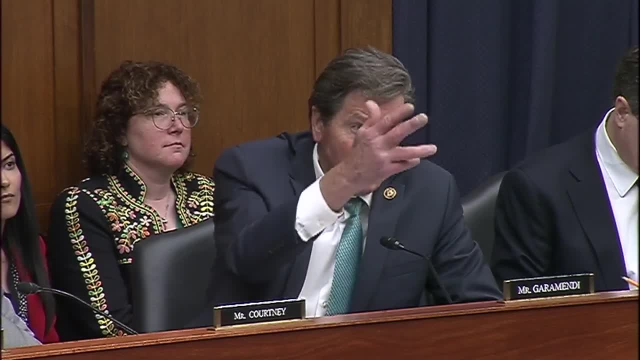 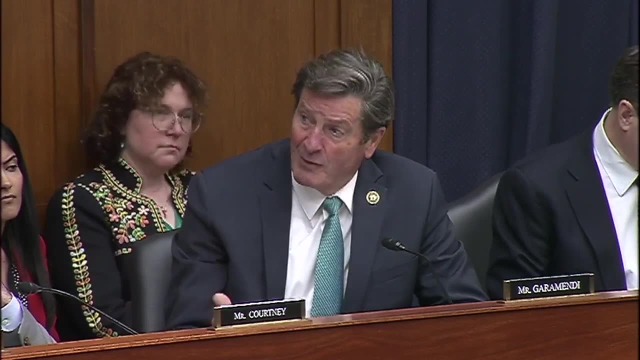 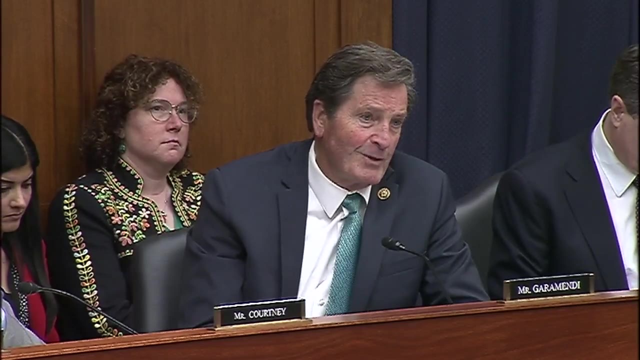 Add maybe 10%. We'll subsidize that, We'll give a stipend, as we do with the craft program, the aircraft program, and we can then build a domestic fleet, same time rebuilding our shipyards. Geez, I'm supposed to ask a question to you, to the witnesses. 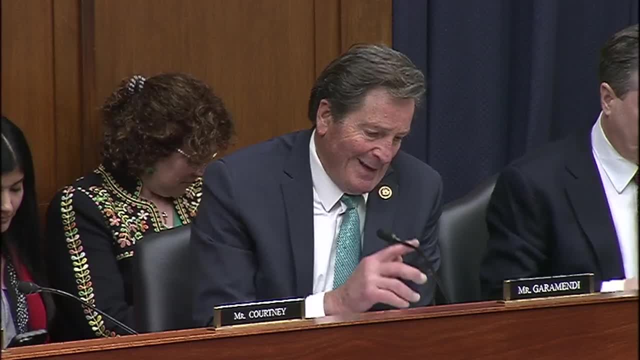 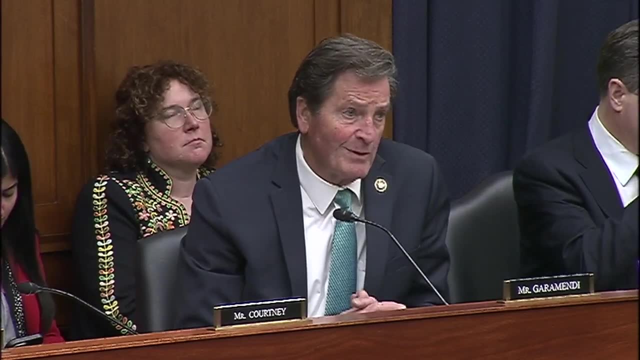 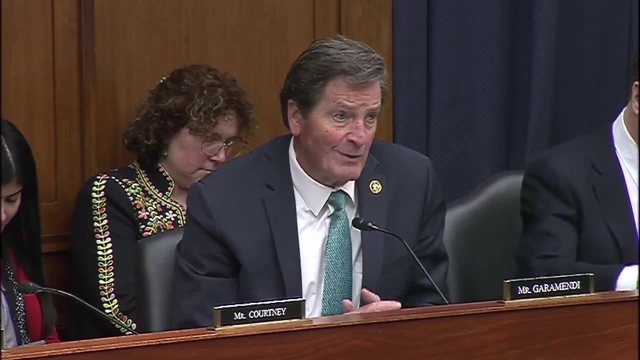 Forgive me, members, I don't know. You say you're agnostic, General Van Oost, You just need the ships. I don't like that reply, And you know why We've had this conversation. I want you to be an advocate for American ships. 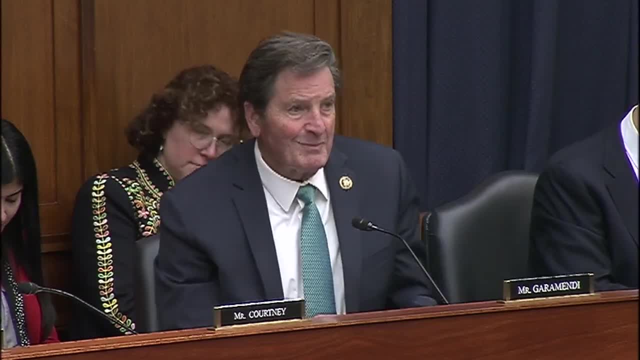 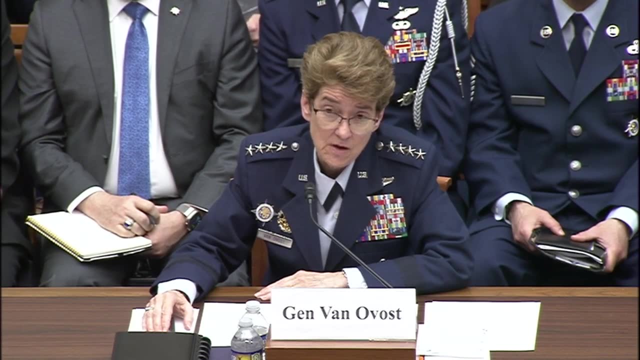 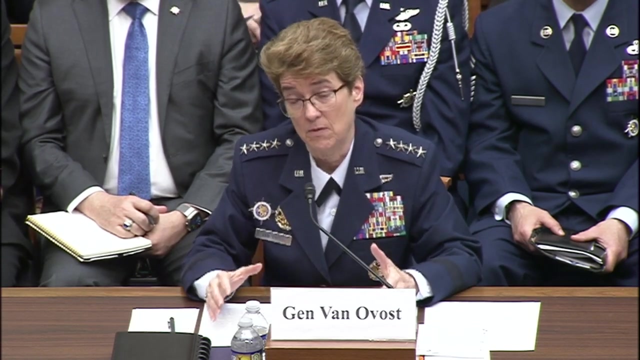 Can you do that? I'm absolutely an advocate for American ships and we owe you a comeback with Marriott. We owe it to the Navy to talk about a creative acquisition strategy that's going to support maritime nation writ large and be part of the national maritime strategy that Marriott's putting together. 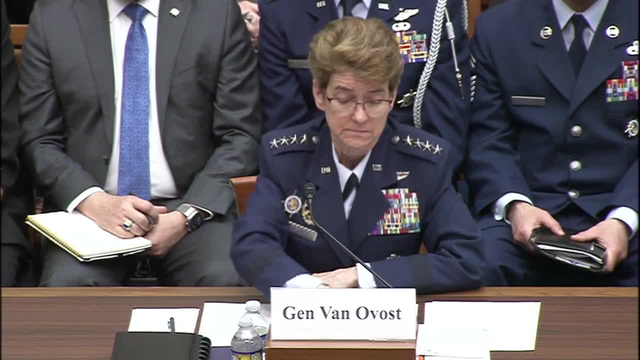 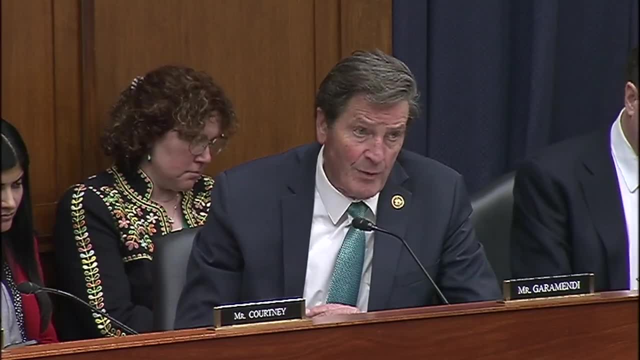 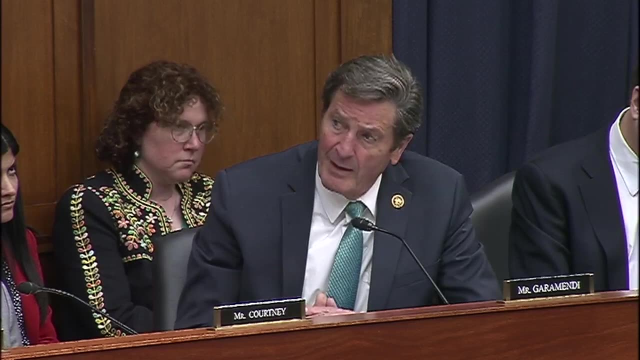 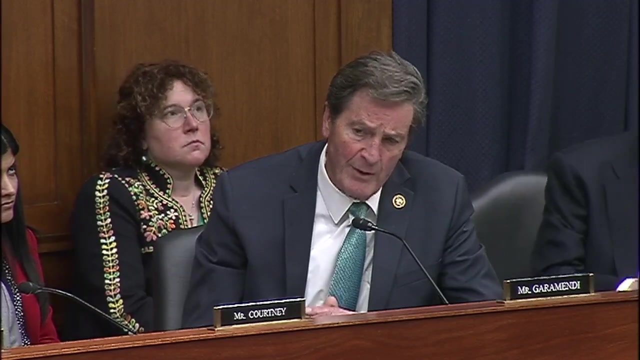 Thank you. I know that we talked earlier about the—my colleagues talked earlier about the mariners themselves- Obviously an ongoing problem, not only across almost every part of our economy. It's about pay, It's about knowledge And it's also about—in most of these cases- we have maritime unions- apprenticeship programs. 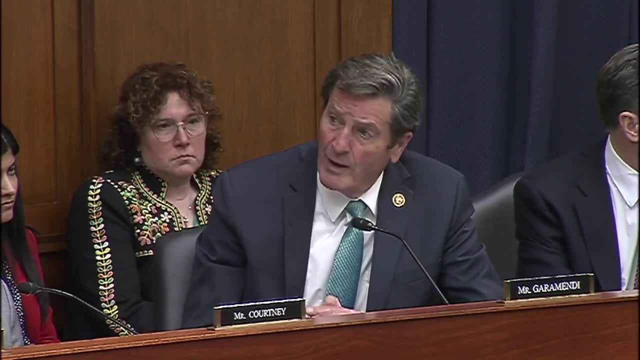 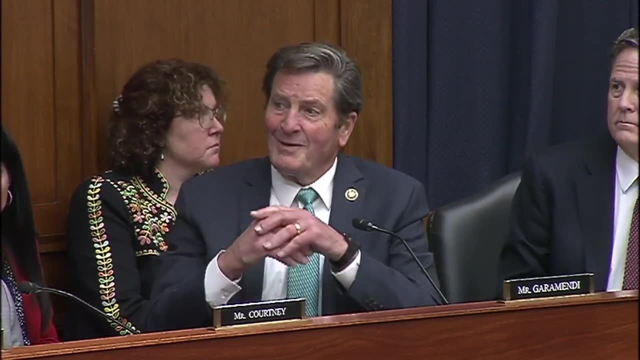 There are apprenticeship programs in some of the more recent legislation. We ought to look at that. use that more robustly. With that, I'm going to yield back. Thank you so very much. Well, I thank you and I will not disagree with Senator Wicker. 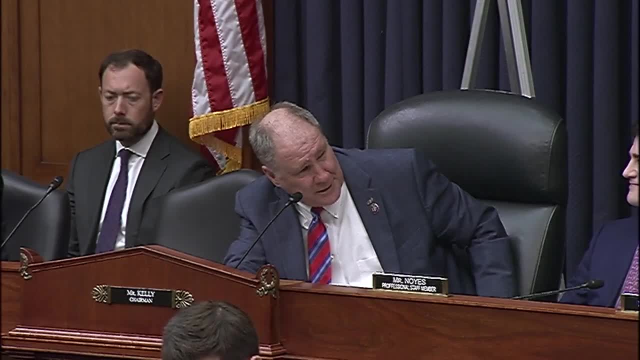 And when he and Mr Garamendi and I all agree on something, we're probably in the right space. I now recognize the gentleman from South Carolina, Mr Garamendi. He's a great man. He's a great man. 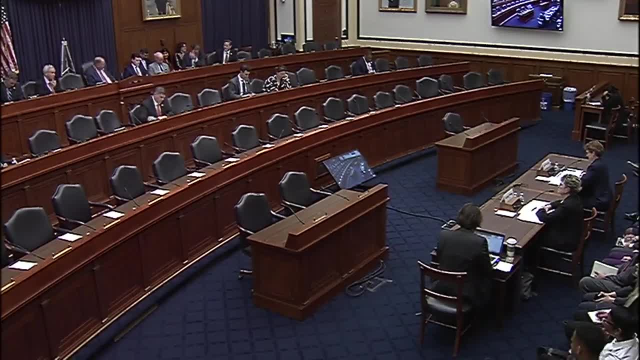 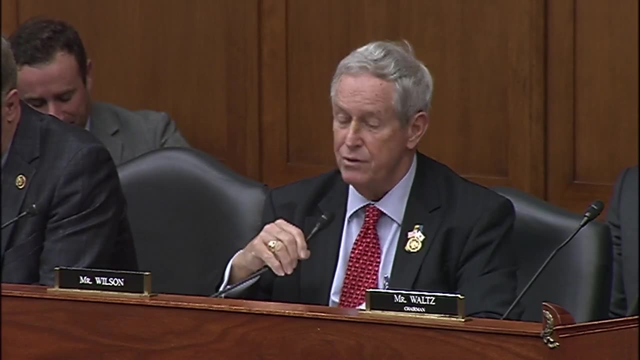 Mr Wilson. Thank you, Mr Chairman. Indeed, it is remarkable that we get to agree together with Congressman Garamendi and General Kelly, And it's wonderful to agree also with Senator Wicker, And indeed we support bipartisan your efforts in every way. 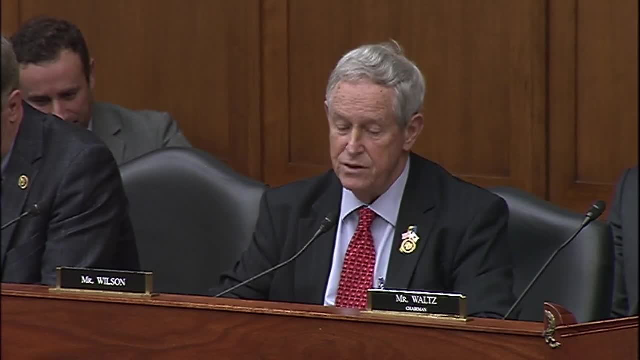 And General Ovost, I want to thank you for your service to the nation and leadership at the United States Transportation Command. and taking the opportunity to highlight South Carolina, We are so grateful that the service members of the 437th Air Wing stationed at Joint Base. 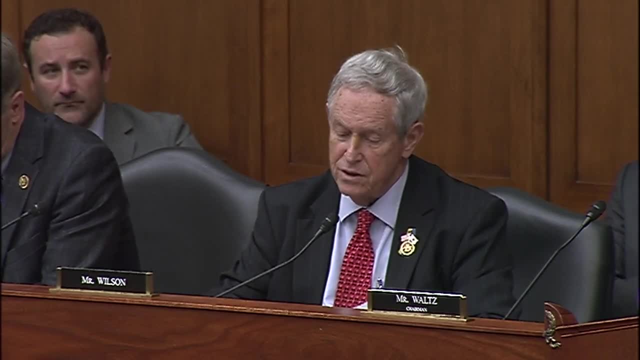 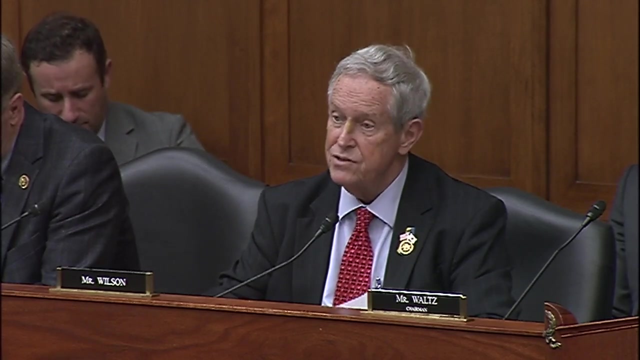 Charleston from the Air Mobility Command under your command of Transcom. The Joint Base Charleston is a great example of the joint readiness across the force and this is due to the leadership within Transcom Enterprise And I particularly appreciate it. My dad served in the Flying Tigers in World War II Army Air Corps. 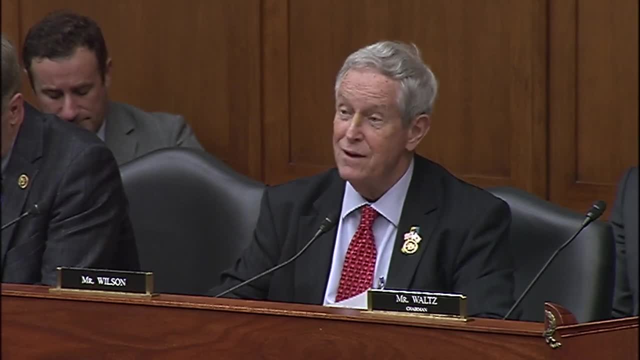 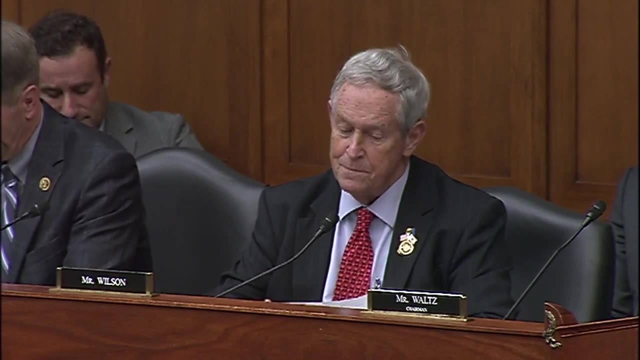 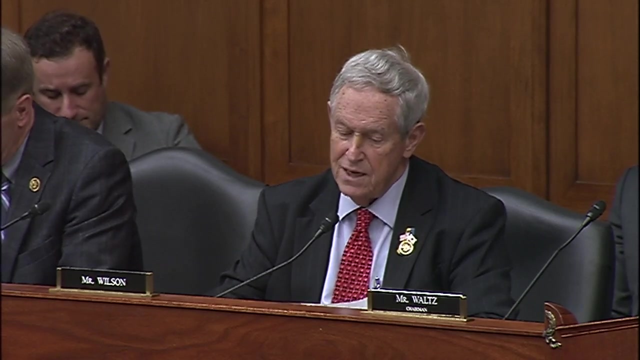 And we used to go visit the Charleston Air Force. We used to go visit the Charleston Air Base to see F-86s take off, which we thought were very advanced at that time. And so, again, your leadership is critical. And in your statement you sadly mentioned that 17 of the 47 ships in the Organic Ready 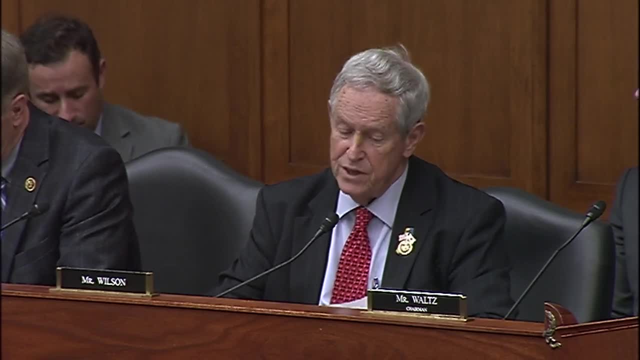 Reserve Force are 50 years of age or older, with the oldest being 56 years of age. This raises readiness concerns for the impact of that age and the life cycle for our Air Force. I want to thank you. I'm sure you've been a great example of that. 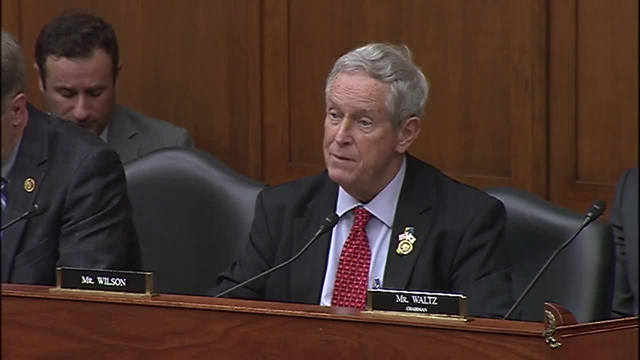 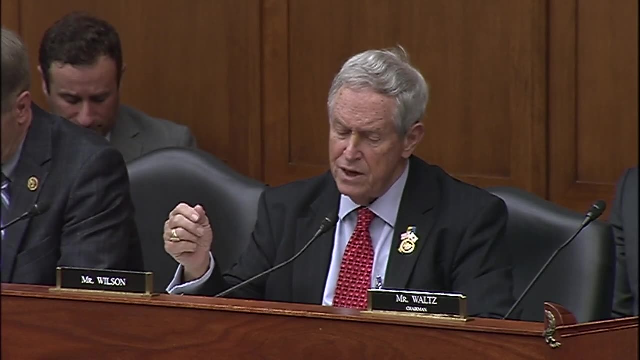 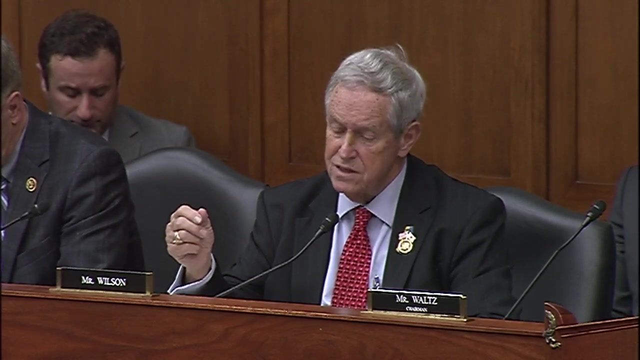 But I want to ask you to pay attention to the fact that you have the bipartisan support that you need. I know you're deeply concerned about the sea lift capacity and that's why I'm so glad. as you clearly see, you have the bipartisan. 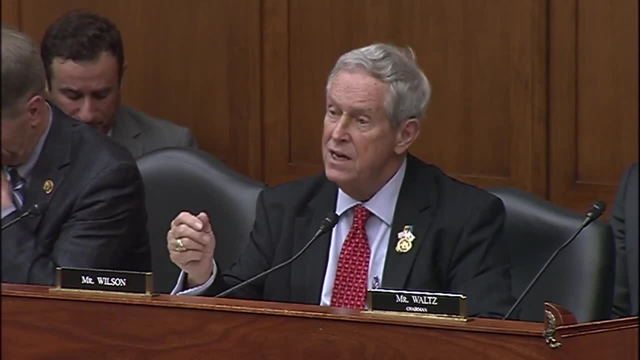 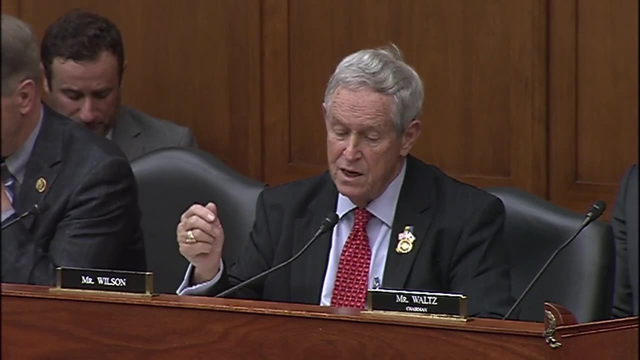 support, Even bicameral, and so have the House and Senate plans we have in the global supply chain, with a direct challenge to our allies of Korea, Japan, India, Philippines, Australia. With that in mind, what is with the ongoing events? 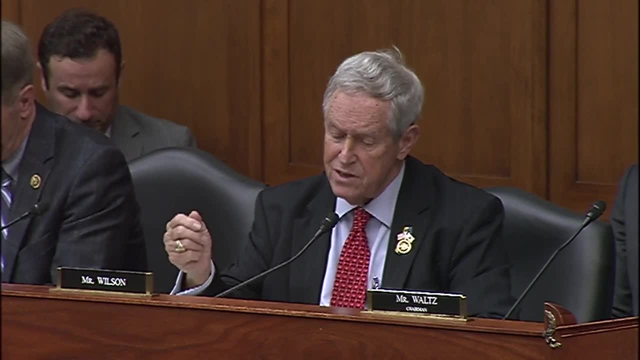 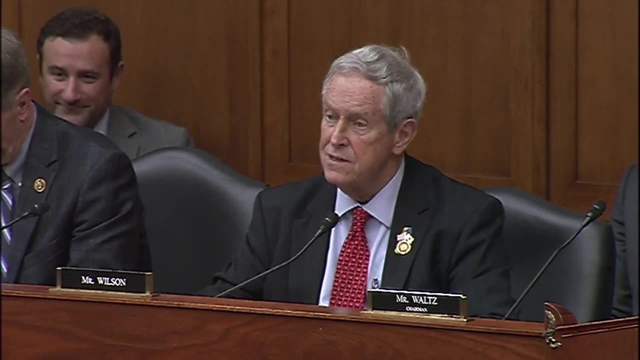 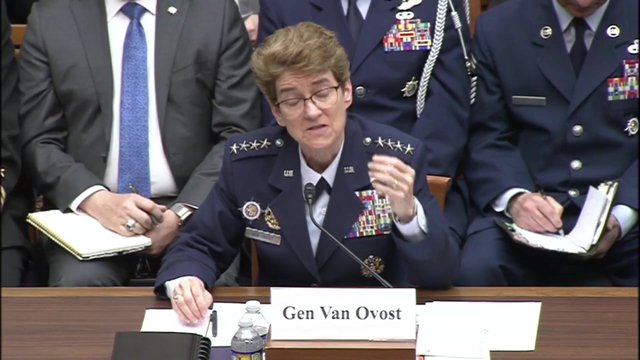 General and Admiral, the and military exercise. what lessons learned have we captured to help improve in the areas that we have against such threats? Yeah, thanks, Congressman, I'll start with. we are very focused on contested lines of communication, like things, like choke points. 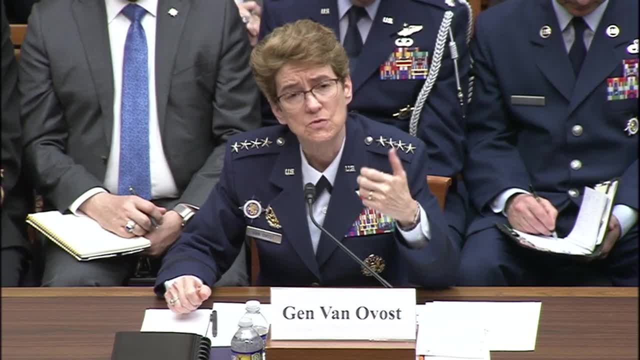 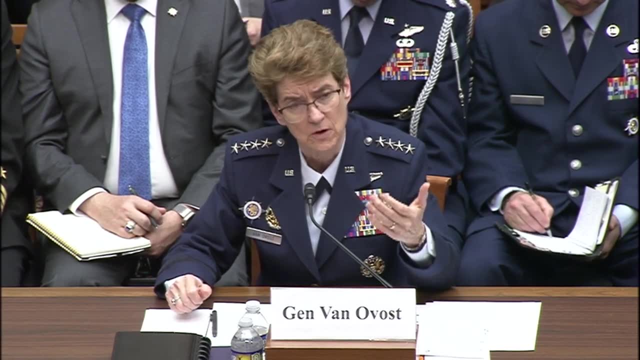 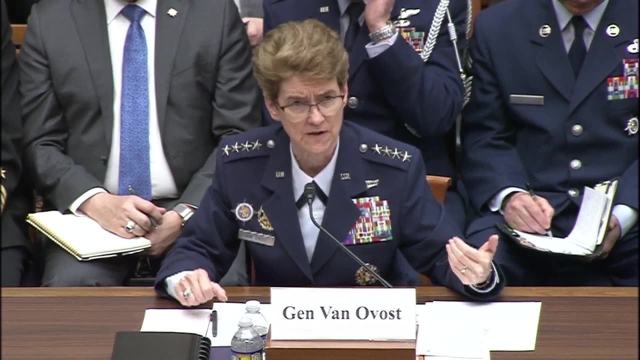 and so we're working with commercial industry to help them communicate with us, to give them the intelligence, and in fact you saw us do convoys with our commercial partners through the straits and into the Red Sea. so we're taking those lessons out to the Indo-Pacific. It's a 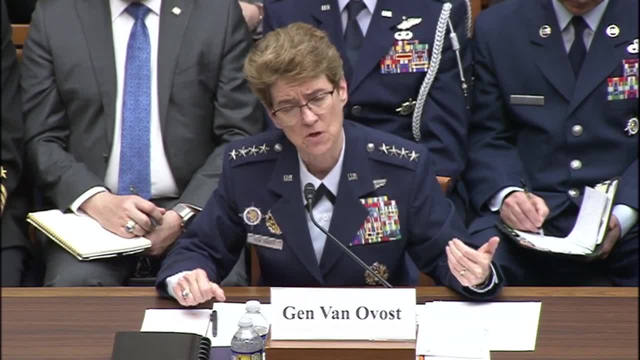 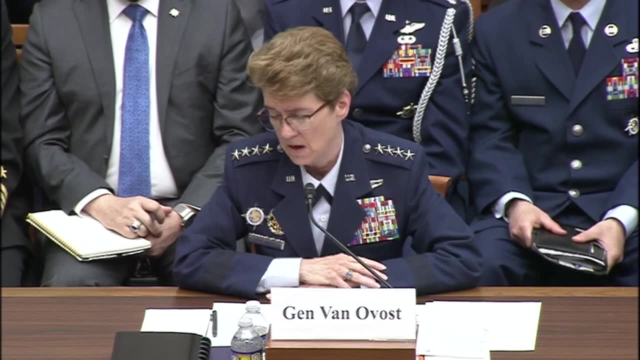 different. it's a different category out there. The threat is much higher. so we're we are also focused on training mariners about how to how to navigate in in contested waters. We know that they will be with us, but it also I think about we are so dependent on our commercial. 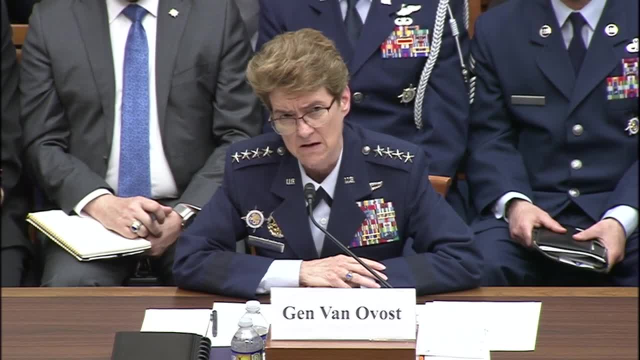 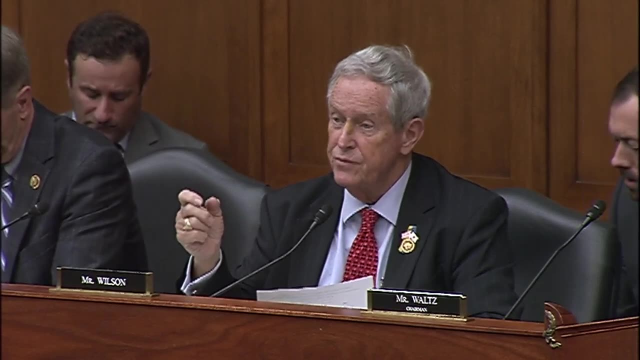 transportation partners. we cannot project and sustain the force without them. so we will absolutely take these contested logistics ideas we and we are exercising them right now in the Indo-Pacific And- and today it was really outstanding- We had Prime Minister Fumio of. 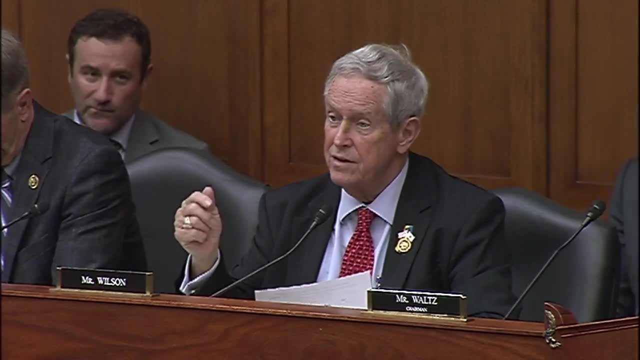 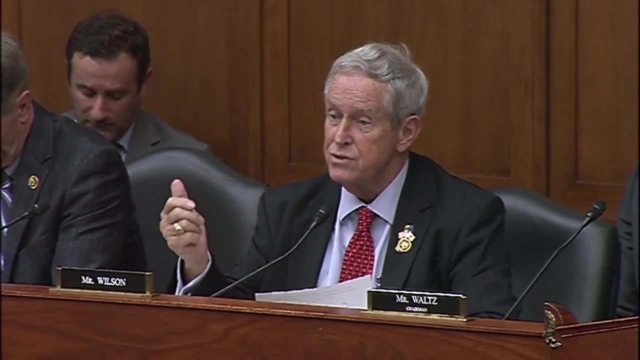 uh Japan speak uh and I hope everybody uh saw his resolve. uh has stated his resolve to work with NATO, to work uh very closely, uh continue with the United States uh, and how important it. 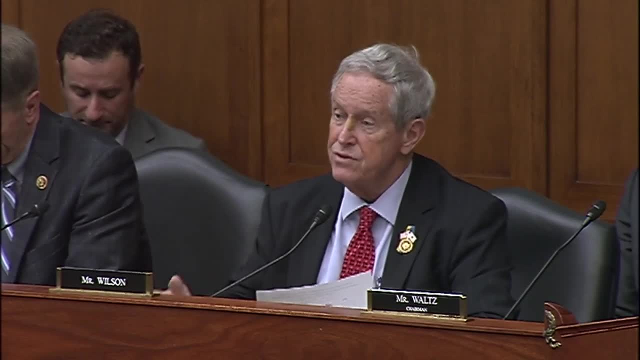 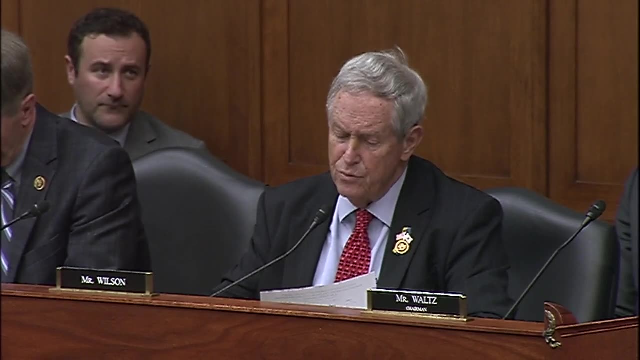 is that we'd be working together, and indeed with the Red Sea routes, and I I know uh Korea too, uh, has been involved. Uh, General Van Obost, uh, would you assess the Middle East as being one of? the most enduring security and stability in the United States? I think Well, China is one of the most enduring uh security and stability challenges, due to the numerous attacks on our infrastructure uh- Iraq, Syria and losing uh three American. 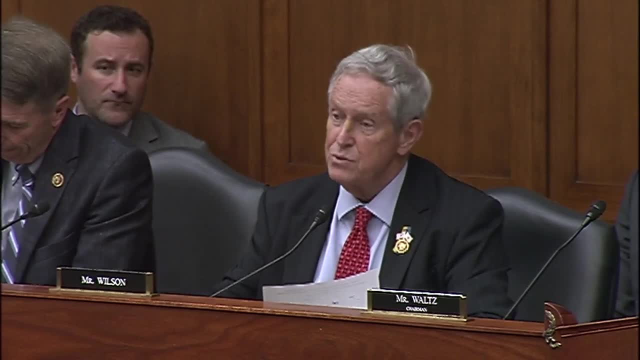 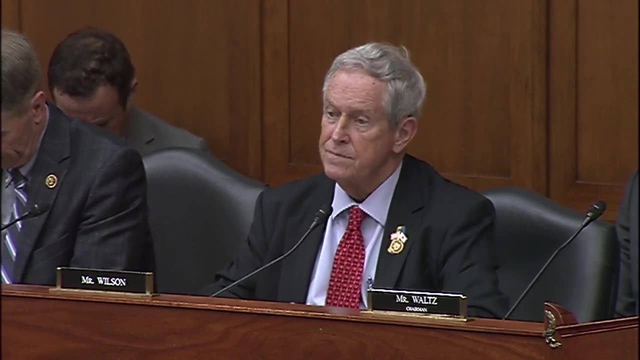 service members in on Jordan uh recently, on January 28th, the horror of that Uh. are there any further steps that Congress can do to better facilitate your efforts? Thank you, Our hearts go out uh to the families of the Fallen Uh when I think about the the. 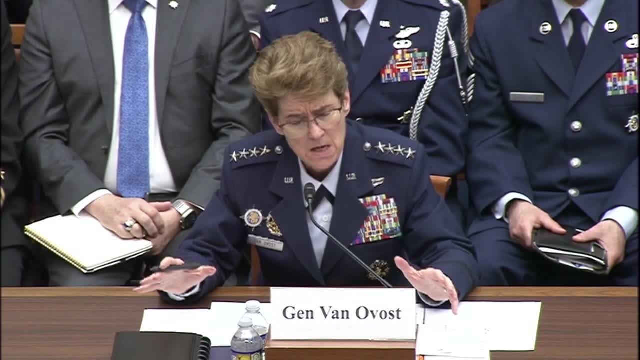 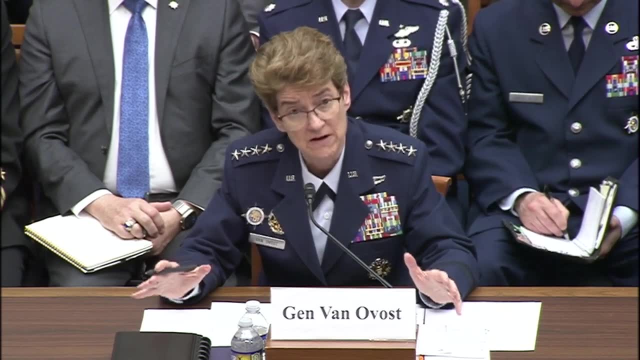 globe, though I have to think about our pacing challenge is China, uh, and an acute threat is Russia, as you know what's going on there with especially Russia and Ukraine and the future of whether Ukraine stands or falls, which is dependent on a supplemental, And I let General Cavoli 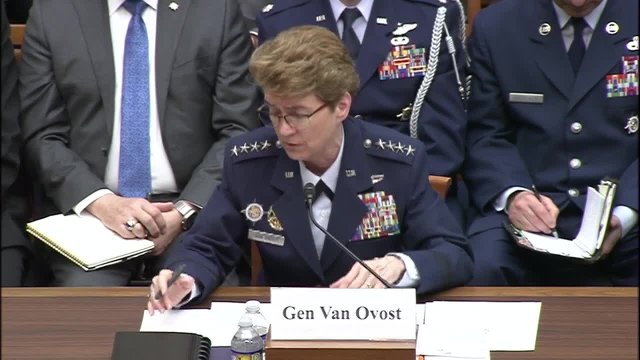 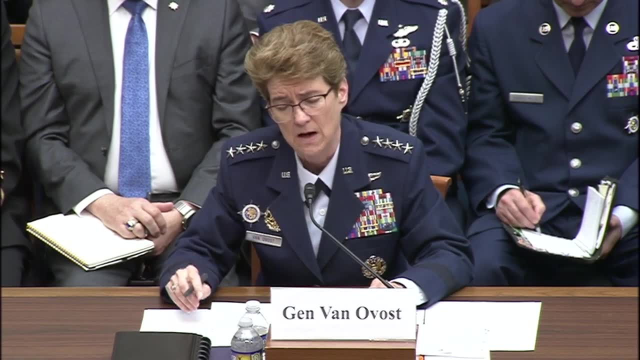 make that statement, but it's critical And we depend on a supplemental as well to continue going. There are enduring threats around the globe, to include in the Middle East. We have great partners in the Middle East And I work very closely with Eric Carrillo to ensure that. 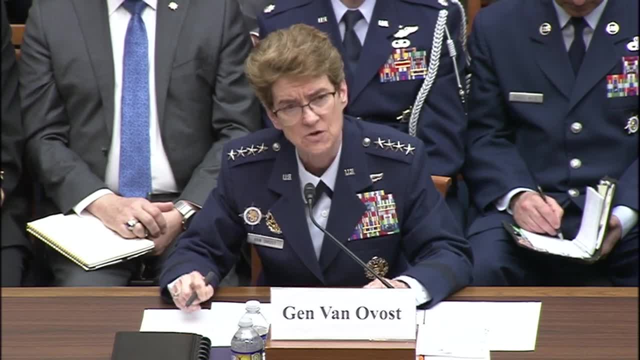 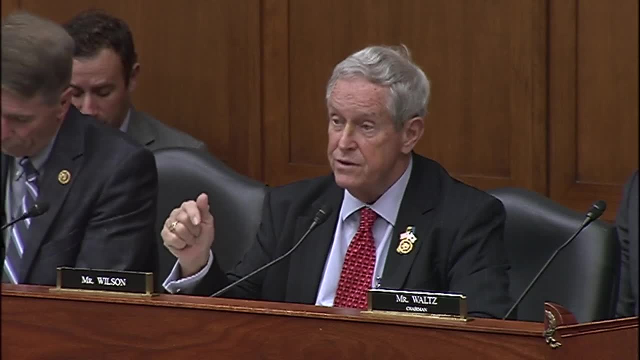 he has the transportation and logistics he needs to maintain deterrence in the Middle East. I think both of you, your service, could not be more important as we have a war between dictators and democracy. I yield back And we're sending every witness to the school you went to. You are succinct and you answer. 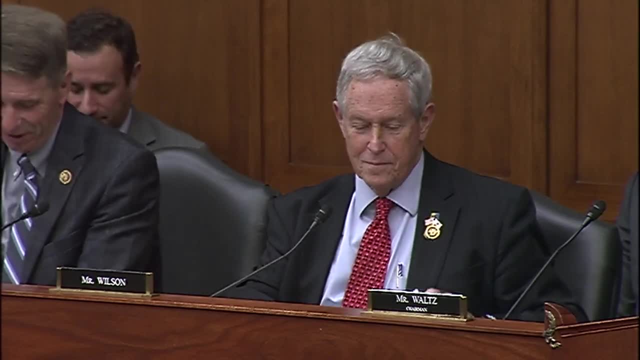 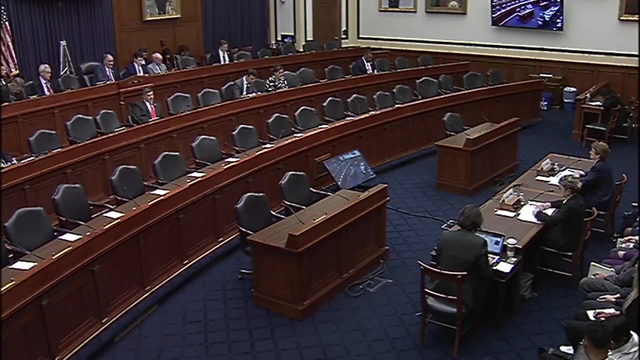 the questions. I now recognize the gentleman, Mr Norcross. Thank you, Chairman, both chairmen and ranking members, for holding this meeting And certainly to our witnesses. very much appreciate the time that we've had to discuss not only in the past but today. 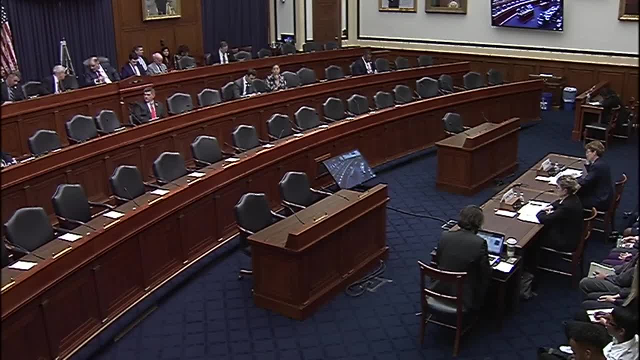 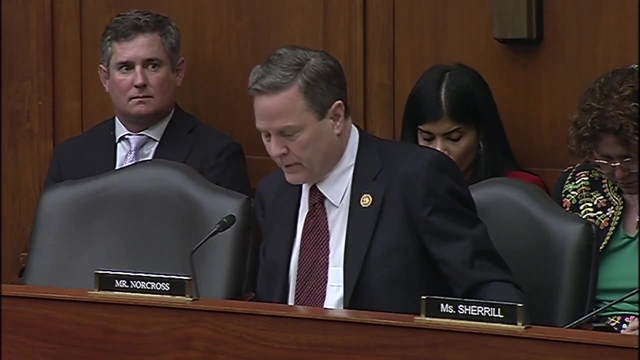 We've heard a lot about the capacity. Mr Walts in his chart up there showing what China is doing, And certainly China follows a rule that we don't. You don't see any of China's naval vessels being made in anywhere but China, and certainly to support boats. 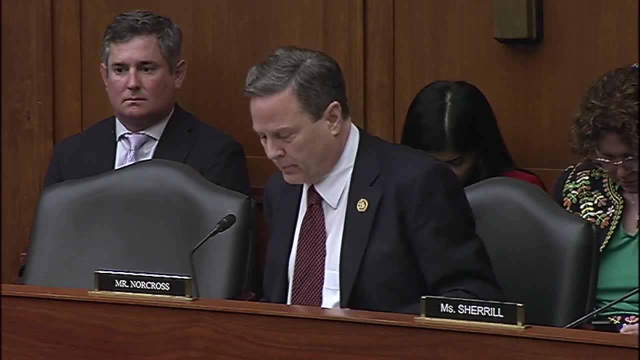 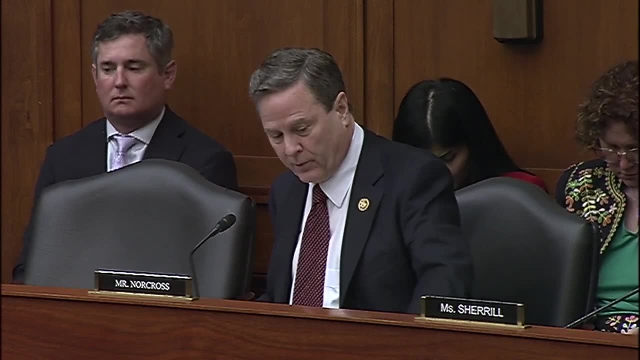 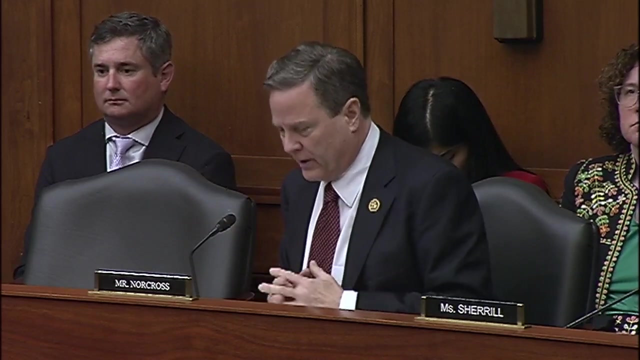 And our conversation, the one that I would like to have today, talks about our industrial base, the ability for shipbuilding- Certainly, sea power has been focused on it- and Joe Courtney and others, The uninterrupted recapitalization. So on one hand, we're having to go out to the used 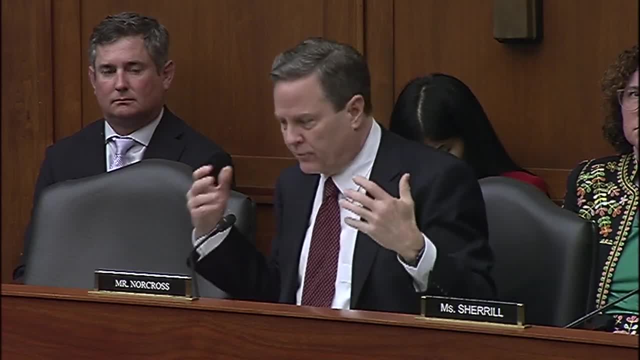 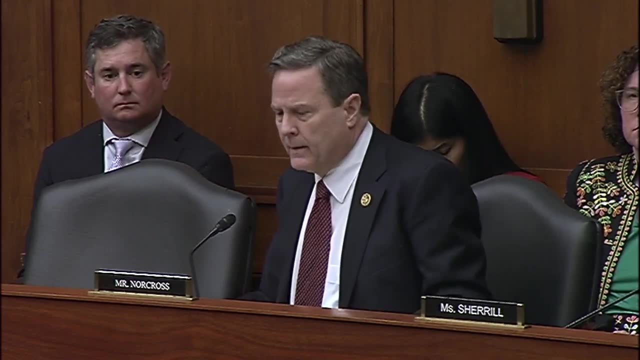 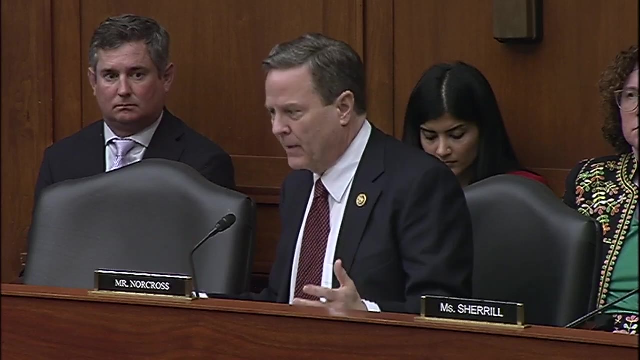 market to purchase ships because they're not available to us in the time factor and the cost that we need them. Yet we don't want to set up that recapitalization to build new from the get-go. So it's a self-fulfilling prophecy. We're not going to have the capacity. 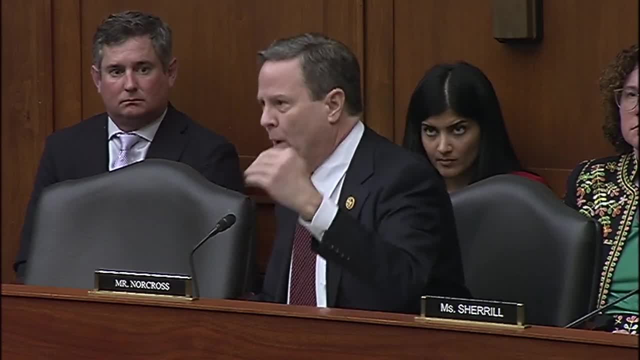 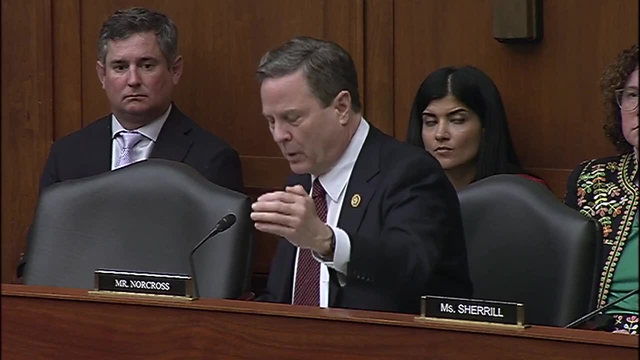 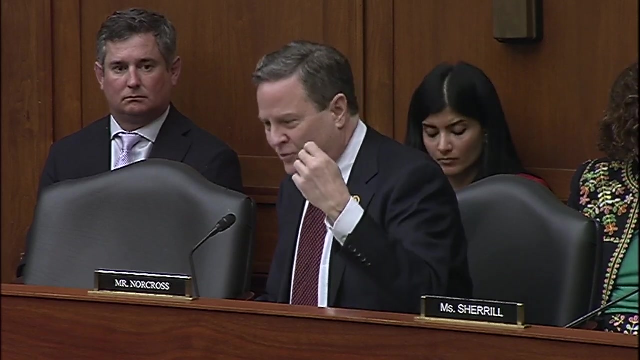 to build this in America. We're going to have to make the decision collectively that we have to build this in America to build up that capacity, Because we talk about supply chain issues particularly came to light during the pandemic. Well, the most difficult part to get of any ship. 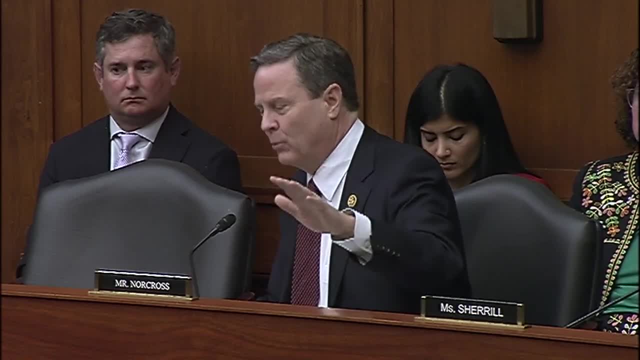 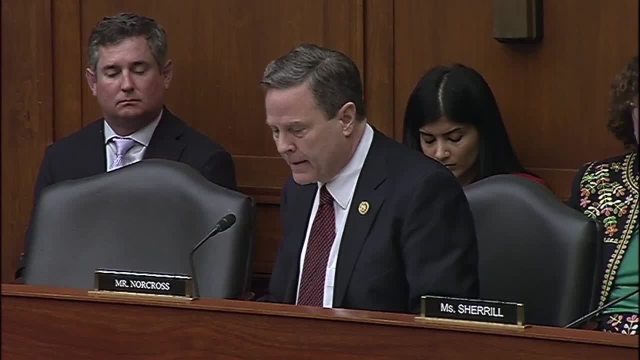 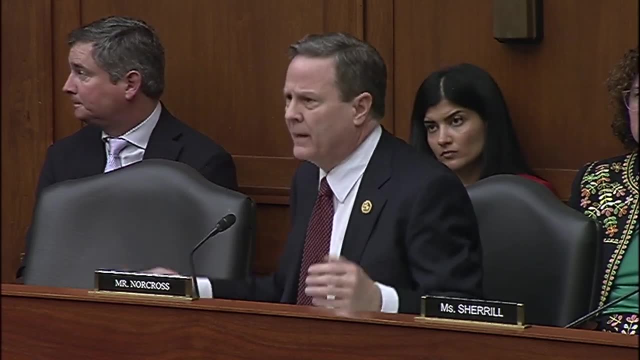 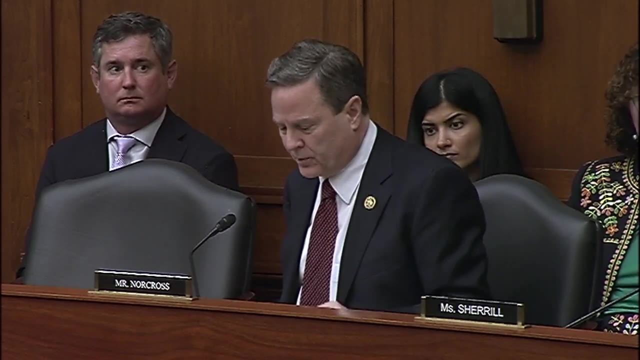 Mr Walts, It takes time and certainly it takes a lot of pressure from us to say we need to build this. How many times do they take it in the Tackling the Jones Act? So what I want to do is the both of you went to the Philly Yard and talked about the construction management model. 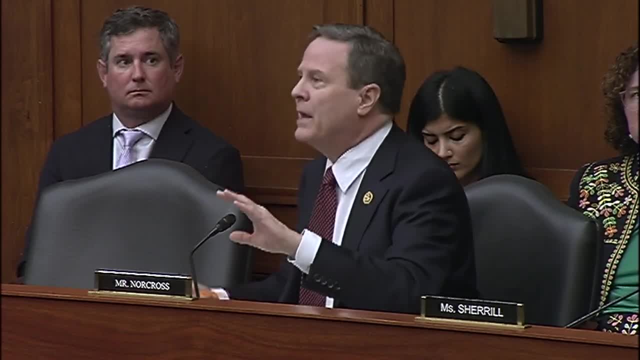 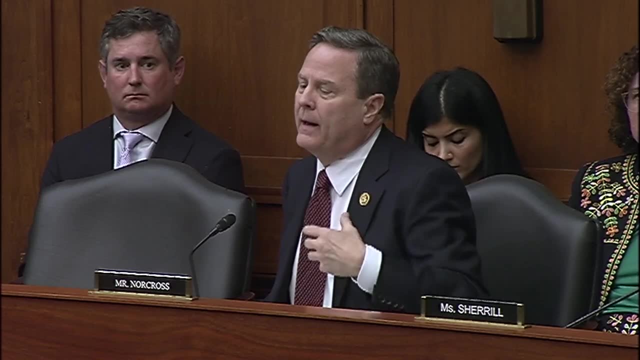 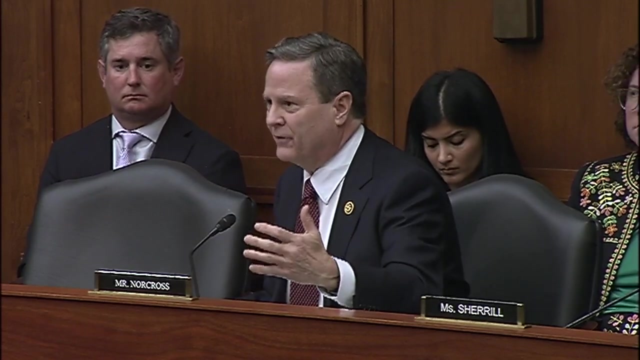 And what we saw there virtually in naval terms, absolutely on time and under budget in naval terms, But what they're doing there and we can expand that model so that that self-fulfilling prophecy of not being able to have the capacity, you have to start somewhere. 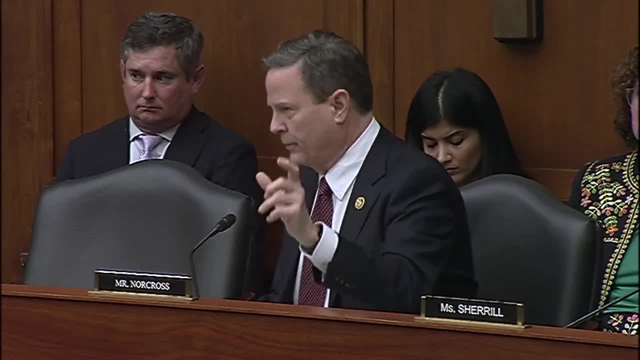 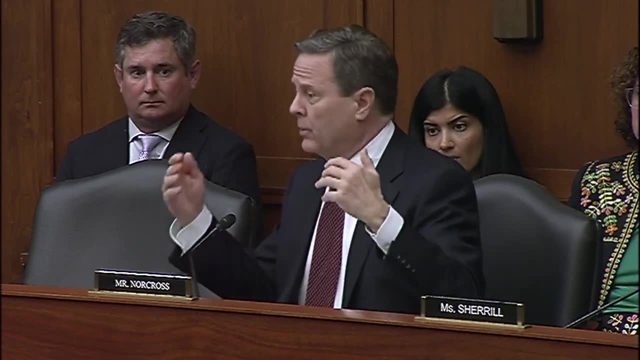 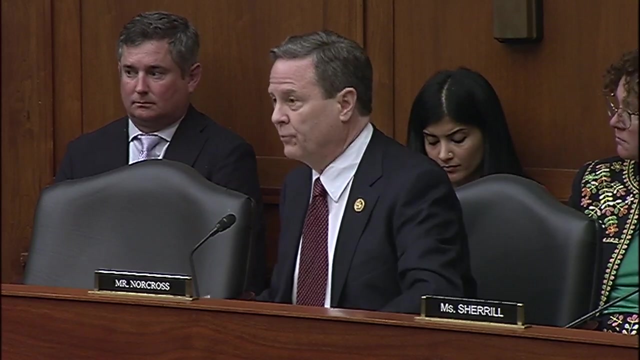 So, Admiral, share with us a little bit what they're doing in Philadelphia under that construction management model and how we can take that and potentially expand it. because they want the work. How can we give them the work they need and, most importantly, have those vessels for what? 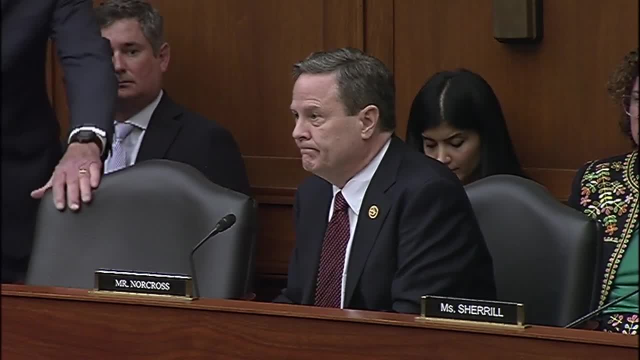 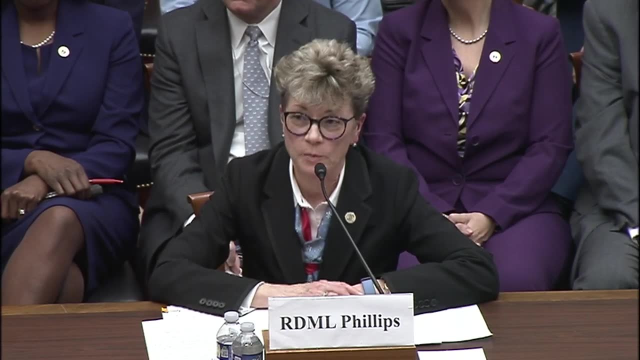 What do we need to defend America? Thank you, sir, for that question. I would add that Philly isn't the only one that wants the work, But certainly Philly has shown, Philadelphia has shown that the Vessel Construction Manager program can work. 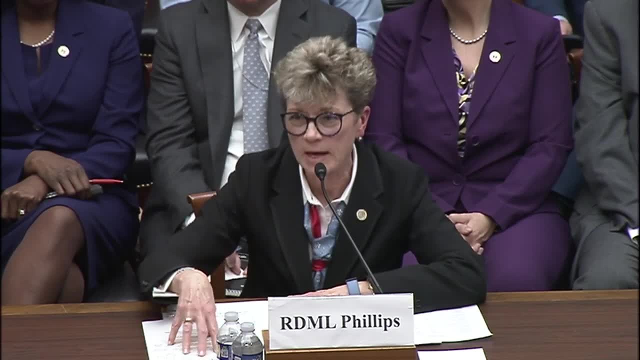 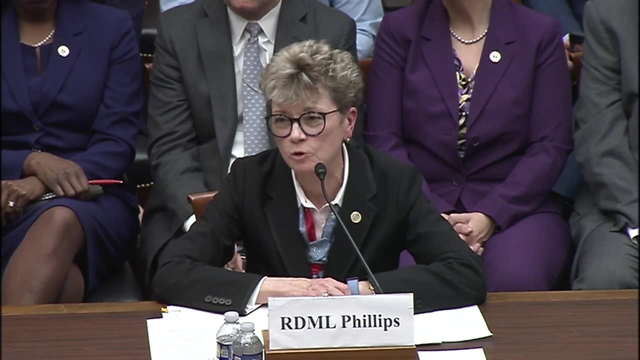 The program consists of us contracting with the Vessel Construction Manager, who then contracts with the Yard to build the vessel as designed. In this case, I believe a lot of the success is attributed to having a strong Vessel Construction Manager first of all. but also starting with 100 percent design with a firm fixed price contract and a very small change order budget and then using commercial best practices to oversee the design, build and implementation of that build with the ship. So that is what has made the Philly ship NSMV program so successful. 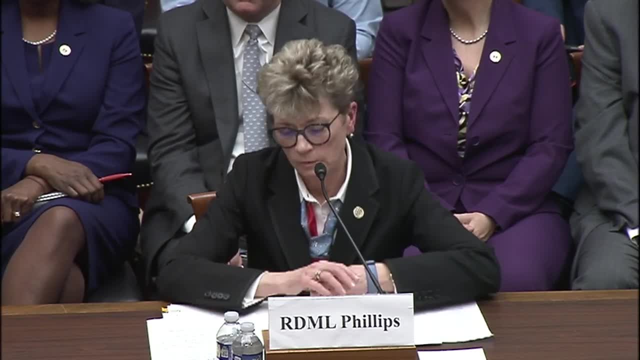 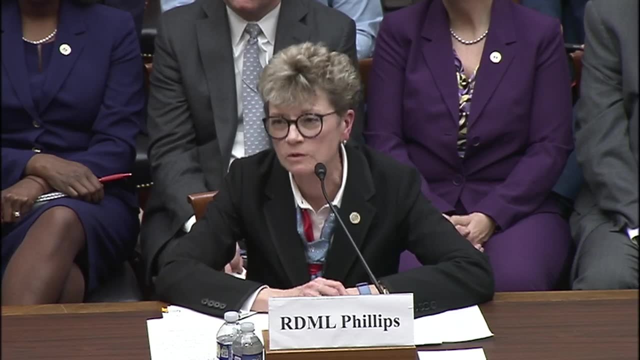 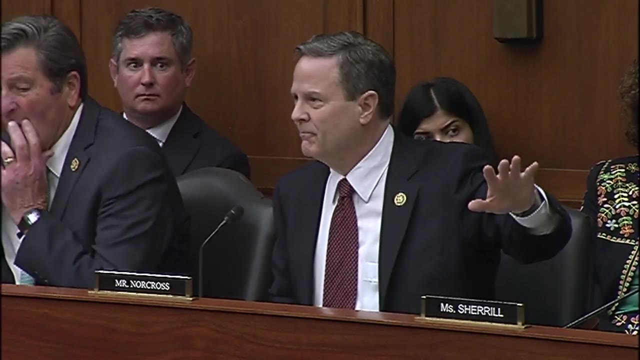 and I believe that can be replicated in many senses to facilitate additional ship construction programs and it can be worked across many yards and many different Vessel Construction Managers. We build those ships differently than we do our vessels. Okay, So we're going to go to war. 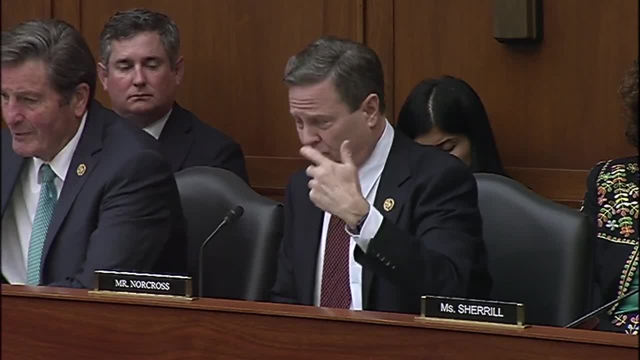 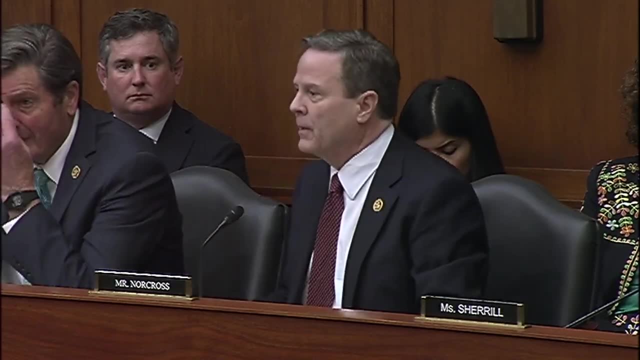 There's no question about that. But the 100 percent design are as close as we can get to it, and we've seen that change. One of the questions that came up is: how can we send a clear message to you? Well, we did it last year in the NDAA. The modified by American provision for major acquisitions used to be in the 50s. We're going to move that up incrementally per year to send the signal to the industry. we're going to buy from American up to the 75 percent. 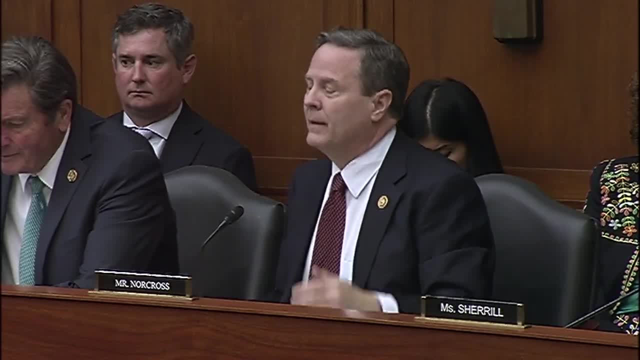 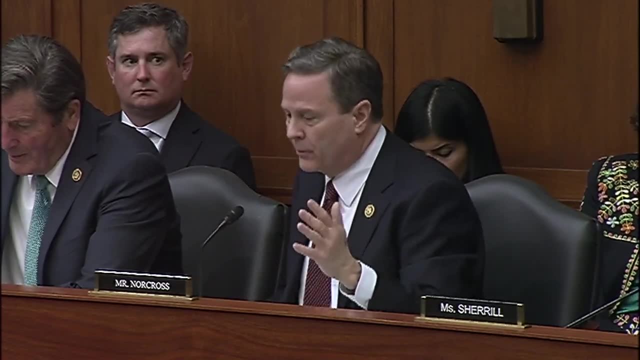 That is the source, That is the sort of signals we are sending, but if we don't exercise it on our end and your end to actually implement these, we're not going to get it the right way and I'm going to yield back my final 30 seconds. 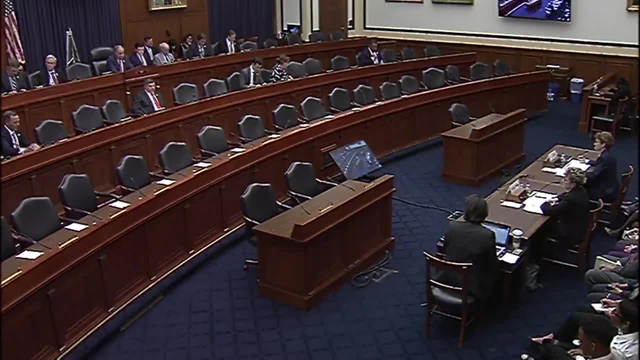 Thanks. I thank the gentleman I now recognize, Mr Scott. Thank you, Mr Chairman. I think I have a little take than some of my some of the previous comments that have been made. I want the American citizens to know we're not talking about aircraft carriers. 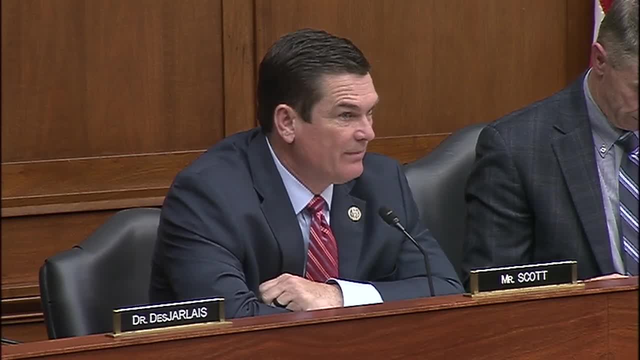 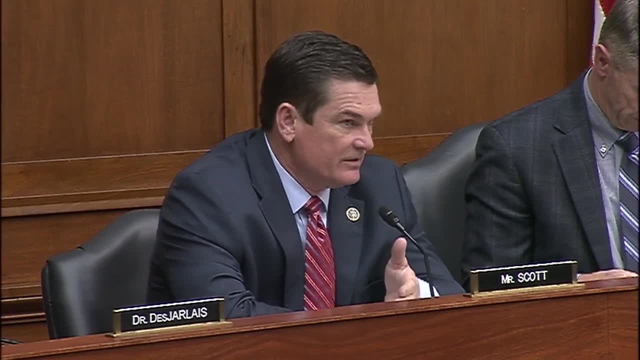 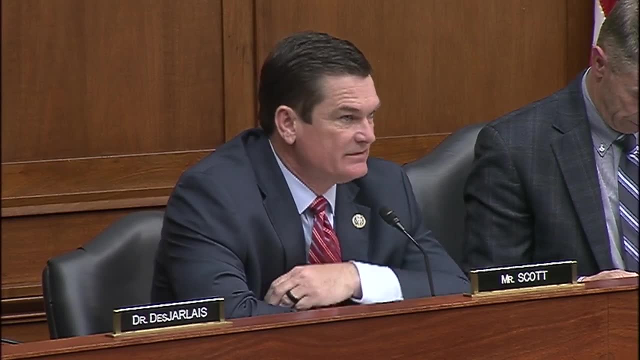 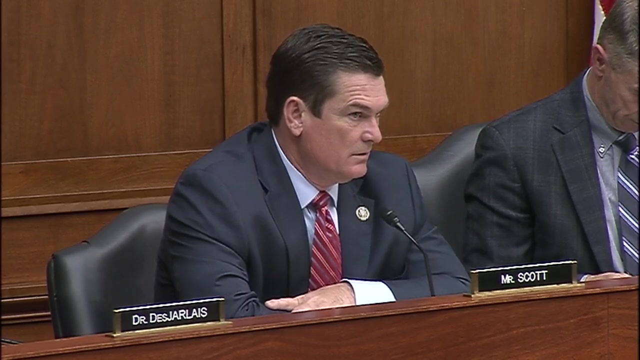 about a roll-on roll-off ship, very similar to what we see in the pictures, unfortunately, of the bridge collapse. Is that correct when we're talking about these roll-on roll-offs? Yes, sir, it is essentially The three most recent ships we bought were ROCONs, so some container capacity. 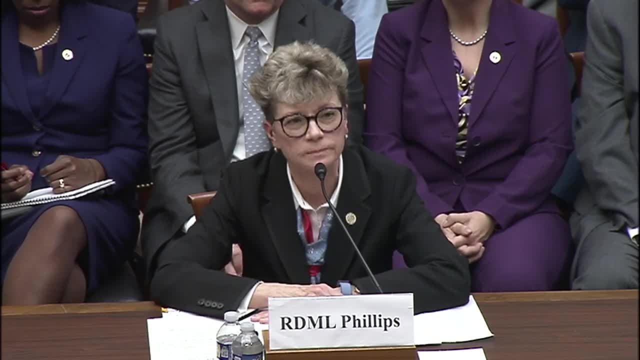 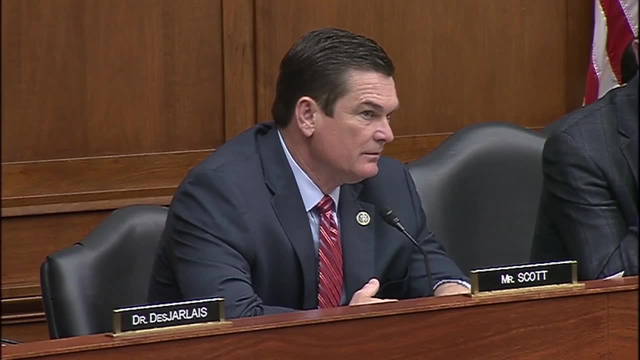 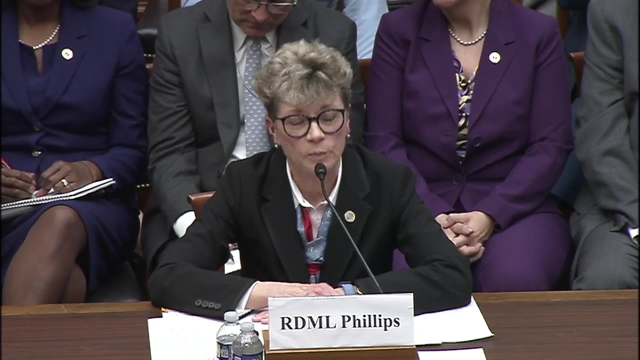 some roll-on roll-off capacity. The two previous are ROCONs, ROCONs. When is the last time that a roll-on roll-off ship was built inside the United States of America, The last commercially built vessels that were built in this country, sir, for international trade? 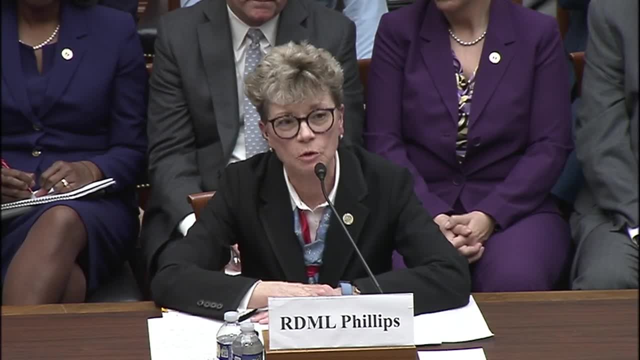 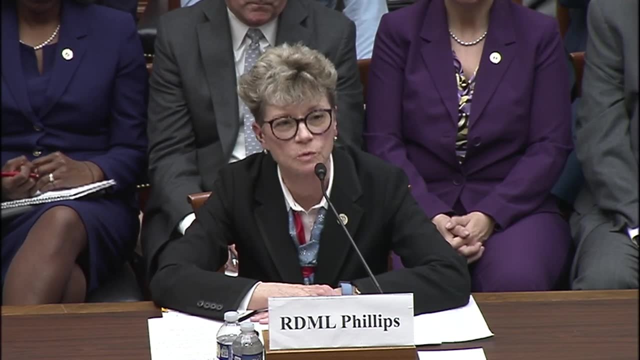 not Jones Act international trade were built in the 80s. We do have Jones Act construction now of. an example would be Mattson and Peja, two West Coast carriers who build container vessels. OK, And they build them in this country. 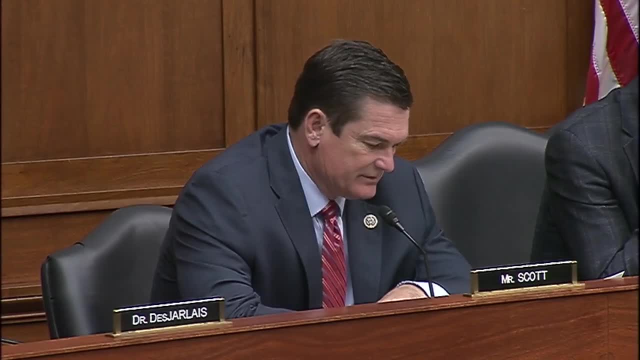 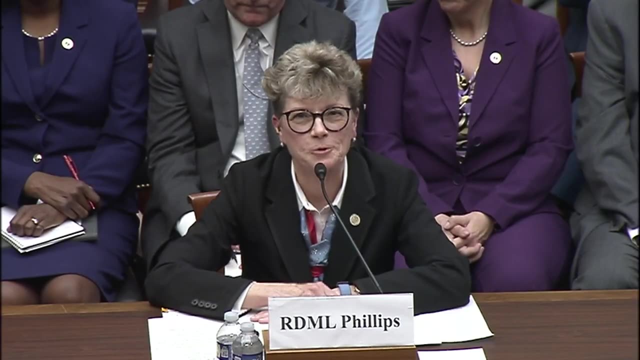 So how many of those container vessels have been built inside the United States in the last 10 years? I can't answer the last 10 years, sir. I know Peja just finished two vessels and Mattson has an order for three in Philly. 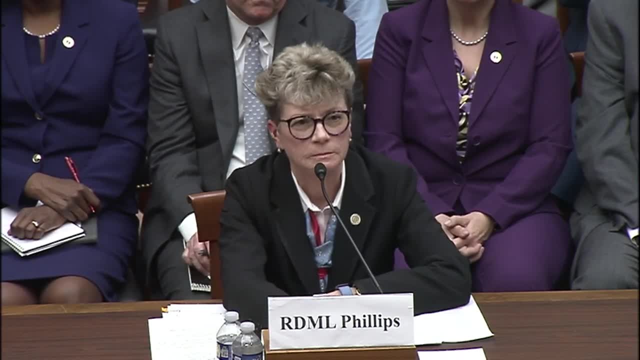 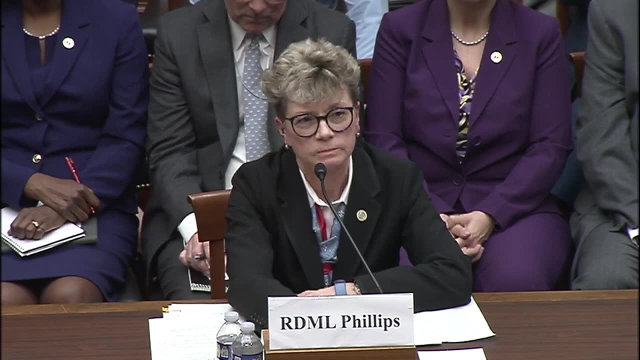 that will follow the NSMB program And how long will it take to build those three? Several years, I would expect. This is an estimate, probably four years. OK, My point is. my point is. my point is: I think that's the point. 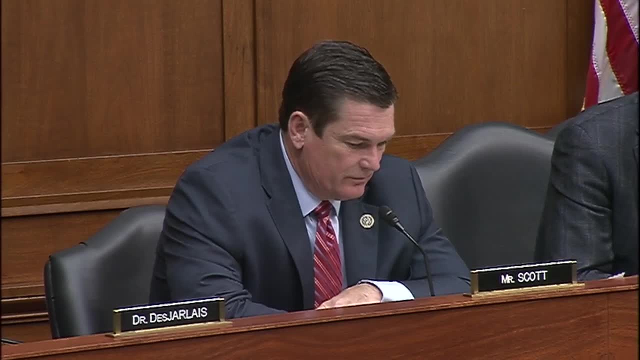 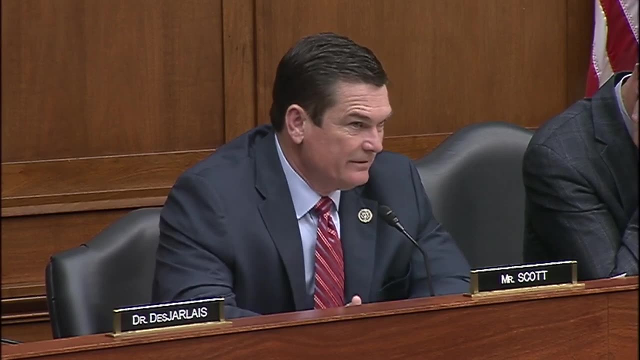 I think, I think, I think that's the point. My point is that if we're going to deal with the capacity challenge that we have and the time that we have to deal with it, you have to accept that the calendar days and the time limit and the capacity is a problem. And I think we should raise the nine-ship limit. And if we get rid of a 50-year-old ship and we end up with a 15- or a 20-year-old ship, until we're able to get new ships built, if something kicks off between now and then, 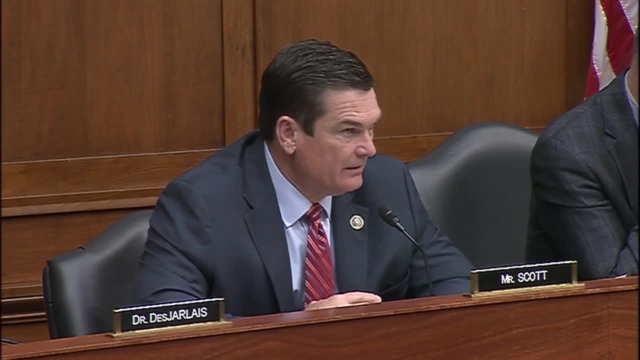 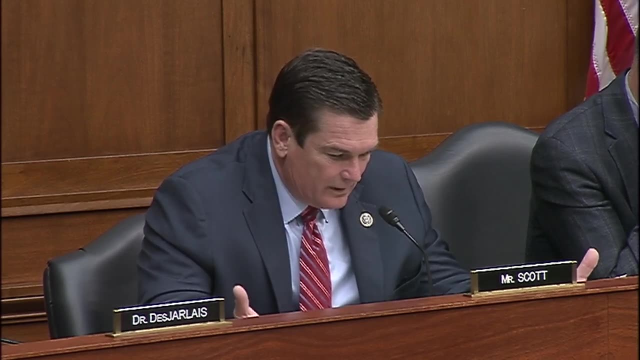 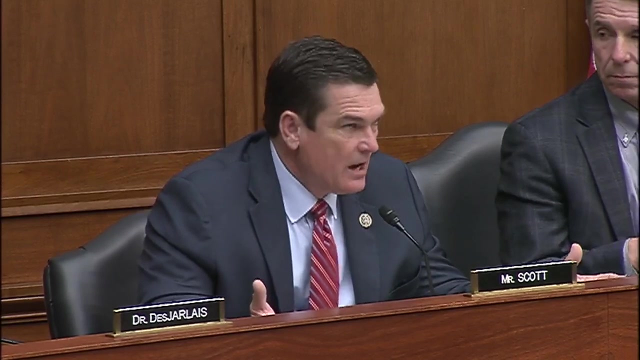 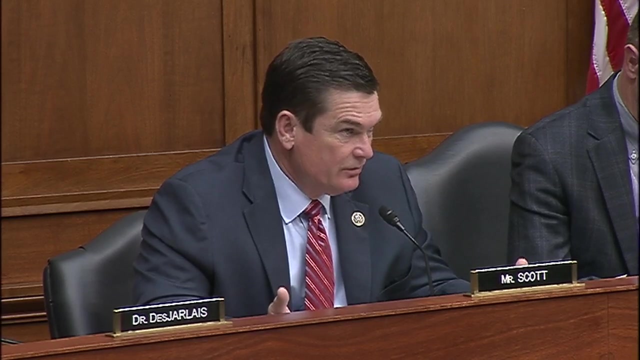 then we're better able to serve this country. And so my question is- you know you've called for, General Van Ivers, the nine-ship limit to be removed. What if it's not removed? How long would it take, if it's not removed, for us to 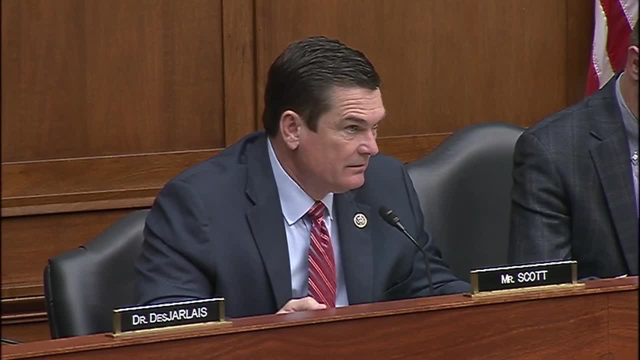 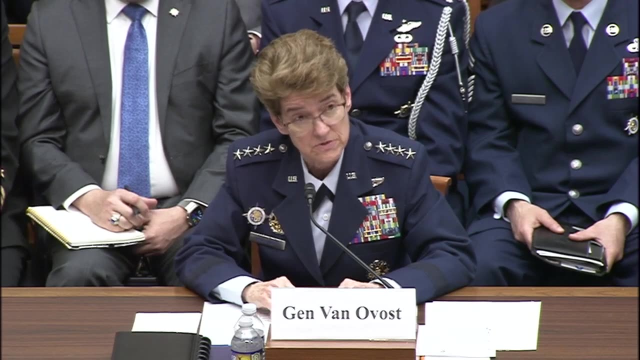 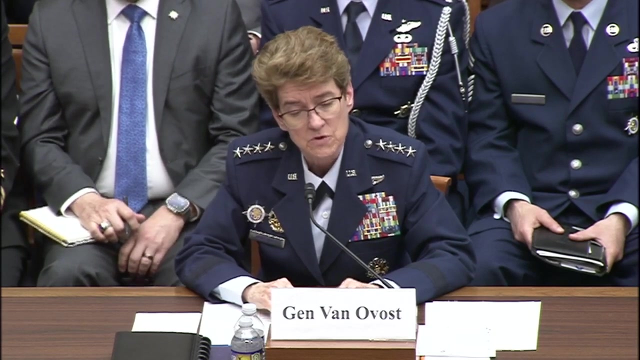 you know, fill the capacity gap that we have. Given the expected decommissioning of the 27 ships in the next eight years, we will be at a much elevated risk to be able to meet our mission requirements, which is why we need to come back to you with a more comprehensive strategy. 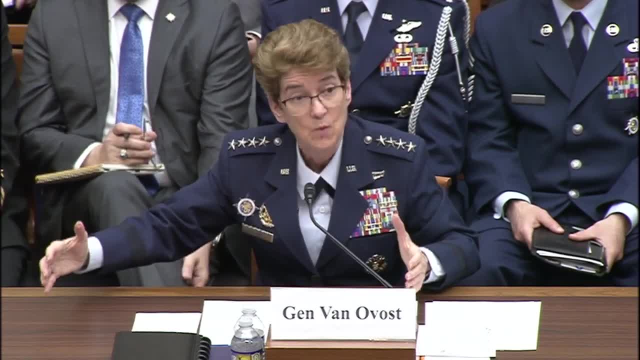 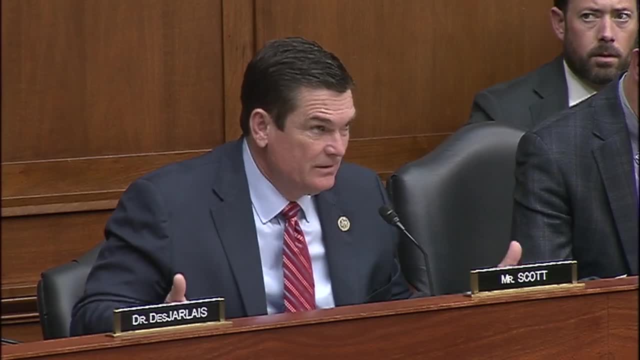 that looks at the near term, the midterm and the far term with the compilation. And so when we talk about the need to raise the limit so that we're temporarily able to use ships not built in China but built in Singapore, built in Japan, 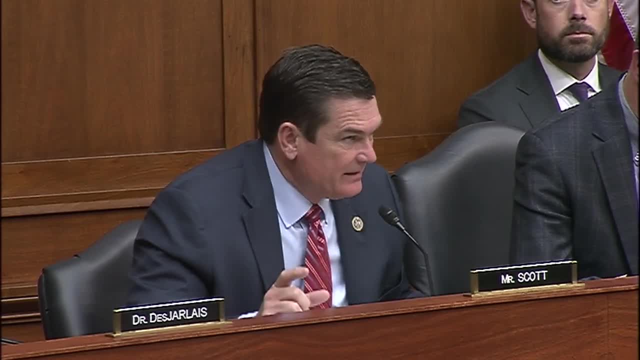 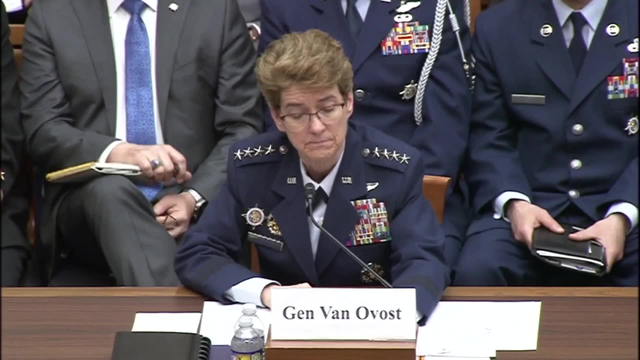 we're standing down how many ships over the next? give me that number again, what you're just giving me: 27,. 56% of the fleet. Okay, so we're going to get rid of 50% of our transportation capacity over the next how many years? Eight Over the next eight years, 2032.. Okay, And it doesn't sound to me like in the last 30 years there have been that many ships built inside the United States in that category. It's simply a question of: do you want to have something to fill the gap? 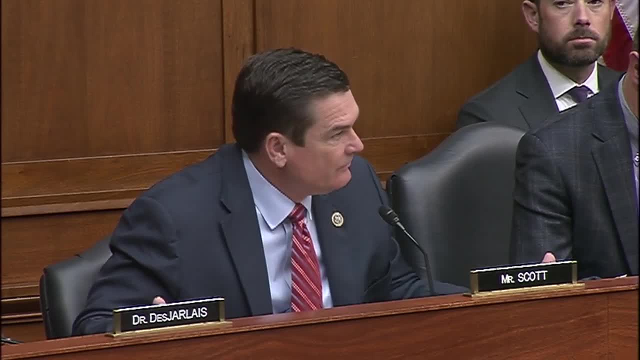 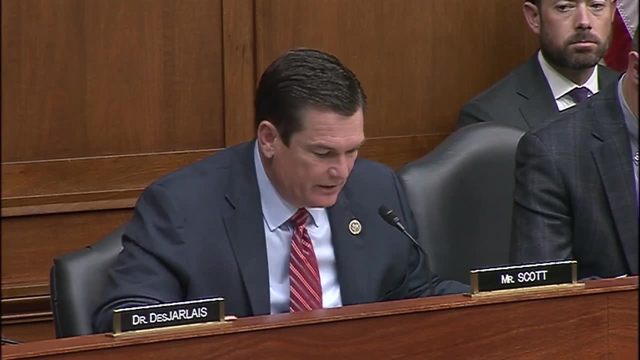 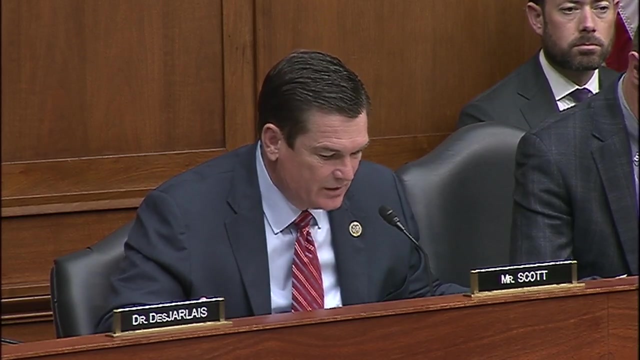 until the US manufacturers are able to fill this or not, if you ask me, So real quick. General Vanova, we talked about the supplemental and the need for the supplemental For you. can you talk to us just briefly about the $550 million, the specifics of that? 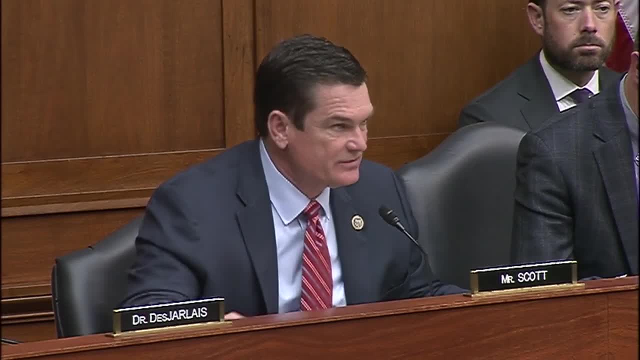 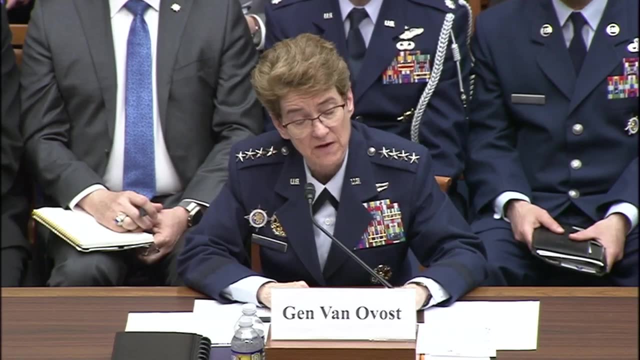 just so that everybody- I think the people on the committee- understand, but just so the American citizens understand the need for the supplemental from the standpoint of Transportation Command. Yes, sir, From the standpoint of Transportation Command. $550 million are earmarked for transportation services. 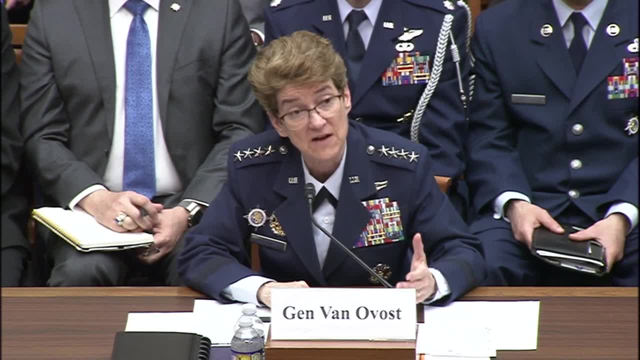 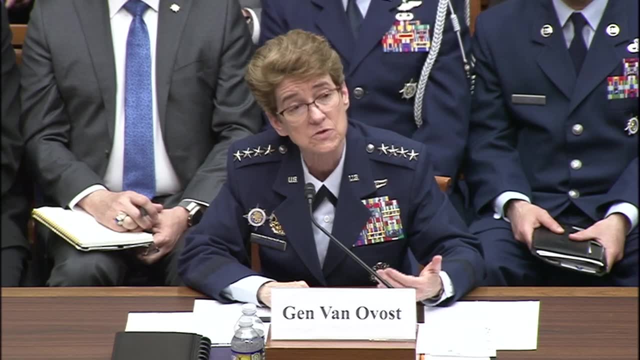 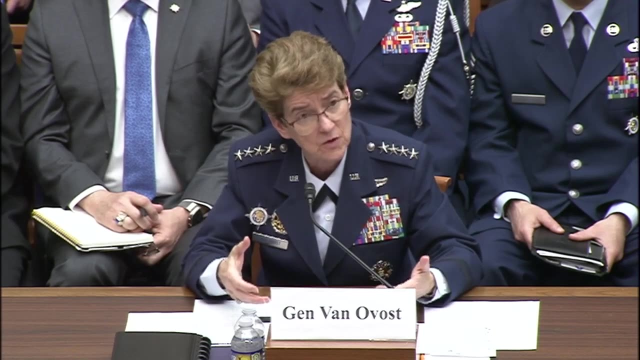 to account for the transportation for the events after October 7th in the Middle East. Those transportation costs have not been recouped, We have not reimbursed and that causes us to drain our funds such that if we have another emergency we'd have to look to see where we'd have capability to provide options for the Secretary of Defense. 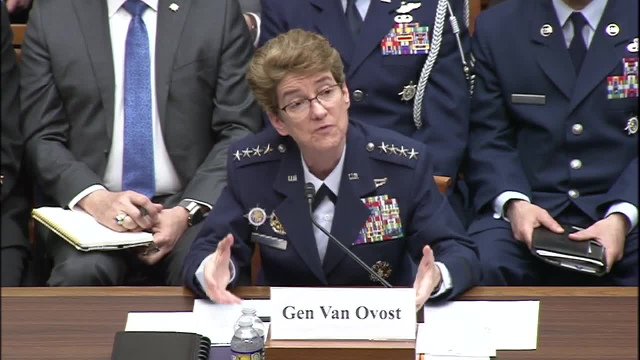 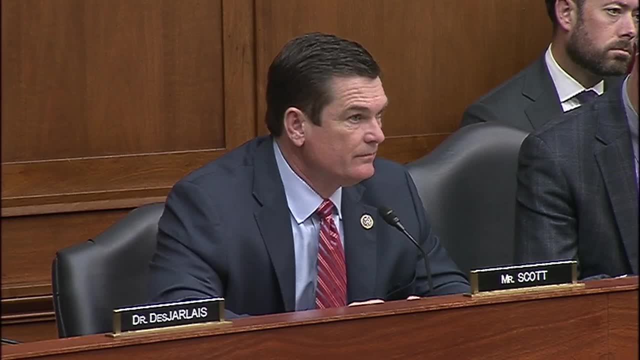 So our Transportation Working Capital Fund is necessary. It's really our readiness function for Transcom, And that money has already been spent because of what happened in Israel. Approximately $180 million has been spent so far, but we are forecasting up to $550 million. 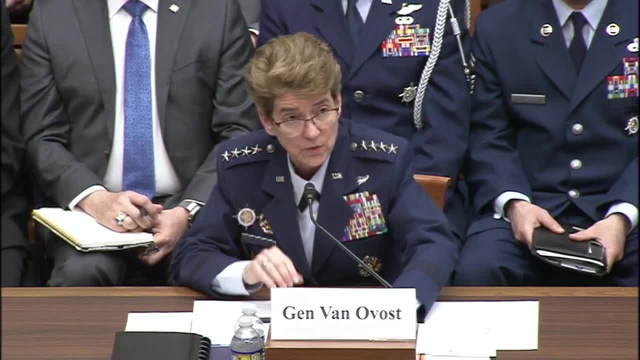 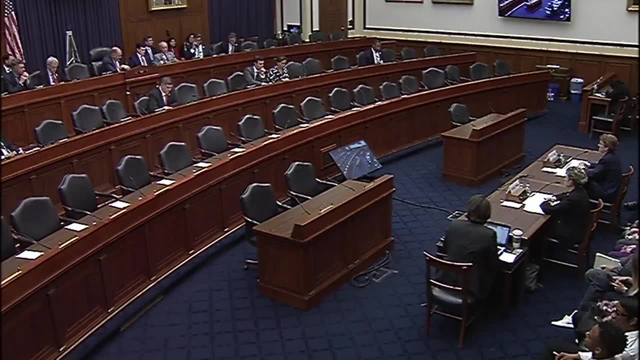 because we deployed forces and we'll have to bring them back In 2024.. Thank both of you for your time and your service. Gentlemen, time's expired. I now recognize the gentleman from Pennsylvania, Mr DeLucia. Thank you, Mr Chairman. 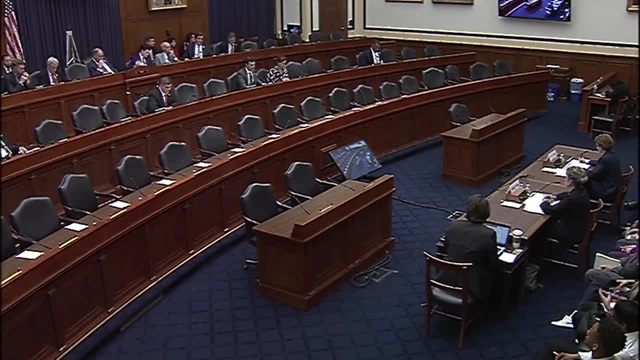 General Admiral, good to see you both. General Van Oost, I'll start with you. I appreciate the Transportation Command report responding to a request I had made in this past year's NDAA identifying vulnerabilities in transportation networks here in this country. 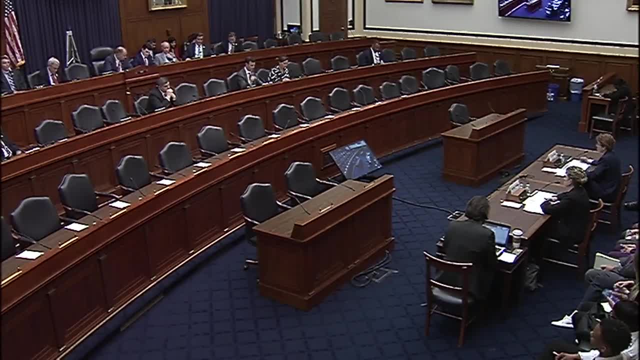 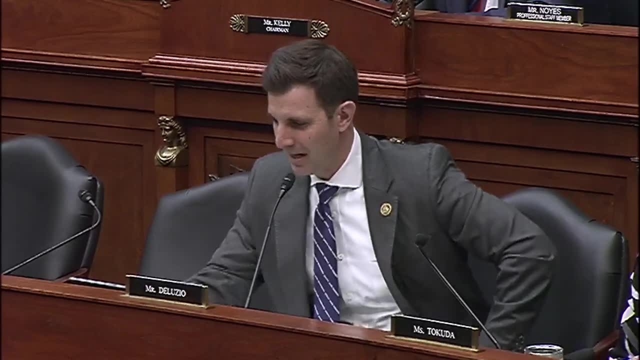 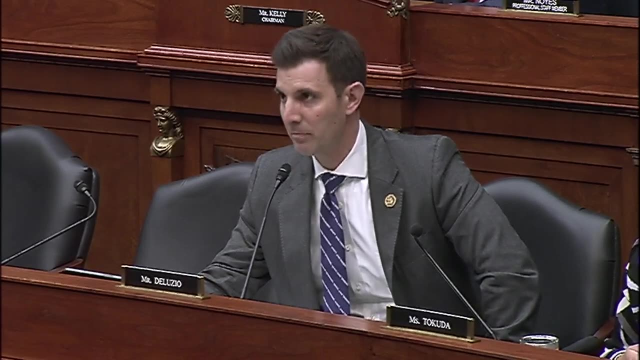 Personnel section under US Transcom concerns regarding transportation. Commercial railroad capabilities report states, and I'll read this brief passage: Over the past decade, the implementation of lean operational processes by the major railroads, commonly referred to as precision scheduled railroading or PSR. has had impacts on the railroad labor force. Across almost all specialized trades, the railroads have reduced the number of employees. Although the intent of PSR is to improve the overall economic competitiveness and efficiency of rail operations, it has arguably sacrificed resilience. In addition to that, there is a lack of transparency in the ability of the rail industry to effectively respond to changes. end quote. 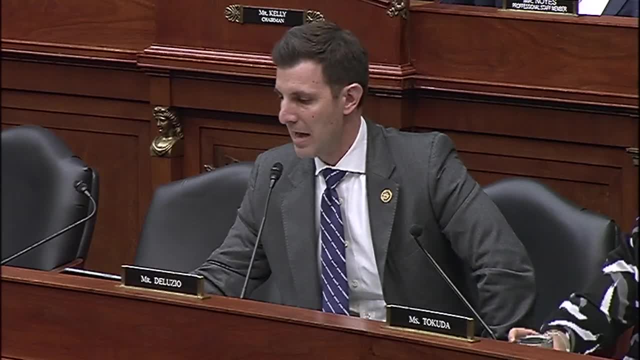 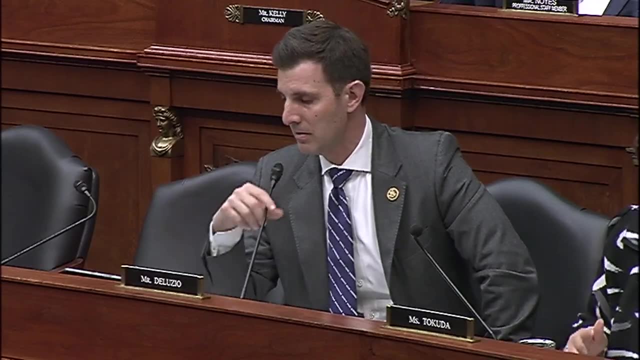 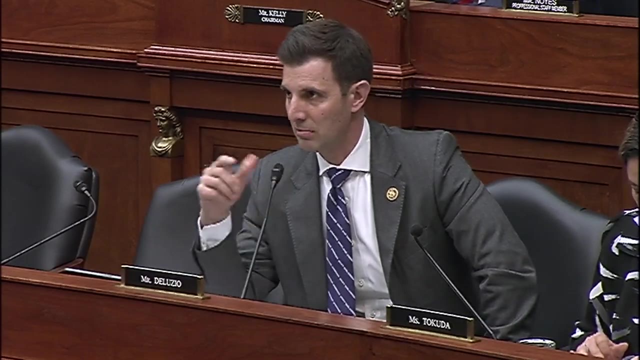 General, the overall assessment in the report is that essentially, freight rail is adequate to meet the needs of your command, Although you identify that risk in the report. just give me a sense of those staffing issues and how they could raise concerns intermediate, longer term to the mission you have to accomplish. 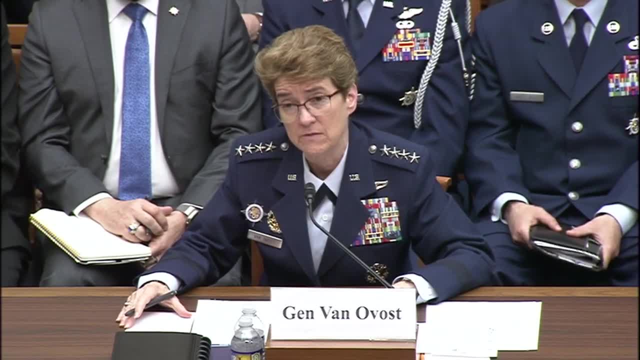 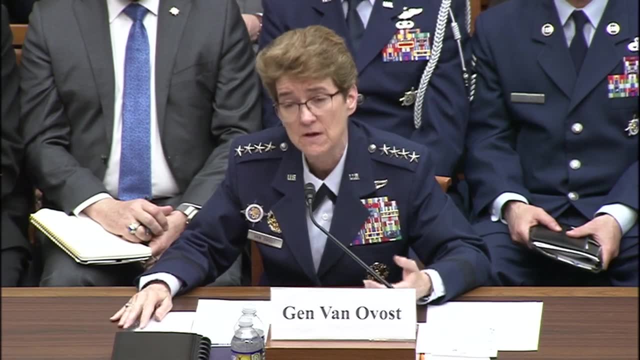 Certainly, I would say, across the transportation industry we are having, we are seeing labor shortages, and so railroad is no, is no exception to that. So as you have less crews, you have less resiliency. it could occur with delays. 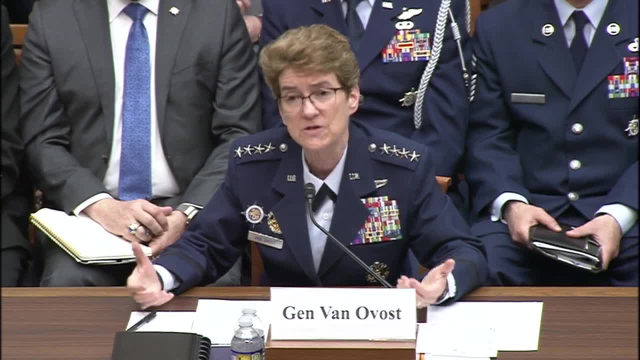 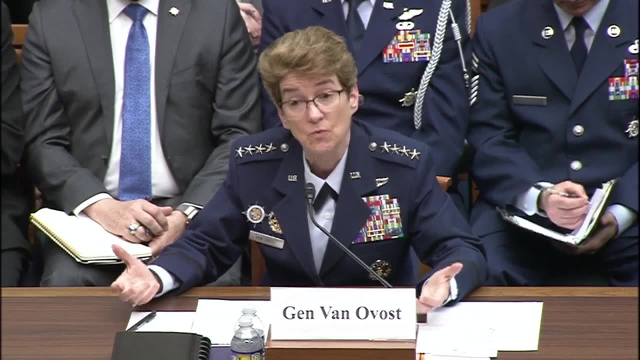 And so we're working very closely with the railroad industry to have to have discussions about how do we ensure resiliency across the networks. That said, should we have an issue on a rail, we do have multiple ways to perhaps offload the rail and go to trucking. 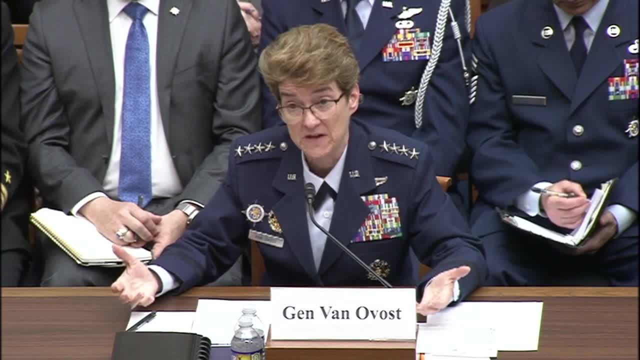 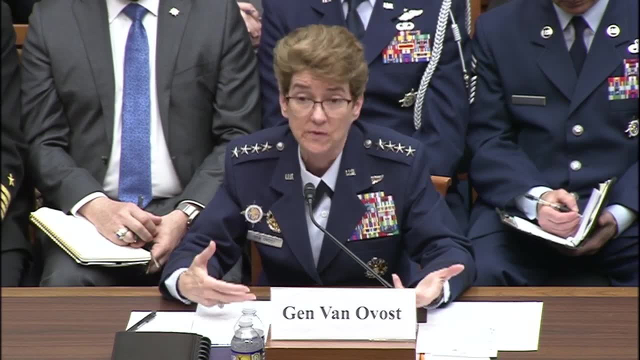 So I work with NORTHCOM With respect to transportation, making sure that it we have robust a way to defend the transportation lines, and I work with the DOT to ensure we have multiple pathways to get our cargo where it needs to go- Very good. 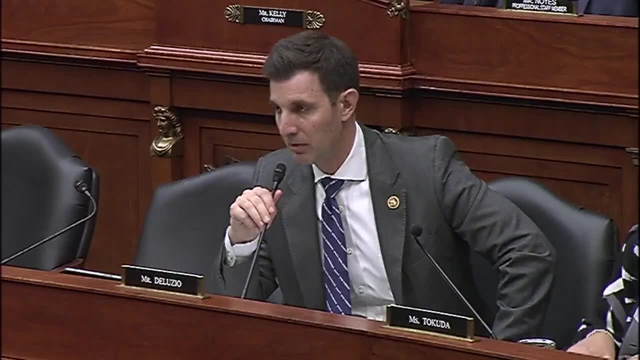 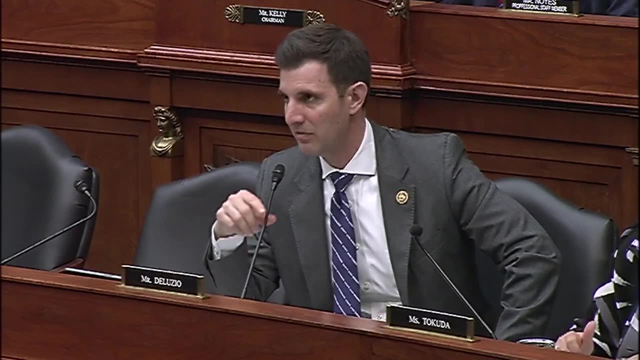 Thank you And I appreciate the department's you know announcement in the last few weeks of implementing two-person minimum staffing. I think it will help with rail safety across the board as part of my Railway Safety Act in general. Admiral Phillips, your testimony last year, the Department of Transportation, 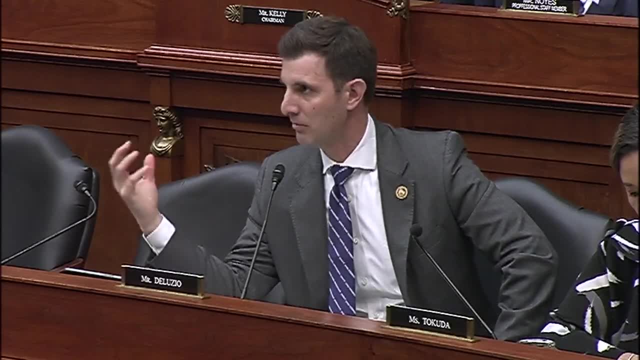 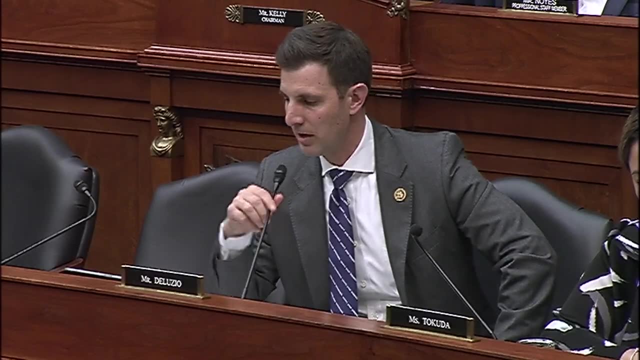 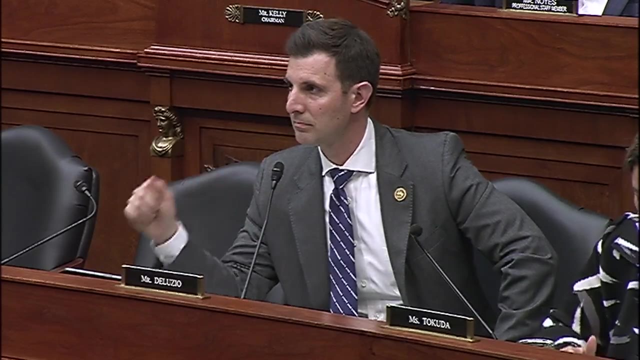 year at last year's posture hearing mentions direction from Congress for mayor had to develop a roll-on roll-off ship design for construction. we've had a little bit of this discussion there. give us a sense, where are things, what kind of updates you have for us, if any? thank you for that question, sir. we thank Congress. 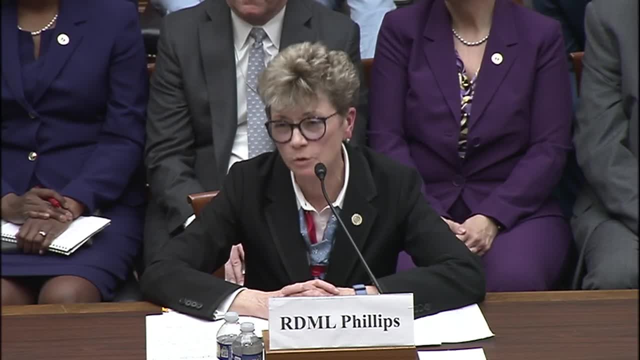 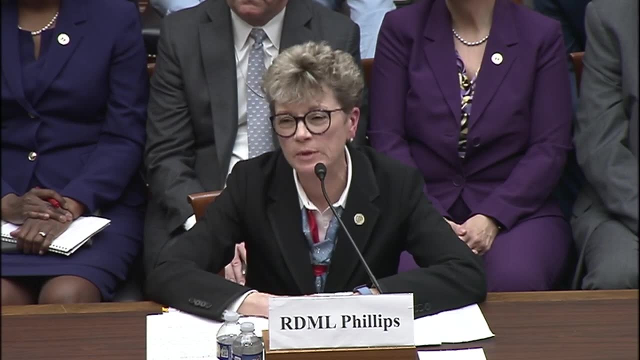 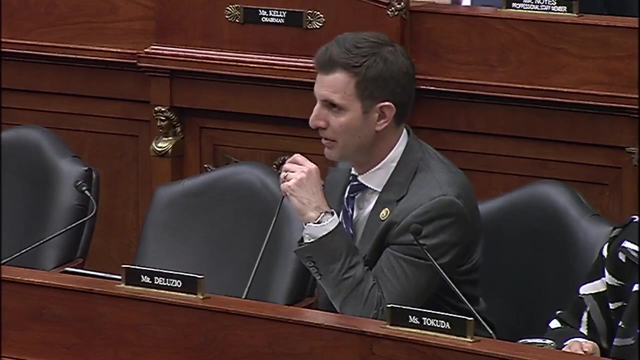 this year. for last year we didn't have any funding to do this. this year we do have funding to do this: 2024 NDA appropriated authorized 12 million and we have an appropriation for 12 million to begin to develop this design. very good, with that in mind, given the pace of things today in votes, I will. I thank the. 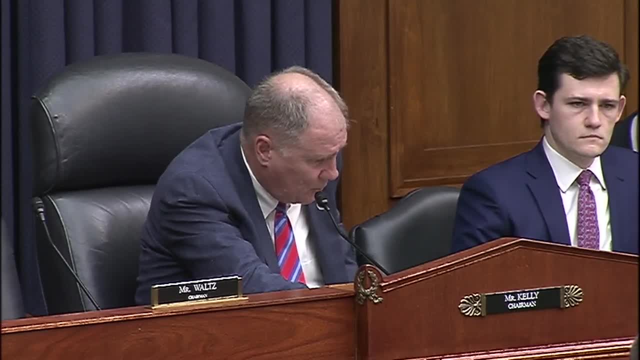 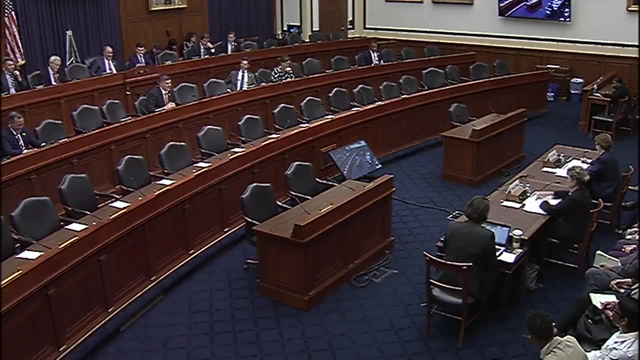 gentleman. I now recognize the gentleman from Minnesota who has an accent, mr Finstad. thank you, mr chair, and thank you both for being here and for your service. many hard-working suppliers of several different transportation systems which fulfill the needs of the people of Minnesota and the state of Minnesota. 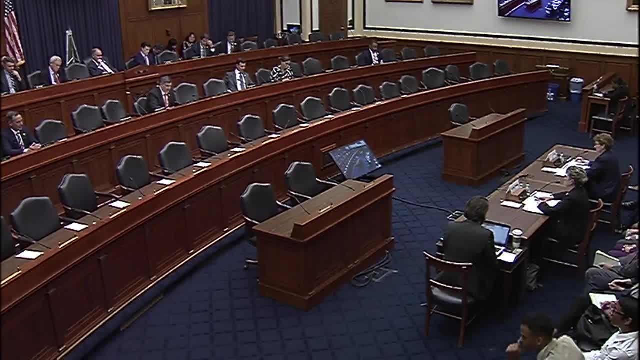 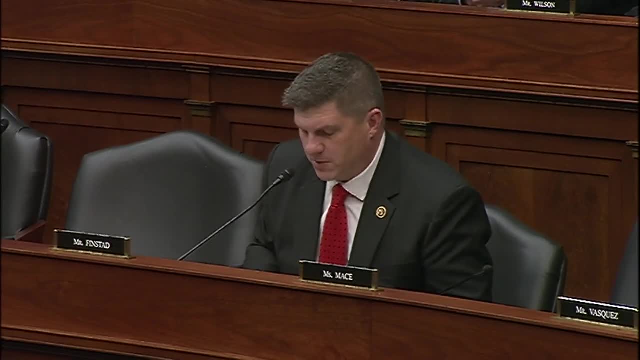 to fulfill missions and requirements for the three subordinate commands of US Transportation Command, live and work in southern Minnesota. the demand signals for the industrial base is critical to our national security projecting power and investing in the defense workforce. it is these private sector workers and innovators that will build and sustain the mobility enterprise employees and 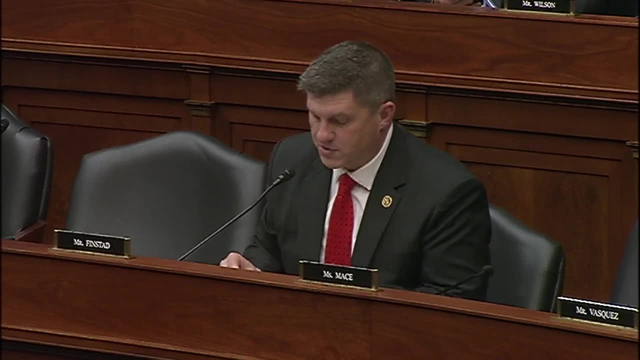 independent contractors alike have a role to play in this most important work. so, with that being said and with the acknowledgement of the time that we have here, general van ovost, I understand that US Transcom favors moving away from the independent independent contractors for truck, for truckers that move freight and household. 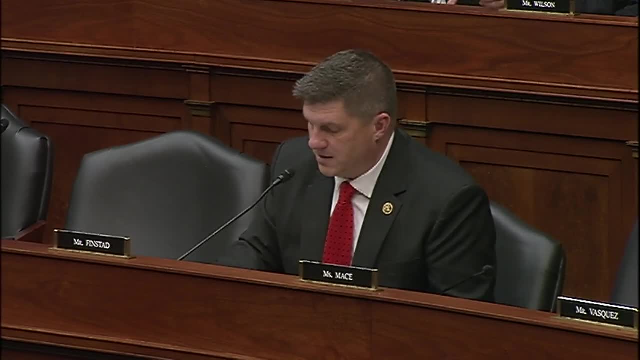 goods. do you think this is a wise move and have you based this course of action on any underlying data, considering that a large portion of our trucking fleet is made up of independent contractors? gosh well, I wouldn't say we're walking away from independent contractors. in fact, if you 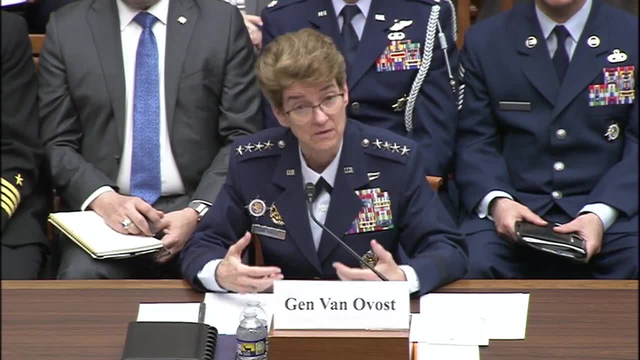 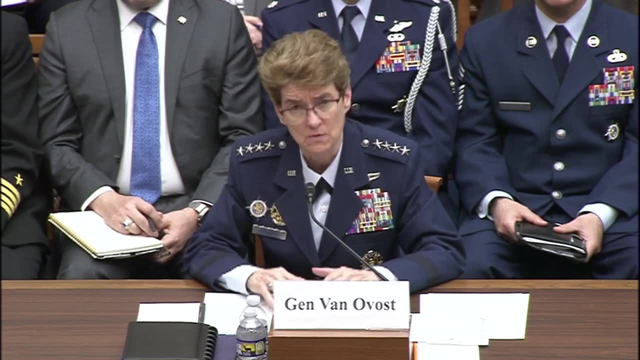 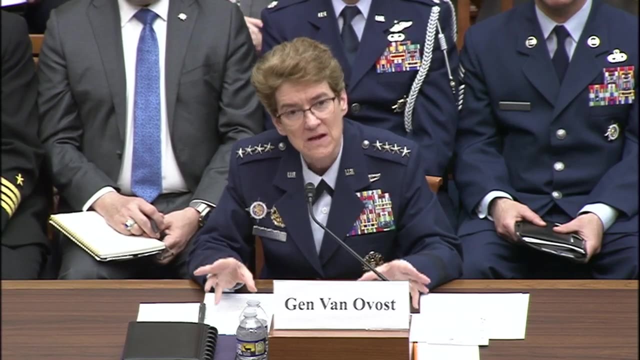 provide quality move services. you're absolutely welcome and volunteer to join the home safe alliance. again, it's a single move manager but we will have multiple sub companies up underneath. in fact, at least forty percent of the contractors up underneath. home safe alliance must be our smaller industry. 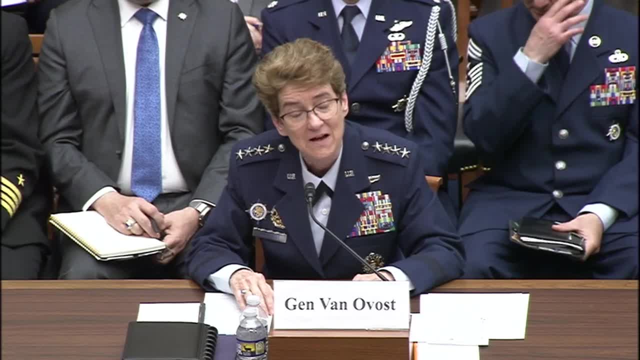 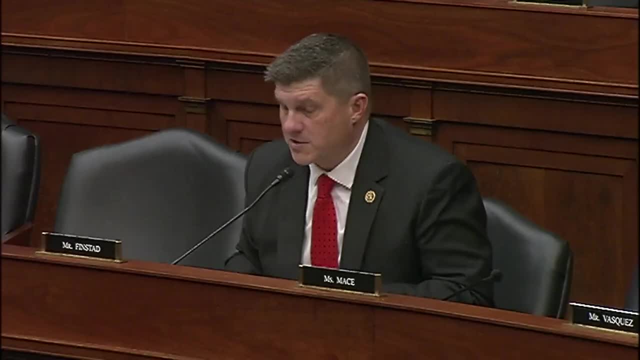 small business owners, and so we are. we are keeping a close eye to ensure that they meet the requirement. in fact, it is a performance parameter for them to meet the requirements and the quality of their service, and we are. we are very grateful to have you here today to give us a chance to be a part of this. 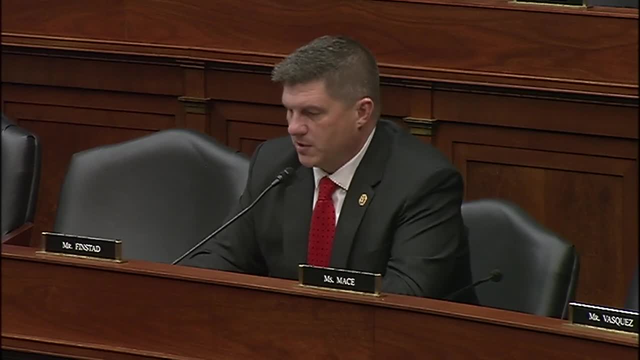 partnership with us and to be a part of the development process and to help these small businesses move away from the independent contractors. so thank you very much. I appreciate your time and your time, and your time and your time is a great opportunity to really strengthen and send signals to the. 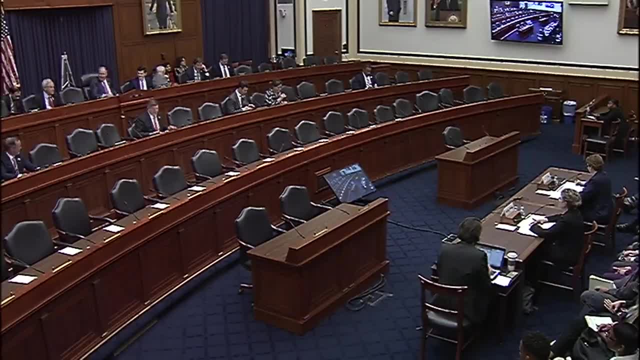 defense industrial base and and I'm just happy to hear hear your response. so with that, mr, chair me and my funny accent will yield back. I now recognize the. Your written testimony highlighted the fact that our forces are not ready, postured or skilled to optimize limited strategic assets for global patient movement. 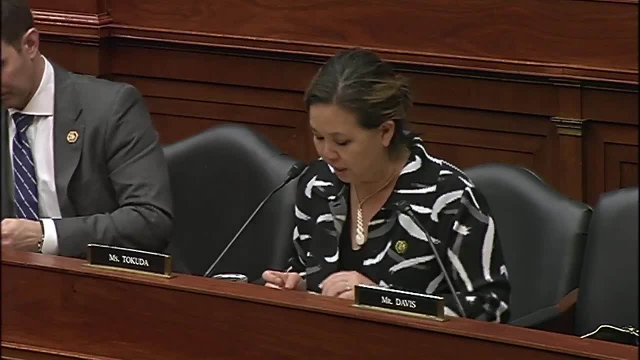 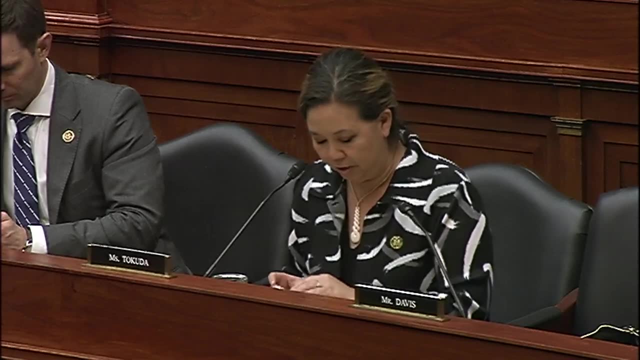 I'm especially interested in the challenges of patient movement in a contested environment and in large-scale combat operations against a peer or near-peer adversary. in the Indo-Pacific- my backyard. The fiscal year 2020- NDAA established a pilot program to enhance interoperability and surge. 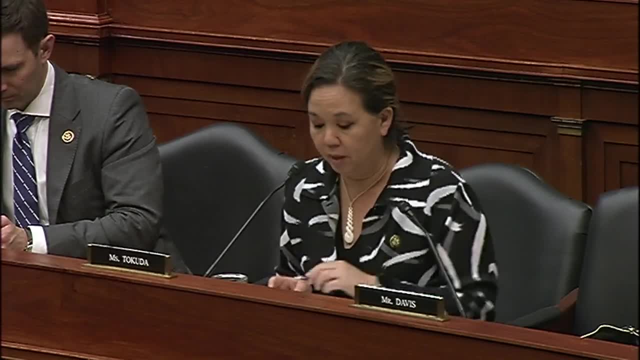 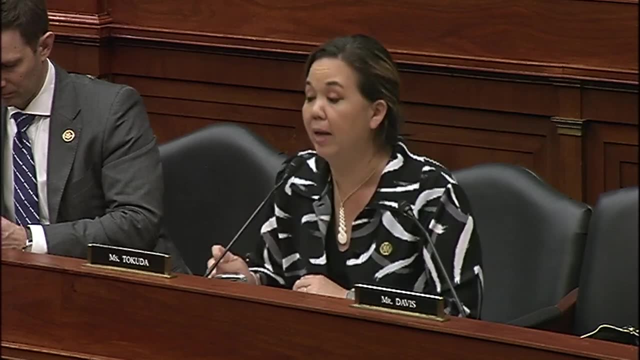 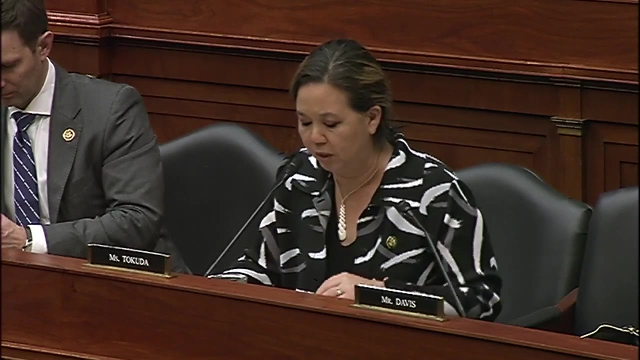 capacity of the National Disaster Medical System, which includes three main components: medical response, patient movement and definitive care. Now, I believe it, conferred by pilot sites, none of which are in the Pacific region. That being said, General, would you please briefly discuss how Transcom works with and? 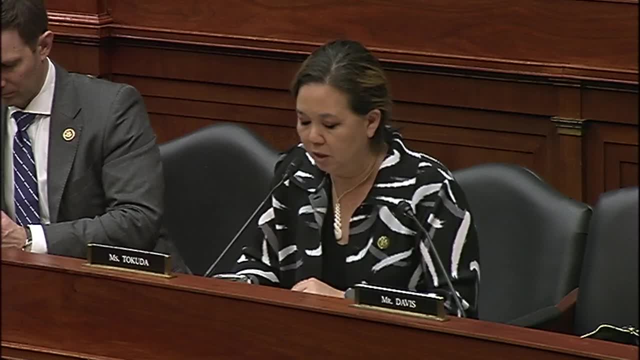 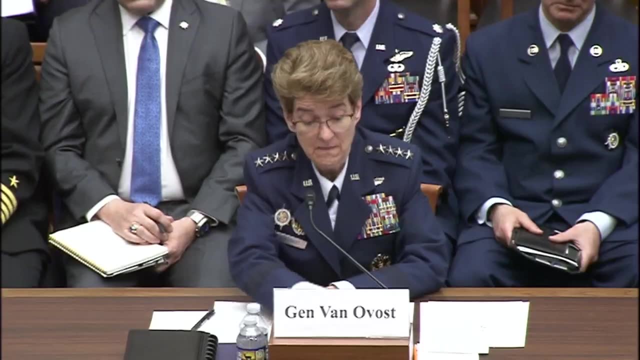 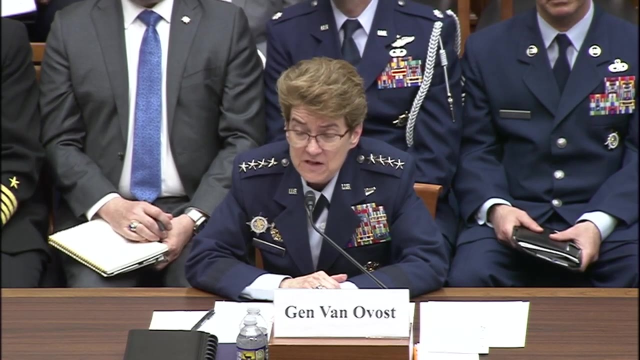 integrates the National Disaster Medical System into your planning for global patient movement in a large-scale Pacific contingency. I'd like to first point out that our air medical evacuation personnel have performed brilliantly over the last few decades to save our servicemen and women around the globe, and I'm immensely proud of what they. 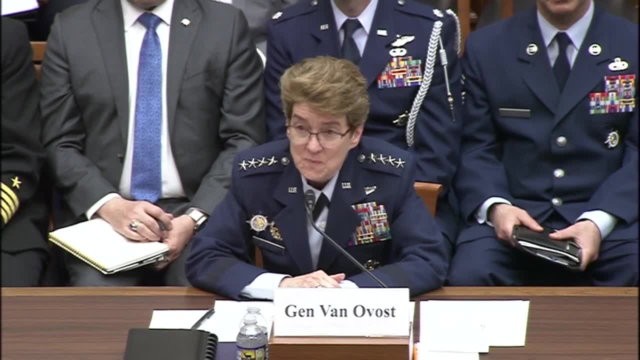 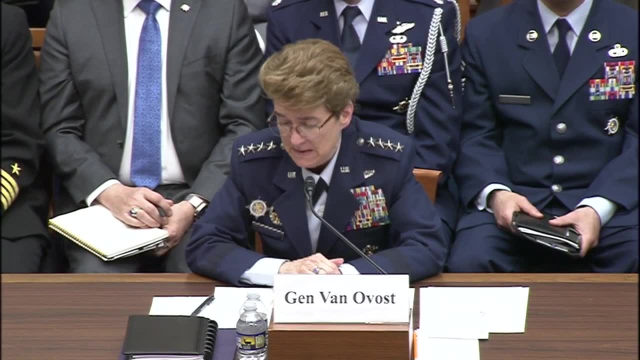 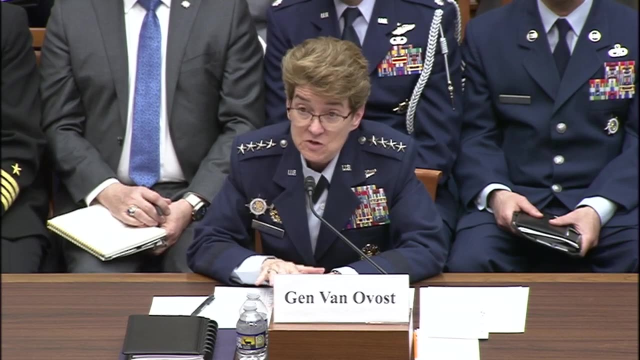 do every day. That said, we are at risk to meet the casualty demand expected in a large-scale combat operation, especially in the waters of the Pacific. In fact, we expect to have to move the amount of the entire patients we moved last year. 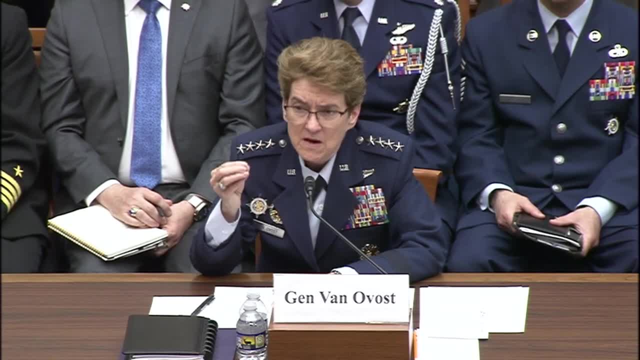 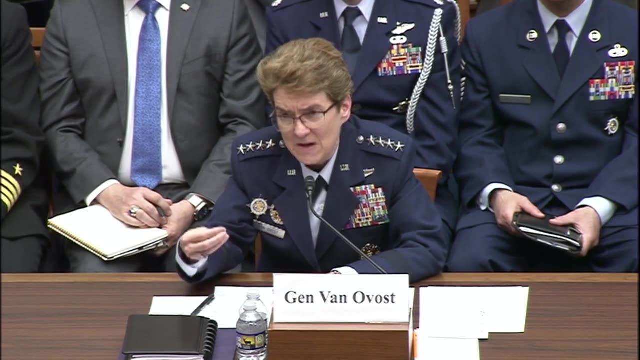 in one week in such an event. This is how we have to think about, how we're going to have to change our concepts of operation and our modes and actually how we deliver. when we think about people having to dwell in theater, how we have to partner more with our allies and partners to provide medical 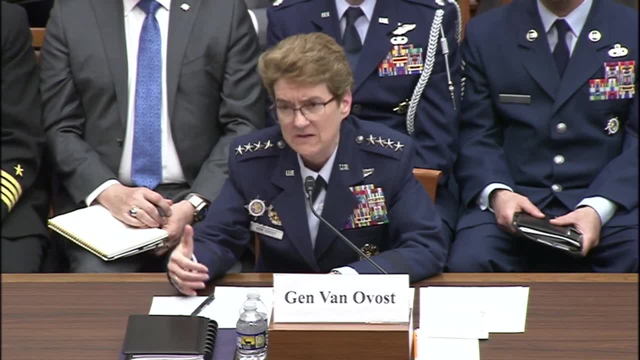 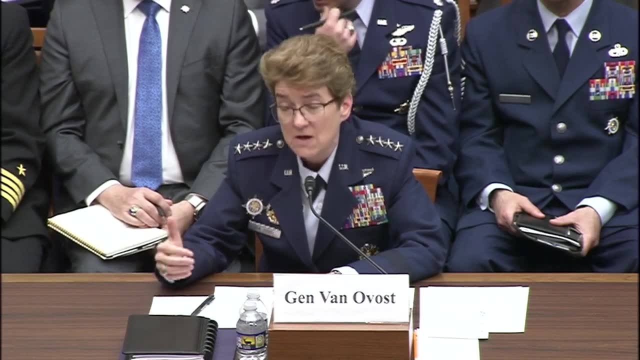 capacity in theater and how do we make those routes streamlined to get back to the United States? And when we get back to the United States I work with US NORTHCOM to work with the NDMS to try to distribute those patients. 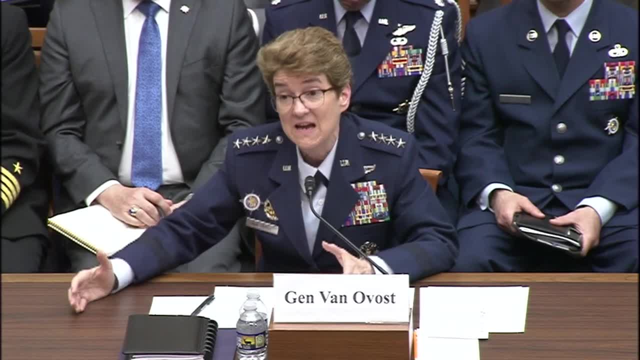 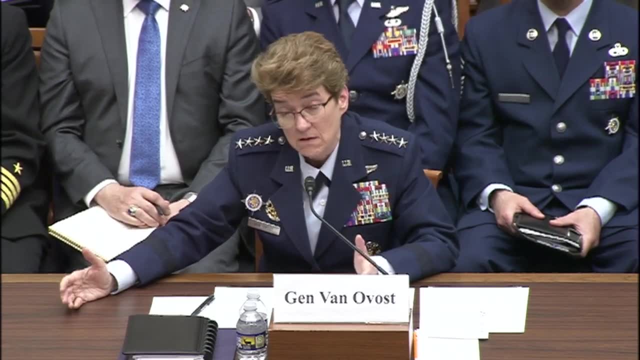 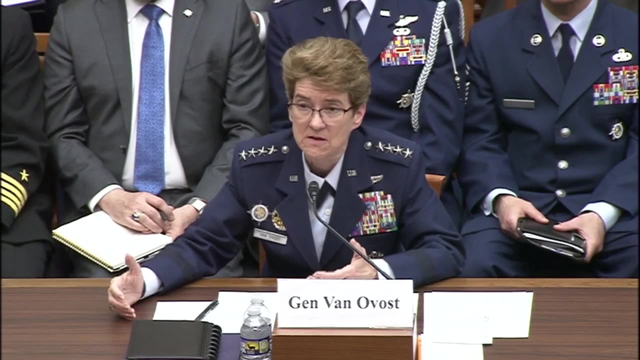 So, again, this is an end-to-end discussion, but it's at the volume that we've just never seen. In fact, we really haven't seen. should we lose a ship? you know mariners in the water, how we pluck them out of the water and how we get them into the system. 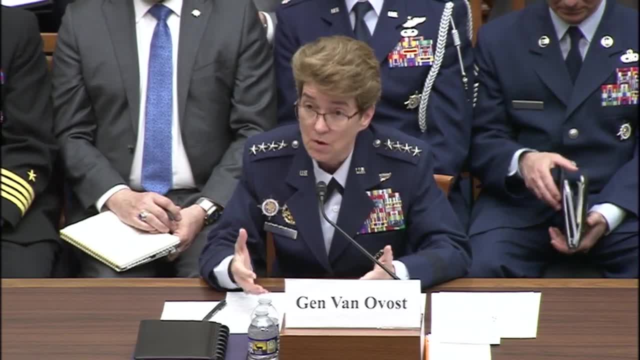 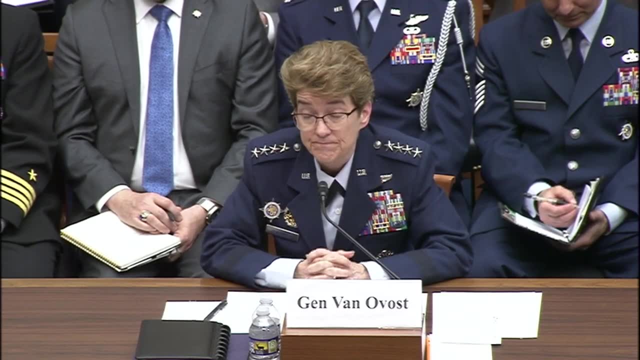 So we are really. this is going to be a whole-of-nation effort. We have to go to war and we're absolutely going to be using all services and resources of our nation to deliver. Thank you, Thank you. I know I'm running out of time. 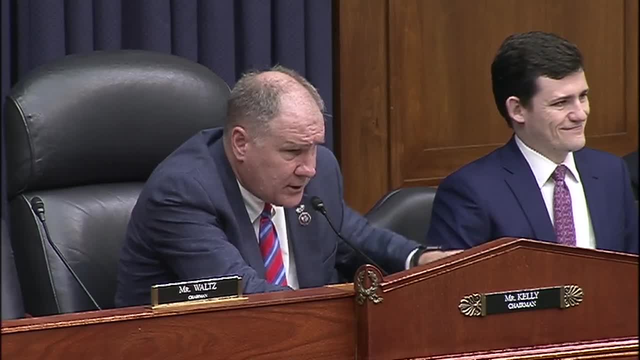 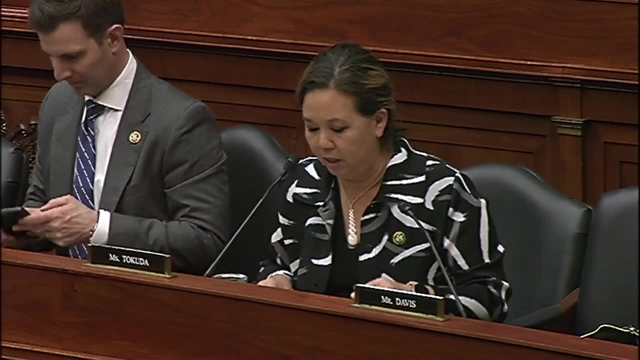 You're not. You've got an additional two minutes because they didn't restart the clock, So you've got an additional two minutes to what's showing. That being said, I know that we do have to go to votes. I would suspect that if we are looking at some kind of large-scale disaster engagement, 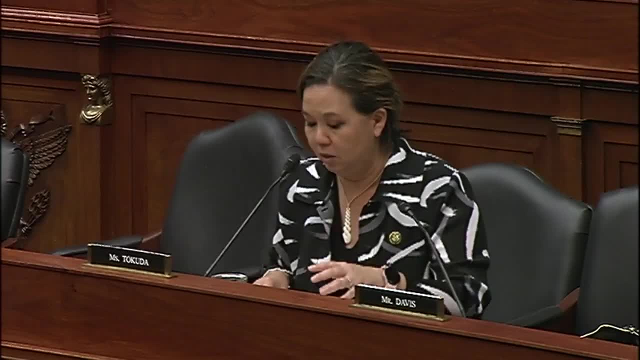 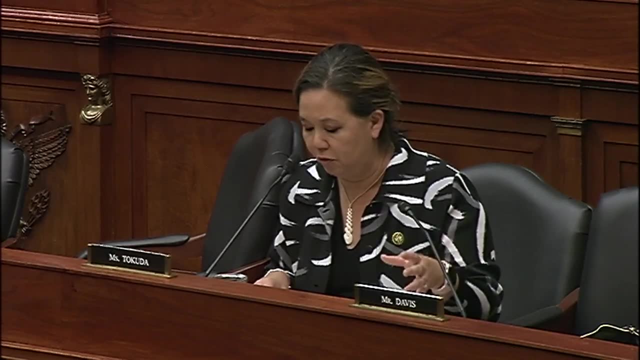 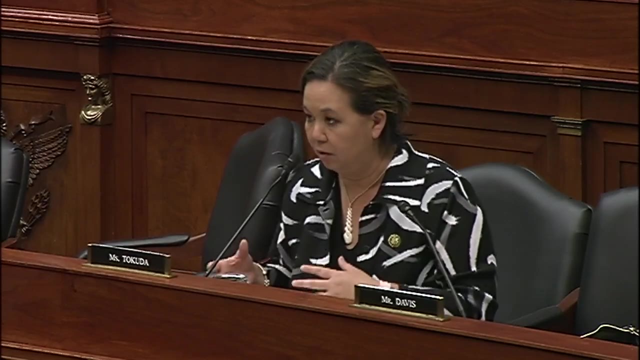 casualties in the Pacific. Hawaii would play a critical role in supporting patient movement and care, especially as we get them towards the continent. You know what kind of challenges do you foresee with transportation infrastructure, both in Hawaii and in the Pacific places like Guam, in terms of our ability to conduct aeromedical 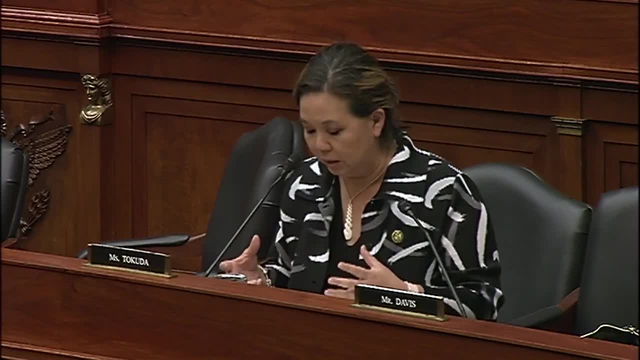 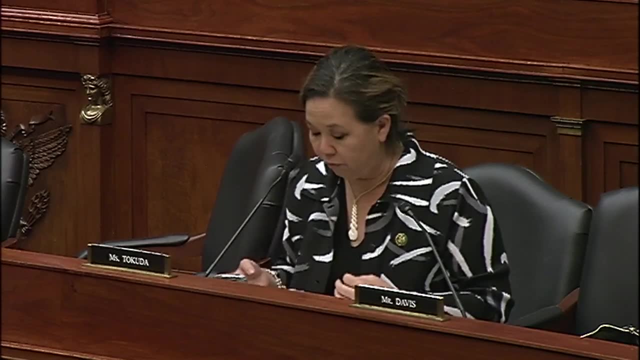 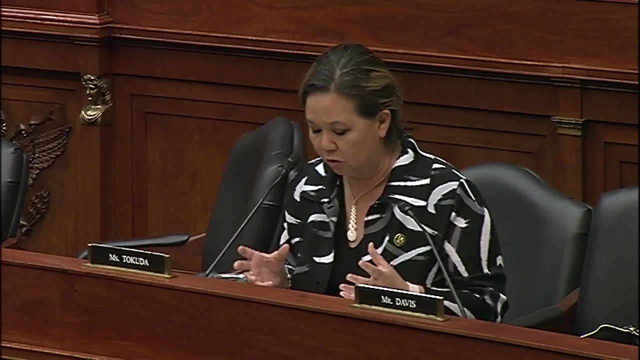 evacuations. Also, one big problem that we face consistently in Hawaii, which will only get worse in the case of some kind of contingency, is having sufficient medical workforce equipment, supplies, facilities to be able to support healthcare needs. As Transcom is thinking through, what kind of surge capacity for healthcare staff and 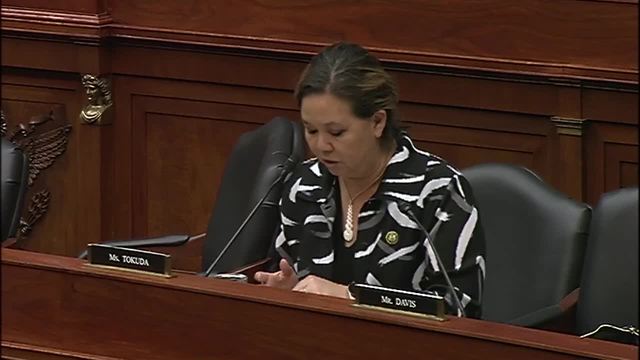 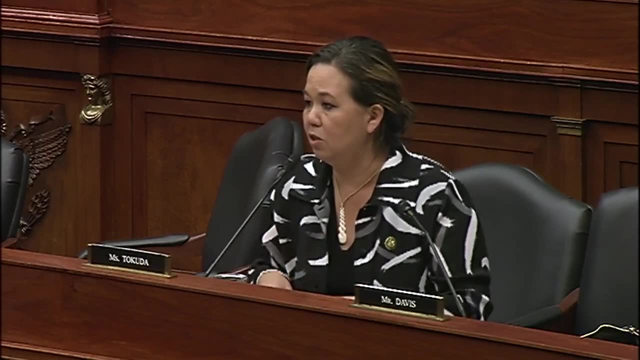 facilities we need to be prepared for, whether military or civilian, to meet any kind of situation, movement or care through the Indo-Pacific, through Hawaii, again to the continent. Thank you, We are doing a lot of thinking about the entire network. 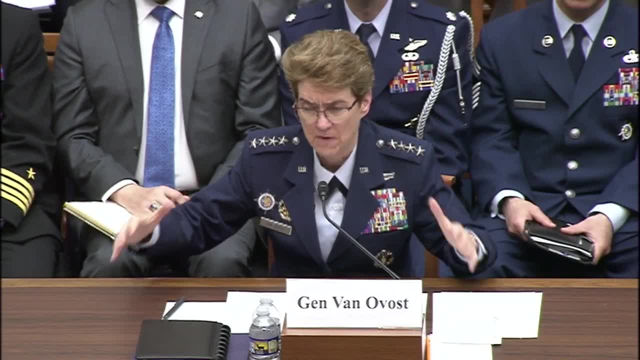 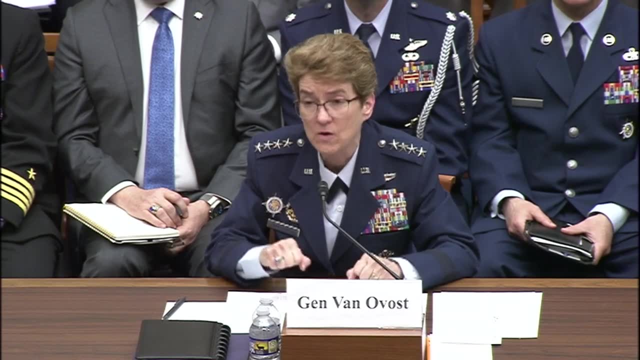 Again, I'm responsible for the end-to-end movement of patients around the globe, So we are re-posturing. where would we hold patients? where could we bring them for rehab? You know a tripler would certainly be, you know, an option for that. 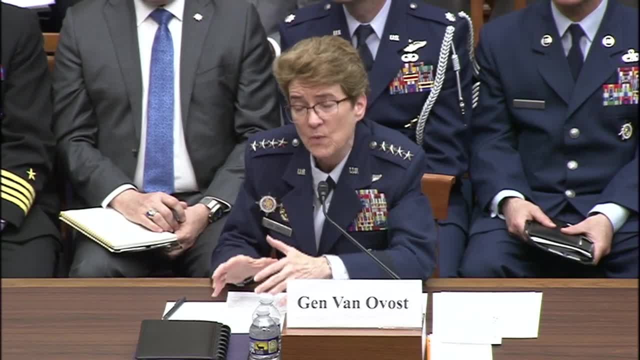 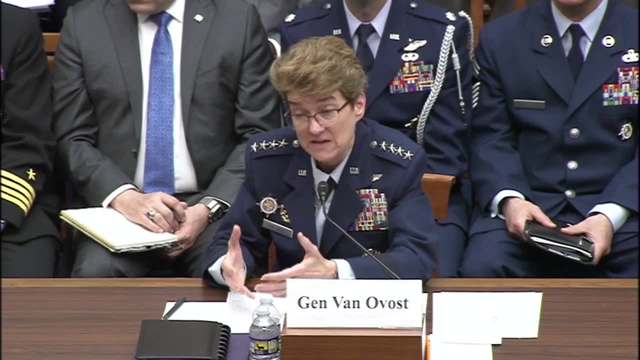 And so, as I work with NORTHCOM and NDMS on where we'd have to expand, we're thinking, you know, about new concepts and new ways to take care of them. So that would be necessarily the downstream work as we set requirements for different. 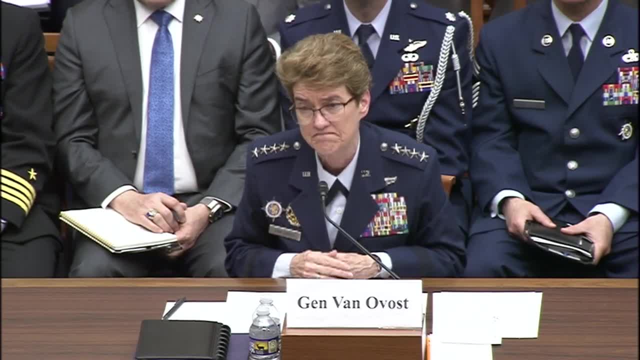 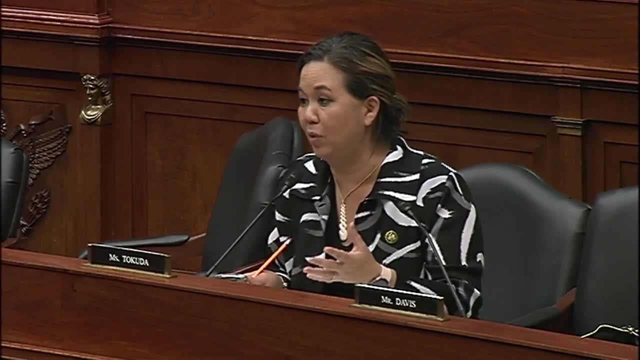 locations around the Pacific and in the United States. Thank you, And you know, I know that, as I said, five pilot sites. perhaps, if there are an extension or additional pilot sites, one in the Pacific would be a valuable one, so that we can really 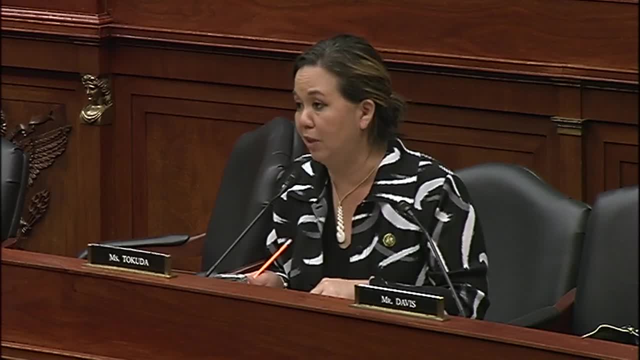 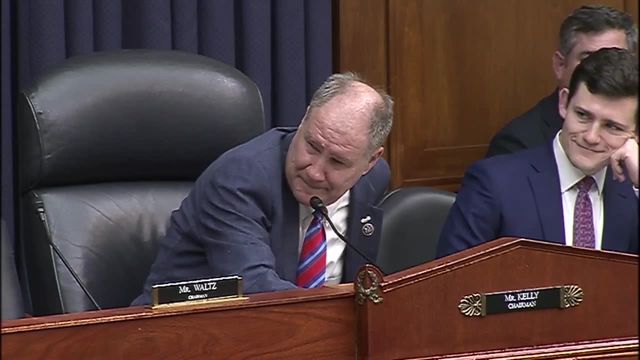 start to look at what will be necessary for us to be able to prepare for any kind of conflict and mass casualties. Thank you, Chair. I yield back. I now recognize Mr Jimenez. Thank you, Mr Chairman. You know, during World War II, for every aircraft carrier that was built by the Japanese, we 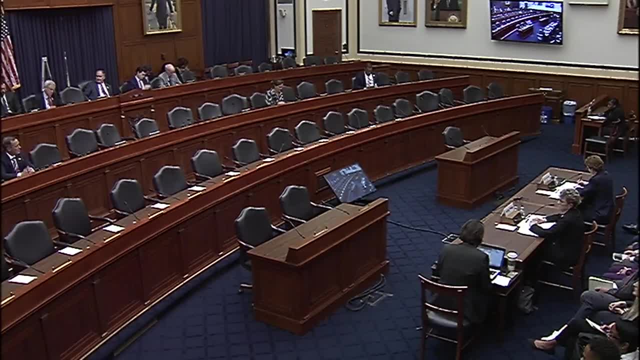 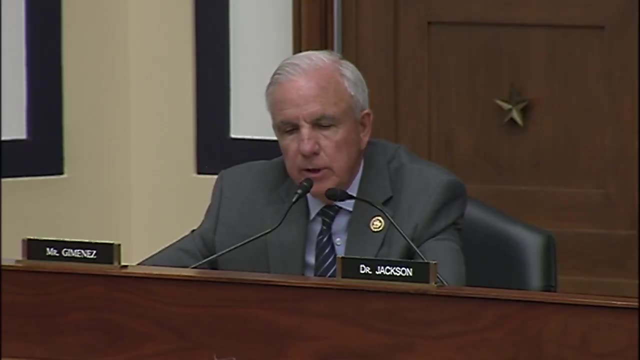 could build six. Unfortunately for us, today we're Japan, China is us, except their capacity is much even – it's even greater than what our advantage was in World War II. We must, Mr Chairman and colleagues. we need to make shipbuilding a defense, a security. 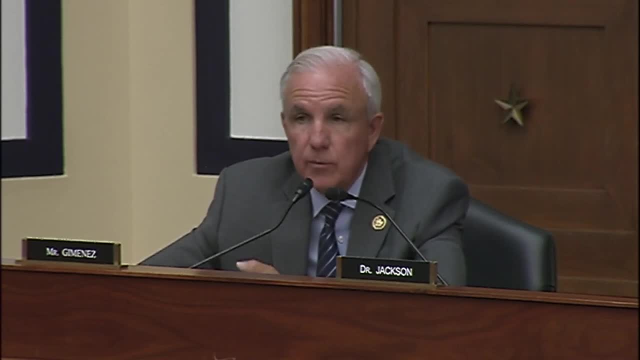 priority And it's not going to be done here. Whatever we do here is peanuts. to be honest with you. when you look at, you know really what shipbuilding capacity is all about. And when we're talking about nine ships or 20 ships, that's nothing compared to the capacity. 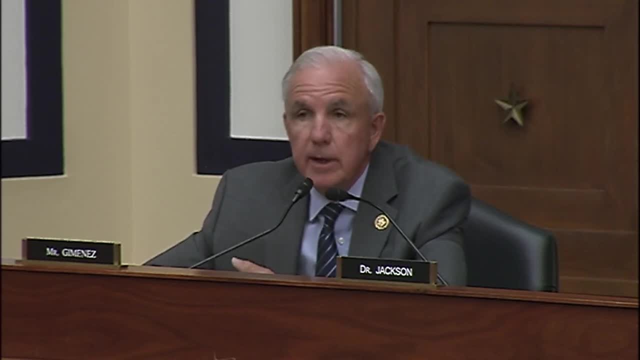 that China has. So we need to play the game that China played. They played it very well. They subsidized their industry. They captured the market, The market. now the world is dependent on them. They've got all the capacity And they did it. 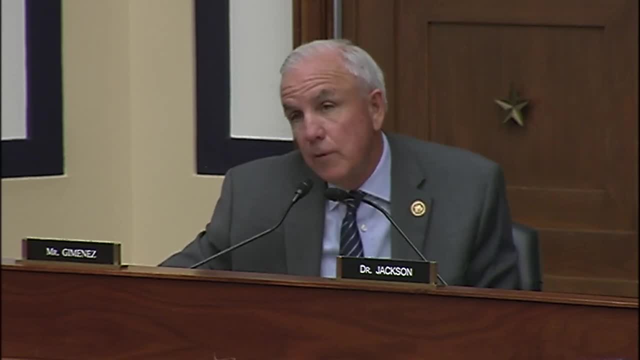 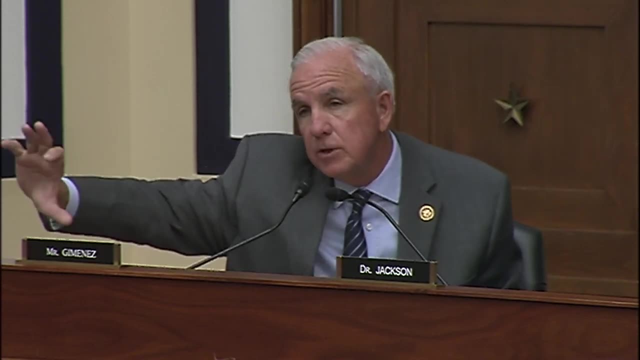 Probably not, Mr Chairman. They're not using what we call fair trade. They use their own –, they subsidize their industries, And that's what they do, by the way, That's what they do for everything that they feel to be strategic. 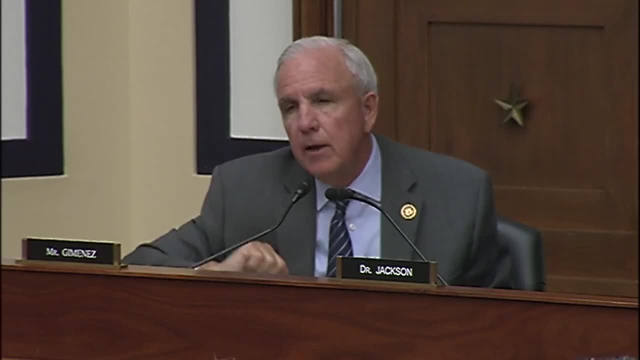 All those industries are strategic for them. They subsidize it, capture the market and then they got it. And so we've got to start playing some of that game, not just here in Hask, but on a whole-of-government approach. 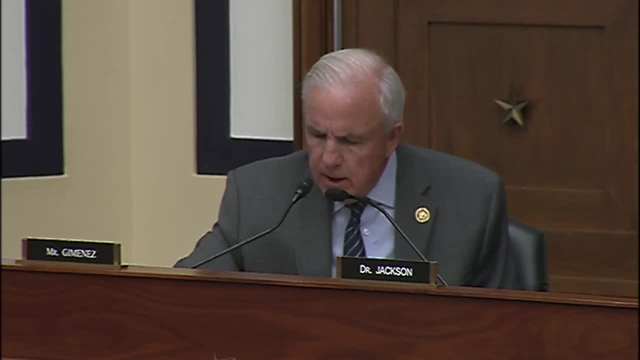 And that's my comment for this. But my question is to you, Admiral Phillips. the Port of Baltimore is home port of part of the military SEALIF Command's National Defense Reserve Fleet. What is the assessment of their ability to respond with the tragedy at the Francis Scott? 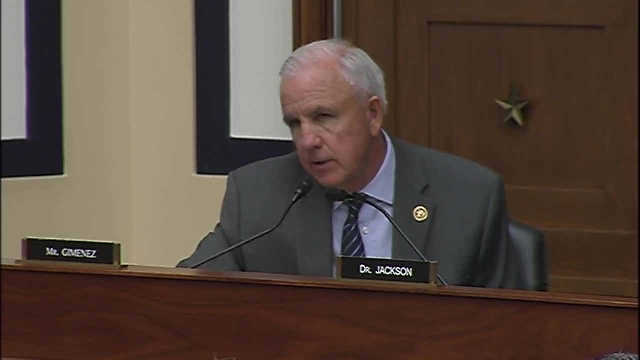 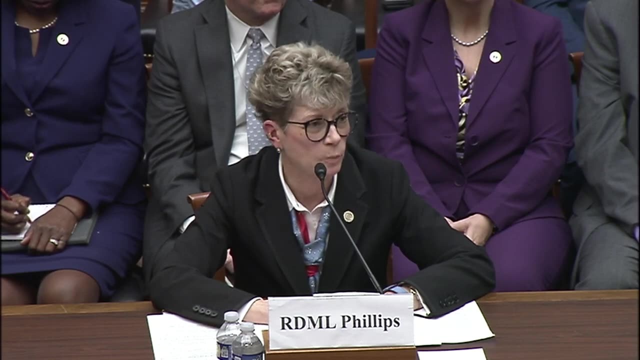 Key Bridge where any of the vessels impact by this incident. Mr Sir, thank you for that question. We maintain – typically we have six ships there. We have four in Port Baltimore right now. Two of the four are under maintenance. The other two would be full-up rounds. 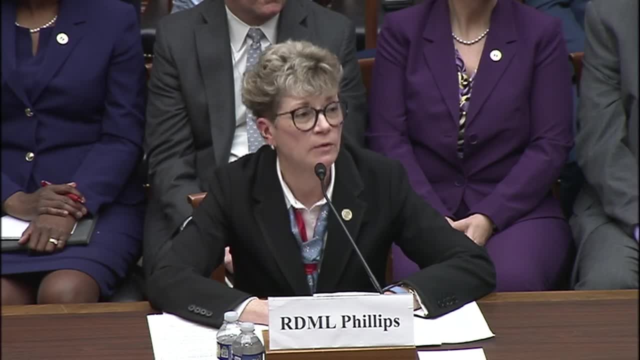 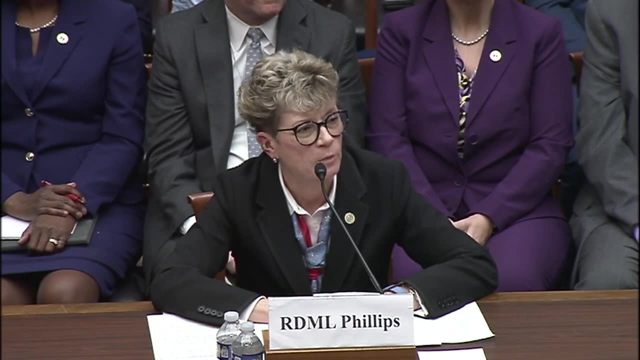 They are unable to leave the port. I would add that we believe, once the 35-foot channel is open, which we expect at the end of April, that they were all – they are all clear. should they be recalled by the Department of Defense? 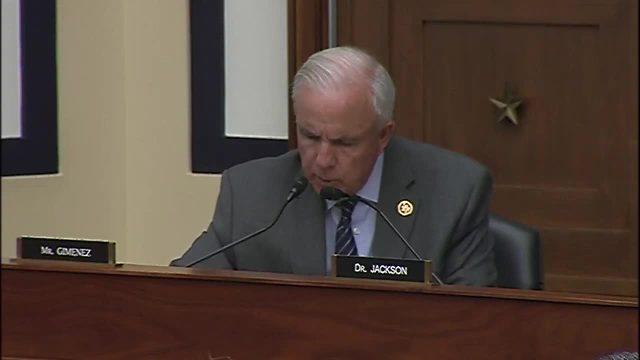 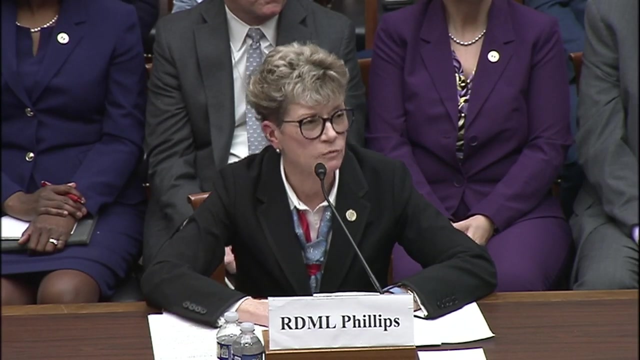 Were you prepared for the event like what happened at that bridge And are there any contingency plans for, let's say, a Black Swan event or deliberate attack on our key infrastructure, like bridges, that could bottle up our fleet? Mr So, sir, as you're aware, there are 48 total vessels in the Ready Reserve. 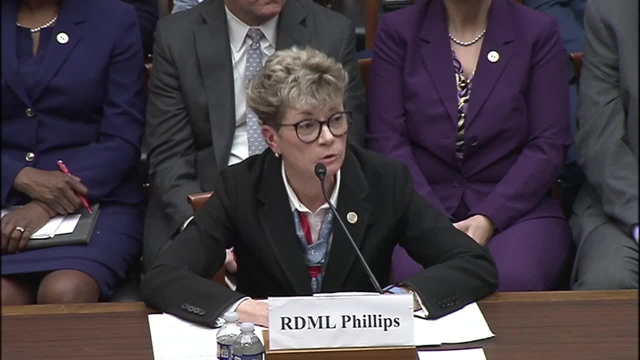 right now There are no additional vessels stationed around the country with similar capacities that would be available. Of course, a Black Swan event is always a challenge to anticipate, But we – that is exactly why we don't station them altogether and we station them strategically. 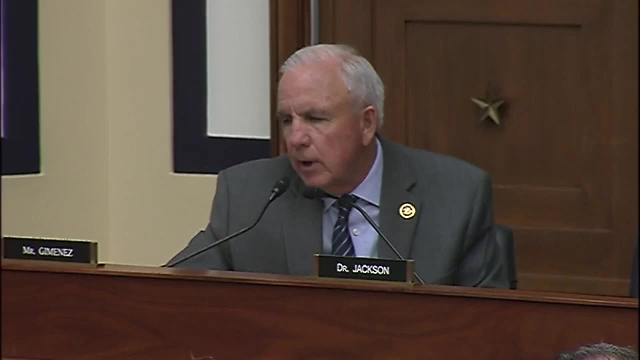 around the nation, Mr. Finally for you, Admiral, I'd really be interested in your views on how we can build – we can restore shipbuilding capacity here in the United States and not on an incremental basis, Somewhere to – it really meets the – you're not having a huge fleet in your video. 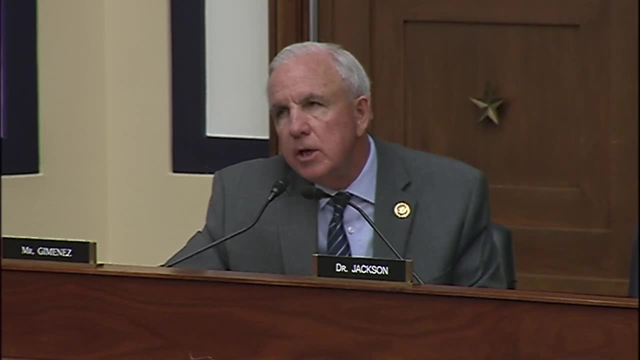 I see that Mr Of course 务 meets the security needs of this country. I really believe this is a critical piece of our security infrastructure and that we have been asleep at the wheel and we don't have the capacity to respond like we used to. certainly don't have the capacity. 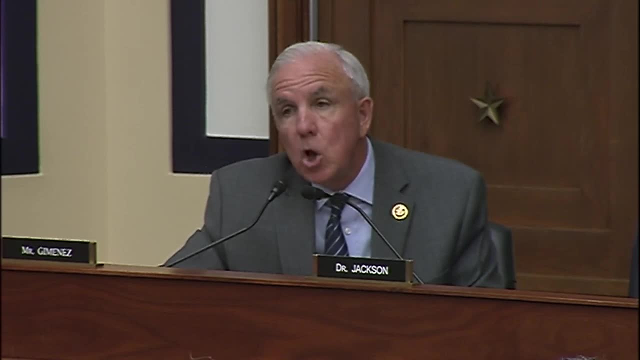 to respond to an adversary like China. This is going to be a long-term thing. It is not going to happen overnight. How can we get back to having at least the capacity that we need to maintain our freedoms here in the United States? I appreciate. 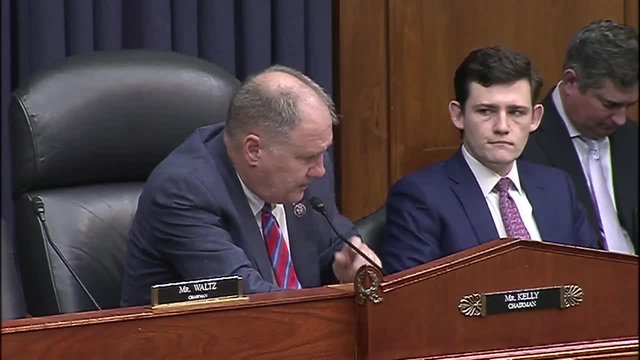 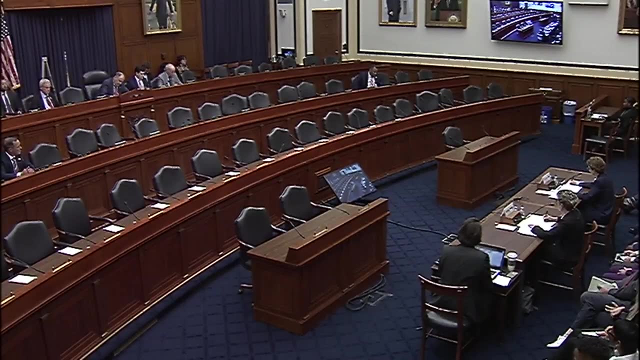 that And I yield back The gentleman in the back. I now recognize the gentleman from Texas, Mr Vesey. Thank you, Mr Chairman General. I wanted to ask if you could talk a little bit about the V-22.. I know that the 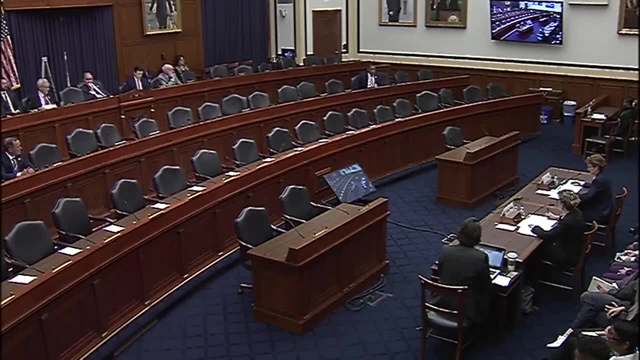 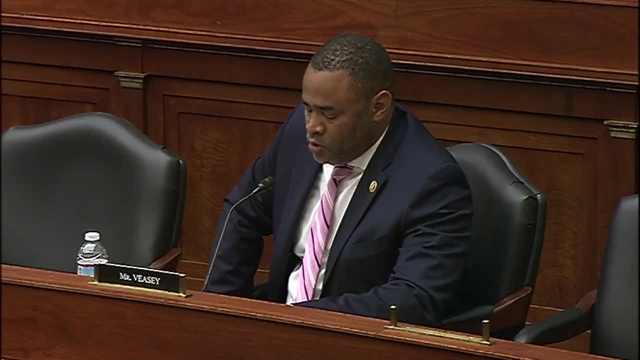 Pentagon has cleared it to fly again and given the unique capabilities that the V-22 has, particularly in rapid intravehicular transport, can you speak to how the V-22 fits in the operational strategy, particularly in terms of missions that require both speed and versatility? 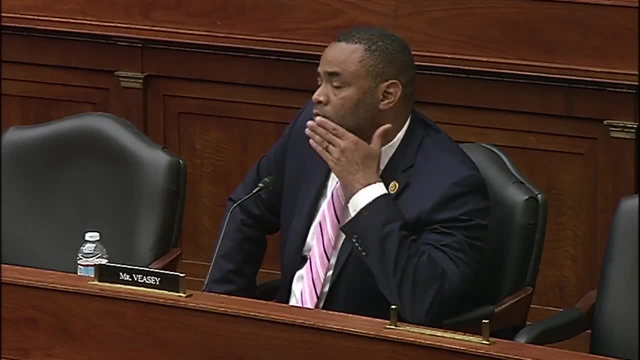 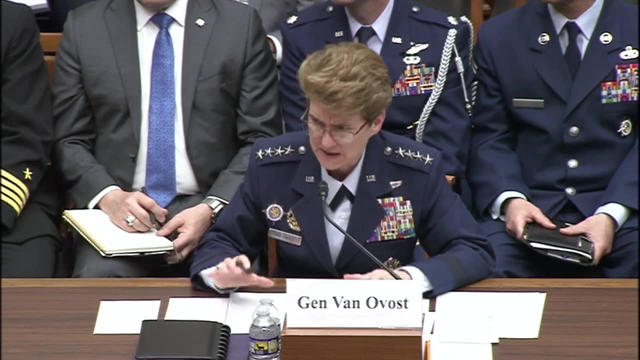 I would love to talk about the V-22. as much as I love it, It is a great airplane. However, I would ask you to speak to the Navy and SOCOM about the airplanes. I don't have them in my web drawing. 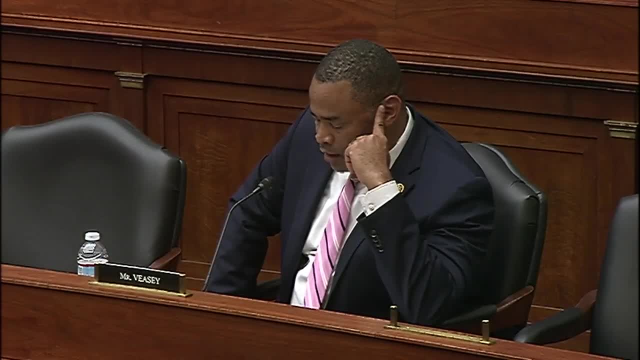 Okay, And then I also wanted to ask you- and I talked with you about this before- I know that it has taken nearly six years, from the initial announcement in 2018, to begin implementing the new military household goods and services, And I know that. 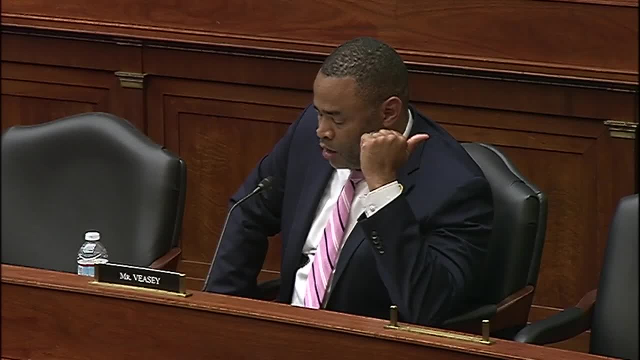 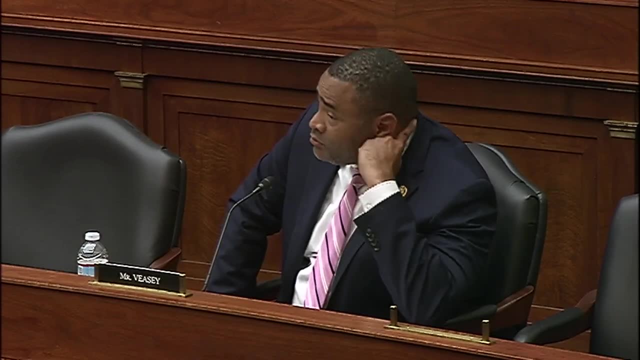 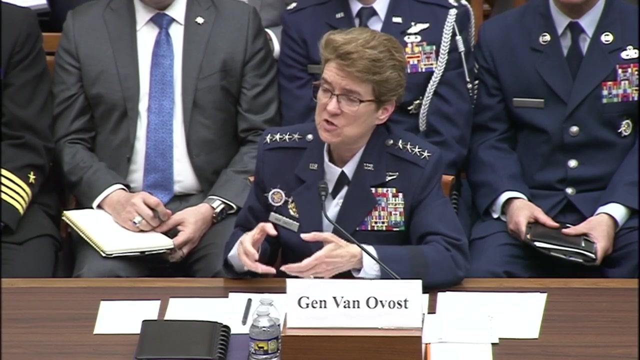 the V-22 has a very good shipment system And I wanted to ask you, why are these specific 14 installations chosen for the initial rollout? Thanks, We were doing a conditions-based rollout and we've started here in April, And we chose those locations because 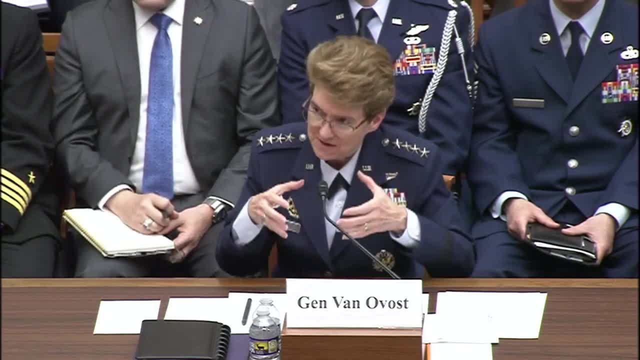 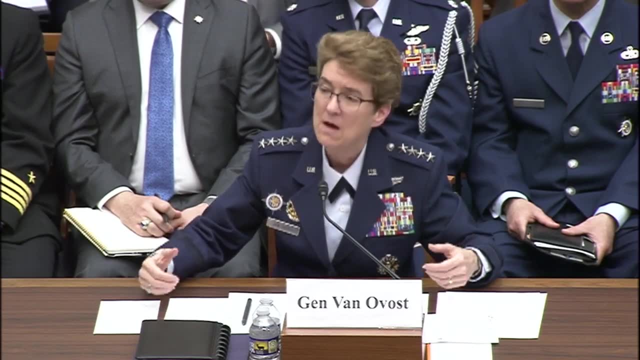 the services said that they were ready, because this is not just a single contractor, We are changing the entire model. So we've worked with the services to train them. They came forward and said: we're ready at these locations And it made sense. 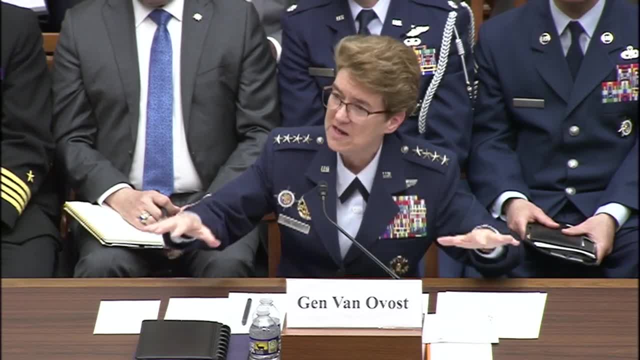 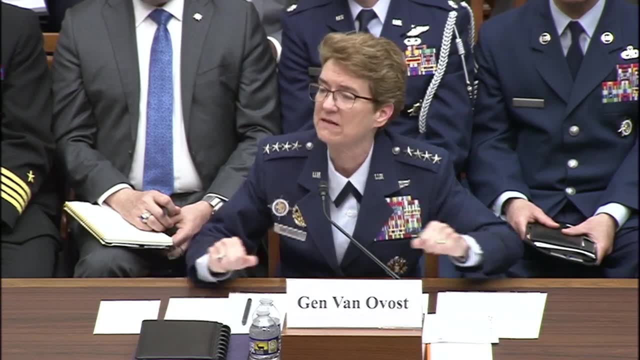 These are local moves within 50 miles, And so, as they chose sort of the heat map of where the most moves would be and where they were the most ready, that's how we selected them. We do all of this in conjunction with the services. 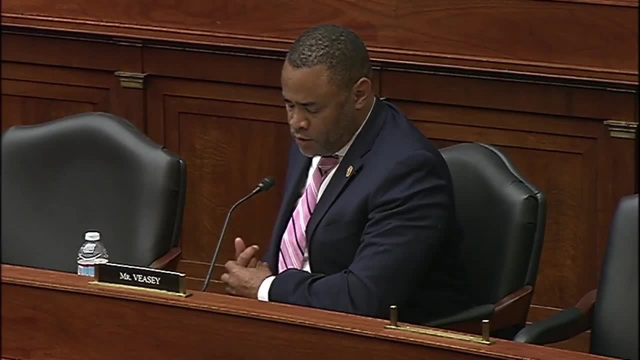 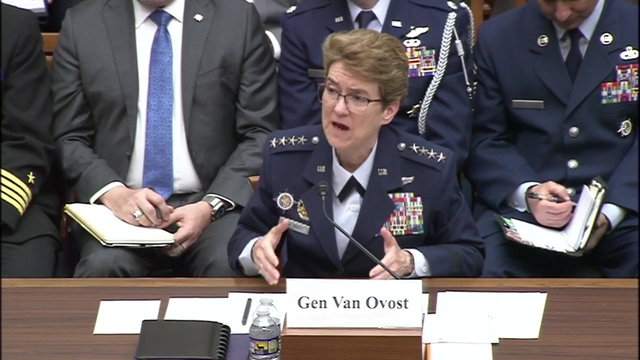 Okay, And what are the parameters for success? in this initial phase And based on the current schedule, when do you foresee the new system being rolled out to encompass 99 percent of service members? Yes, So we are going to pause bringing on new capability during the 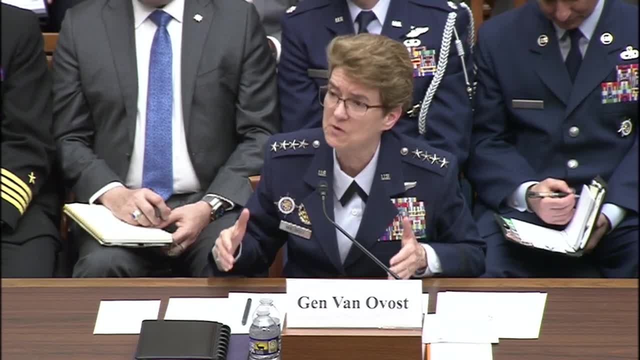 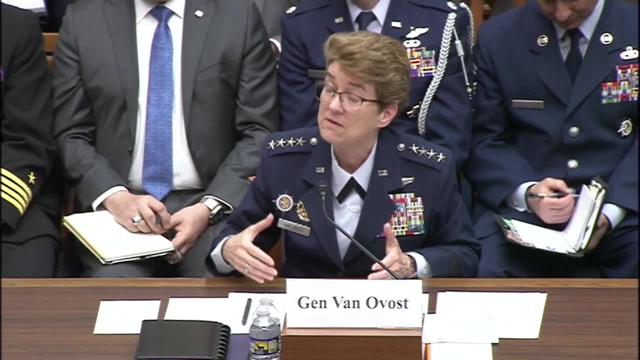 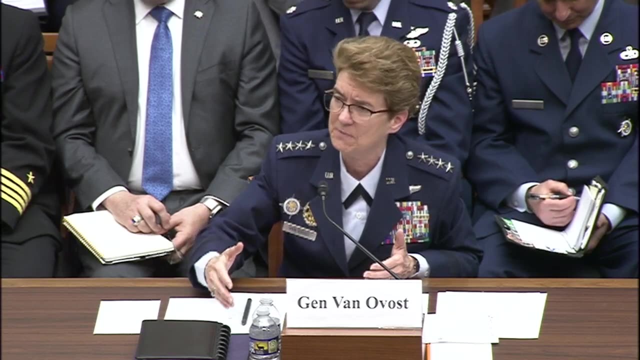 peak season to reduce risk and really focus on customer experience. So the vast majority of this season will be done under the old tender of service system And then we'll begin full domestic ramp-up through the end of this year, about September, through December And then all the way through to next year. 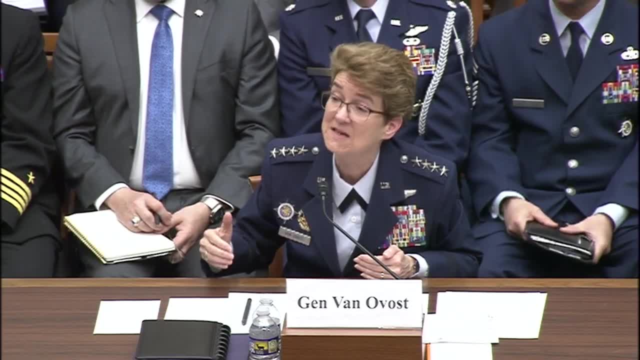 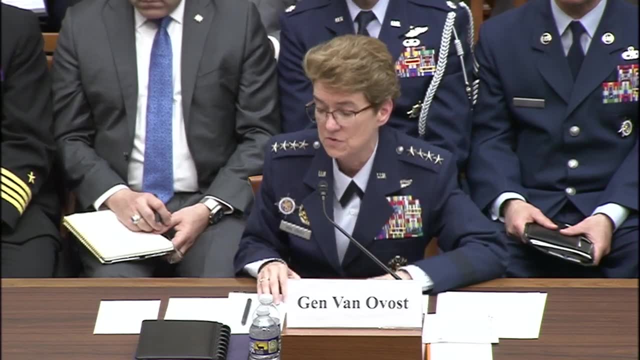 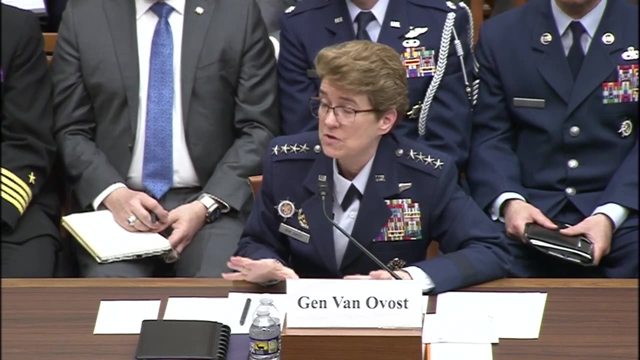 we'll start doing overseas moves beginning in September And then ramp up from there Again, deliberate, conditions-based approach to this capability. That said, we have, you know, almost 30 metrics that we watch. We gather data every day, do analysis weekly on the metrics. 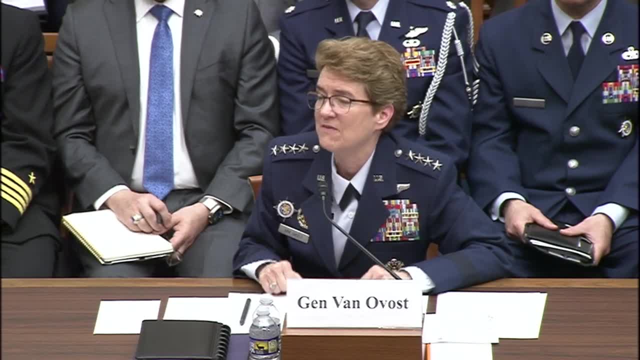 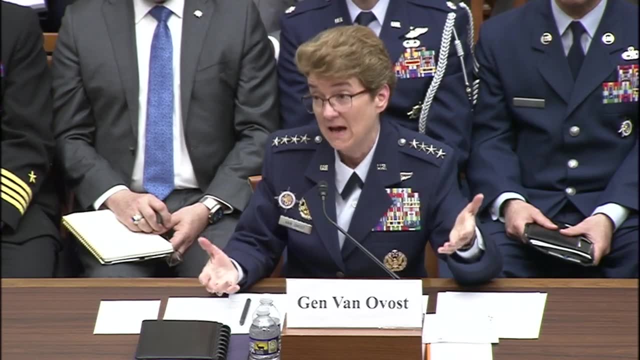 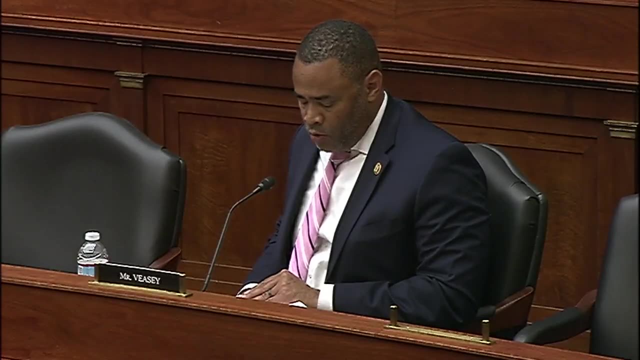 that they're going to be graded against So immediately we will be able to see if there are any concerns and provide immediate feedback, And that feedback is also available well to the services and to the company and some vendors. Yeah, I wanted to ask you also: how do you think the moves? 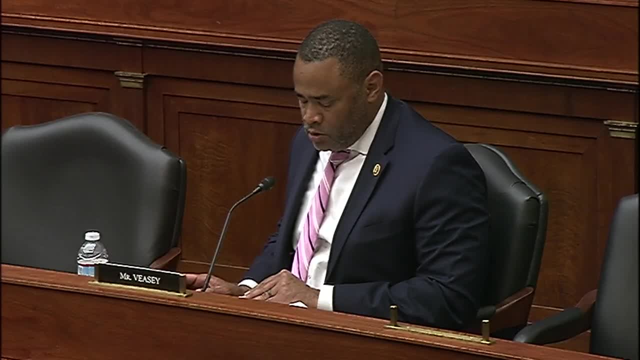 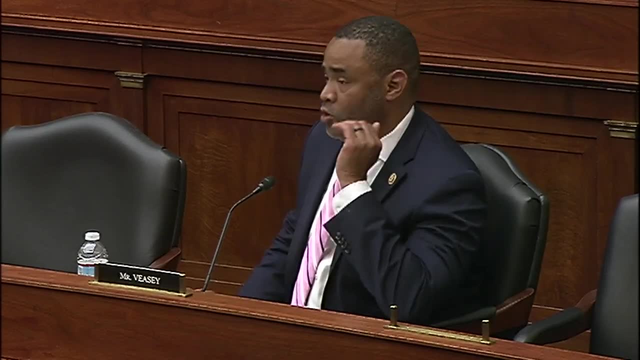 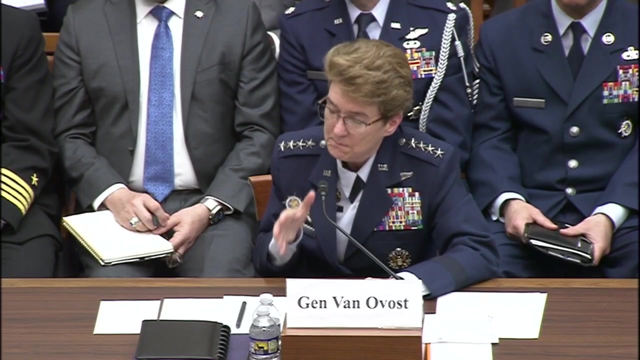 if you look at the current experience versus the new system that you want to put in place for the military move-in system, what steps are being taken to ensure that the enhancements are going to be effective? Absolutely, Look, the current Tender of Service program does not provide consistent. 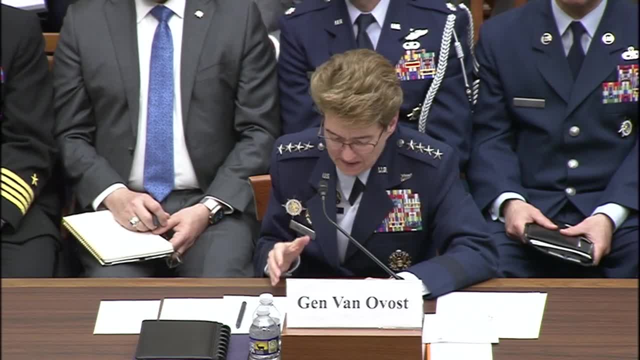 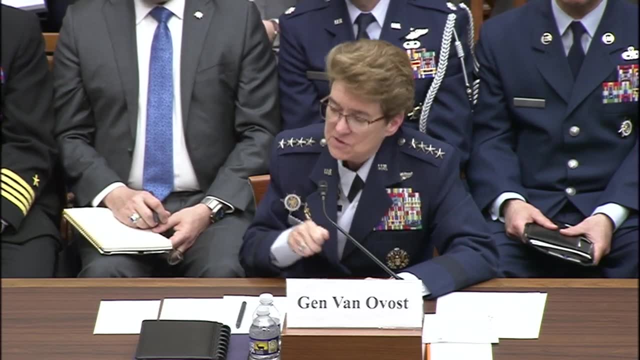 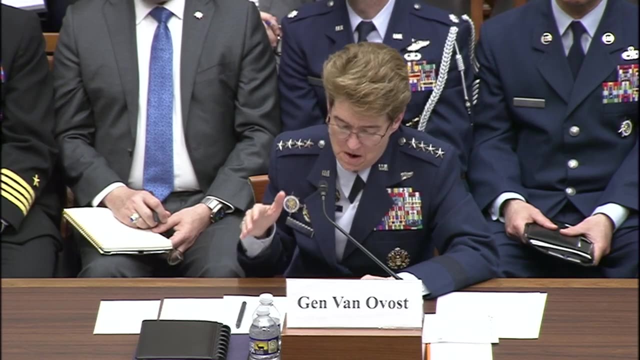 high-quality moving experience for our service members and their families, and it's difficult to hold industry accountable for performance failures. So this complete change in how we're doing household goods, as really mandated in 2018 by Congress, this is going to help us achieve a standardization and integration. 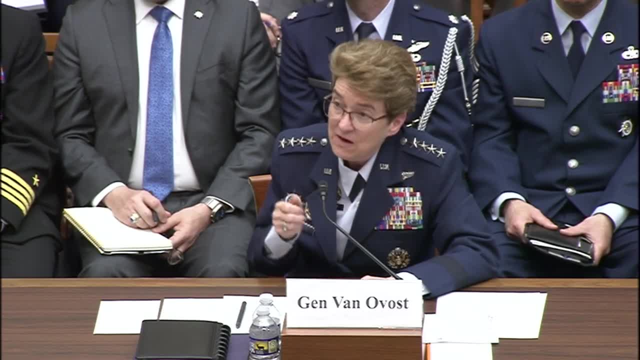 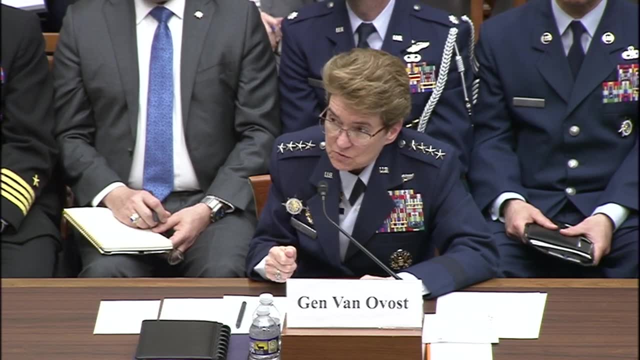 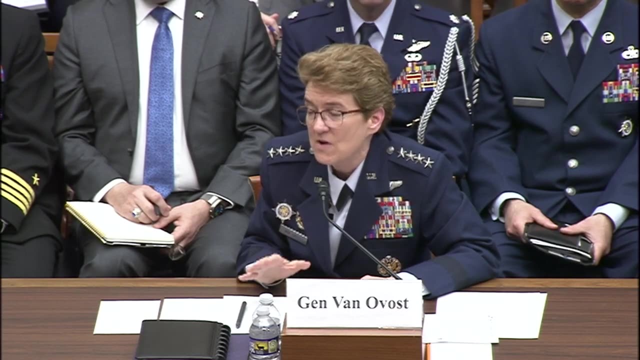 and capacity management that we can achieve today. Accountability with defined standards, with trained personnel, modern digital management tools where you could do the move on your iPhone, enhanced communications and simplified claims- again that we do not have today. So, given all of those changes, we think it's going to be a radically different experience. 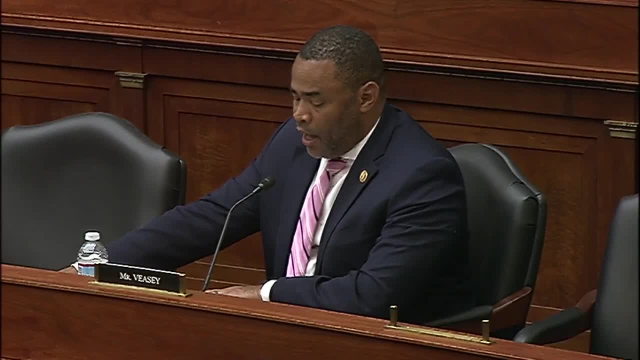 And speaking of the accountability that you just mentioned, how is this new system as far as service quality is concerned? how is it going to handle potential issues that you hear from families dealing with loss, damages of people's belongings during the move-in? 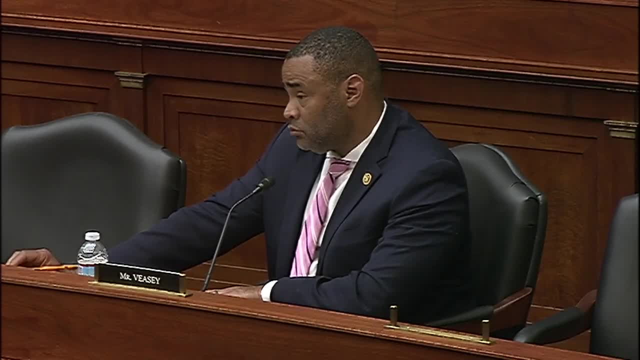 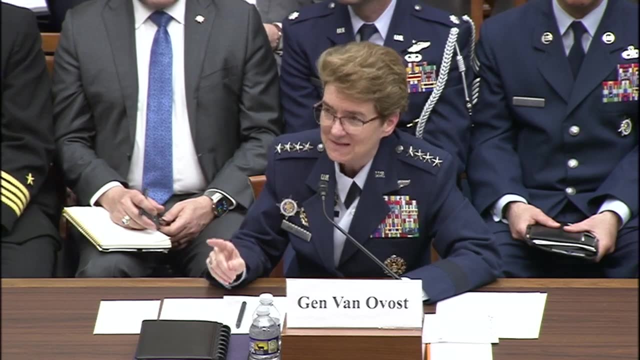 Yeah, we now have a 24-7 contact center, and the quality assurance representatives that are at the locations that will visit on-site are cleared to immediately make a call if there is a problem, which then gets funneled to a center that's going to take care of the problem right away. 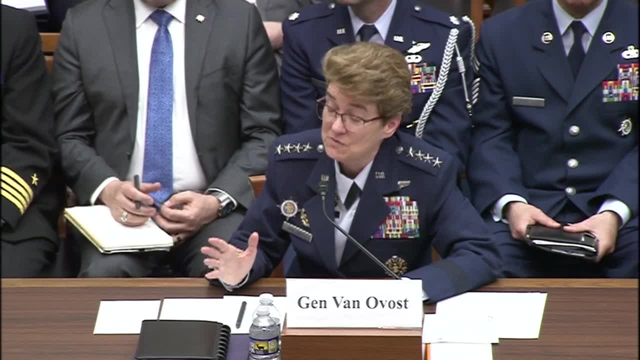 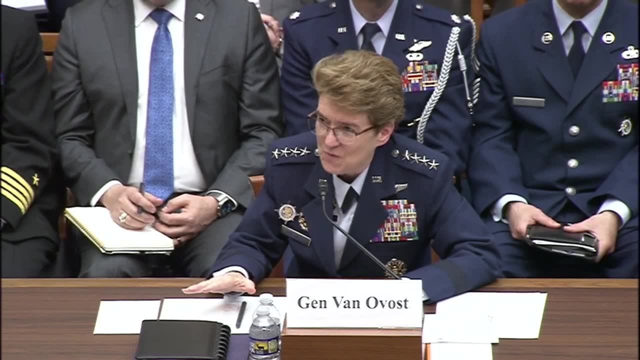 So we will know immediately if things start to go off the rails, because what we really desire is that our service members and their families have a confident, pleasant, quality move, no matter where they're moving. Yeah, thank you very much. Thank you, Mr Chairman. I yield back. 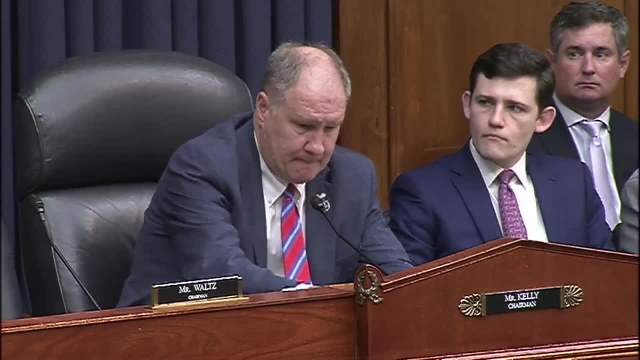 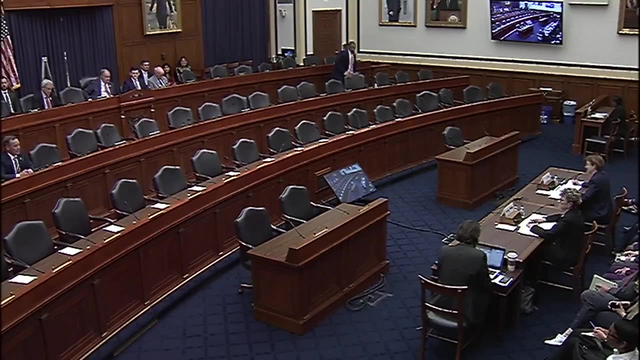 Now I recognize the gentleman from Guam, Mr Moreland. Thank you, Mr Chairman, Thank you, General. Thank you, Rear Admiral, for your testimony, And, General, I appreciate your visits to my office. It's been really helpful. 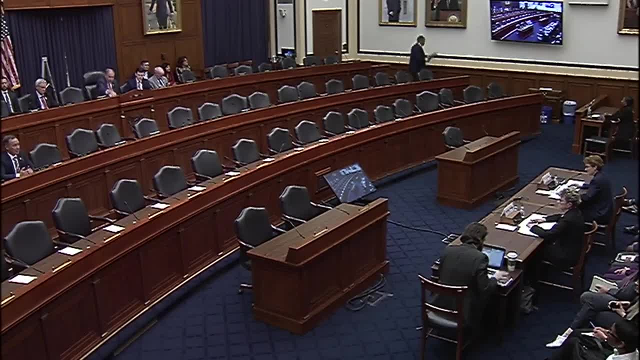 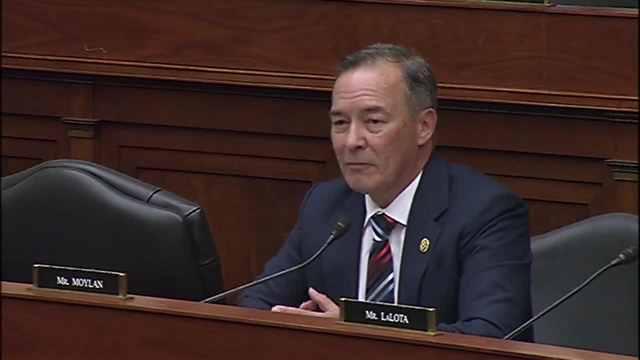 And I truly support your objective to ensuring that we have the fleet that is necessary, absolutely. And once we get those ships into, especially the Indo-Pacom area, we've got to get it loaded and unloaded And General. in our last meetings we talked about the urgency. 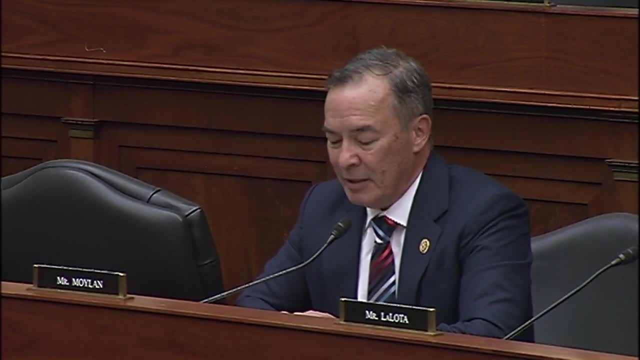 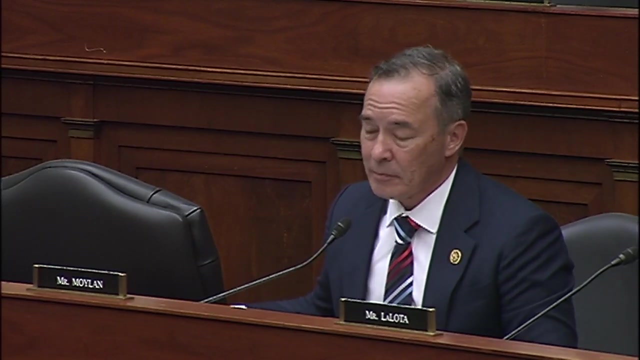 of funding the Port Authority of Guam and its unique role for the Department of Defense. Can you please elaborate on the necessity of the Port Authority of Guam in US transcom operational structure and what infrastructure there is critical to your mission? Thank you, I'll tell you it's an understatement to say how important Guam is. 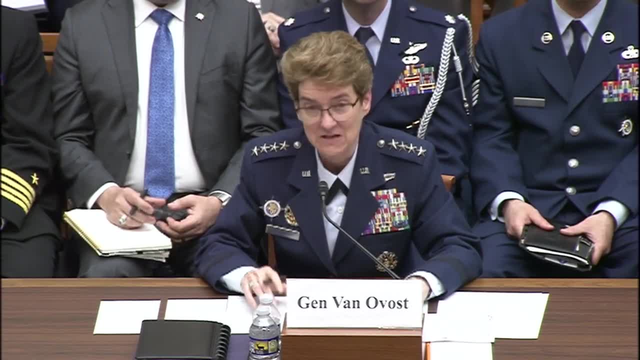 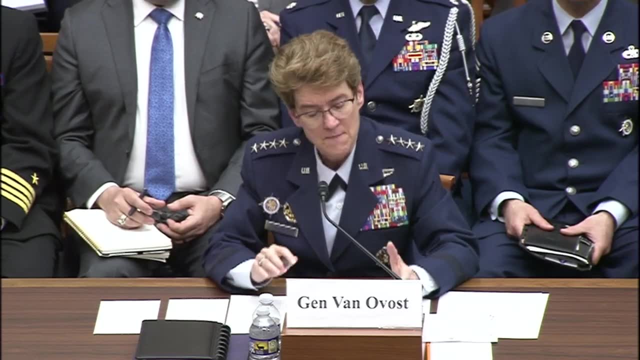 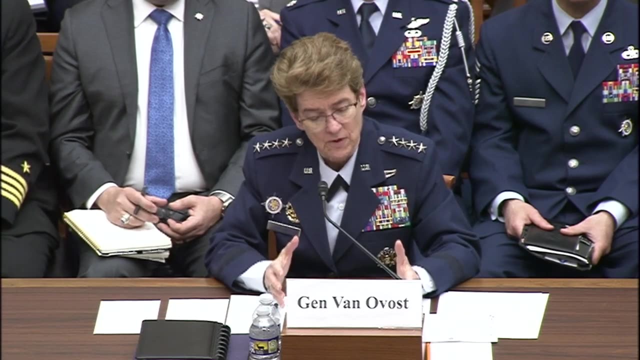 to our operations in the Pacific. So thank you for your leadership out there and thank the committee for the support of the infrastructure and resiliency work that we're doing out there right now. So Guam is critical And the Navy port, Navy seaport of Guam is critical for us for a lot of our deployment requirements. 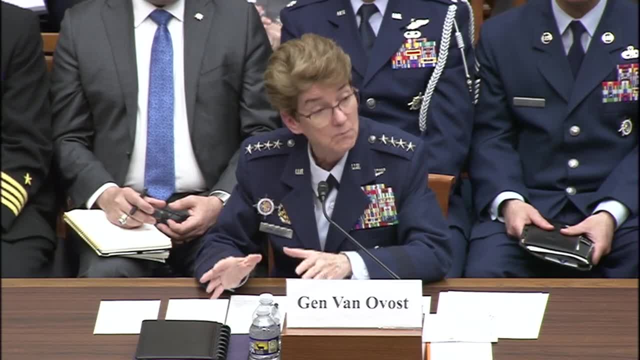 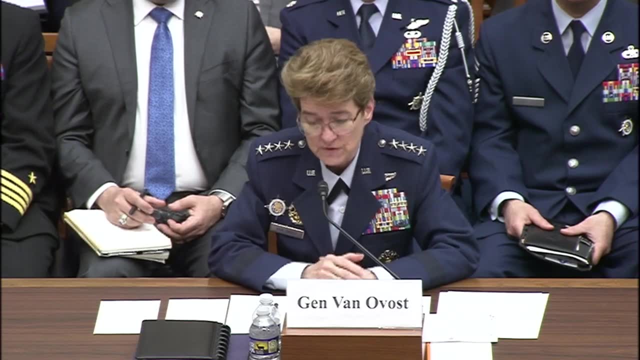 And then the civilian side of the port has been important for our sustainment, if you will, and construction materials, which are really critical again right now, as we're bolstering our posture and helping the services and our allies and partners come out there and get settled in. 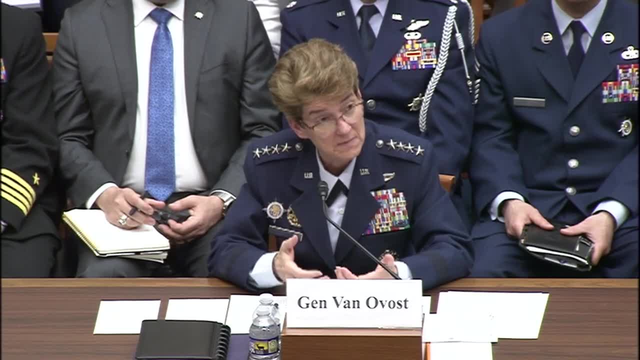 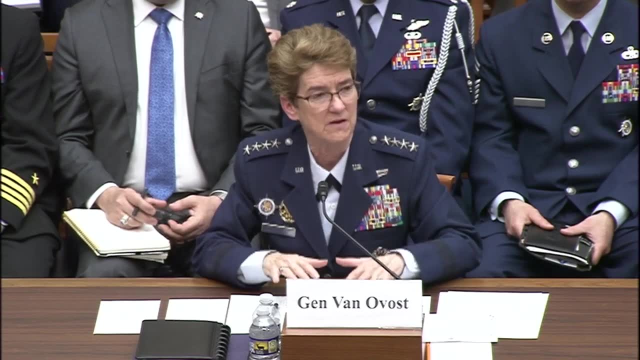 So I think about Guam all the time. In fact, there's a new two-star commander that's going to roll out and be responsible for integrating all of those projects together. I look forward to working with him or her on how do we help to ensure that we can phase in? 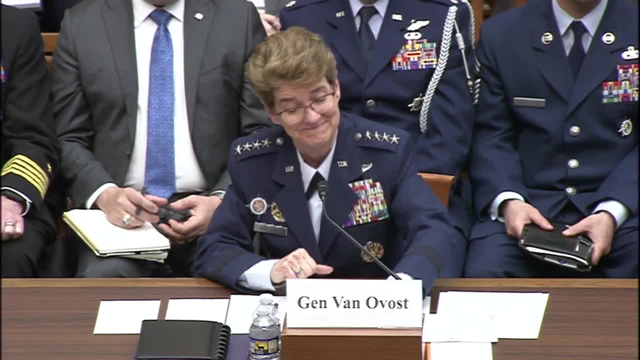 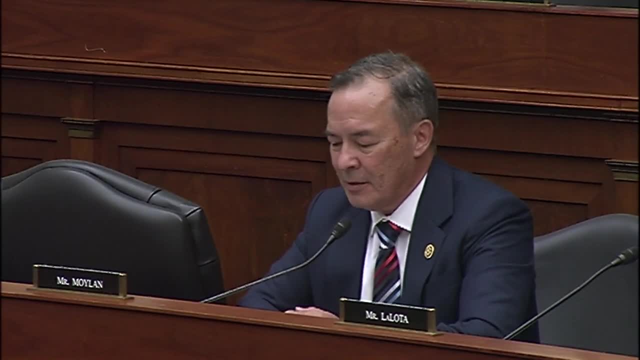 and meet the requirements of the buildup there, Thank you. And the new general is the one star that's dubbed up. Hoffman will continue on there with his family, So that's wonderful. Along with that line there's two pieces of infrastructure I'm concerned about. 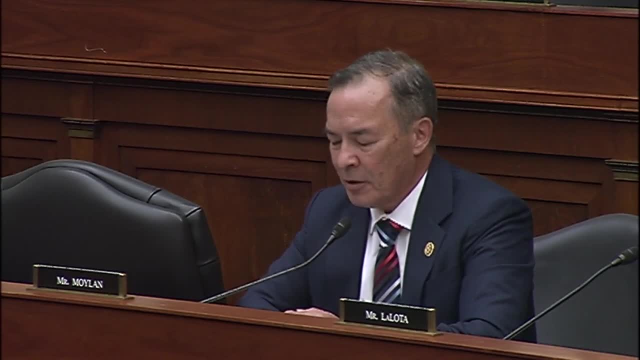 to include the port of Guam's gantry cranes, which are in need of replacement, and the harbor's breakwater, which reportedly, one more typhoon could destroy. If these two pieces of infrastructure fail, the people of Guam could lose access to commercial shipping. 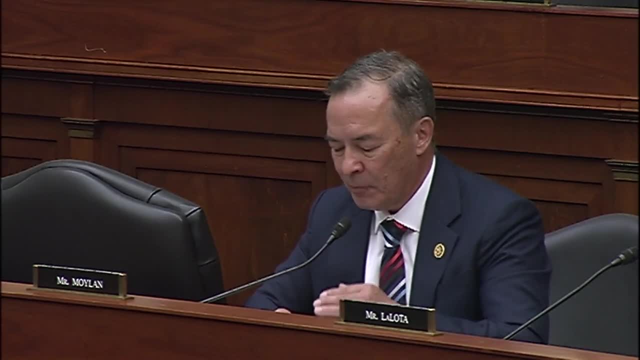 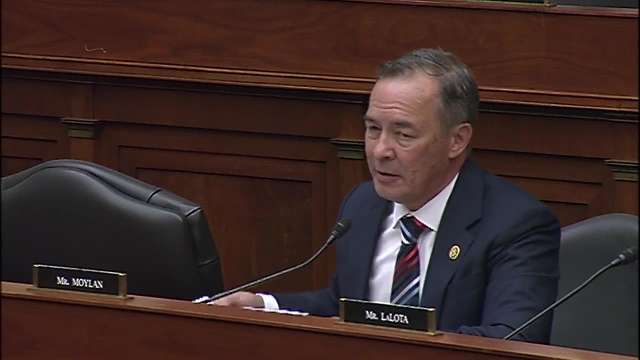 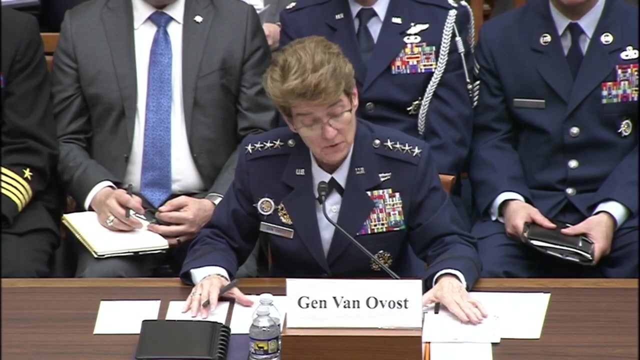 Considering that approximately 40% of cargo moving through the port of Guam is for the military, how is the Department of Defense will be impacted by this infrastructure deterioration? Certainly, we like resilient options with respect to berthing and where the cranes are the Navy port and the civilian side of the port. 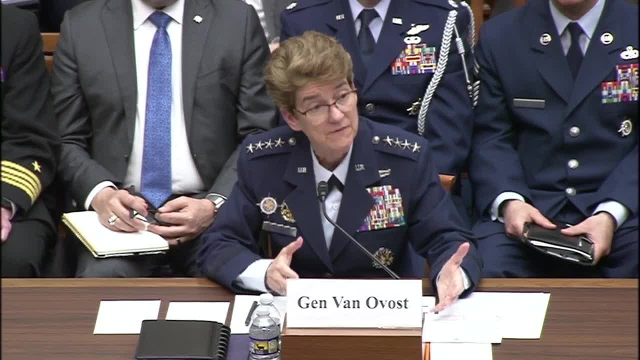 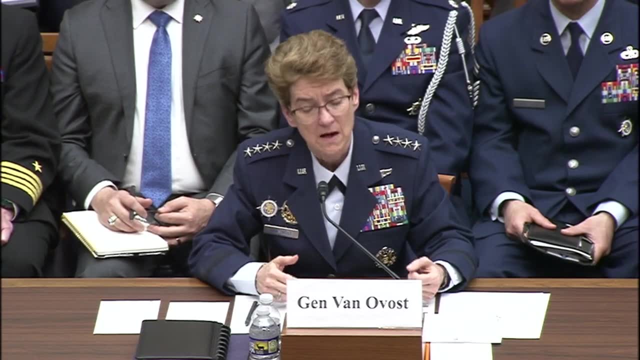 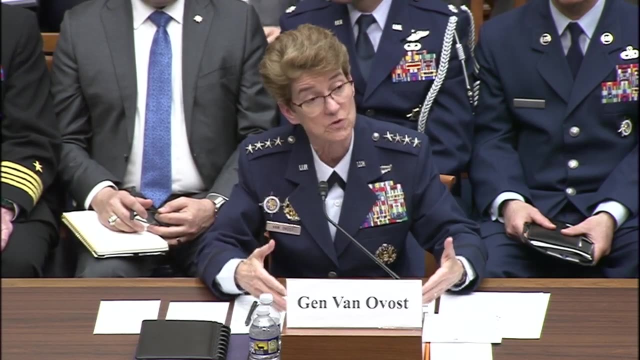 As you know, the Department of Defense does not fund the infrastructure. on the civilian side. I turn to our maritime administration partners for opportunities for loans, because essentially we get billed to use those things. It's that money that goes back. It goes back to reinforce and reinvestment, supposedly by the civilian contractors. 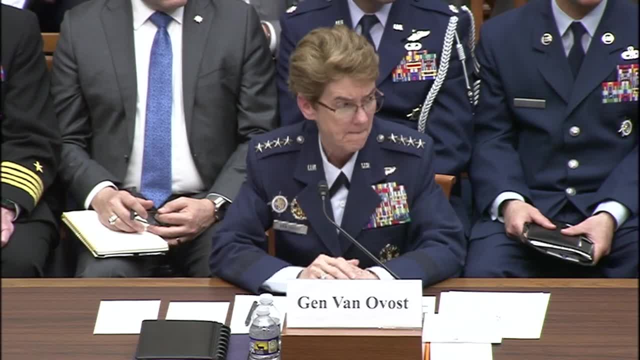 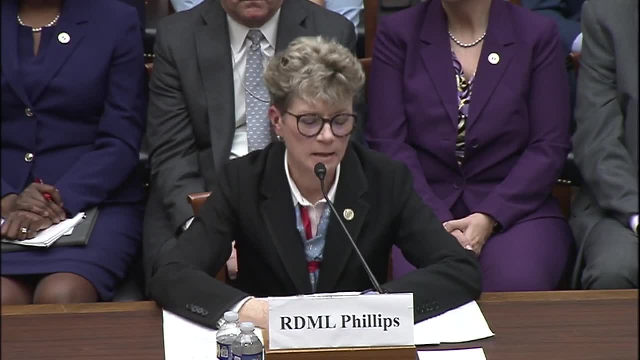 So I defer to Admiral Phillips. Thank you, ma'am Congressman. thank you. We have received letters from the governor on the topics you are mentioning exactly, and we have also been visited by GovGuam and Port of Guam staff many times. 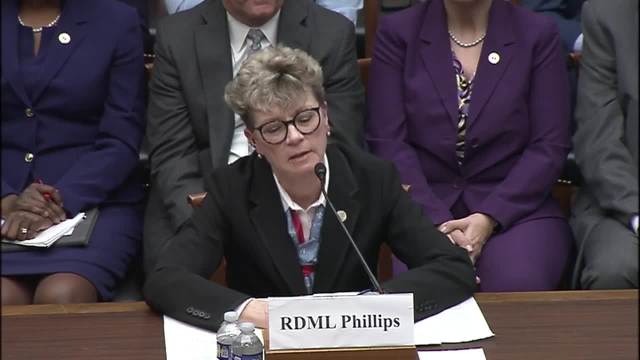 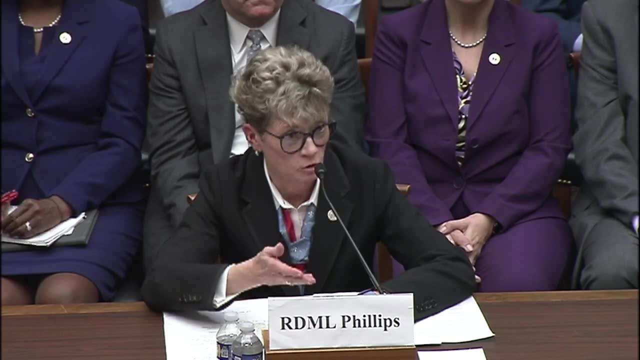 I see them often at AAPA and I thank them for their interest and their visits. As you're aware, we have a discretionary grant program, Port Infrastructure Development Program, which is an opportunity for Guam. They are a strategic port so they are a part of that process as well.